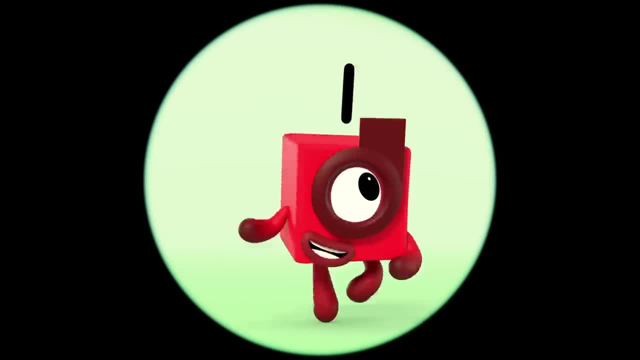 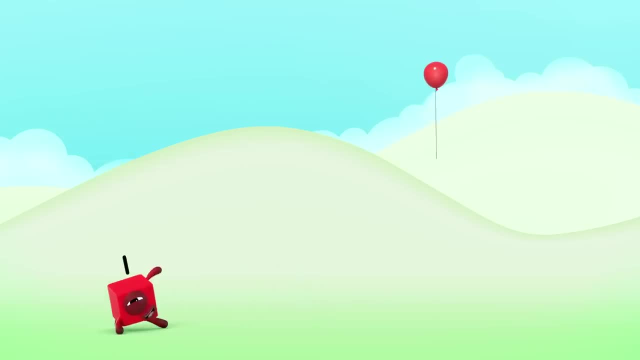 Ooh me, A Step Squad. all by myself, I'll give it a go. Oh, Step one, chase the balloon. My plan is working perfectly: Hush, hush. One plus two equals Three. One, two, three, Three escaped balloons. 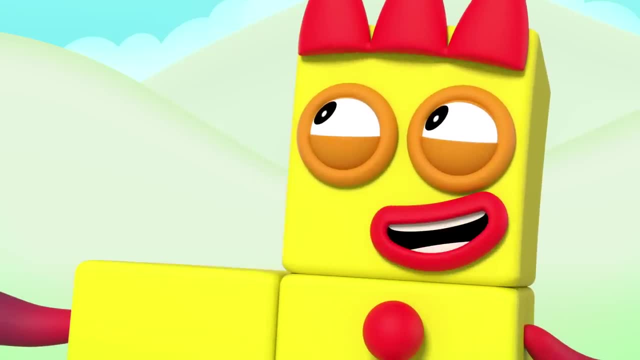 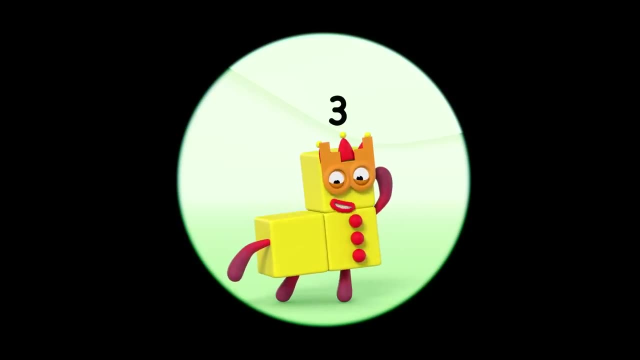 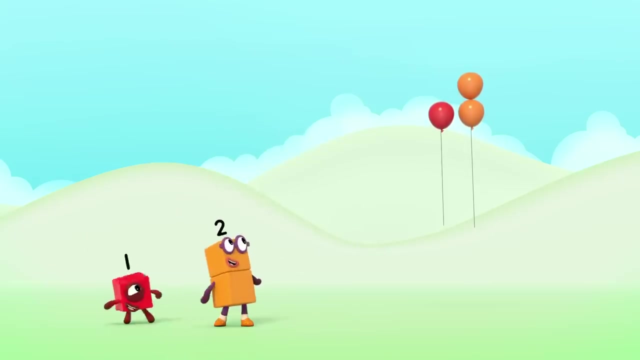 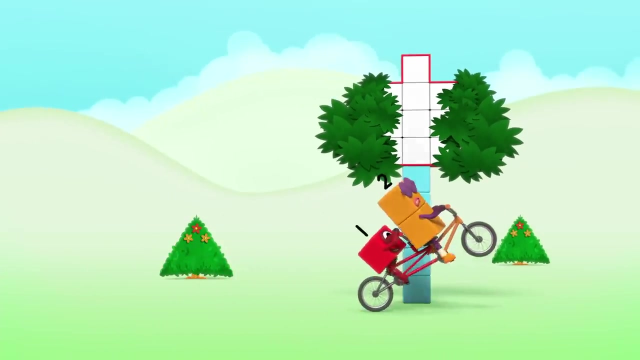 If only Step Squad were here. The super special secret Step Squad is here. Look at me, I'm step-shaped too. Maybe I can be a Step Squad. Step one: chase, Step two: peddling hard, Hush, hush. 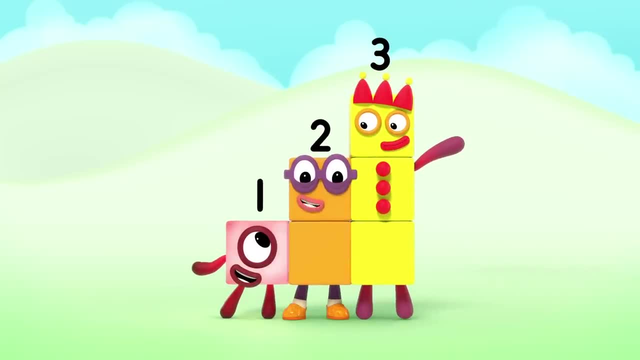 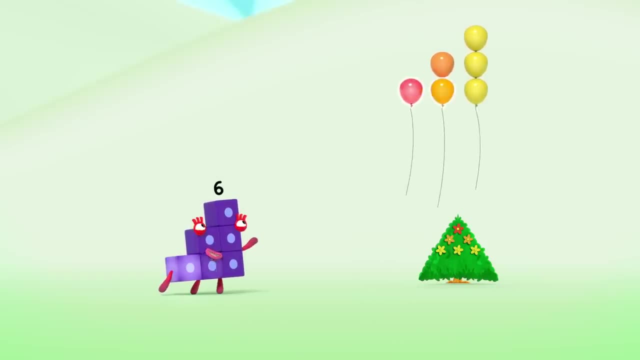 Look out: One plus two plus three equals Six. One, two, three, four, five, six, Six balloons have now been freed. I know exactly who we need. The super special secret Step Squad is here. Look at that. 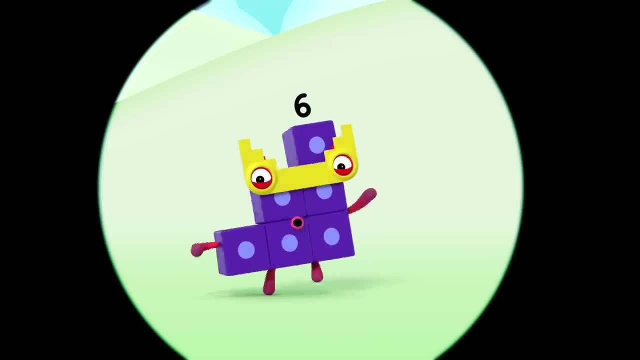 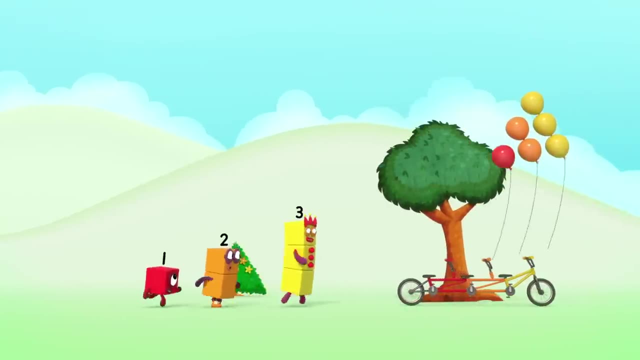 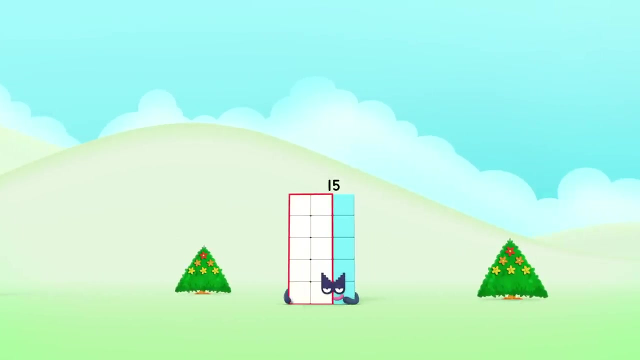 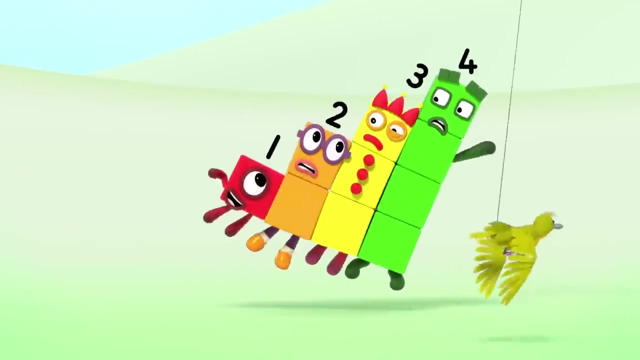 It must be true, I can be a Step Squad too. Step one, chase. Step two, peddling hard. Step three with a net, Hush, hush, Hey, Whoa. One plus two Plus three Plus four equals. 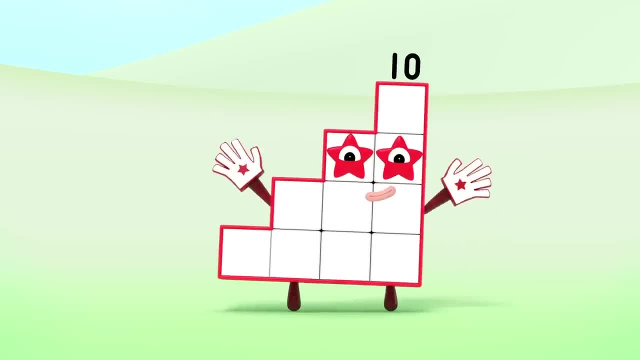 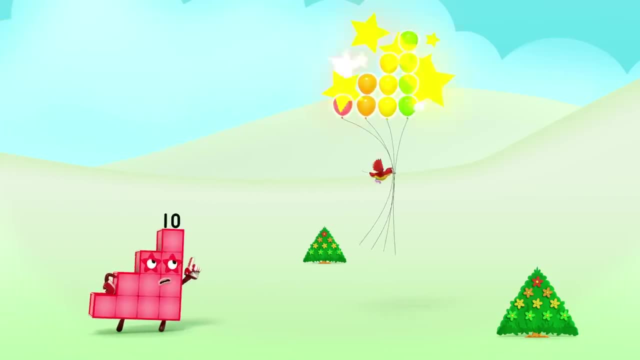 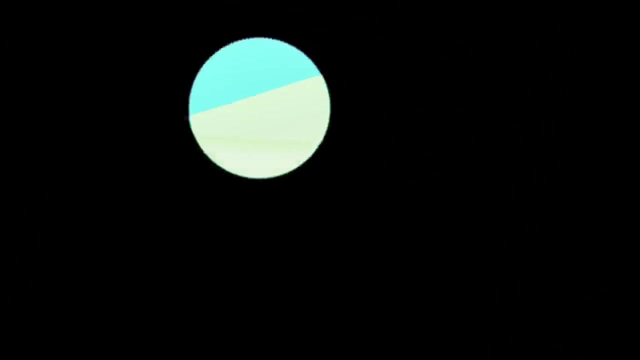 Plus four equals Ten. You, naughty bird, You bring those one, two, three, four, five, six, seven, eight, nine, ten, Ten balloons back. I need Step Squad, The super special secret. Step Squad is here. 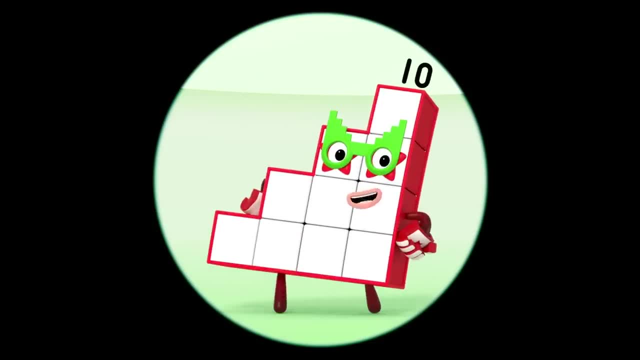 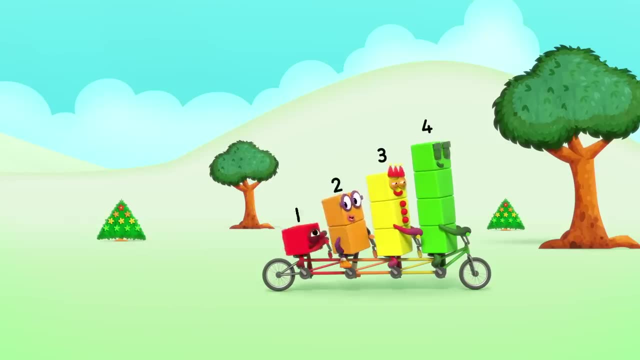 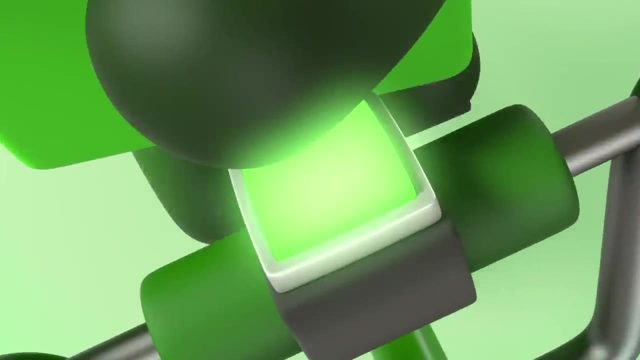 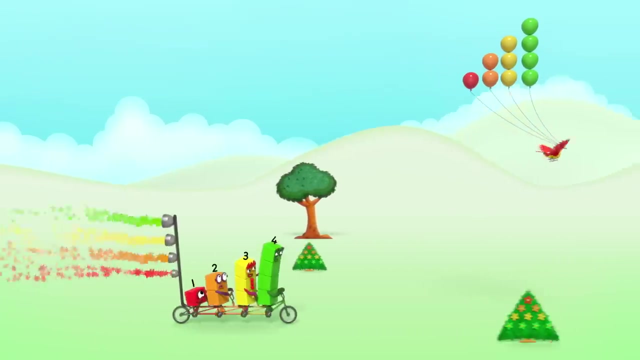 Can it be? Yes, it can. I'm a Step Squad too. Step one: chase. Step two: peddling hard. Step three with a net. Step four: press the square button. Whoa Hush hush. 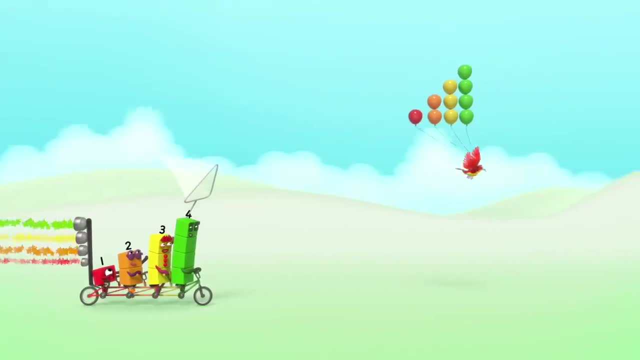 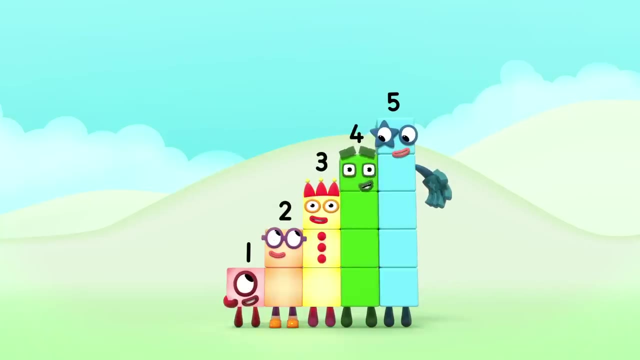 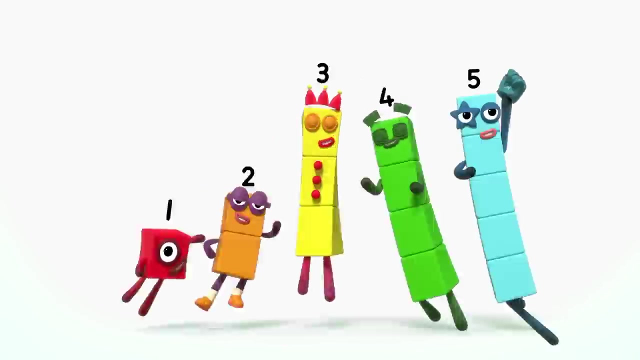 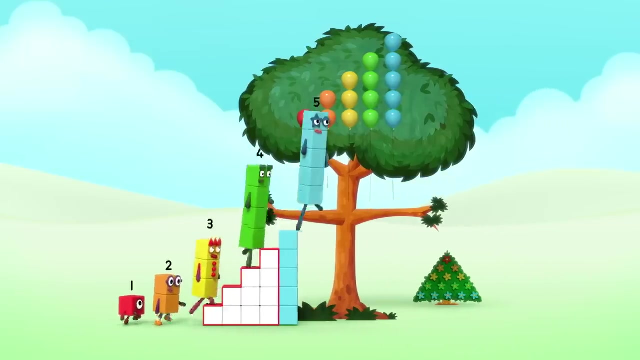 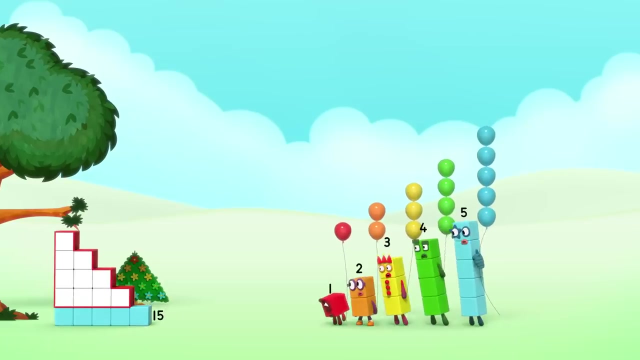 Grab them, Whoa. One Plus two Plus three Plus four Plus five Equals Fifteen. The super special secret Step Squad is here. Step Squad up the steps, Step Squad down the steps. Agent Fifteen. 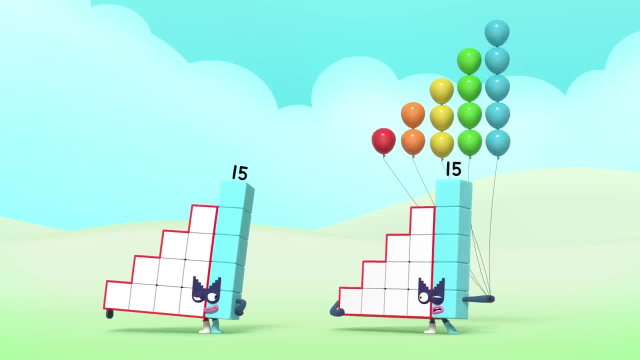 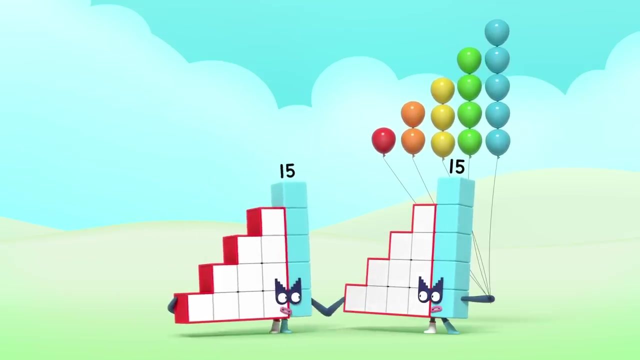 Does this make me a double agent? You passed my test with flying colors: Red, orange, yellow, green and blue. Well done all of you. All of us, All of you, Step Squads Fifteen. you're a Step Squad. 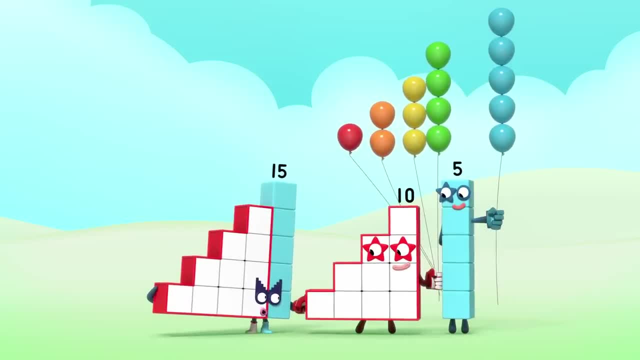 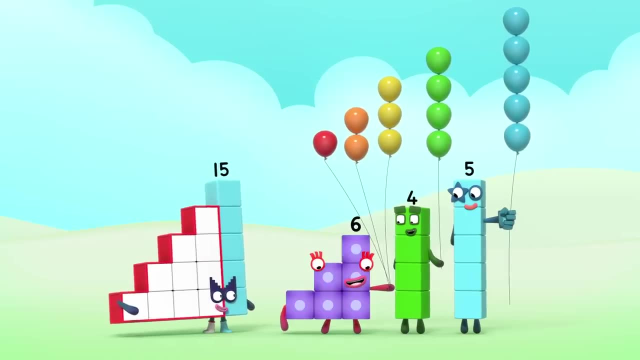 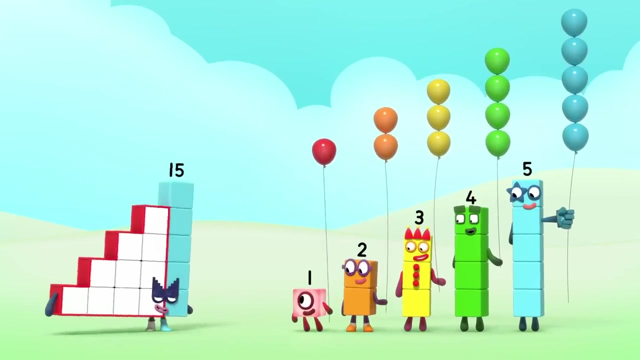 And ten. you're a Step Squad too. One, two, three and four. Six, you're a Step Squad. One, two and three And three. you're a Step Squad. One plus two And one. you fit the pattern. 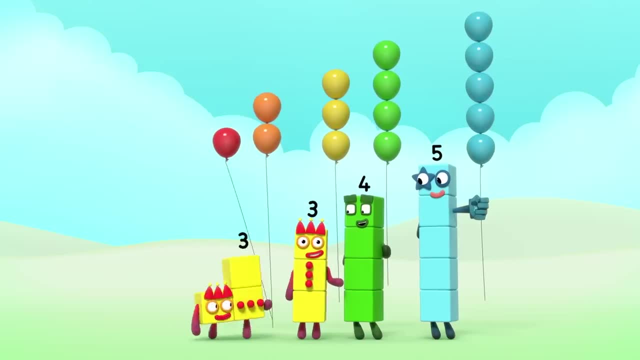 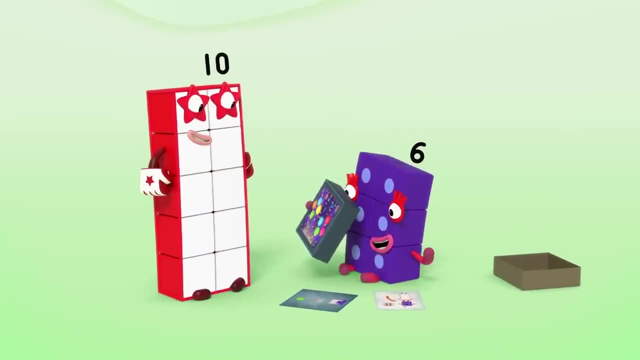 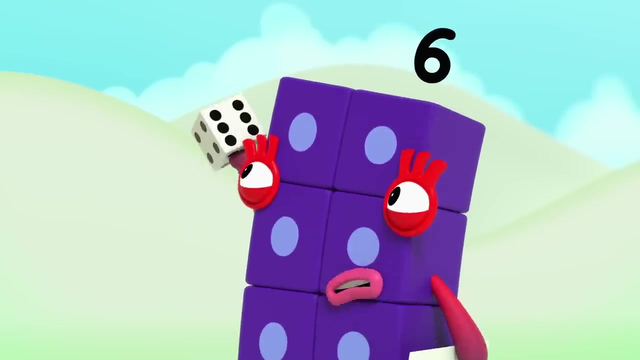 So you're a Step Squad as well. One, three, six, ten, fifteen. Step Squad. It's late to play my new game. It's called Party in a Box. Ooh, First roll the dice, Let's roll. 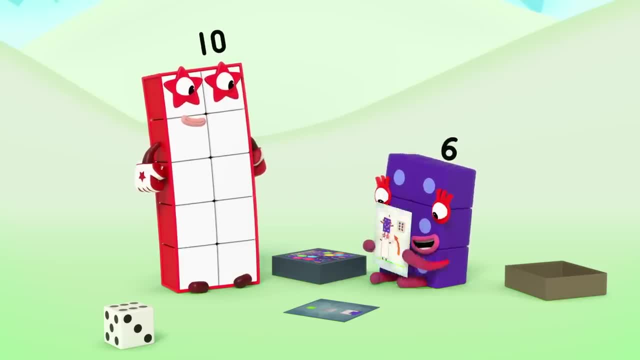 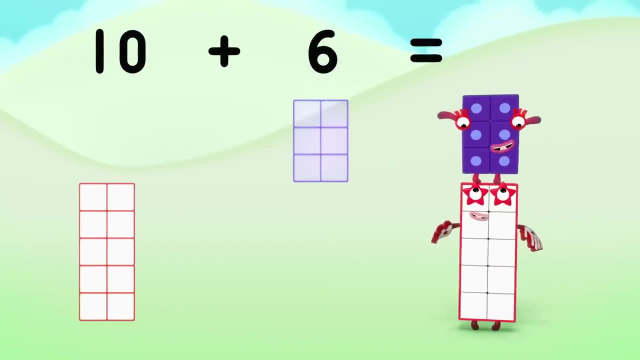 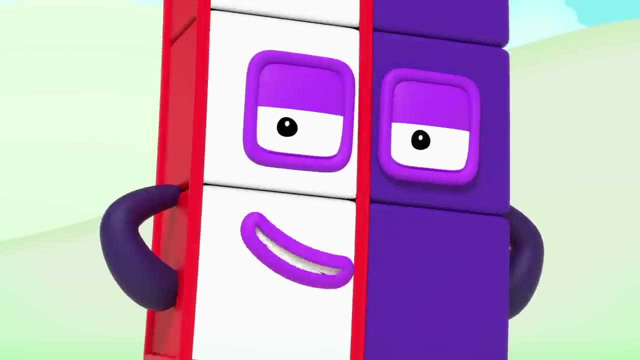 Six. If you roll a six, jump on your friend's shoulders. Hmm, Ten plus six equals Sixteen. Oh look, here I am then. Well, that's nice, isn't it? Right, then let's get on with it. see what shapes I can make. 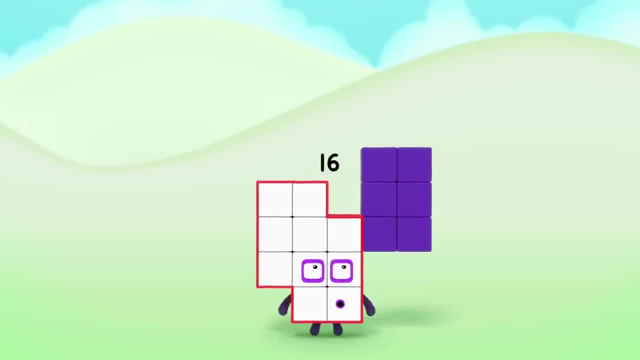 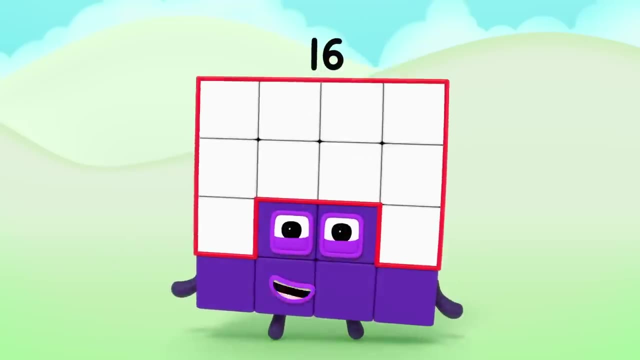 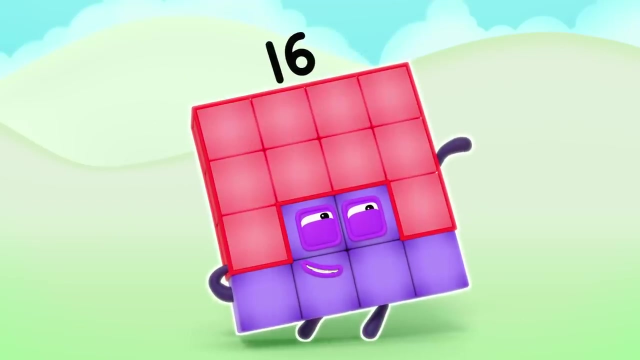 Yeah, Hmm, Ooh, Um, Aha, Oh, oh, no, no way, I can't believe it. I'm so excited. Guess what? I am sixteen And I am a square. Woo-hoo, Right then, what do squares do? 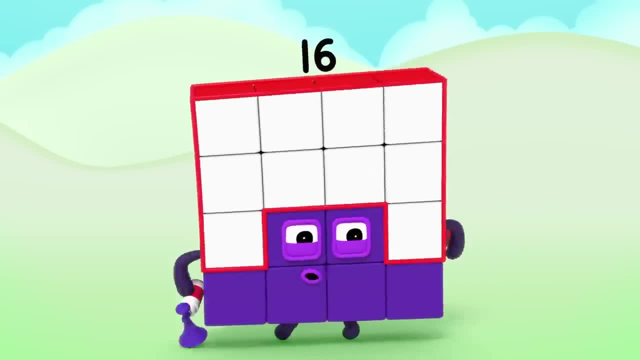 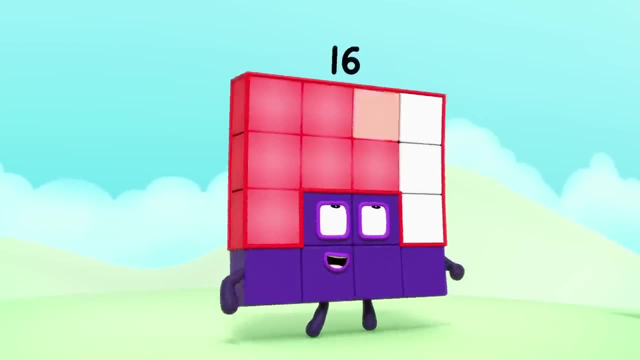 I bet it's really amazing. Wait, no, let me guess I know Square party One, two, three, four, five, six, seven, eight, nine, ten, 11,, 12,, 13,, 14,, 15,, 16.. 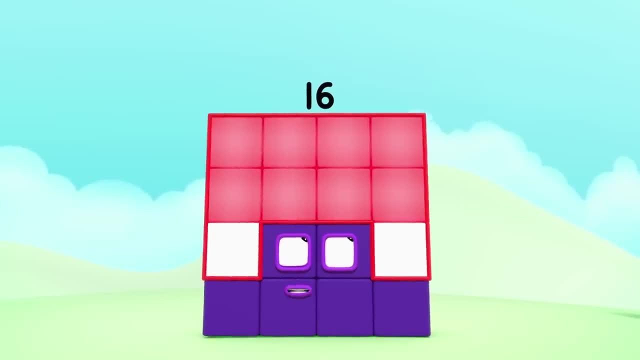 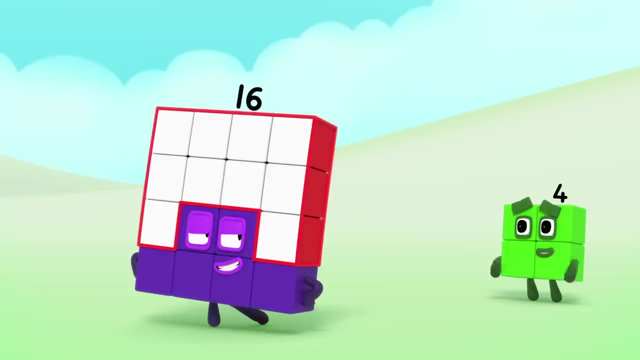 I am. sixteen, Square is a box And guess what? I've got 16 blocks Square, A really big square. Sixteen, Ten and six. I like this game. Sixteen, Ten and six, Party Sixteen. 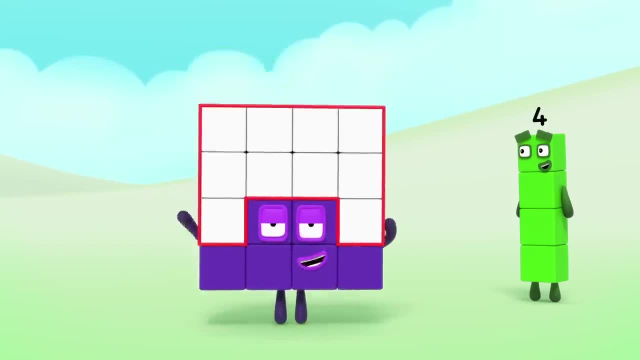 I am sixteen, I'm ten and six And I've got loads of party tricks. Two, one, two, three, four. I'm a big, big square. I knew you would All right, Here we go. Five, six, seven, eight, nine. 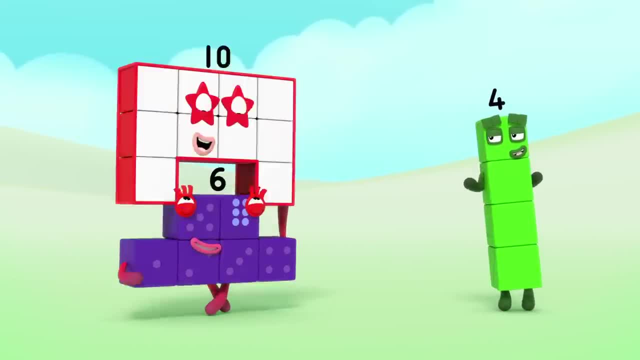 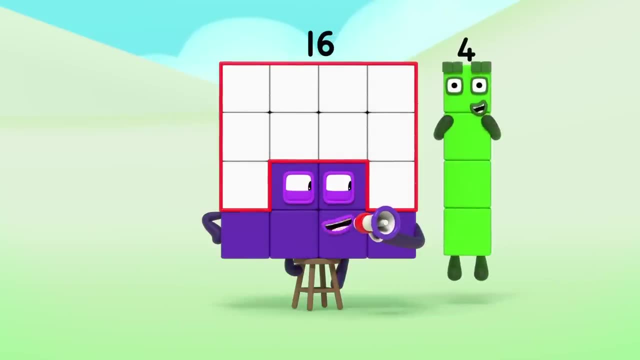 One, two, three, four, Hi Six. Oh no, Okay, You are the big square Party tricks. Lie down, stand up, Lie down, stand up, Lie down, stand up, Keep going. Four by four, four by four, Four by four. 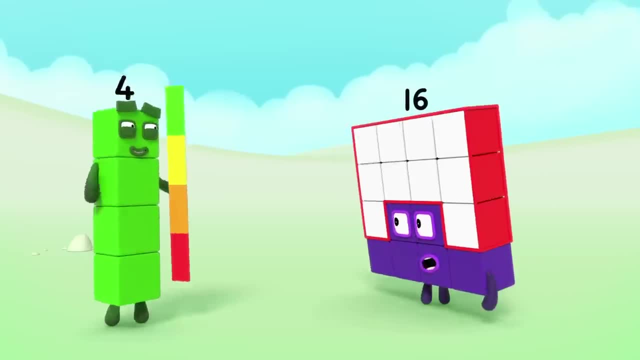 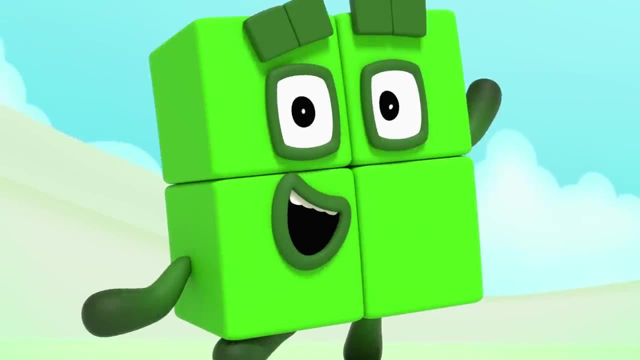 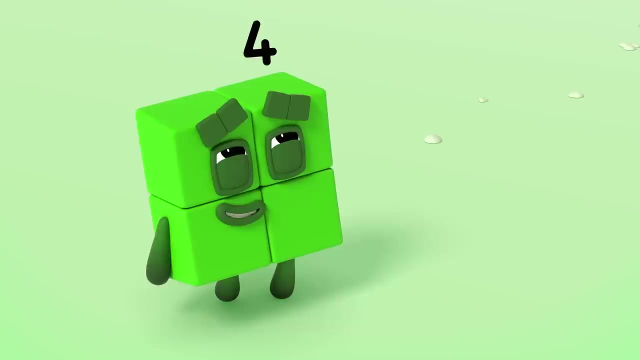 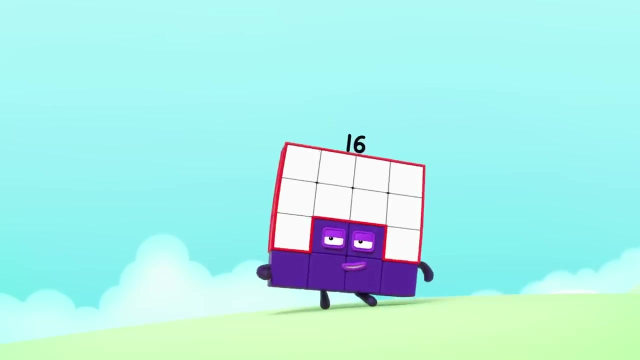 I am a square, Are you sure? Of course I am. I'm four by four, Sixteen. I have four columns And four rows. Four, lots of four. I'm four of those. A square made of squares. We can do the splits: Four fours, Four fours, Four fours. 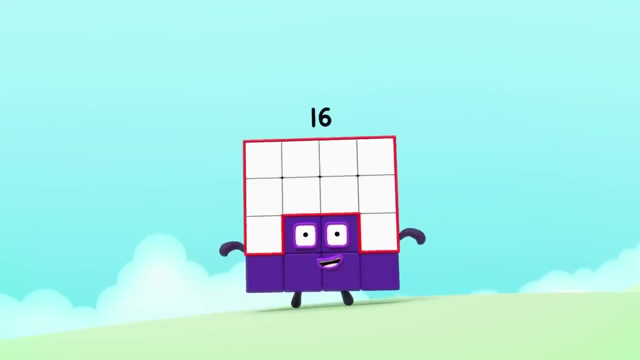 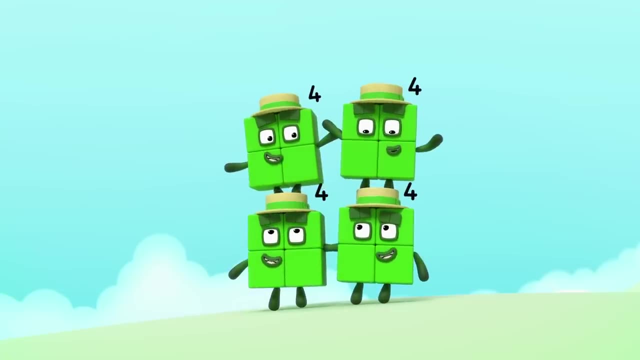 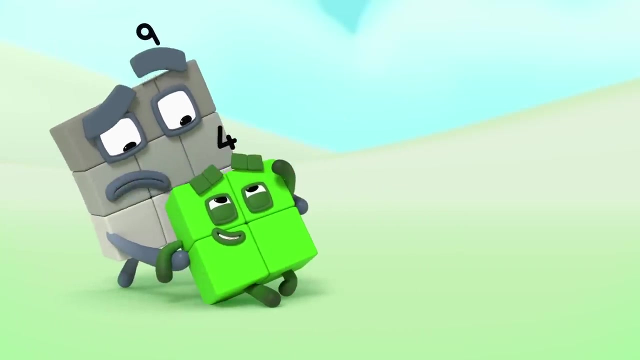 Sixteen Still here. One, two, three, four, Four fours. One, two, three, four, Four fours. One, two, three, four, Four, fours. You know what four, fours are. Sixteen, Oh, um, it's all right. four, It's only a really big square. 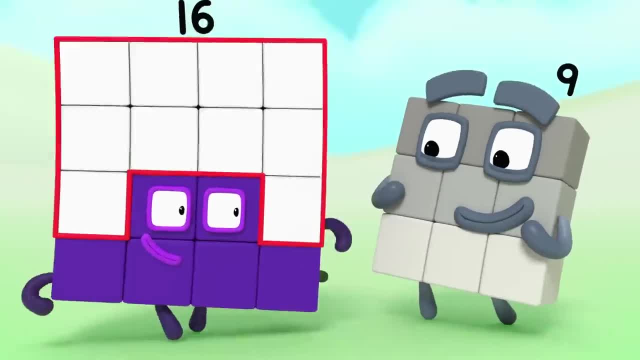 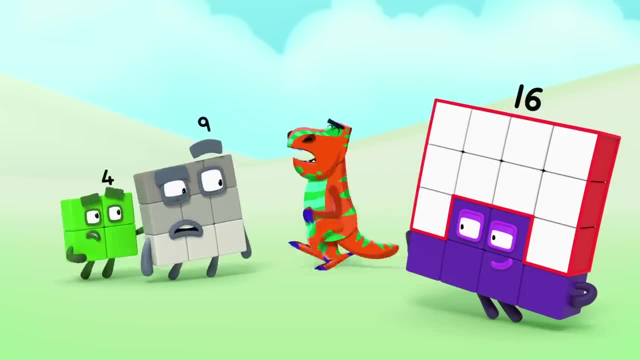 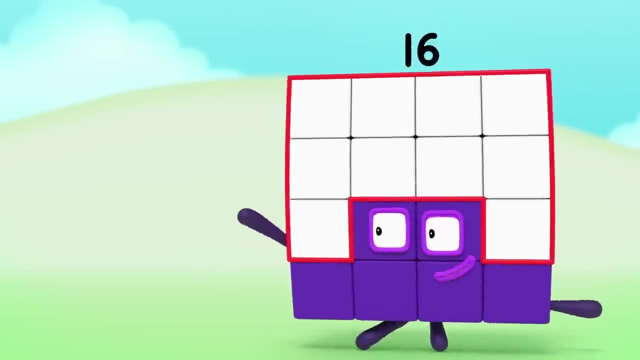 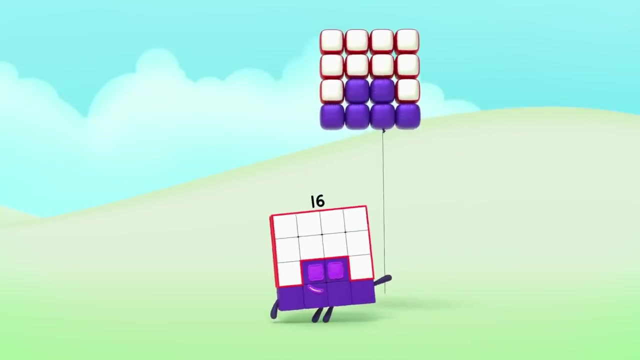 Wow, I am sixteen. I'm four by four. I'm larger than a dinosaur. Well, Well, Well Later. Rexy, I am sixteen. I mean no trouble, But have you seen me? Bob and Devil, No Alone. Sixteen. I'm going to split in half now. 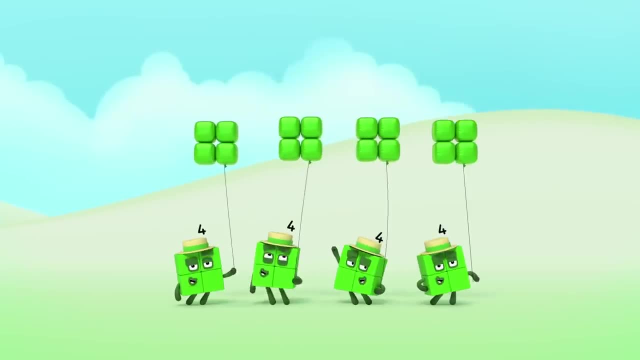 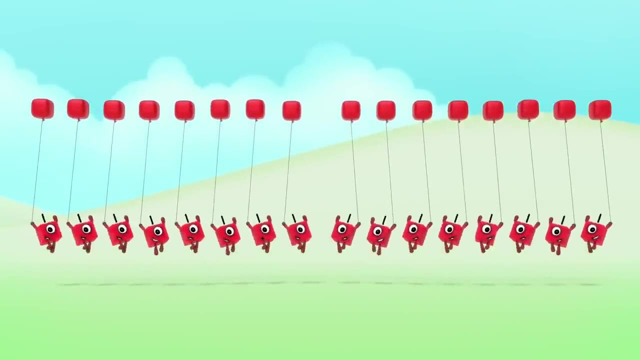 Two, eights. We're going to split in half now Four, fours. We're going to split in half now Eight, twos. We're going to split in half now Sixteen ones. Hooray, We're going to double up now. Eight twos. We're going to double up now. 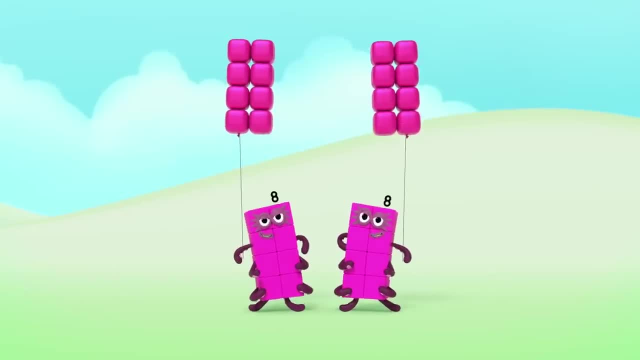 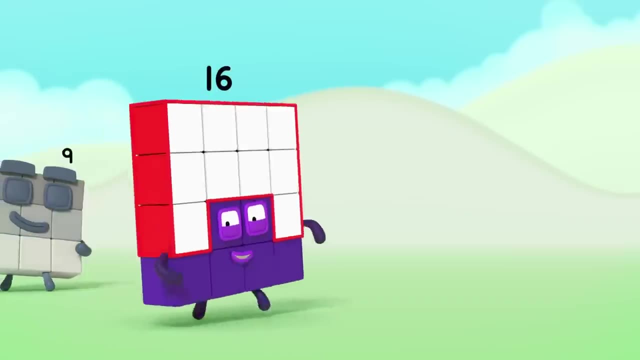 Four, fours, We're going to double up now Two. eights, We're going to double up now Sixteen, I'm going to- Ow, it's me silly. Do-do-de-do, do-de-do, do-de-do, do-do-de-do. Well, come on then. 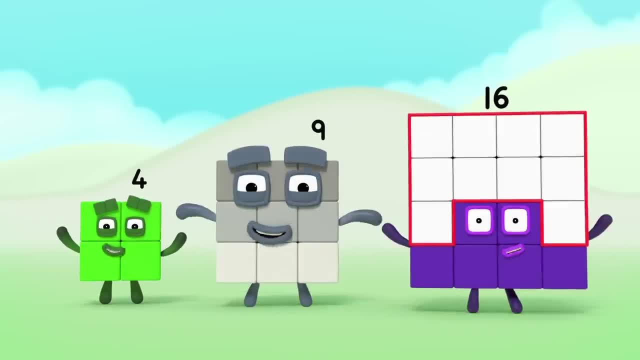 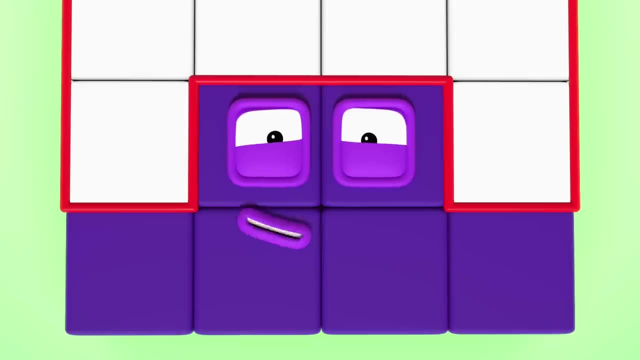 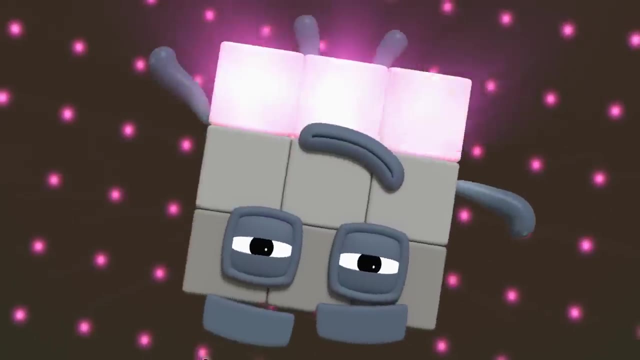 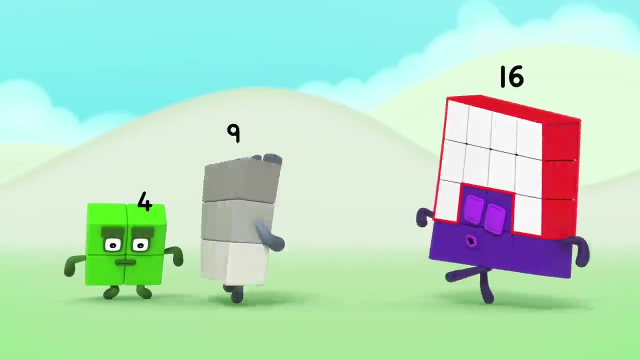 Hmm, Square dance, Square dance, Disco floor. I am the square, I am the square. Freestyle: Do-do-do-do, do-do-do, do-do-do, do-do-do, do-do-do, do-do-do, Huh, Huh. 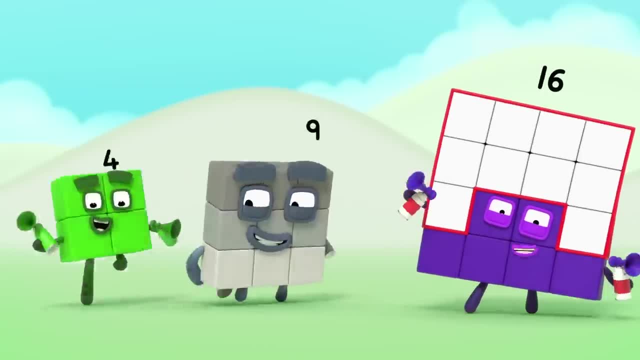 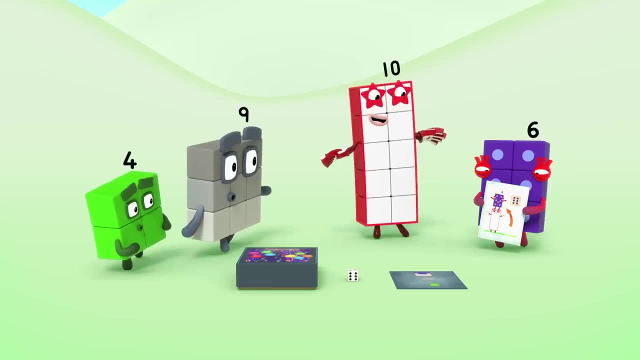 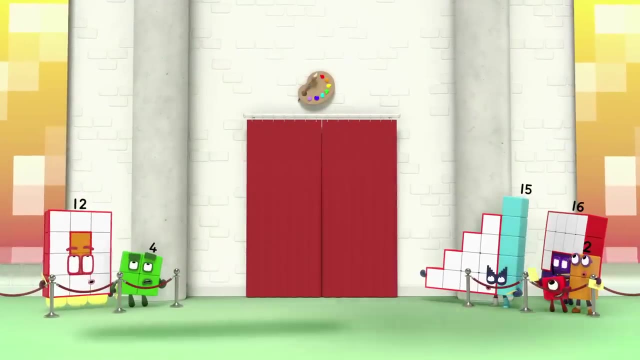 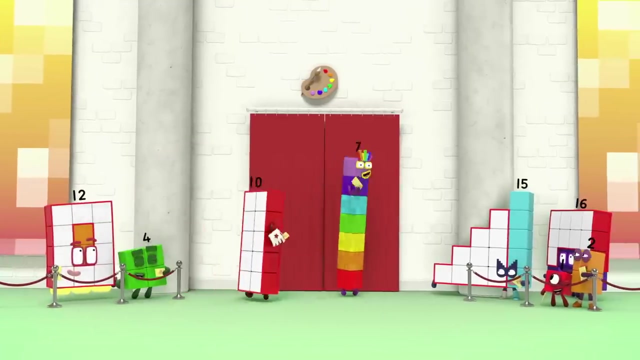 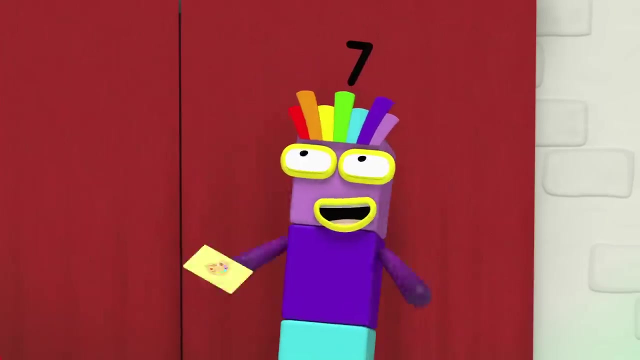 Square party, Square party, Square. Now that's what I call a party game. Thanks for the lift Ten. Are we in time? Yes, Just about. That's lucky. I wouldn't miss the opening of Numberland's first art gallery for the world. 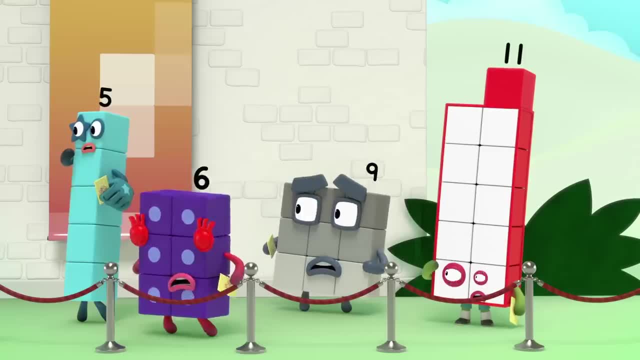 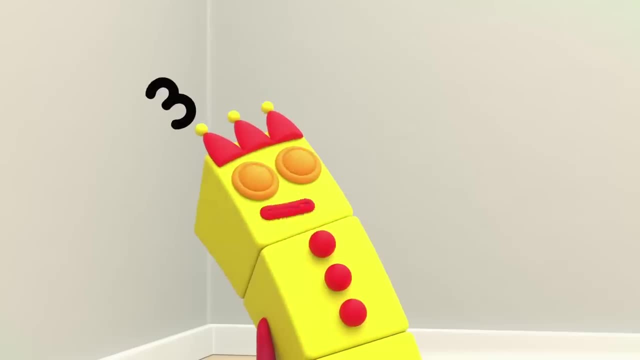 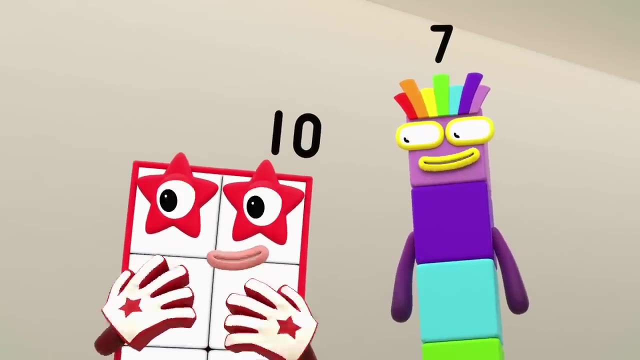 You and you. I like it, but where's the art? I spent so long making sparkly invitations. I forgot to get any. Ooh, Can we, Can we help? I thought you'd never ask. Are you sure you're a rocket? 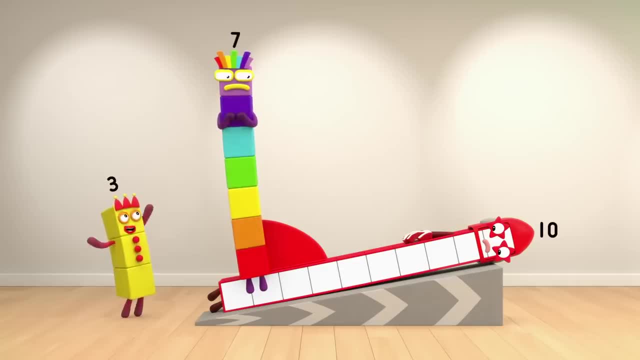 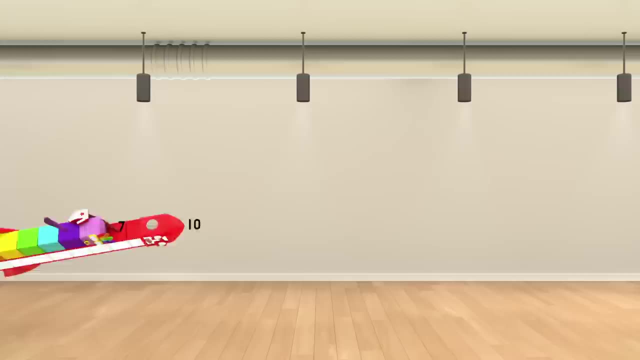 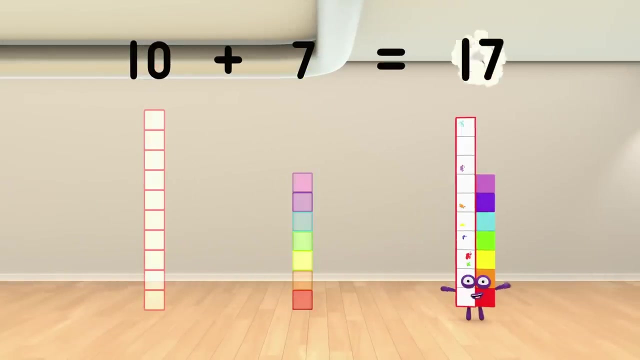 You're full of colours, Fly through the museum and make art, But No, Ten, nine, eight, seven, six, five, four, three, two, one stop Whoa. Ten plus seven equals Seventeen. 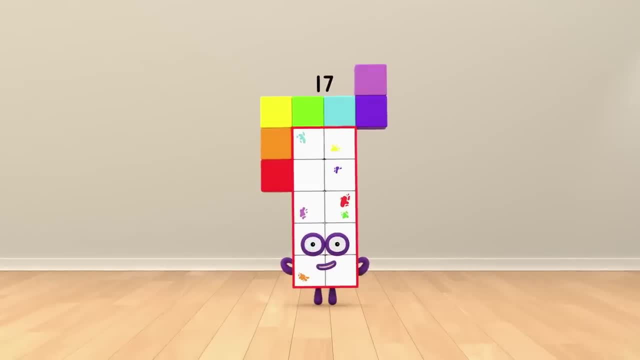 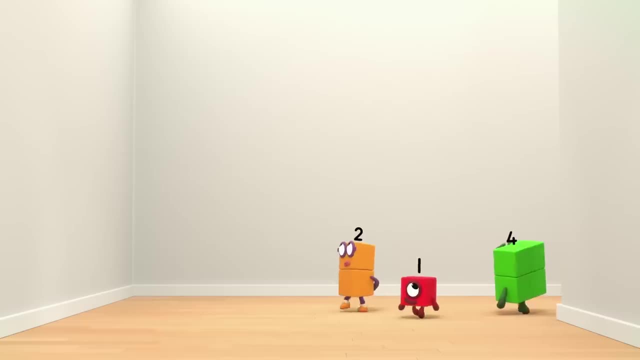 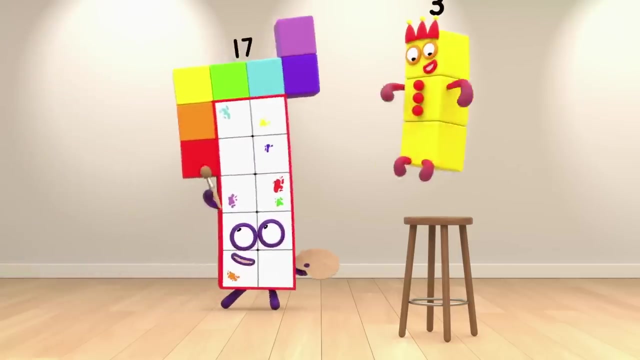 Ooh, Now there's a surprise. I am seventeen and I love to paint. They're coming in. Oh Go, go, go, Don't mind if I do. Some painters only paint portraits. Majestic and serene, I can also paint portraits. 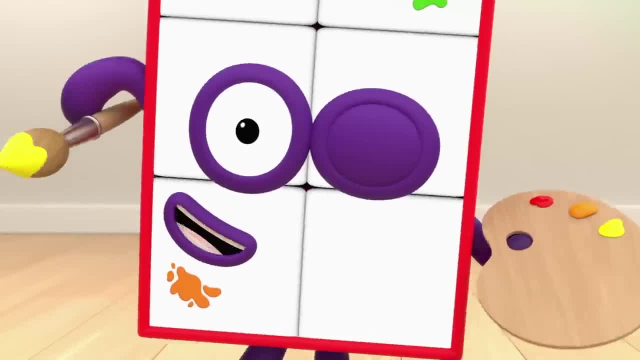 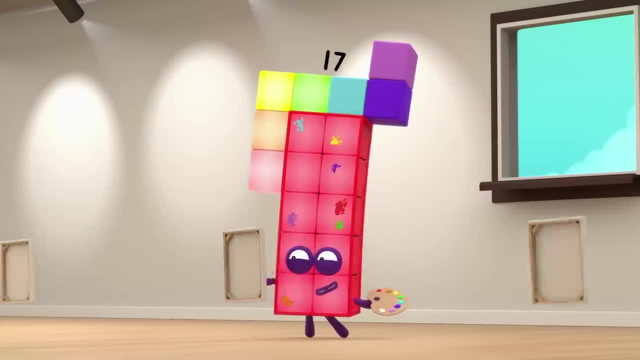 But I paint seventeen, One, two, three, four, five, six, seven, eight, Nine, ten, eleven, twelve, thirteen, fourteen, fifteen, sixteen, seventeen. Look at me, Blue, No, Blue, Look at me. 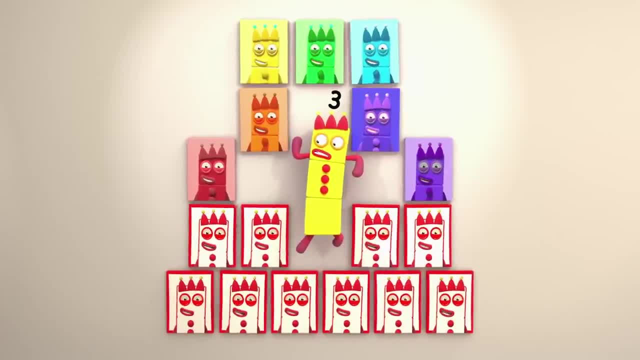 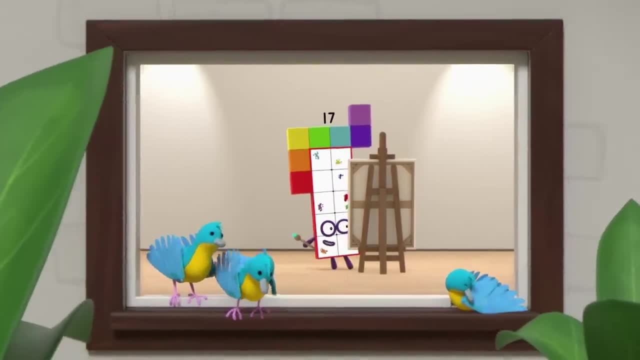 Hmm, Nice Juxtaposition. Some painters like to paint bluebirds In a lovely nature scene. I paint only a few birds When I paint seventeen, Ten and seven, Seventeen, Ooh, Hey, Oh, Hey, Oh, Hey, Hey. 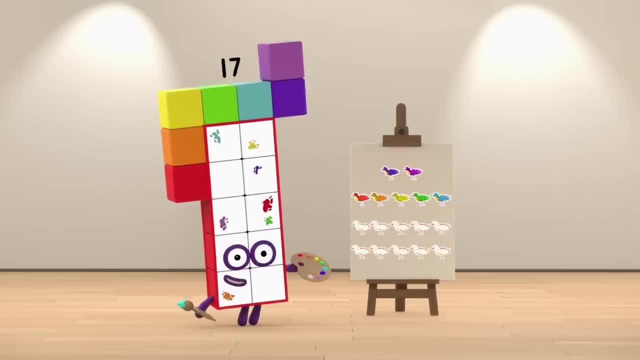 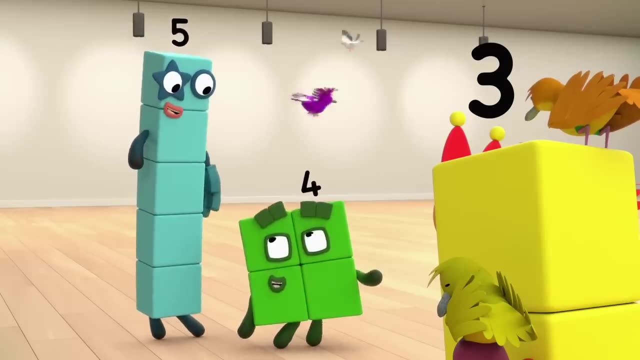 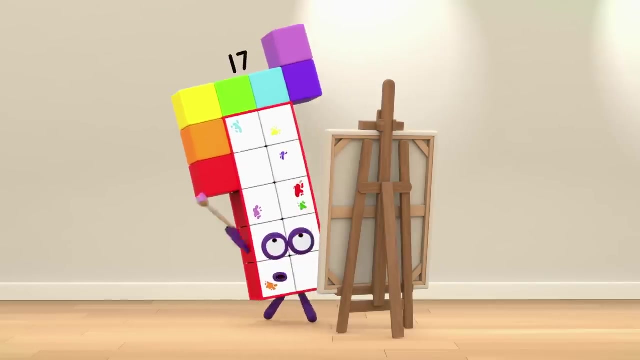 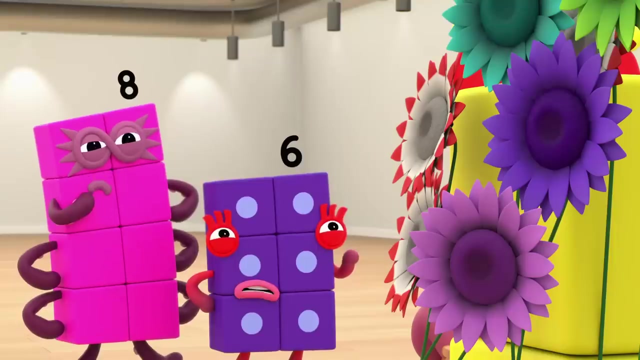 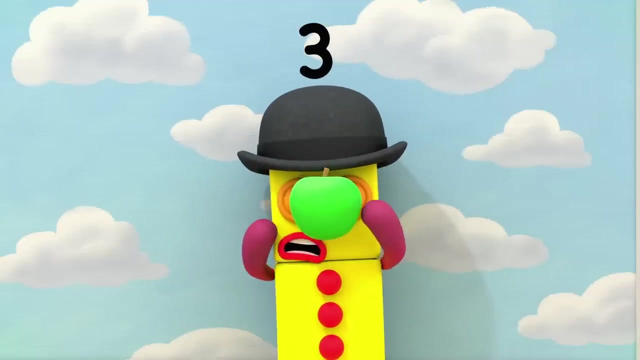 Ooh, Ooh, Ooh, Ooh, Oh, Oh, Oh, Oh Oh. Some painters paint flowers. they look so sublime. I paint for hours. seventeen of everything takes time. What Nice juxtaposition. Some painters like to paint apples in brilliant shades of green. 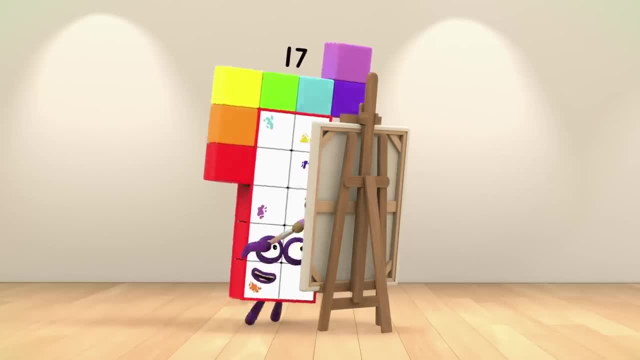 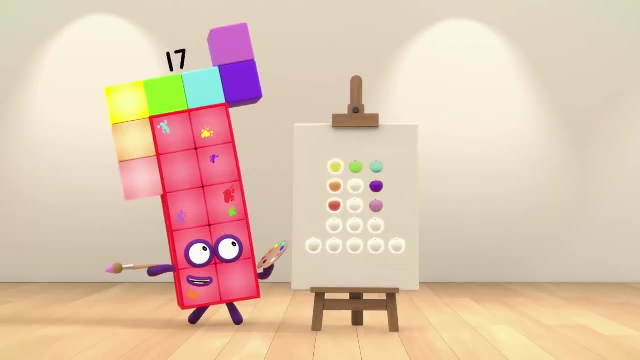 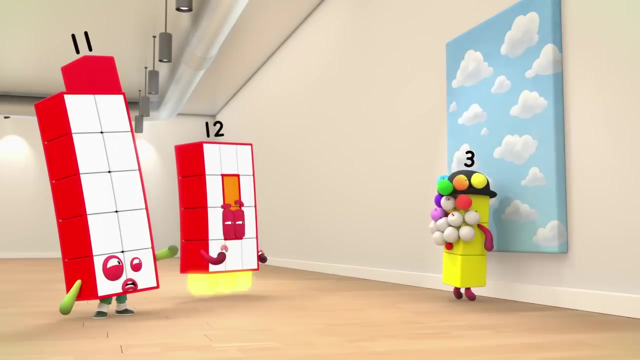 I can also paint apples, but I paint seventeen. One, two, three, four, five, six, seven, eight, nine, ten, Eleven, twelve, thirteen, fourteen, fifteen, sixteen, seventeen. Hey, no, get off, silly apple. 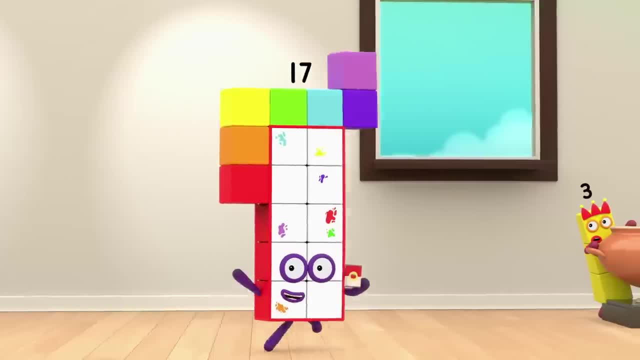 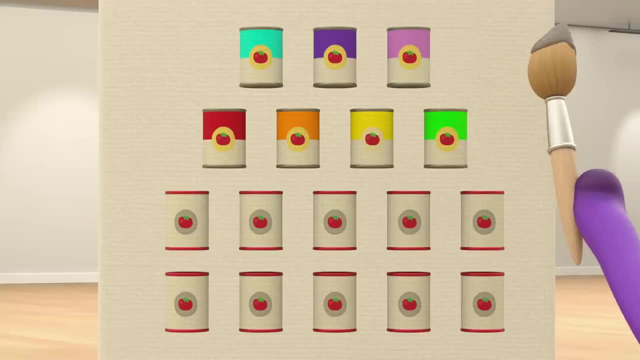 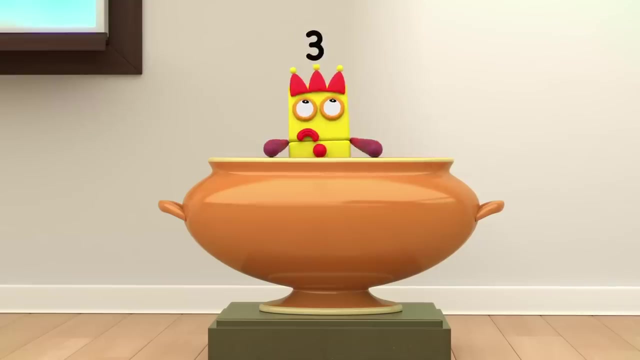 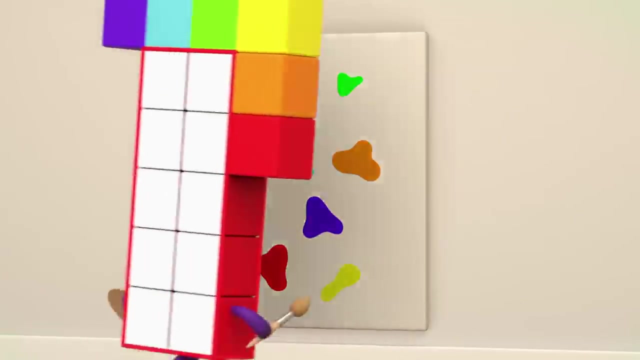 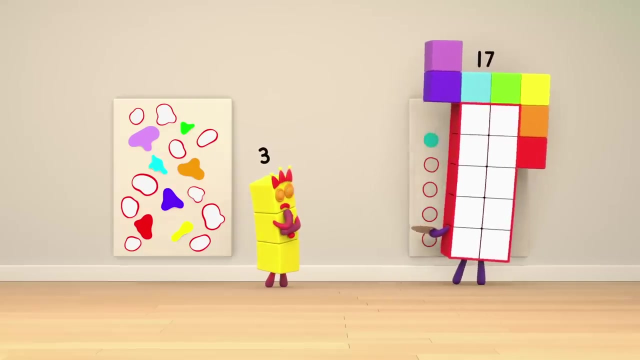 Nice juxtaposition. Some painters like to paint soup cans. I like a whole tureen, So I paint plenty of soup cans. I paint seventeen, Ten and seven, seventeen. I'm a student, Nice juxtaposition. Some painters paint splatters, some painters paint dots. My number's. what matters, seventeen, is lots and lots of spots. 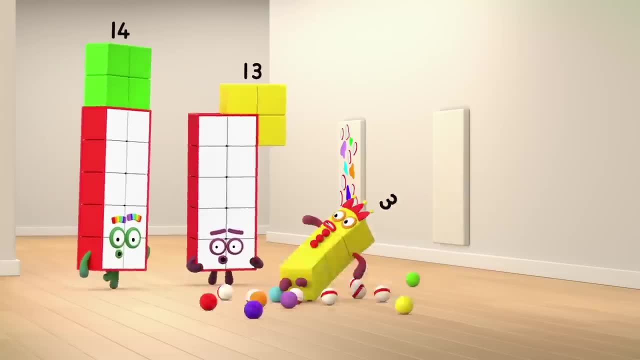 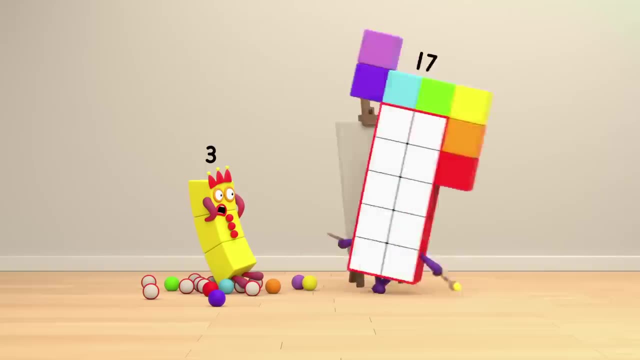 Oh, nice juxtaposition. Hold that pose. Some painters like to paint soup cans. I like a whole tureen. Some painters like to paint faces that look like they might scream. I can also paint faces, but I paint seventeen. One, two, three, four, five, six, seven, eight, nine, ten. 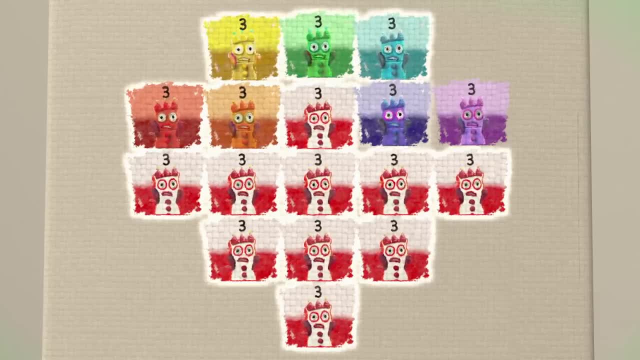 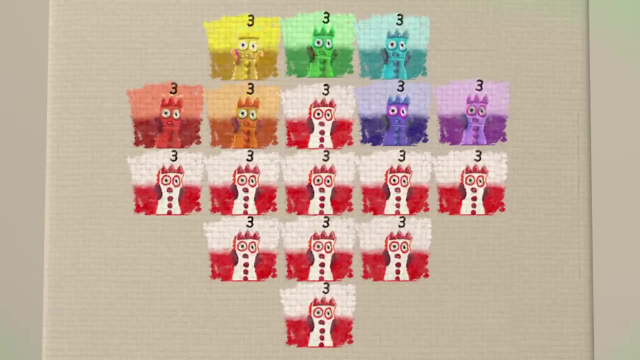 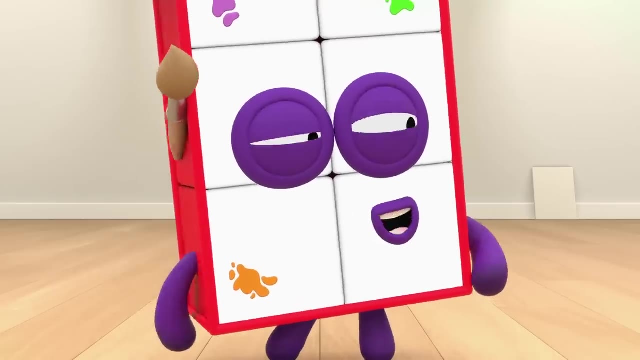 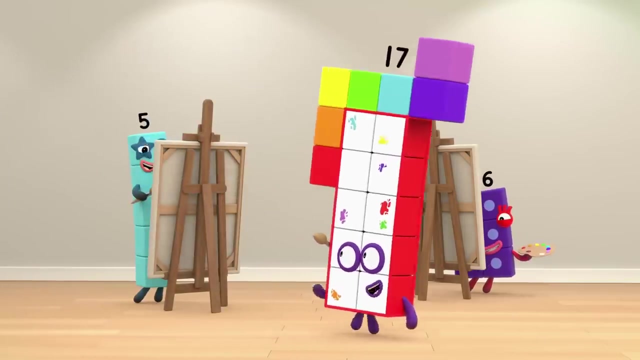 Eleven, twelve, thirteen, fourteen, fifteen, sixteen, seventeen. I scream, you scream, we all scream for ice cream. Yummy, Wait, I know what this gallery needs: Your art. Let your imagination play. Paint what you want, go your own way. A piece of paper's purpose is to be a picture one day. 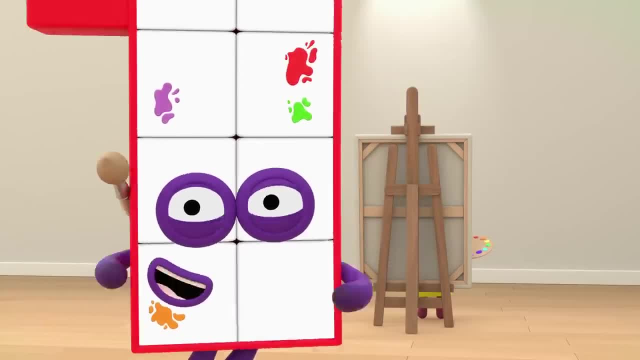 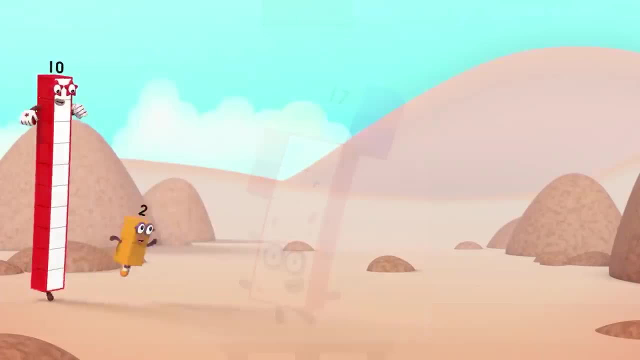 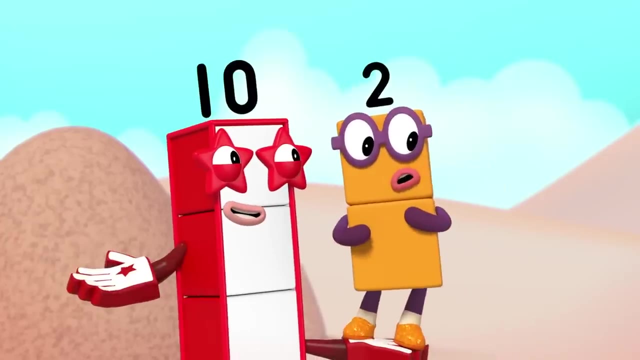 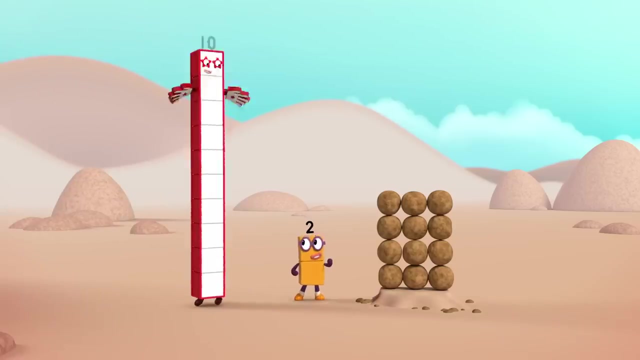 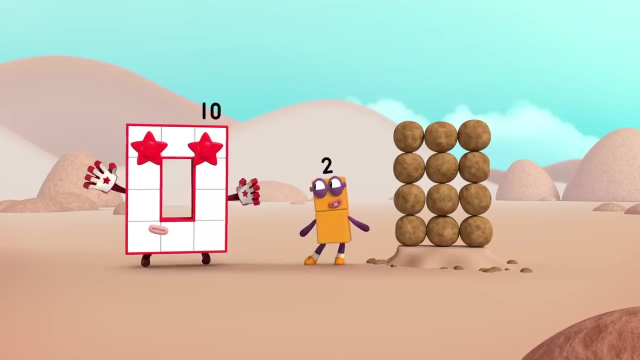 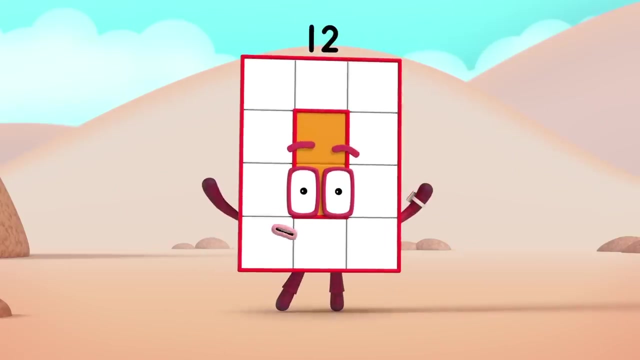 You could be an artist- the best there's ever been- But why paint only one of things when you could paint seven, Ten and two, Ten and two? Take a look, Ten and two, Ten, Nine, Ten And two, Ten And two, Ten And two, Ten, And look at that. 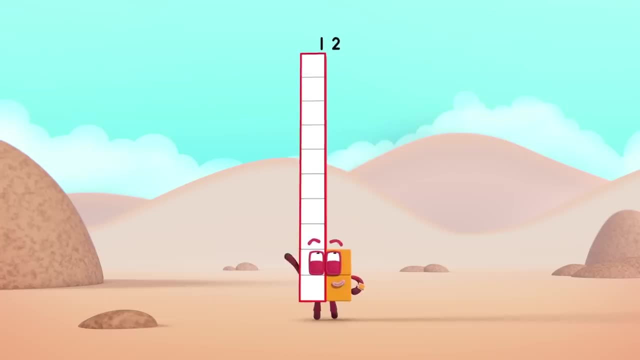 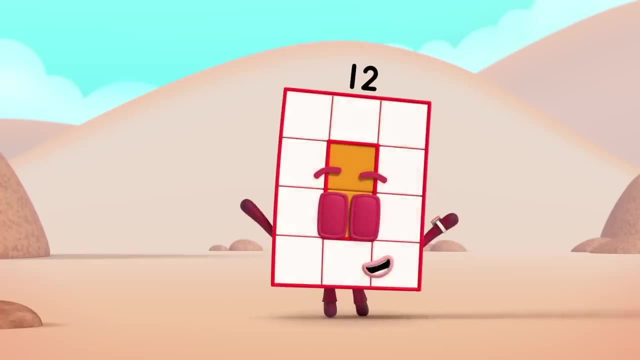 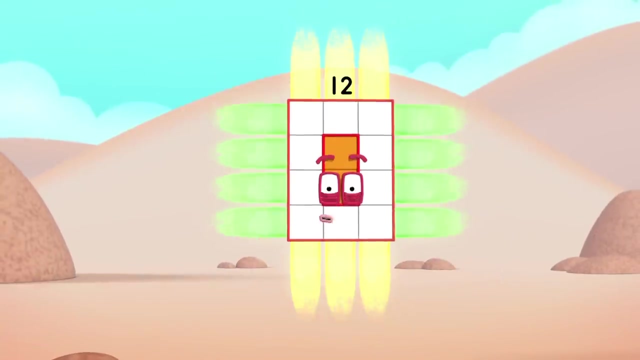 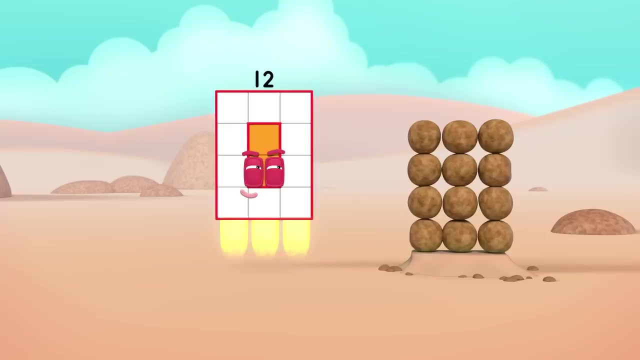 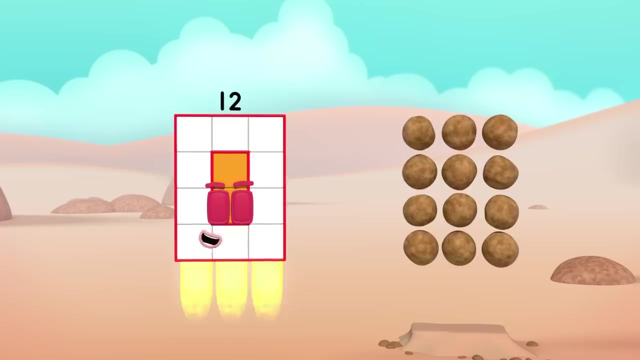 Hey, I'm ten and two Twelve. Yes, I am twelve And I am a super rectangle. The rocks are in columns and rows, My blocks are in columns and rows And that's called an array, Array. Hey, I'm rectangular twelve. 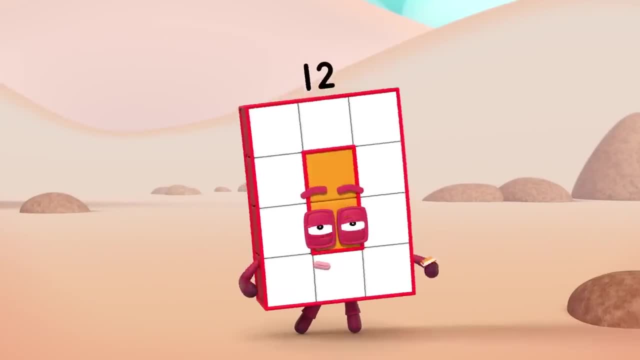 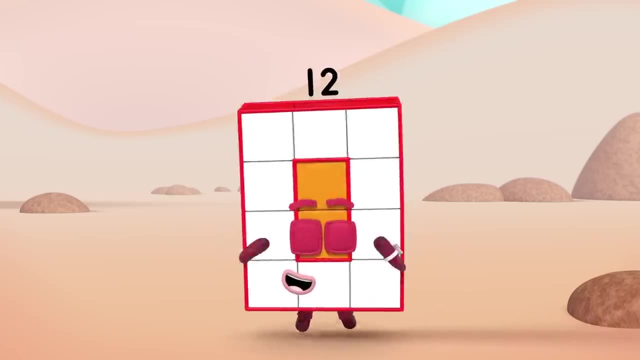 I'm ten and two, I make arrays. that's what I do When I put my blocks in columns and rows, I make an array, and my rectangle goes like this: Three By four. Today's the day for an array display. 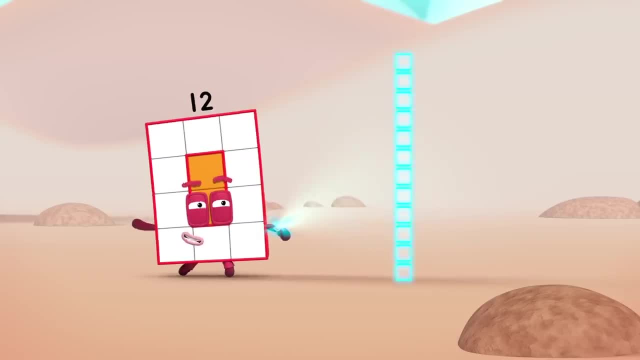 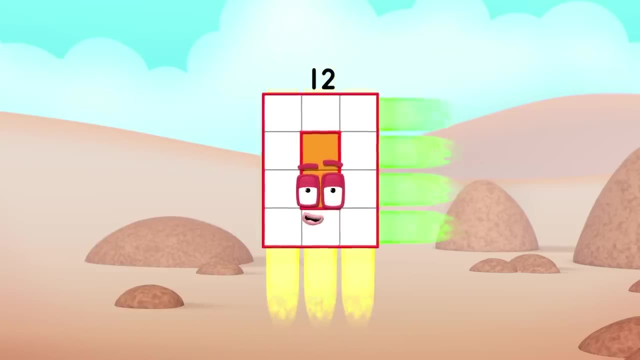 I can make arrays all day. I make arrays in many ways. Stand back, let's play arrays away. Three by four is my first array. Three, lots of four- you could put it that way, And if you're not following what I say, 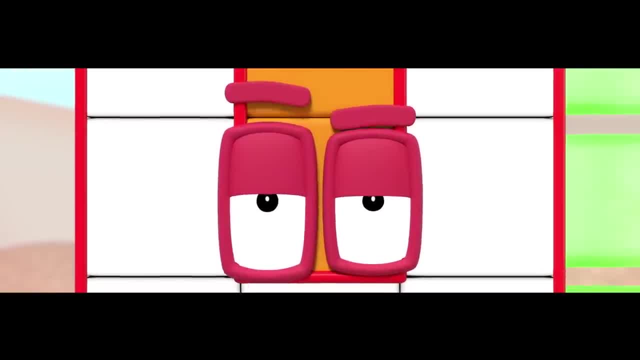 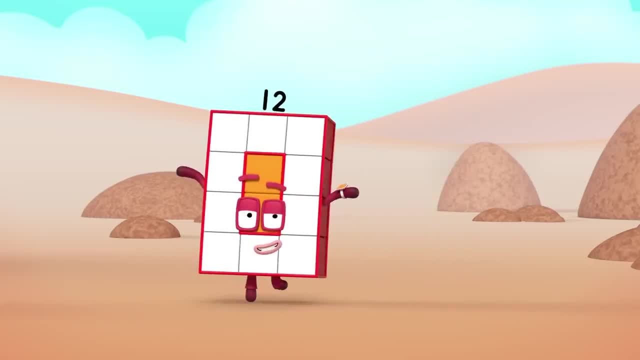 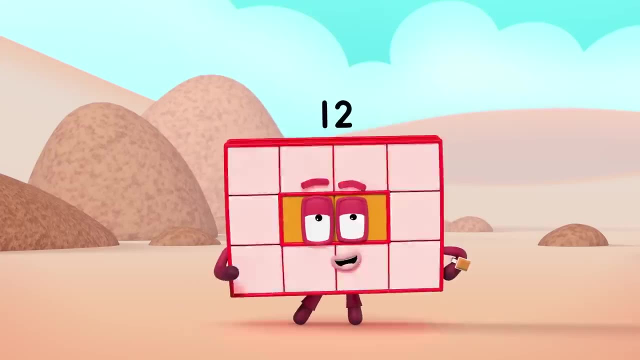 I'll rectify that right away. Breakaway: Three, fours, A four and a four and a four. Rectangle, right Turn: I'm rectangular twelve. I'm ten and two. I make arrays. that's what I do. 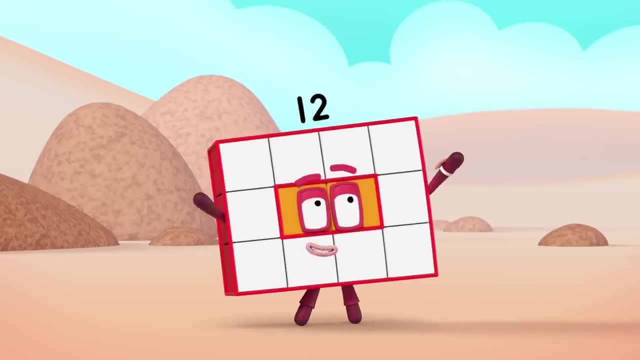 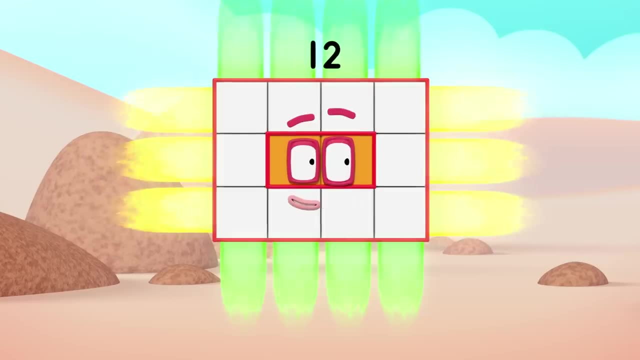 When I put my blocks in columns and rows, I make an array and my rectangle goes like this: Four By three, Four by three's. my next array: Four, lots of three- you could put it that way- And this rectangular display is about to show you how it's made. 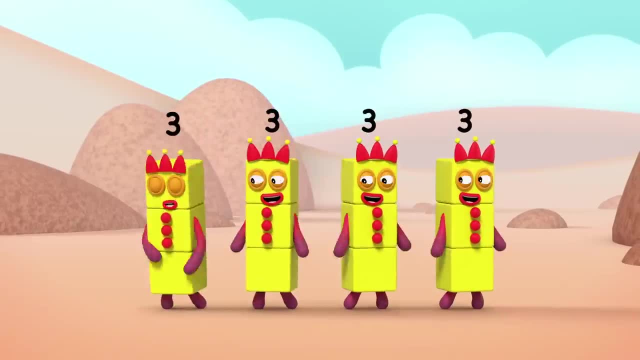 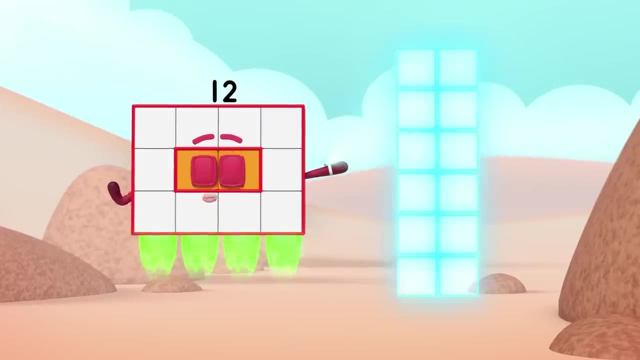 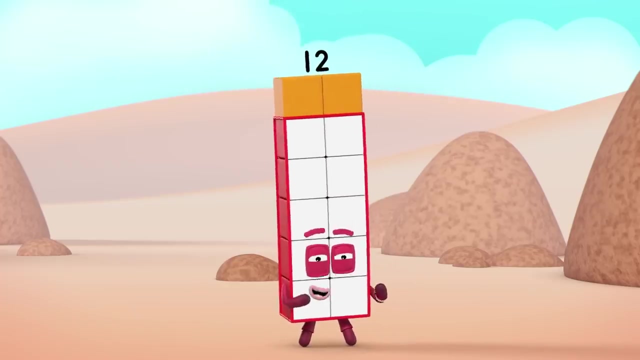 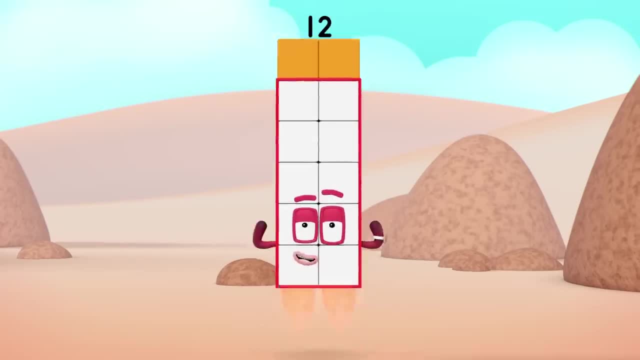 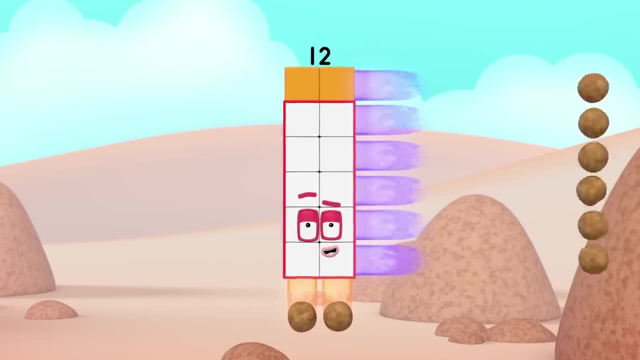 I make an array and my rectangle goes like this: Two By six. Two by six is another way. Two, lots of six. Do you hear what I say? Another rectangular array. So let's split without delay. Breakaway: Two sixes. 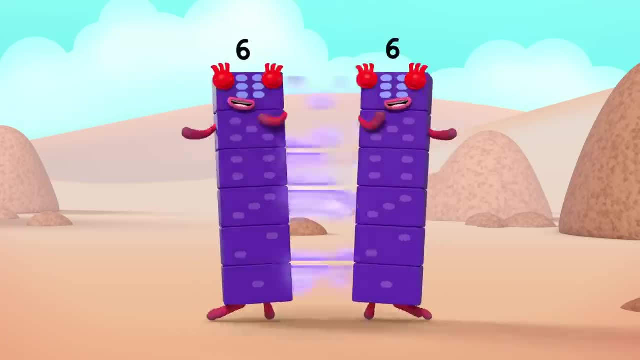 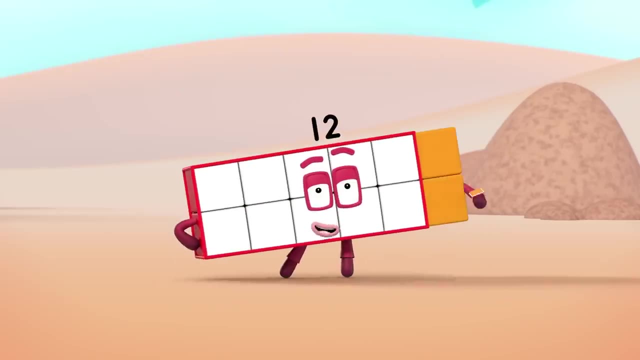 Let's roll Double. six, Ten, I'm rectangular. twelve, I'm ten and two, I make arrays. that's what I do When I put my blocks in columns and rows. I make an array and my rectangle goes like this: 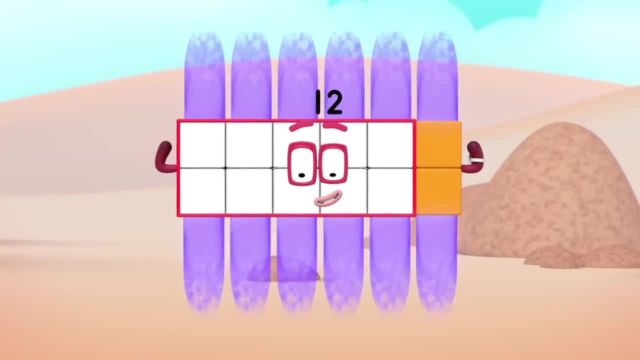 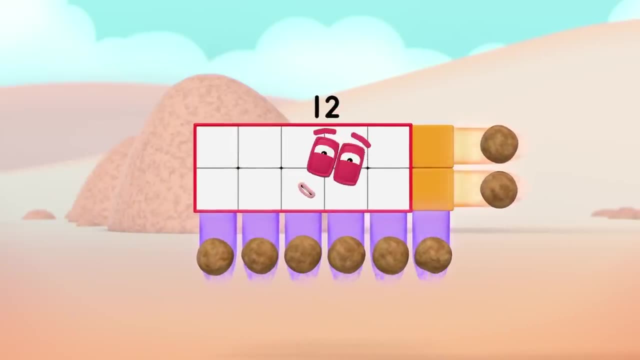 Six By two. Six by two is next in line. Six, lots of two. It's a clever design And if you want to see how all this fits, I can break it all to bits. Breakaway: Six, twos, One, two, one, two, one, two. 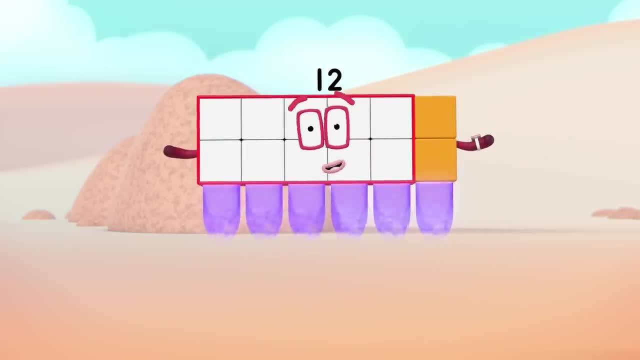 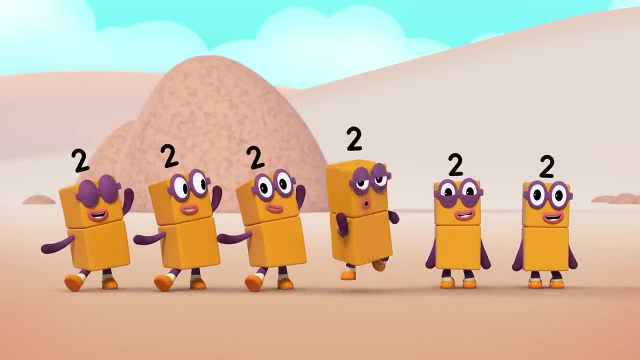 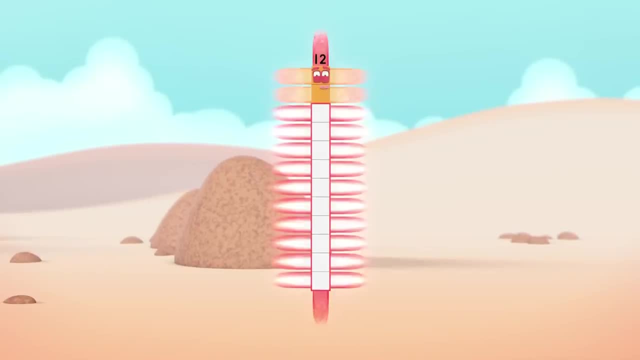 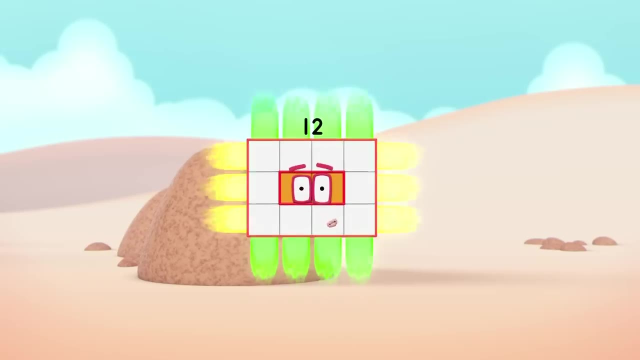 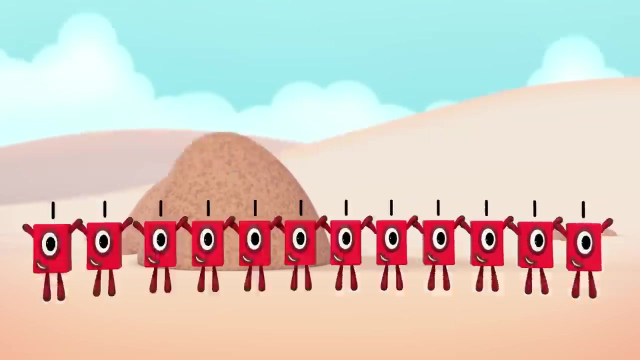 Switch Two By six. Two One By six. Switch Three By four. Turn Four By three. Switch Six By two. Switch Twelve By one. Breakaway One, Two, Three. 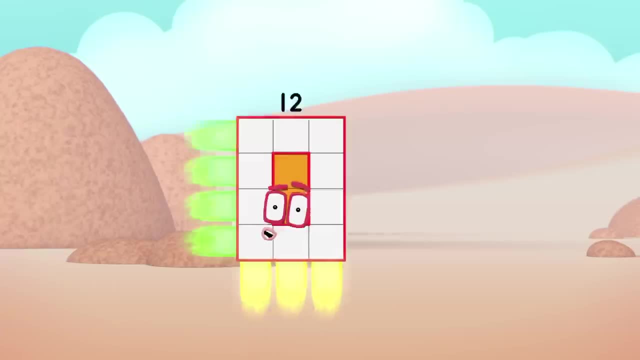 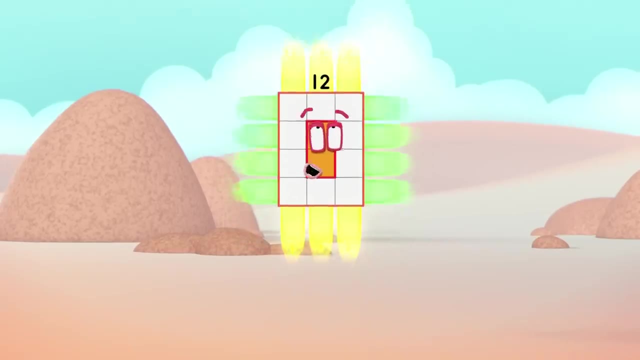 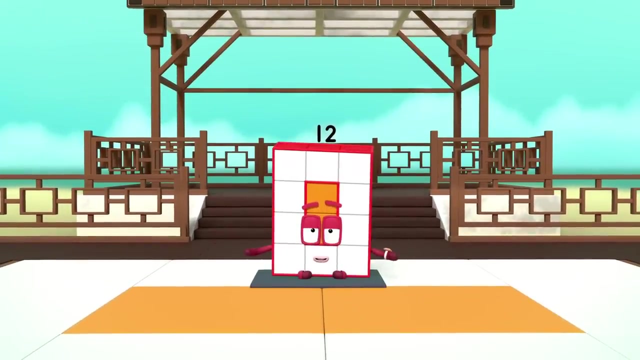 Four, Five, Six, Seven, Eight, Nine, Ten, Eleven, Twelve- It's a new crease, to coin a phrase. You'll be in a daze when you fix your gaze on my amazing array displays. I am twelve. 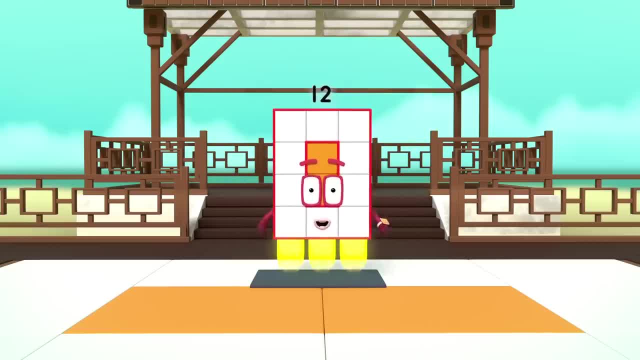 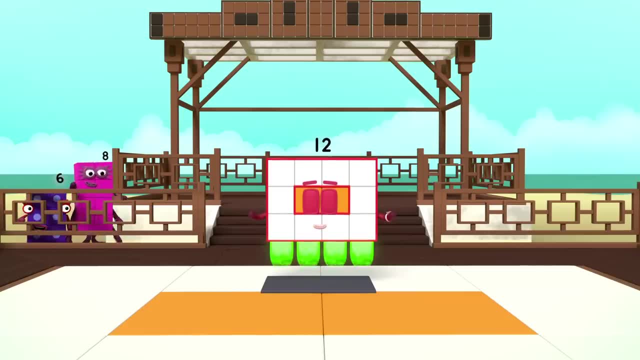 I am three by four. I am a rectangle Turn. I am also four by three, Abu, And I am a super rectangle. I can take many forms, Switch. I am six by two Turn. I am two by three. 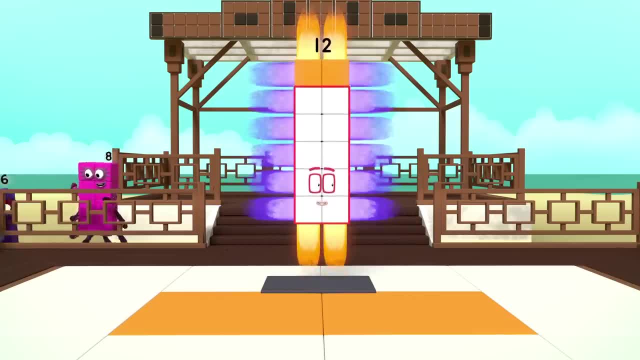 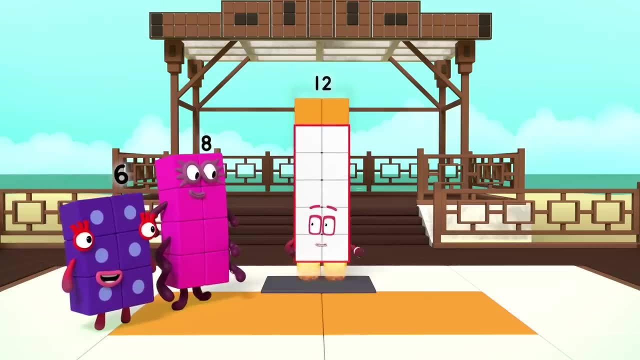 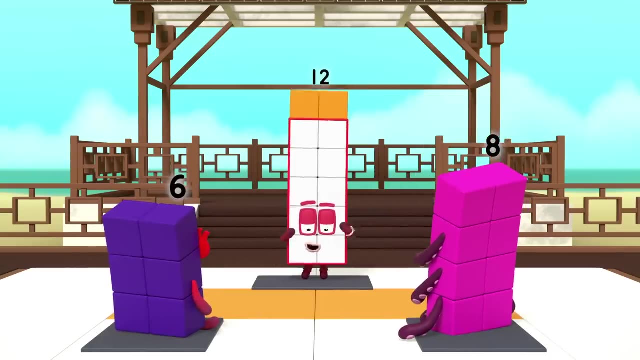 I am four by four, I am five by three, two by six. I am a rectangle. Welcome, my friends. Would you like to master the way of the rectangle? First you need to stand so your front makes a rectangle shape. Watch and tell me when. 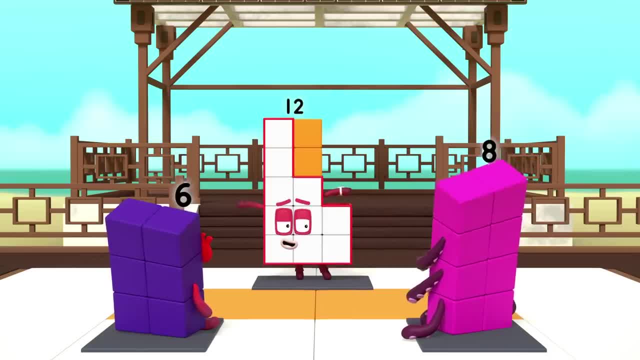 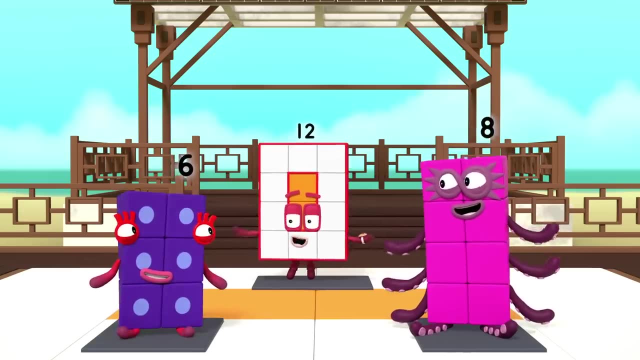 I'm making a rectangle. No, No, No, Yes, Well done. Now look at your own fronts. What shape are you making? I'm a rectangle. That's right. Your blocks are arranged in neat columns and rows. Now concentrate on. 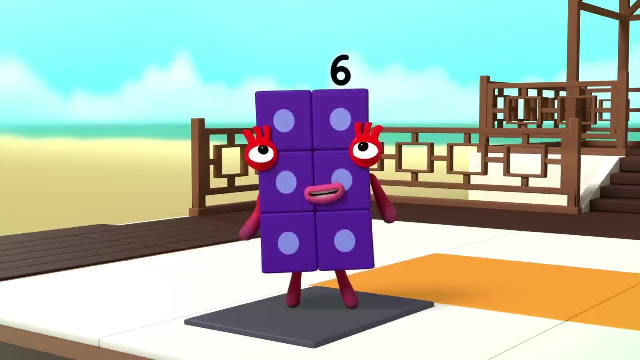 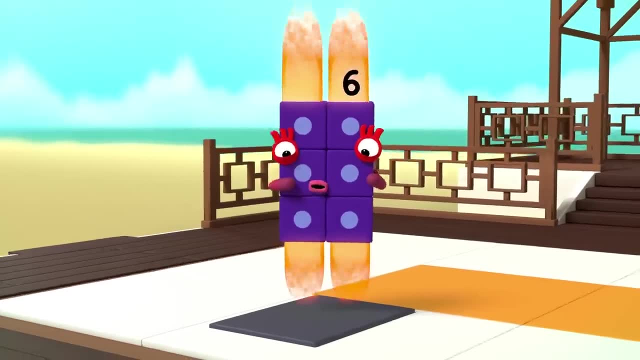 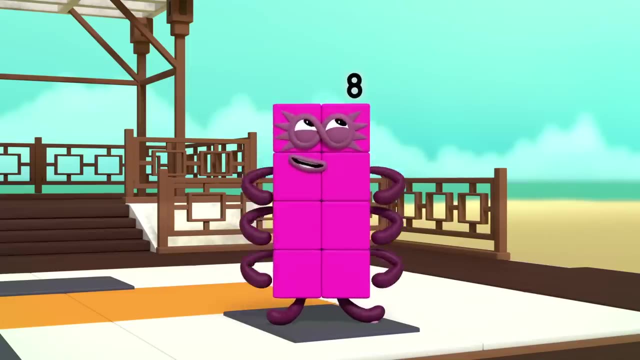 how wide you are. I am six. I am two blocks wide by three blocks tall. I am two by three. I am a rectangle, Hee-hee-hee Ugh. I am eight. I am two blocks wide by four blocks tall. 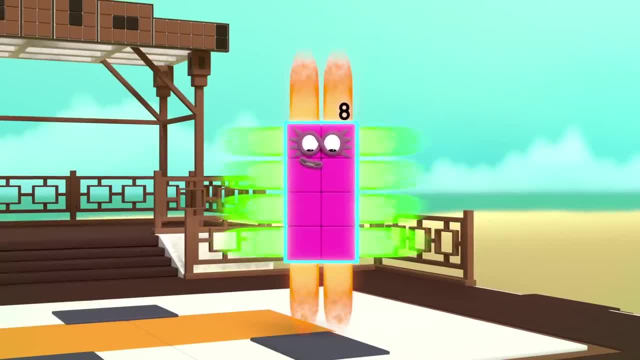 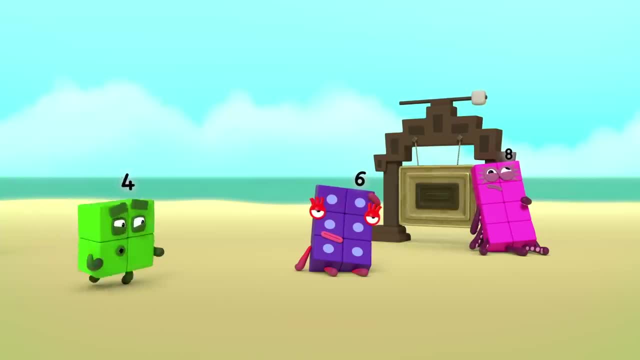 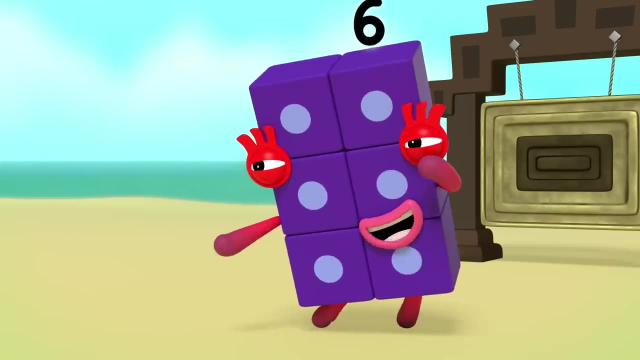 I am two by four. I am a rectangle Up, up and away. Whoa, Oh, I heard a bang. Are you okay? Six, I'm more than okay. I've mastered the way. Hey, where are my rays? 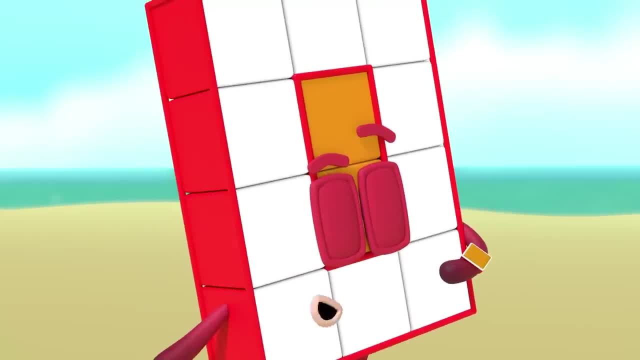 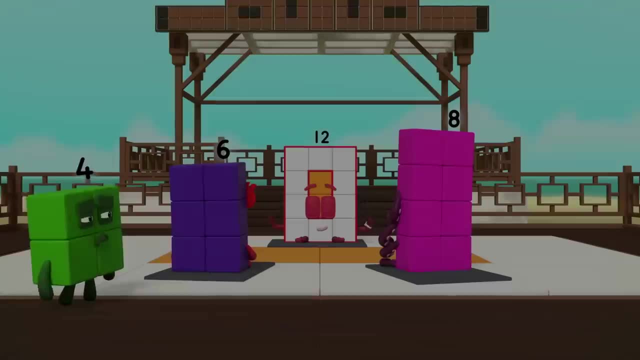 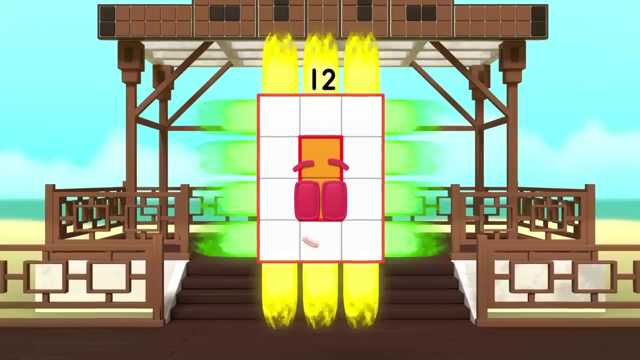 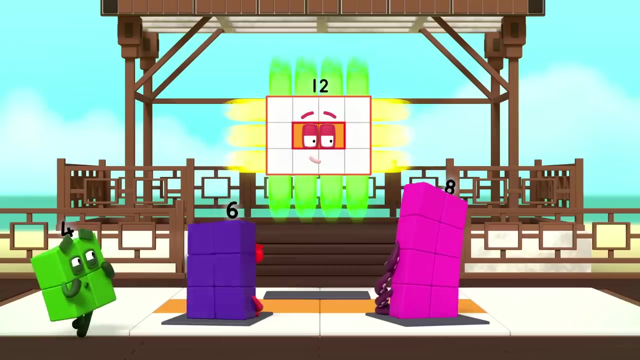 You need to concentrate. It gets easier with practice, So let's practice. It's time for the turn. I am twelve. I am three by four, Which means turn. I am also four by three. See Whoa, I am six. 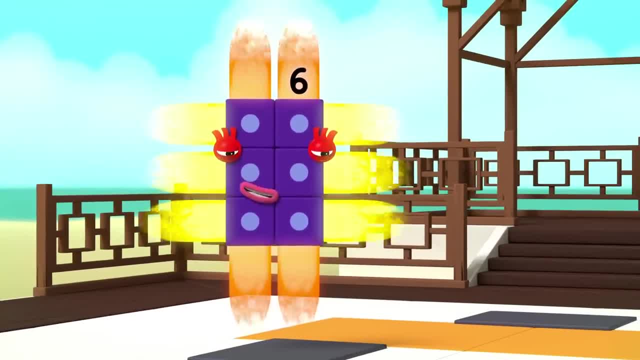 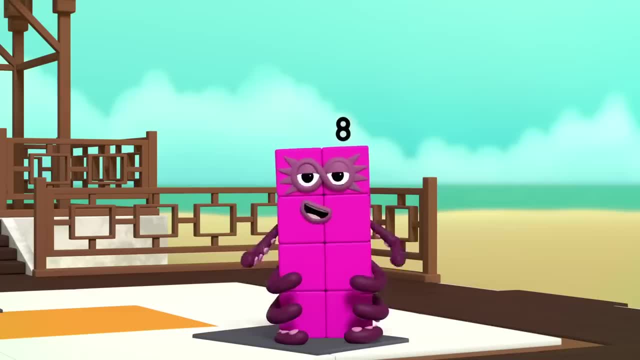 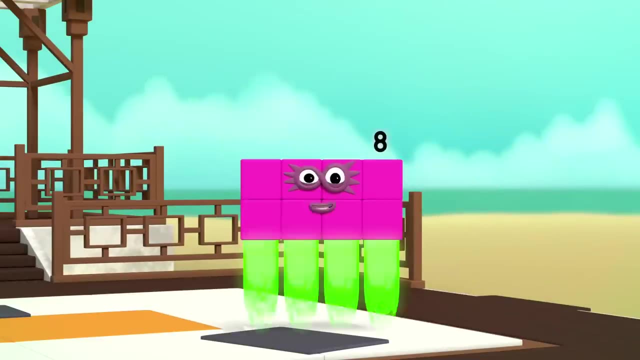 I am two by three, Which means turn. I am also three by two, Hoo-hoo-hoo-hoo, I am eight. I am two by four, Which means octoblock turn. I am also four by two Turn. 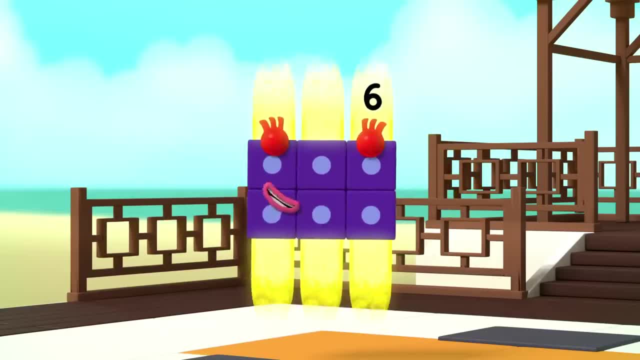 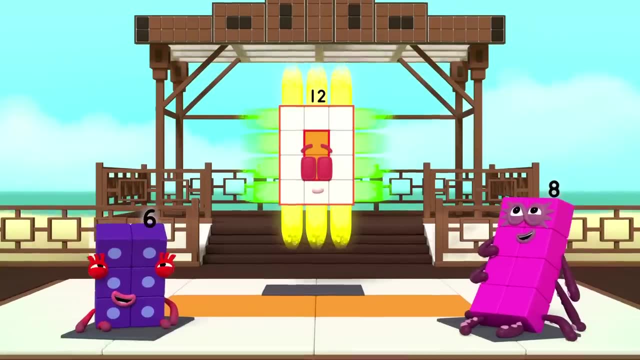 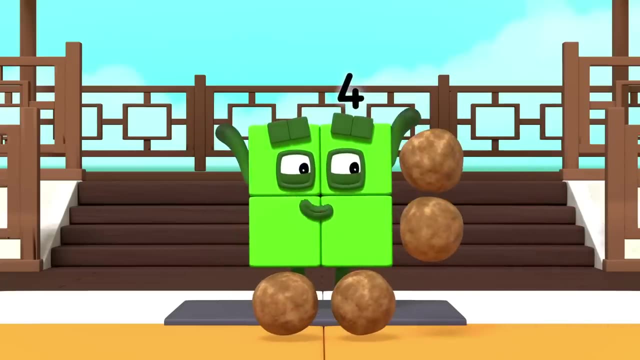 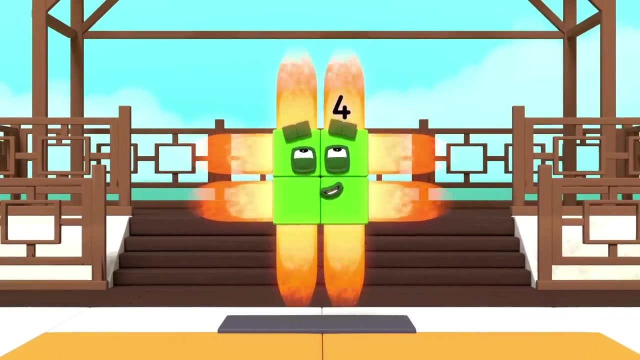 Two by three, Turn, Three by two, Turn, Turn, Turn, Turn, Turn. Oh, let me try that. I am four. I am two blocks wide by two blocks tall. I am two by two. Yay, And I am also turn. 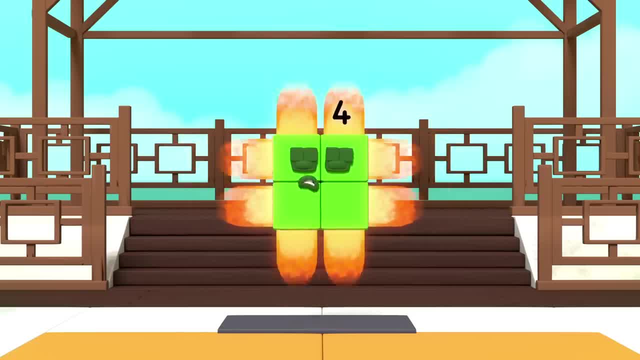 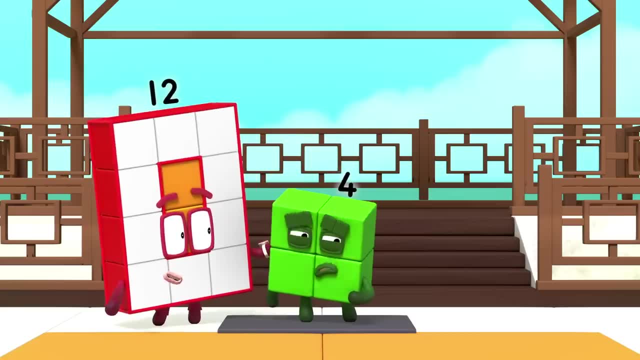 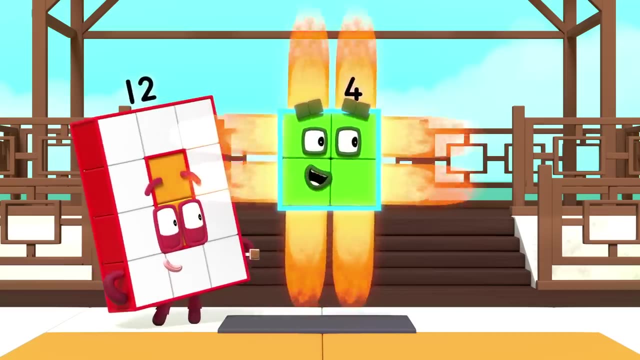 Um two by two. That's the same again. Did I go wrong? No Four, You're a special kind of rectangle that is the same number of blocks as tall, Two blocks wide by two blocks wide, Just say two. 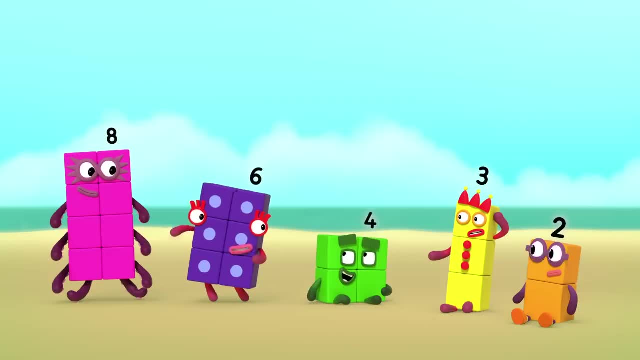 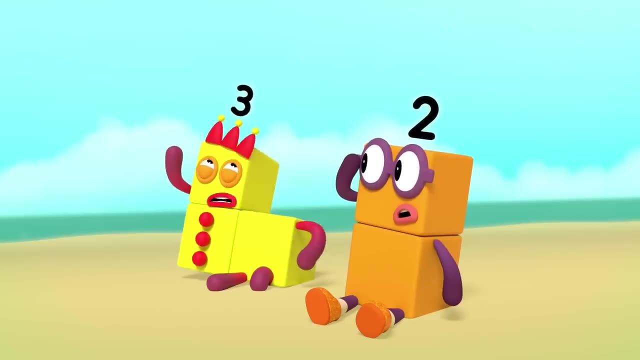 K recommended One, two, three, And I'm tall about seven feet. Woo-hoo, C'mon, This is ça. We need more said bats. if it's gonna make me mistake, I can't Perfect, I don't know where to go. 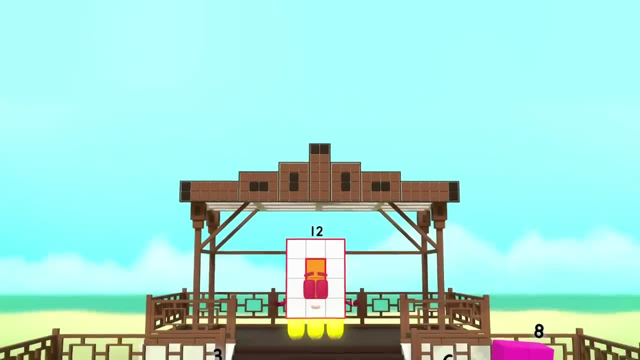 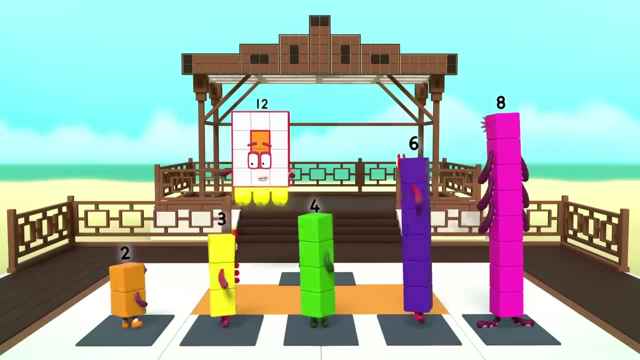 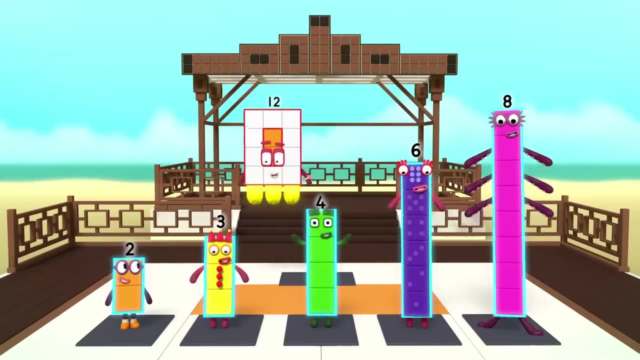 But I'm pretty sure I can catch him, Maybe. Hmm, Hey, Now, what shape are you making? Oh er, A rectangle, A tall, thin rectangle. I am one block wide And I am two, three, four, six, eight. 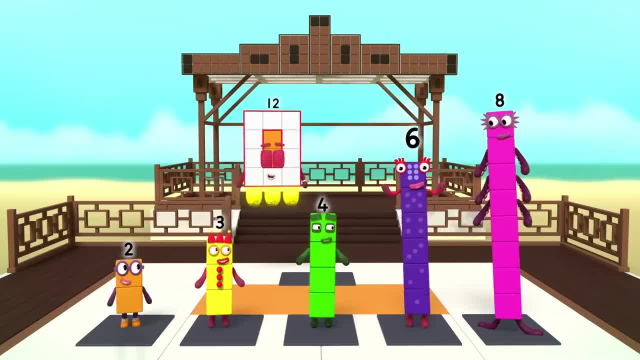 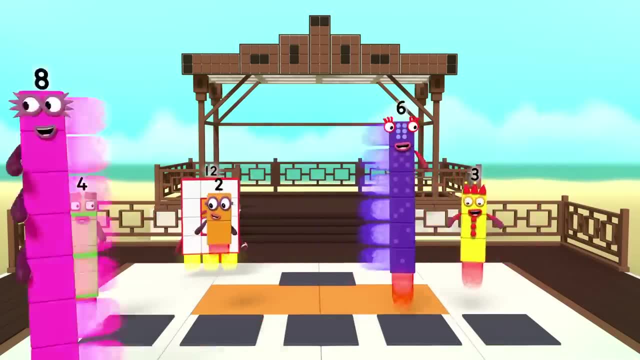 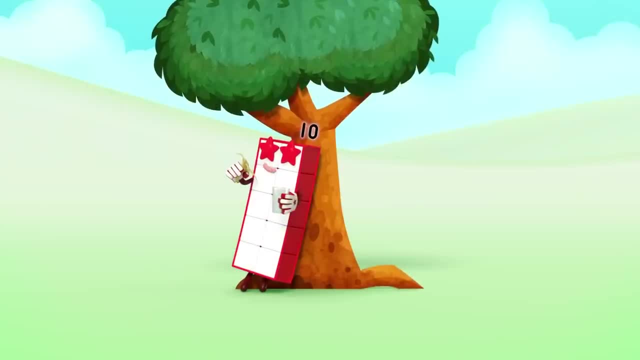 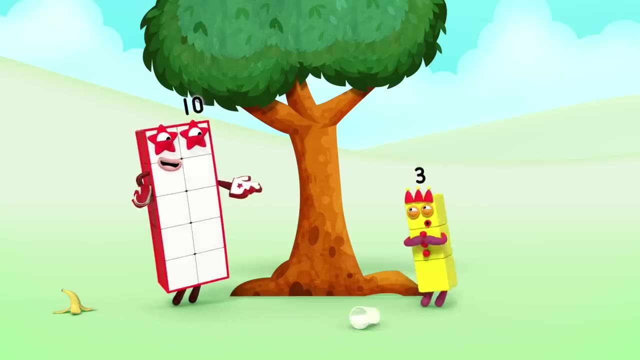 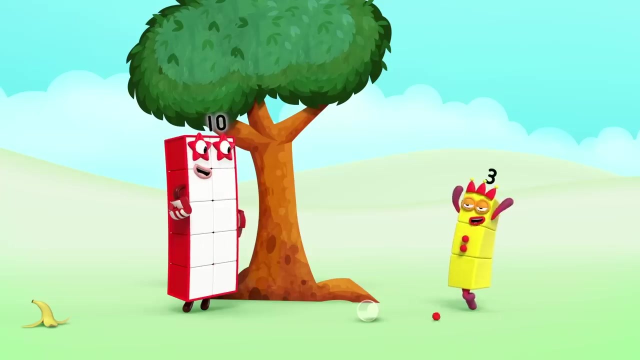 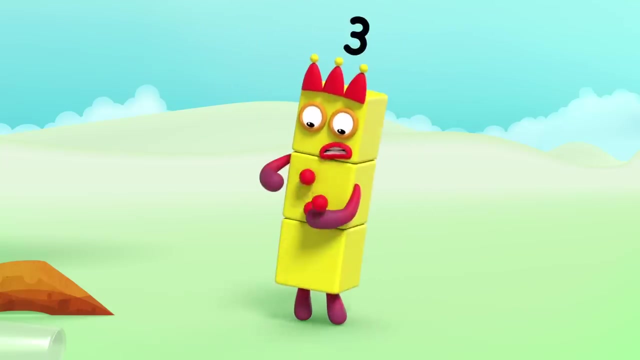 Ooh Whoa, Bam, bam, bam, Whoa. Three, Oh sorry, Ten. I'm just so excited to show you my new trick. Look at this. Oh, Is that it? No wait, I'm not having much luck with mine. 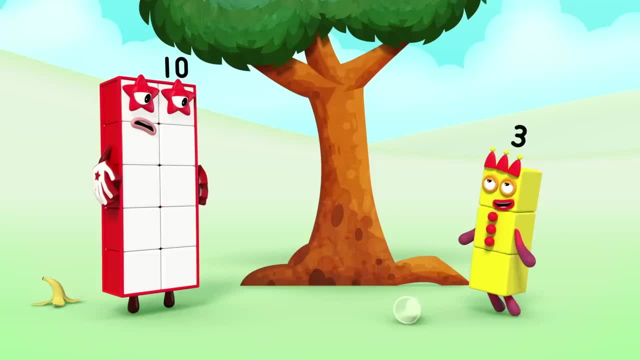 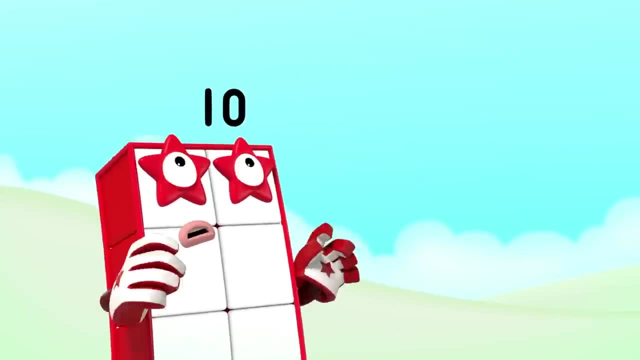 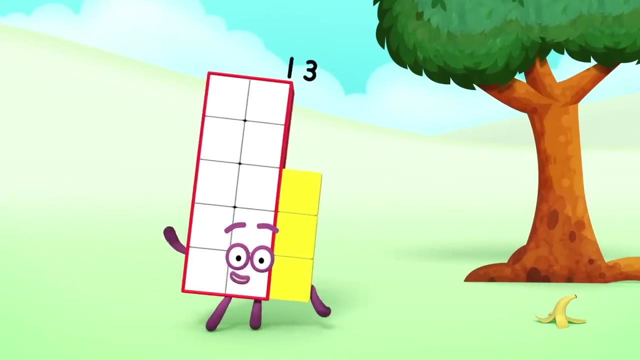 I've got to get back to work today. Oh no, My new trick: Ready, steady go Ha. Ooh, Whoa, Whoa, Oh, Oh, Unlucky, Oh Hi, Who am I? 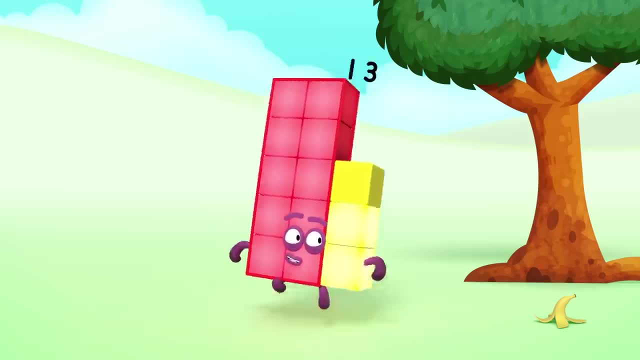 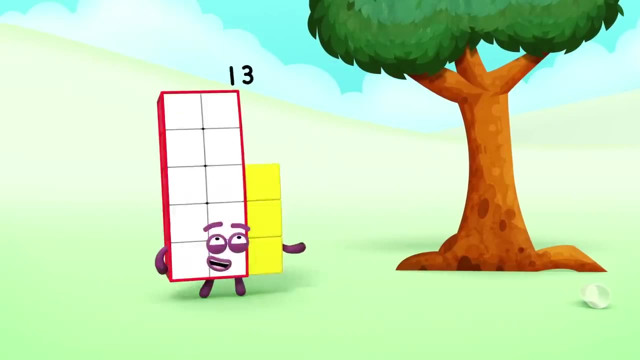 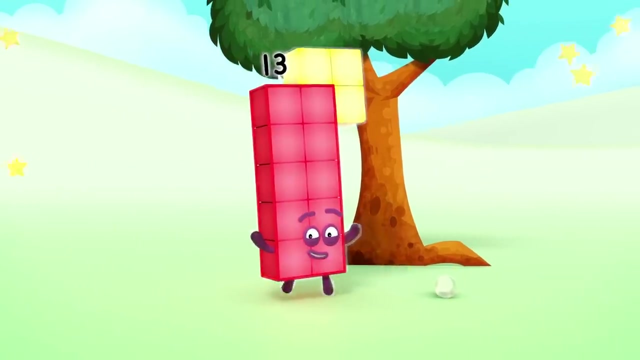 I'm one, two, three, four, five, six, seven, eight, nine, ten, eleven, twelve, thirteen, Whoa, Whoa, Wow, Whoa. Oh, my three fell off. Never mind, I am 13.. 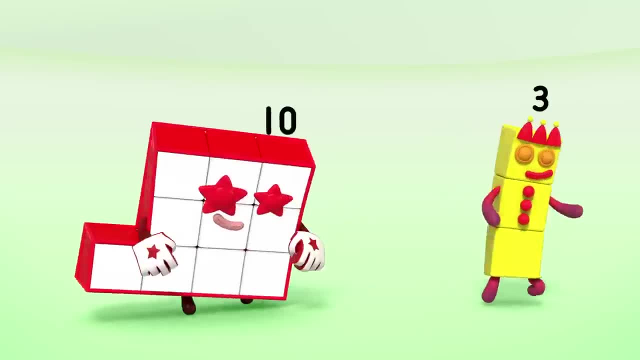 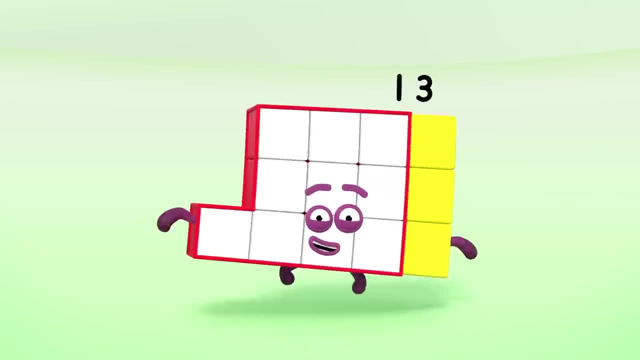 Oh, whoa Ha Ha, ha, ha, ha ha. Oh, unlucky, Try again, I am 13.. Ha ha, ha, ha ha. Hooray Ooh Ha, ha, ha, ha ha. 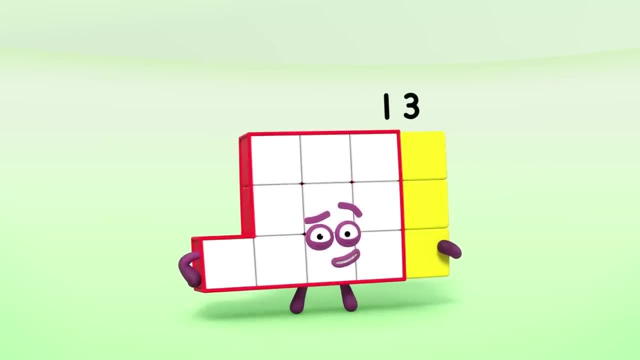 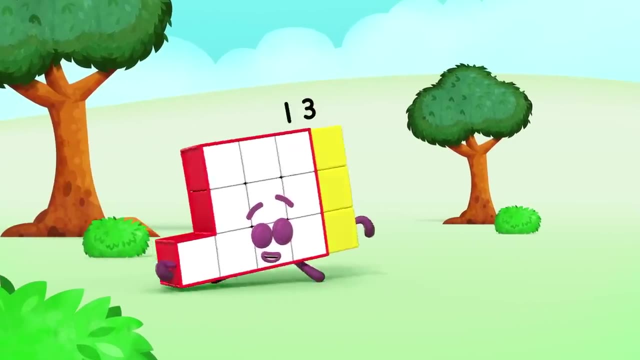 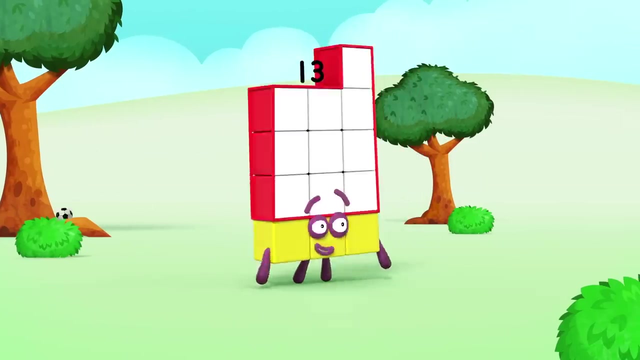 Oh Ooh, And I think I might be a little bit unlucky. This is me, ten and three expecting to run out of luck. Sorry, It's all jolly japes. when I get into scrapes, I'm always coming unstuck. 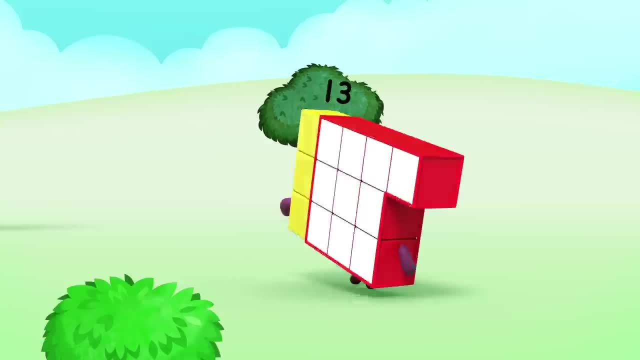 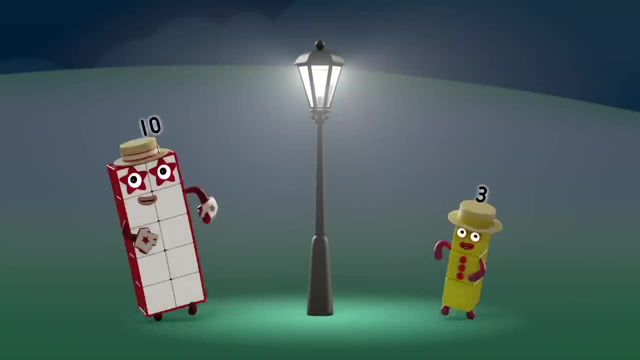 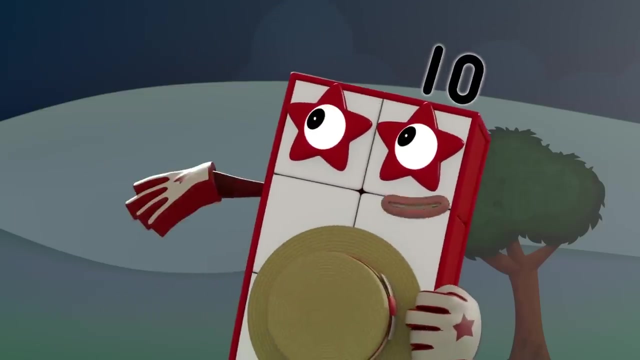 Oh, I'm the clumsiest number you've ever seen, Unlucky, I'm 13.. Oh, It's happened again: a three and a ten. Somebody should tell him that it's happened again. I don't have the heart to be fussy or picky. 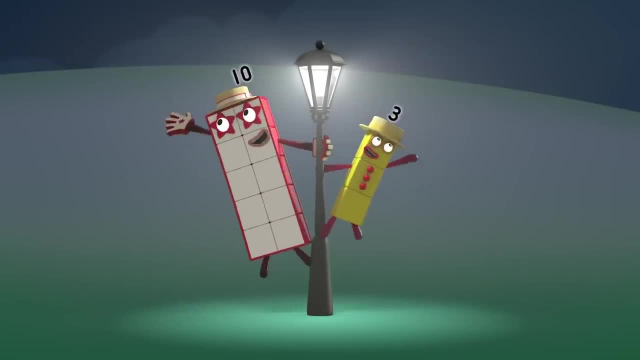 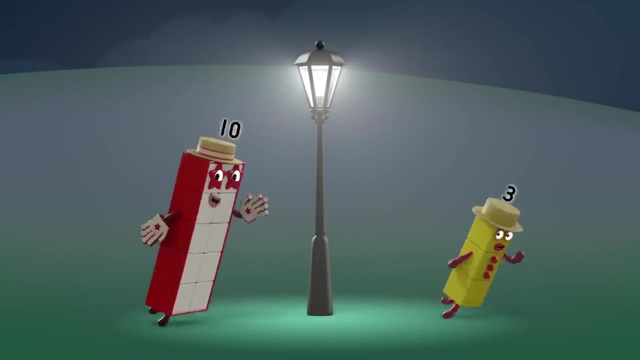 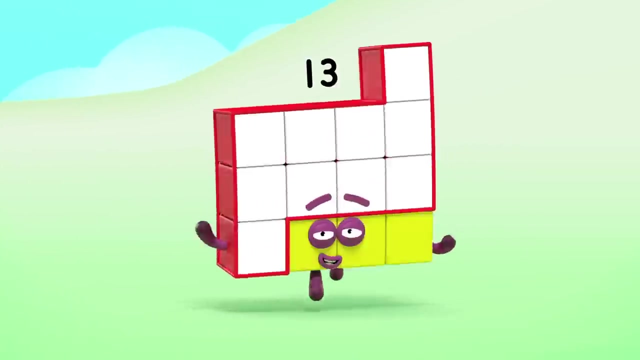 But he's falling apart. He's a bit unsticky. It's happened again and no one knows when. Somebody should tell him that it's happened again. Me again, three and ten, Expecting to fall down a hole. Ha. 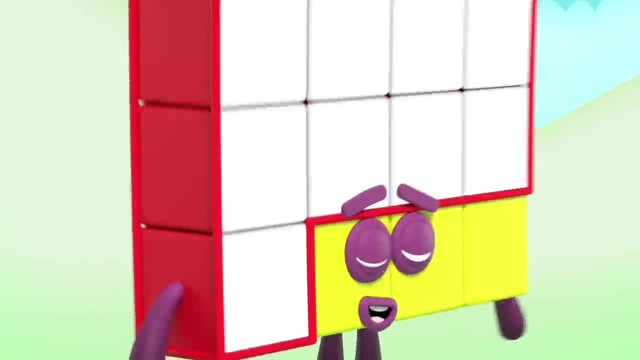 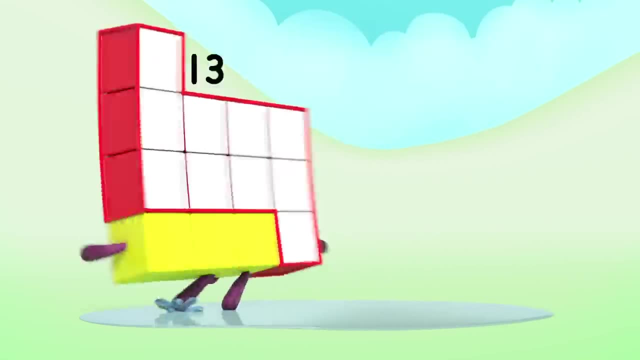 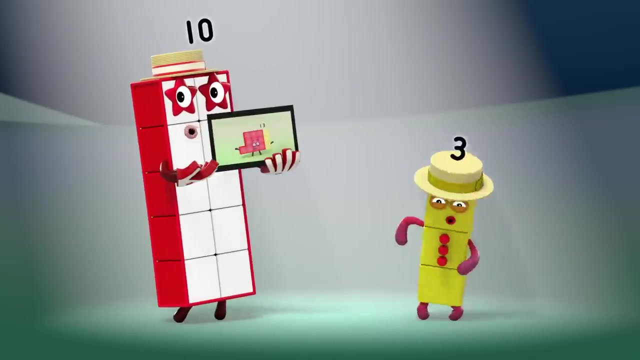 I jump through a hoop and step in the puddle. That seems to sum up my role, And wherever I end up, I might have seen unlucky number 13.. Oh, It's always the same when he says his name. Somebody should tell him that's the name of the game. 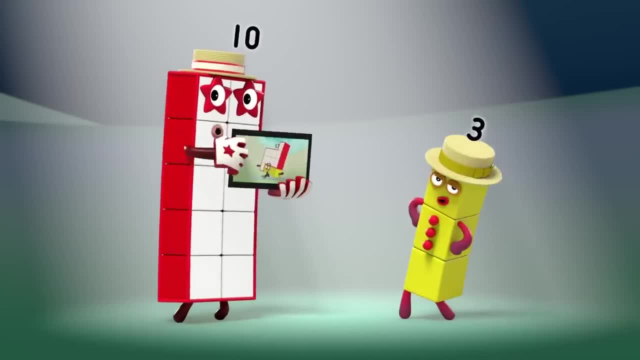 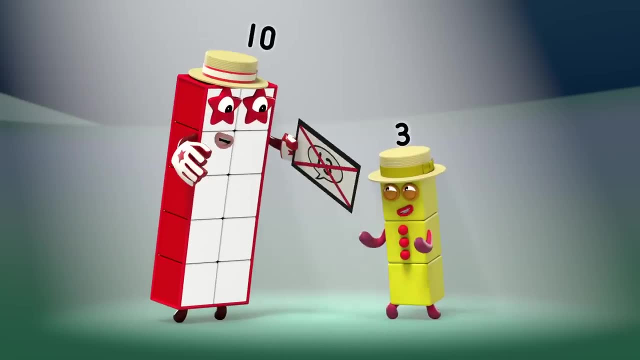 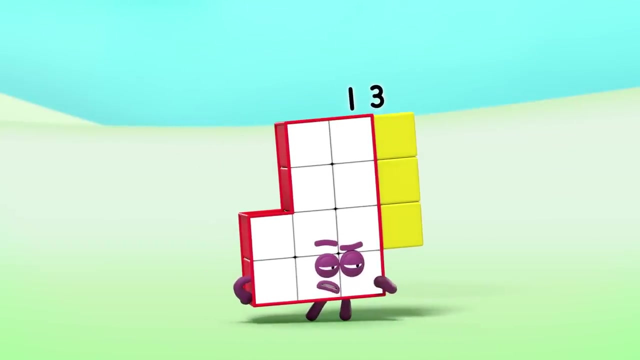 It's happened before- A total disaster. But he's going to need more than a sticking cluster. It's always the same. We know what to blame. Somebody should tell him not to mention his name. It's getting routine. I say I'm 13.. 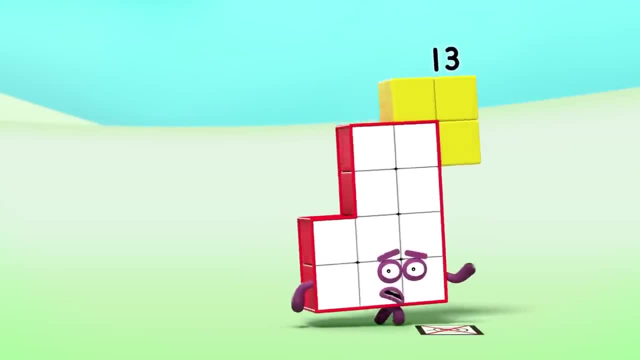 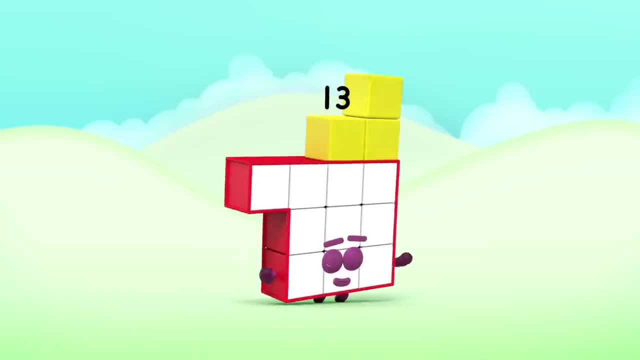 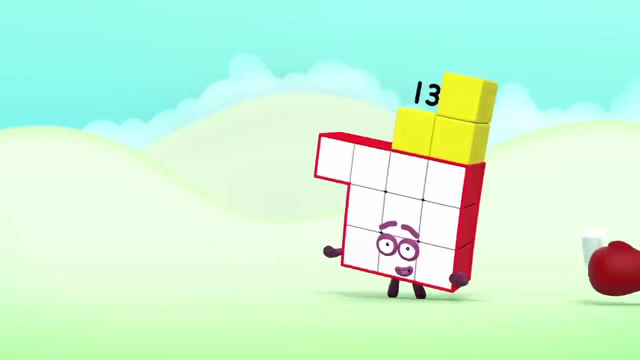 Keep it together. This is absurd. You know what I mean. I say it's 13.. End of my tether. Don't say that word. It's always the same. It's getting routine. They ask me my name. I say I'm th. 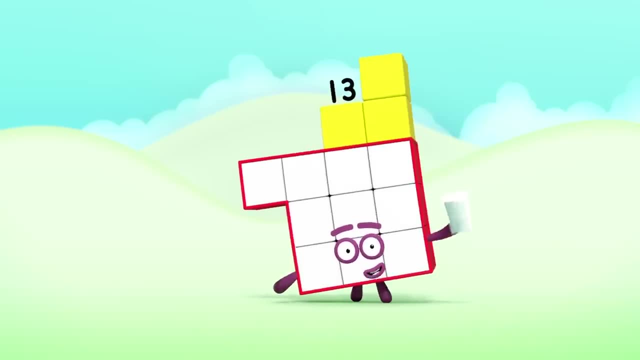 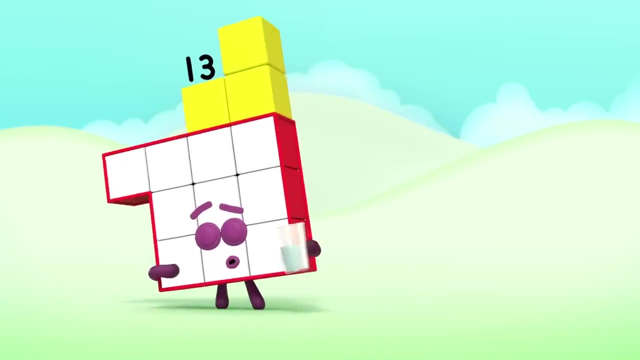 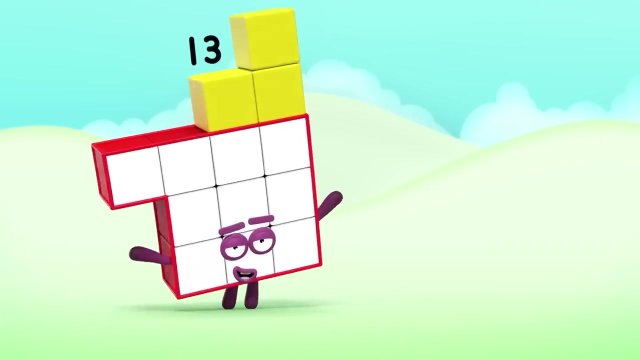 Thirsty. I say I'm thirsty. They ask me my number. You know what I mean- And I always say it's th Thursday. I always say it's Thursday, Andy, Jack, and it's their time, Woo-hoo. 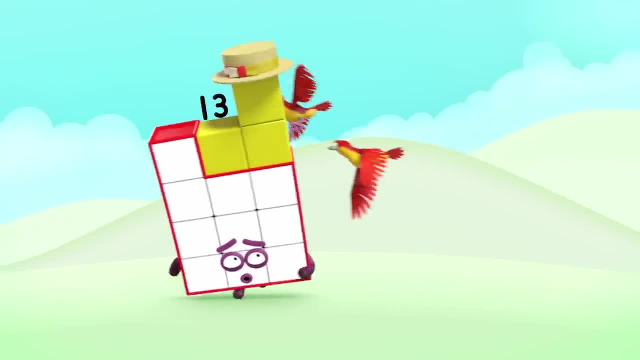 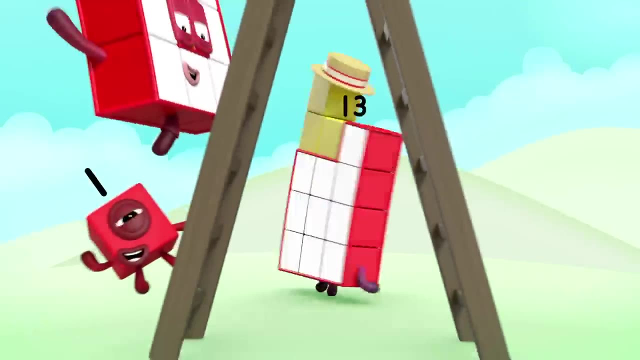 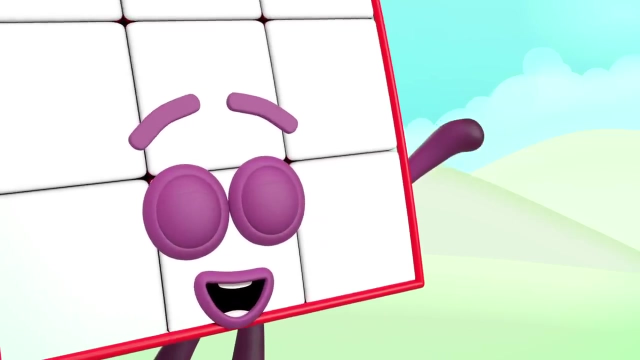 This is me. Ten and three, Turning this into a game. I'm changing my luck. I won't come unstuck As long as they don't say my name. Call me one more than 12, or ten and three, Whatever you call me, I'm still me. 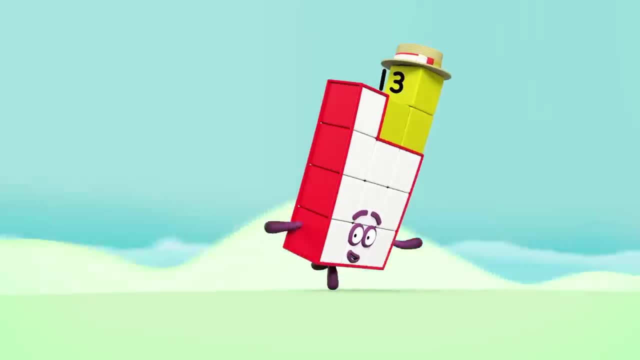 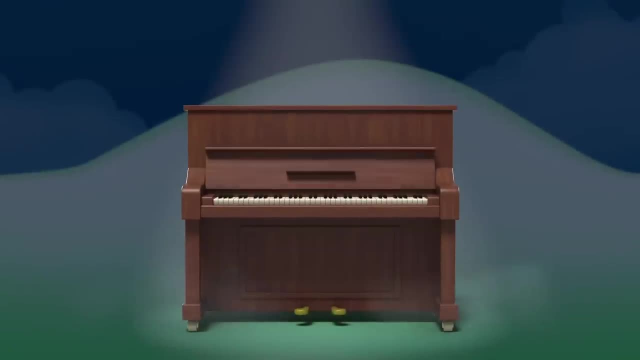 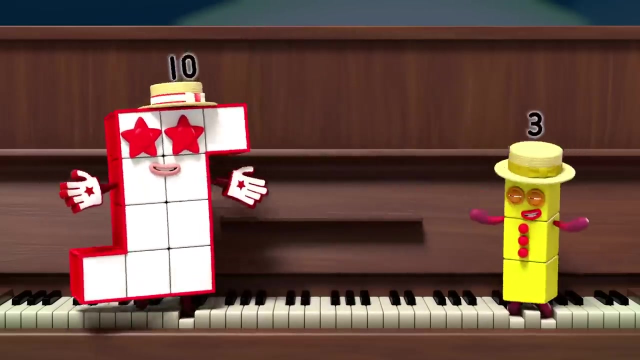 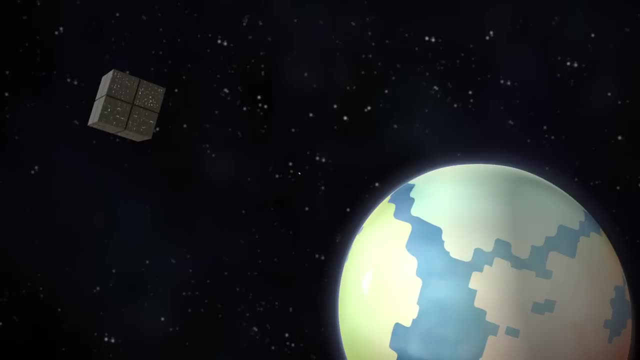 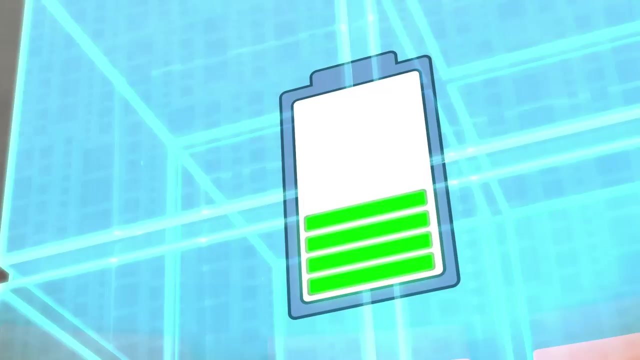 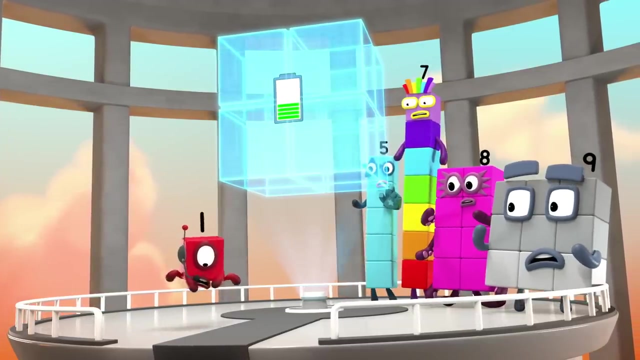 Coming Number Basic. I'm in position and heading for the Blockstar Careful 12.. The Blockstar's battery's running out. You need to change it before the whole thing drops out of the sky and smashes into Numberland. 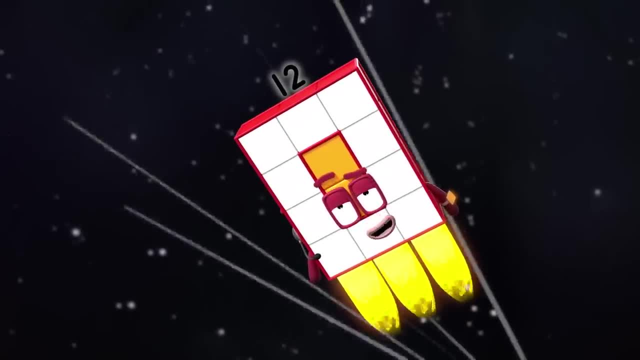 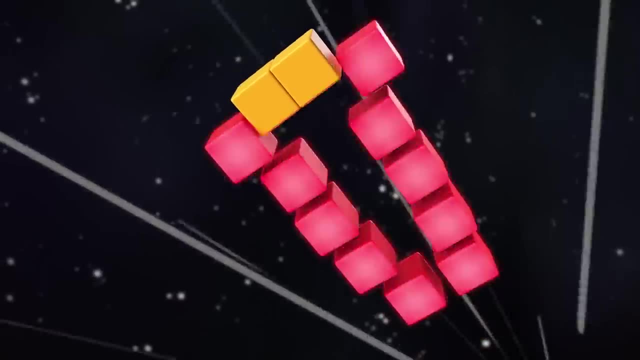 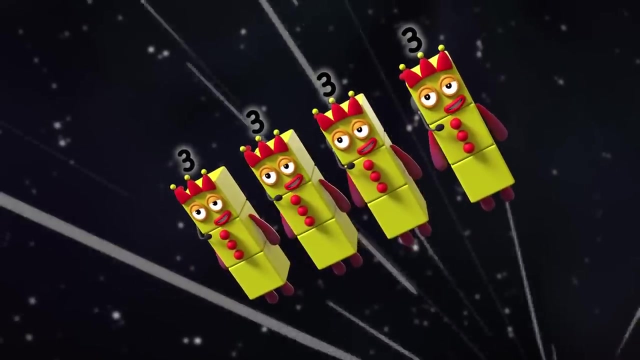 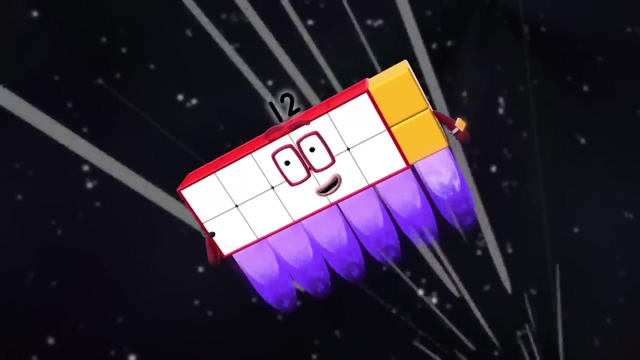 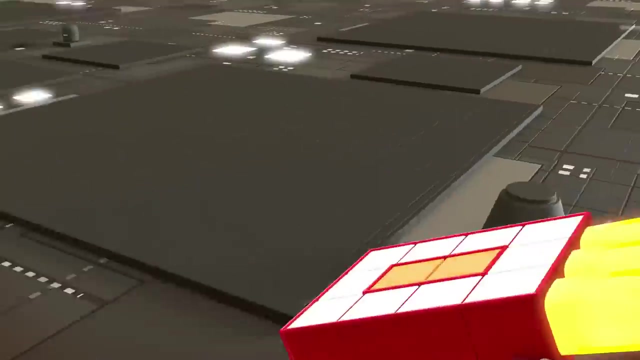 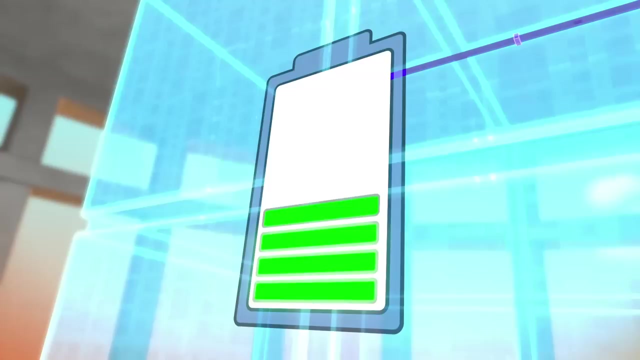 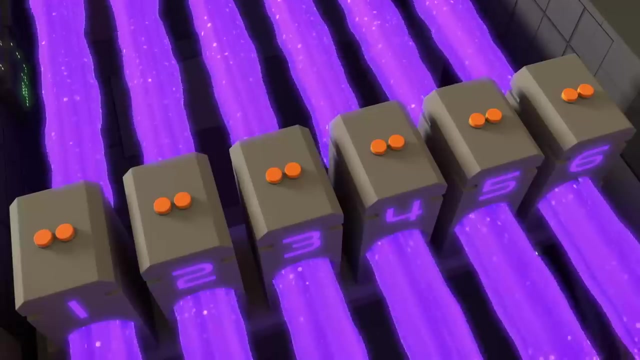 That block is no match for a super rectangle like me. all teams reporting switch two sixes standing by. You need to turn off the force field before you can get to the battery. Yes, six of them. each has two buttons on top. you need to press all the buttons together. 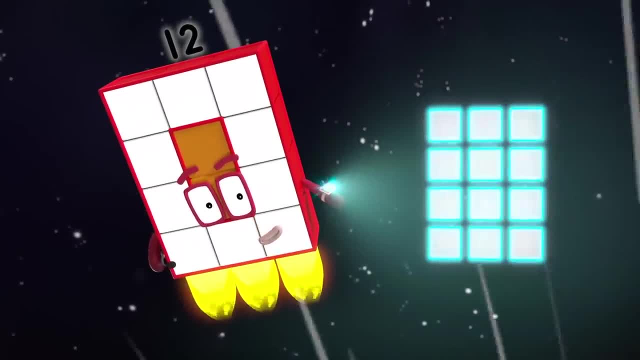 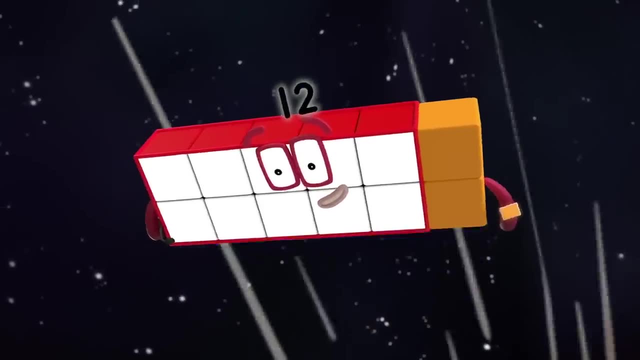 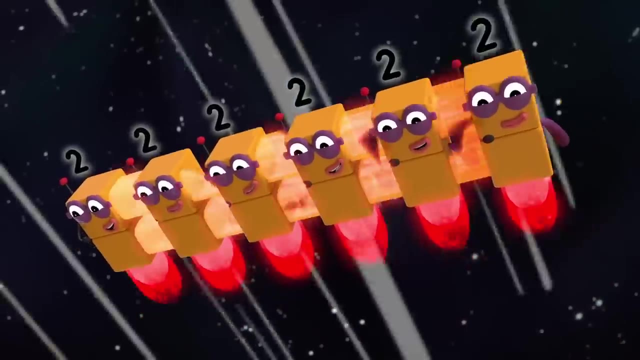 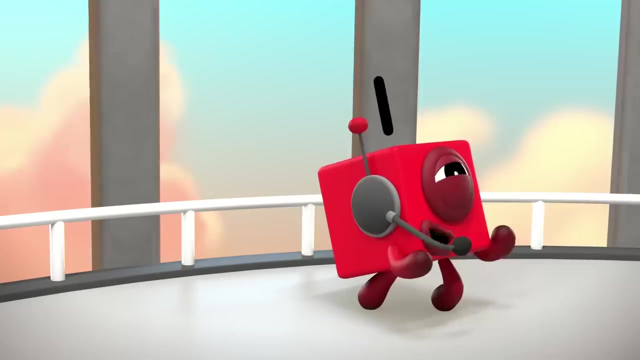 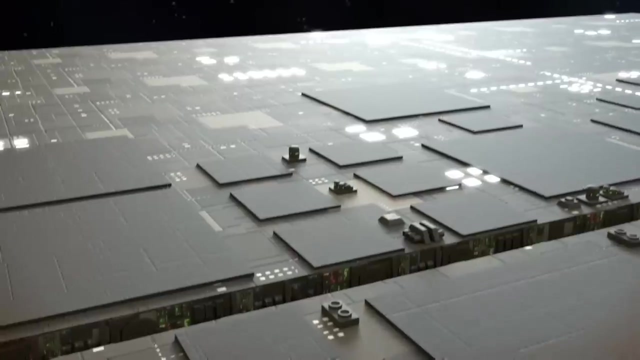 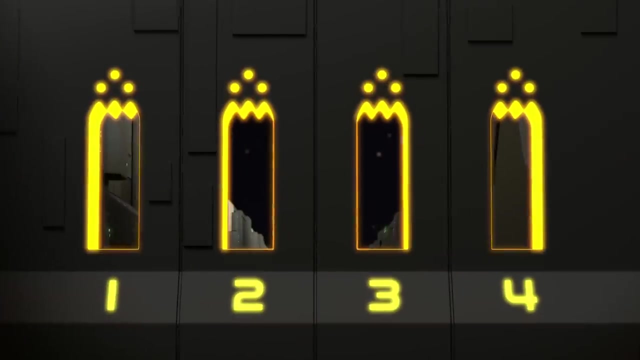 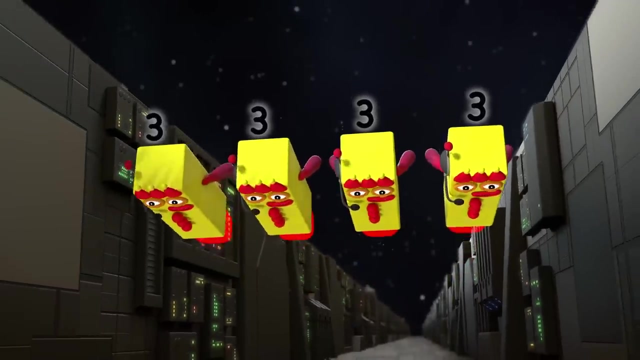 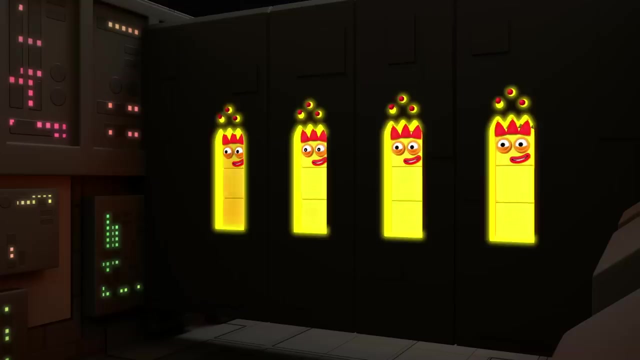 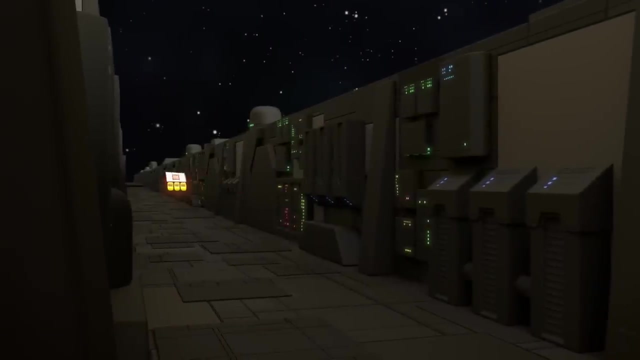 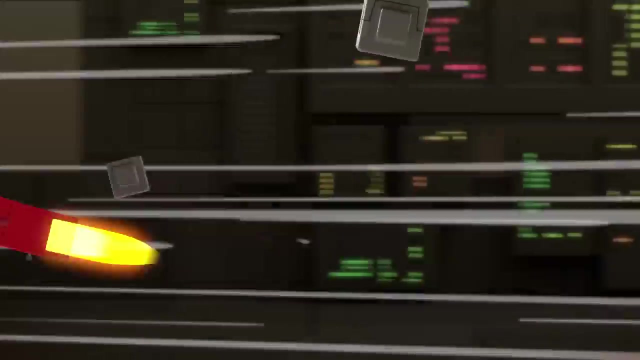 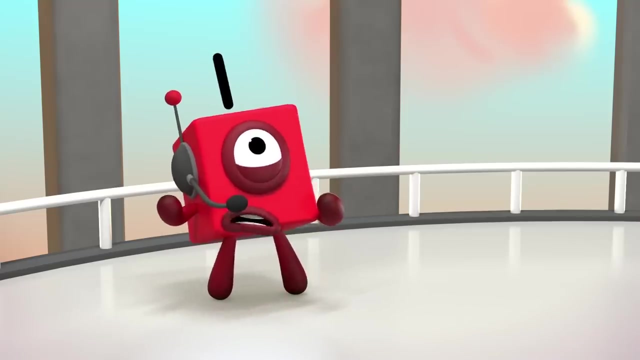 six towers, two buttons each array display. This calls for switch. You've done it: 12, now head for that battery. There's no time to lose. I'm on it. switch, Pull up 12. you're going to hit no time. Oh, Those ships have gone haywire. it must be the low battery. don't let them slow you down. 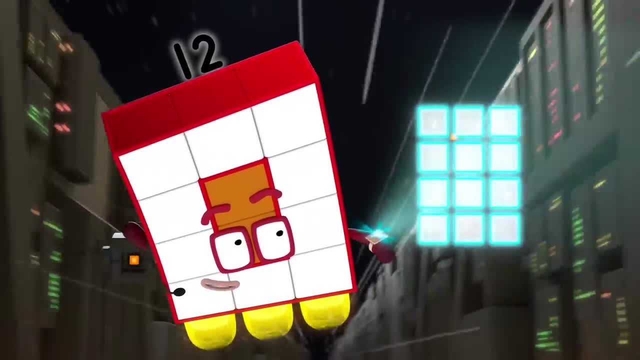 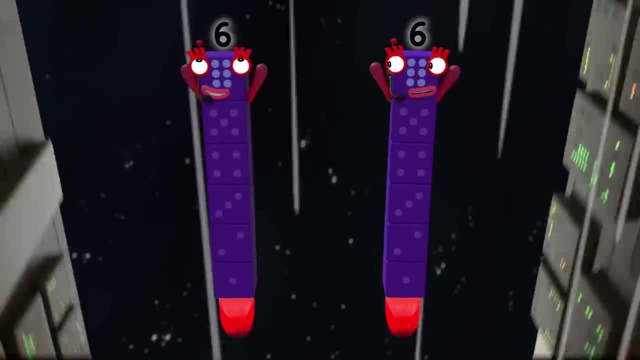 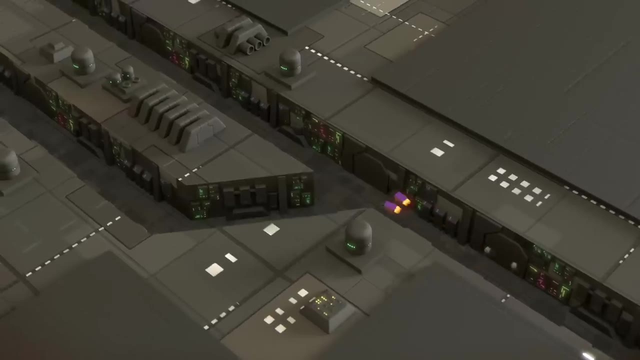 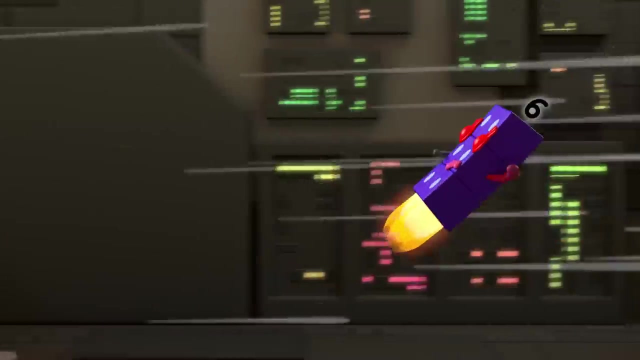 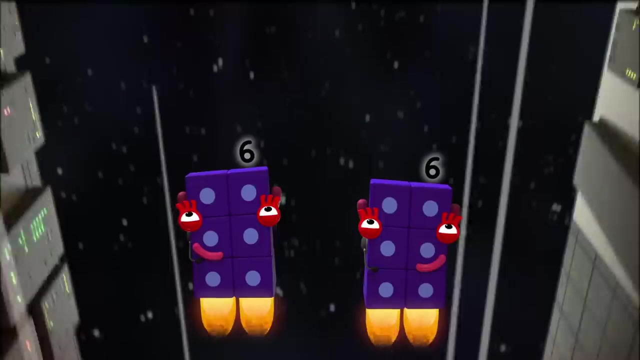 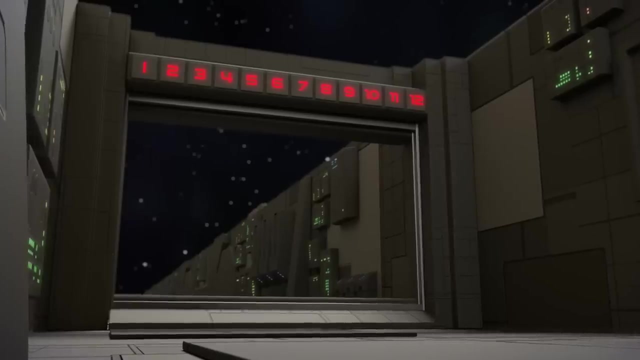 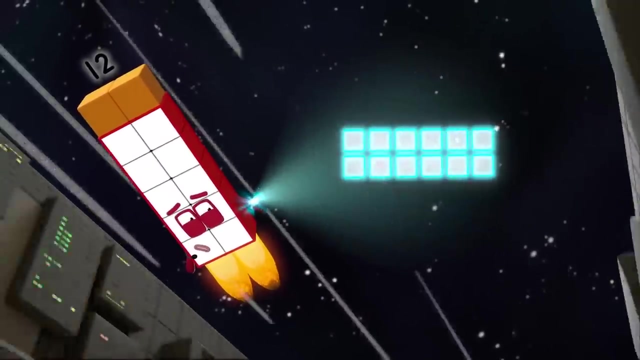 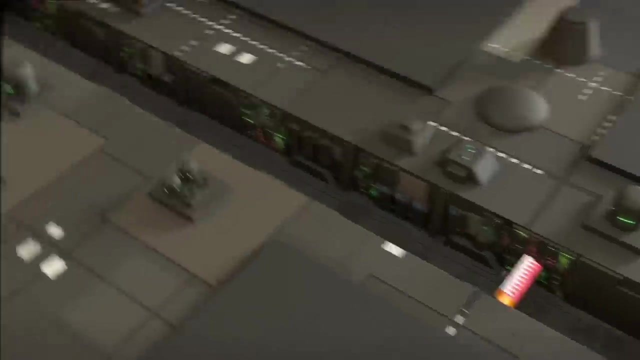 Oh, Wait, this place, I've got just the team switch. Two sixes. we've got a great escape technique. Let's play a game of hide-and-seek. switch Oh 3. Yup, I've got a bad feeling about this. a racist plant, Oh, Do you? 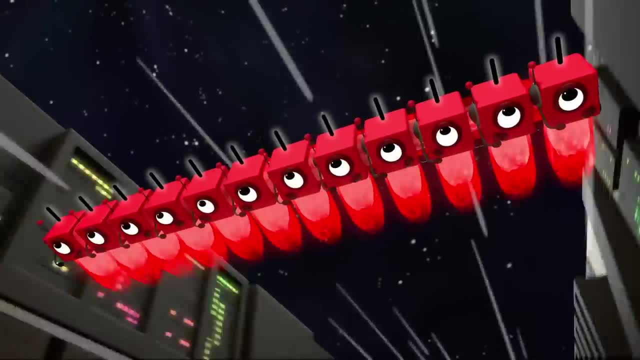 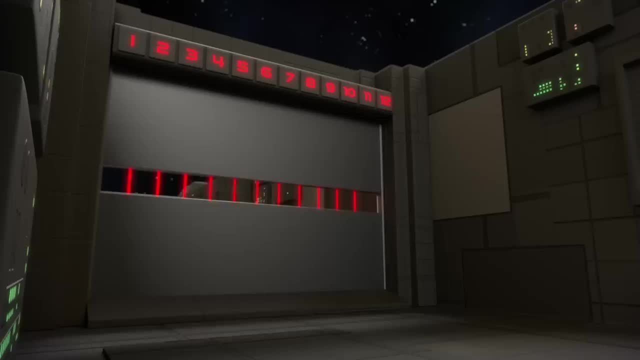 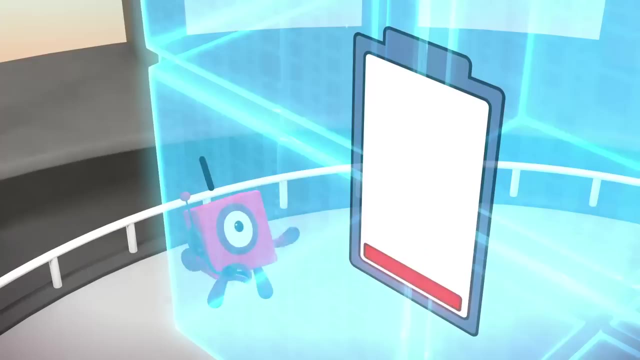 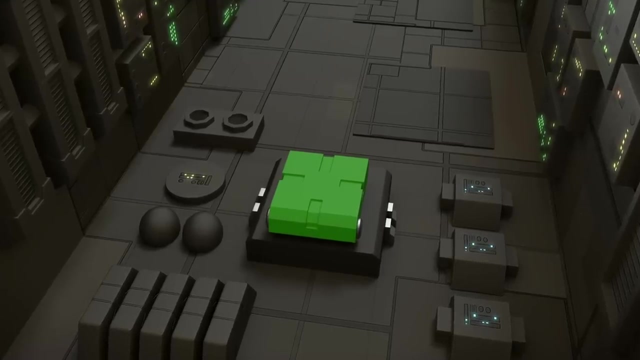 Wow, Look out 12!, 12, what Phew. Wow, Battery level almost dead, but you're right on top of it. You need to open the cover, take out the old battery, then put in a new one as fast as you can. 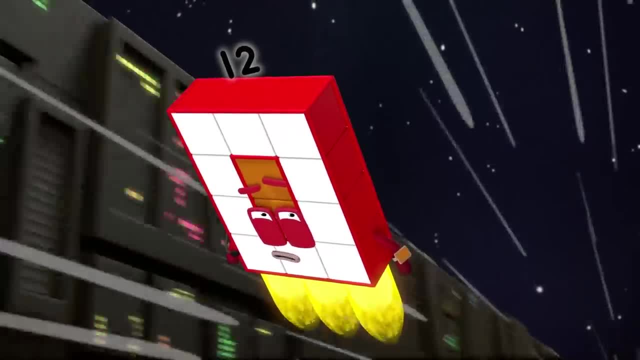 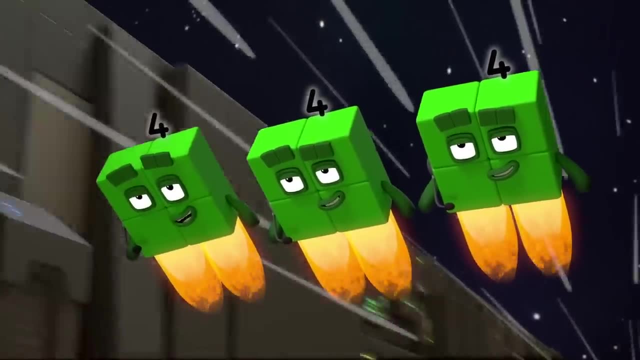 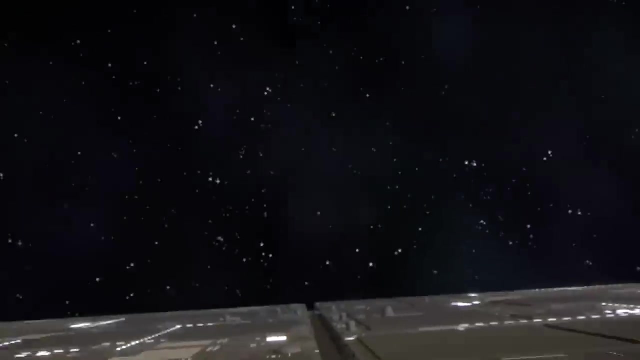 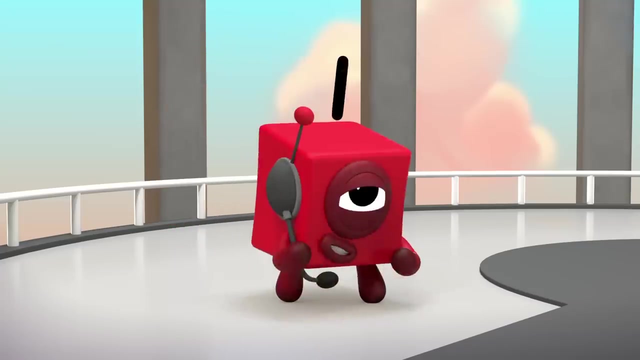 Phew, That's three different tasks, But I can do them all if I use the fours. This is it, Target approaching One, two, three, four. Ho-ho, You did it. Now witness the power of this fully operational disco cube. 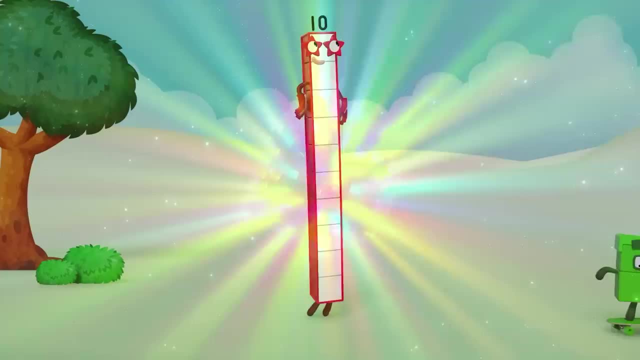 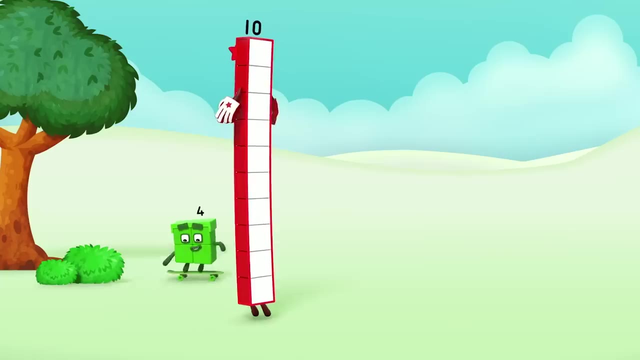 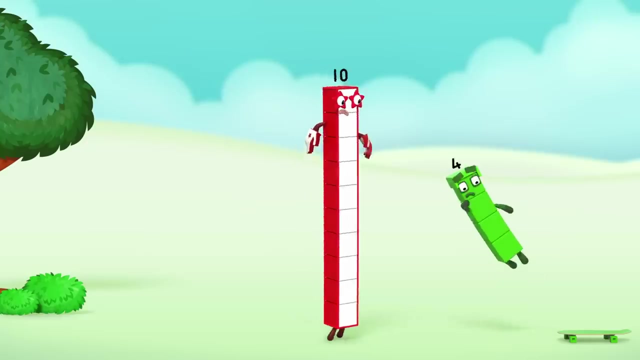 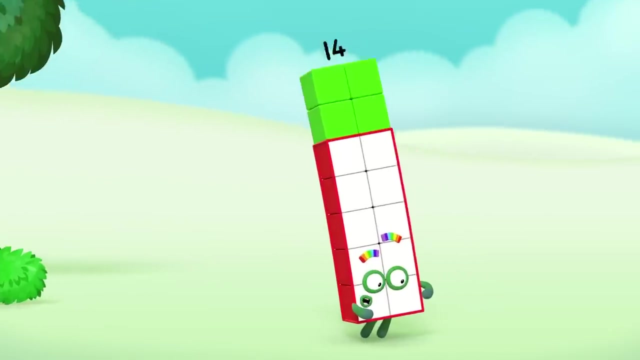 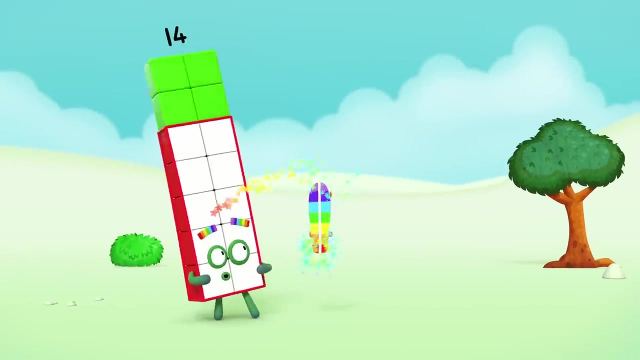 Hello 10!, Hello 4!. Look at my new skateboard: Square wheels. 10 plus 4 equals 40!. Huh, Whoa, I'm a totally new number dude. Check it out. Sweet stripey skateboard. 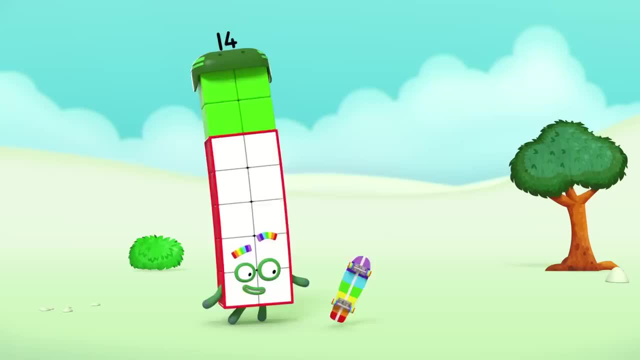 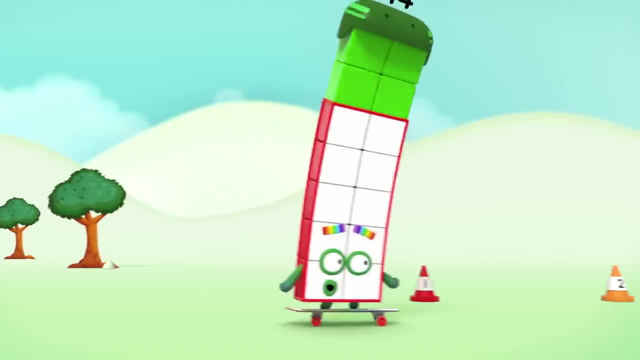 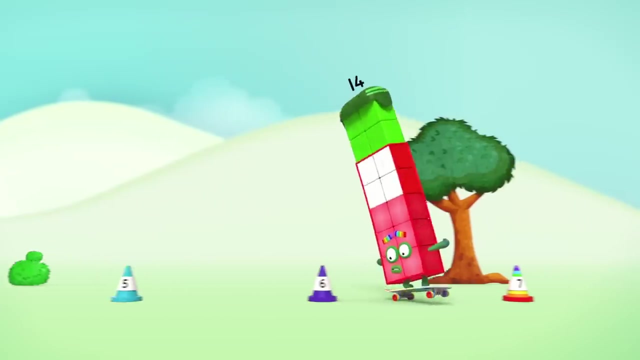 I am 14! And I live to skate. One, Two Oop Three, Four, Five, Six, Seven, Eight, Nine, Ten, Whoa Eleven, Twelve, Thirteen, Four, Five, Six, Seven. 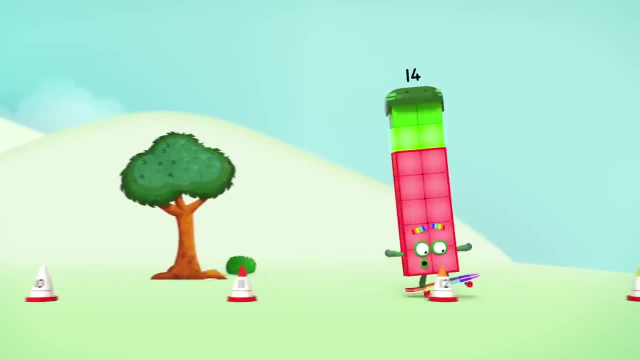 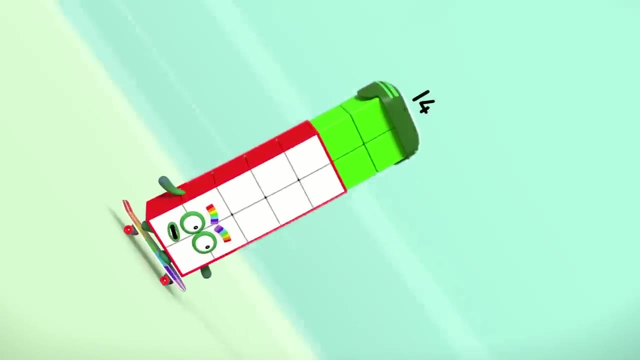 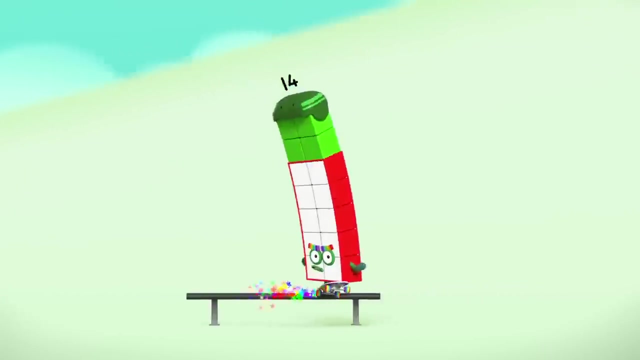 Eight, Nine, Ten, Whoa, Eleven, Twelve, Thirteen, Fourteen, Extreme. I want to be a skater. I want to be greater than the rest. I'm gonna ride to a tail slide. I want to be better than the best. 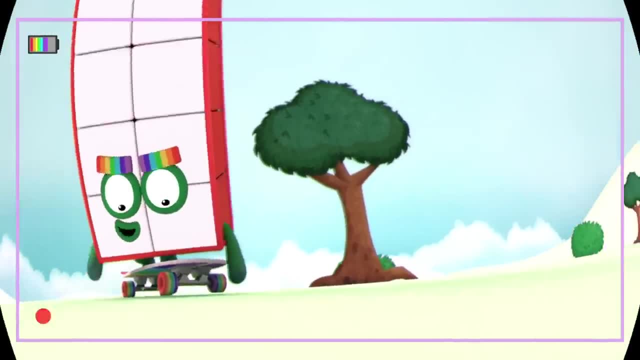 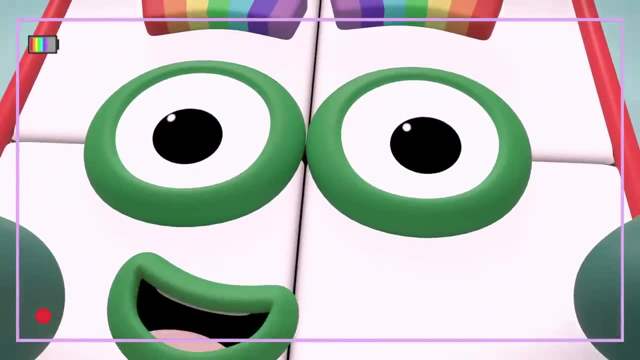 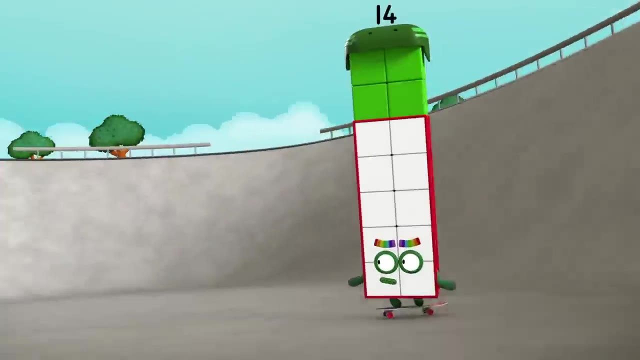 I'm gonna nail all the tricks, All the ollies, pops and cake flips. Trust me, sooner or later I'm gonna be a skater. I'm 14!. I'm ten and four. I'm also double seven. 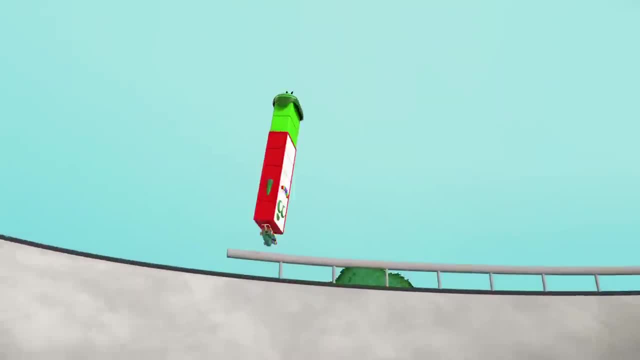 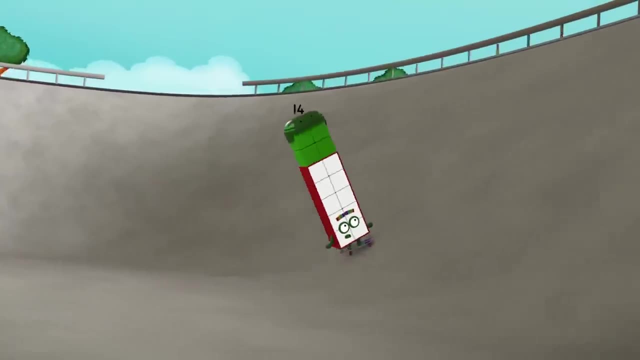 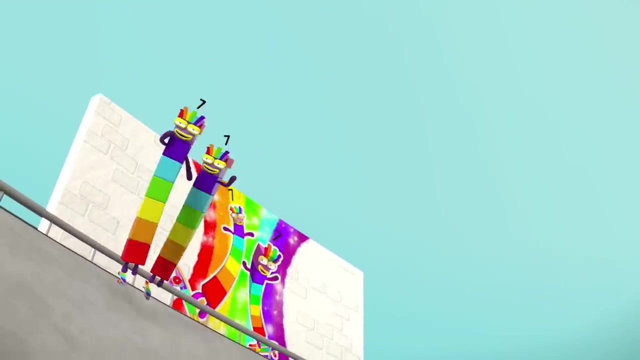 I'm riding on an elevator straight to skate to heaven, And whenever I get into a fix In the middle of one of my brand new tricks, I've got my lucky double To get me out of trouble. Lucky double seven. Maybe you've got a lucky double too. 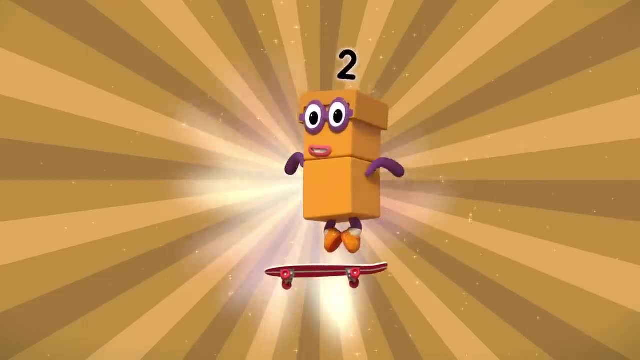 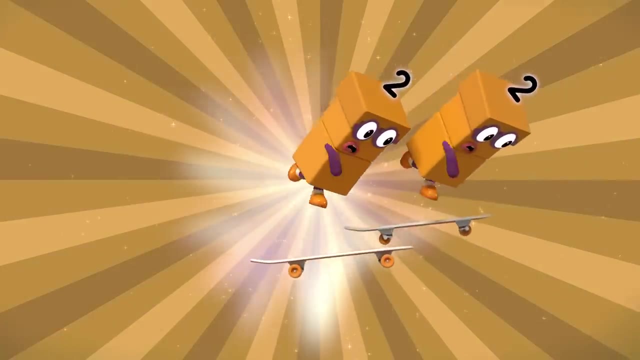 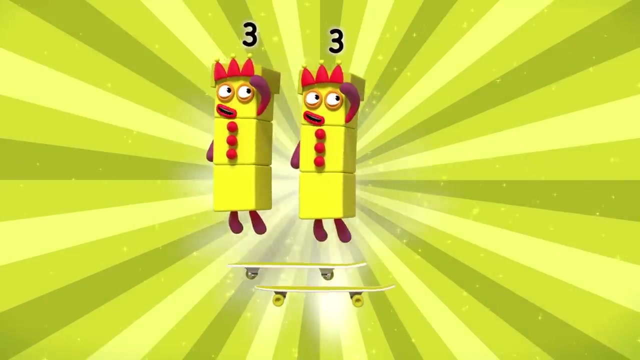 Hello, I'm two And I can split into ones. Double one, double the fun. I'm four and I'm double two. Whoa, two twos. I think we may need grippy shoes. I'm six and I'm double three. Well, we'll be saying, look at me. 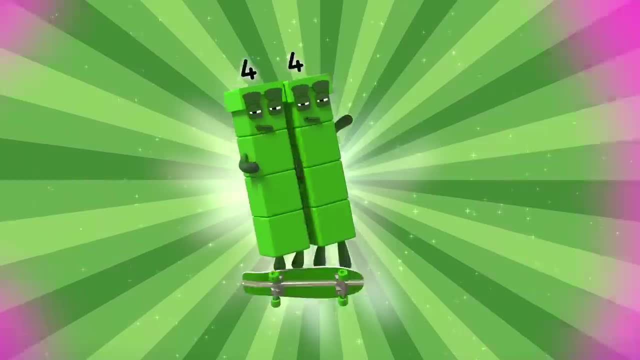 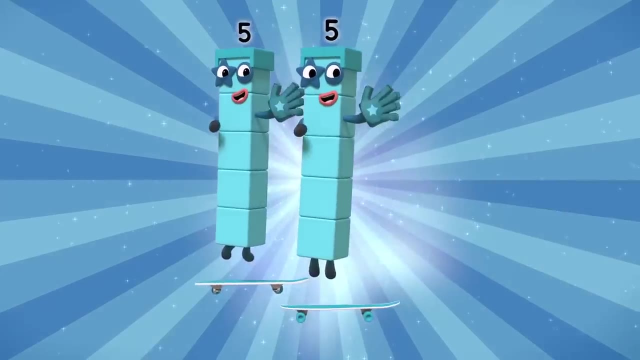 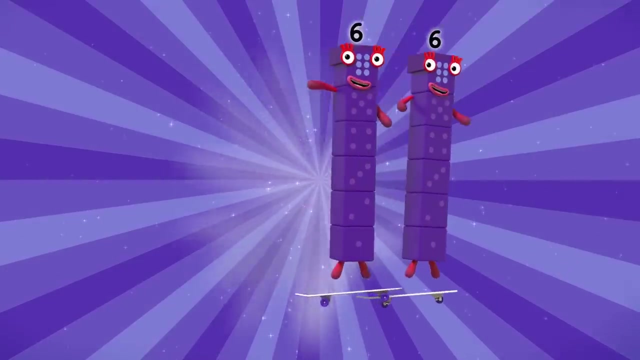 I'm eight and I'm a four and a four, Double four. have you seen us before? I'm ten and I'm double five- Two big hands. Now we can do a double five Hands And jive. I'm twelve and I'm double six. We don't need dice to do these tricks. 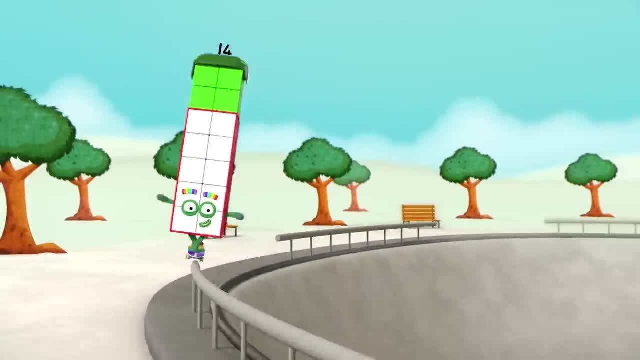 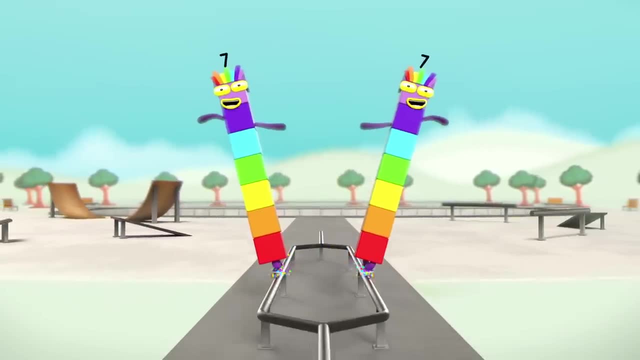 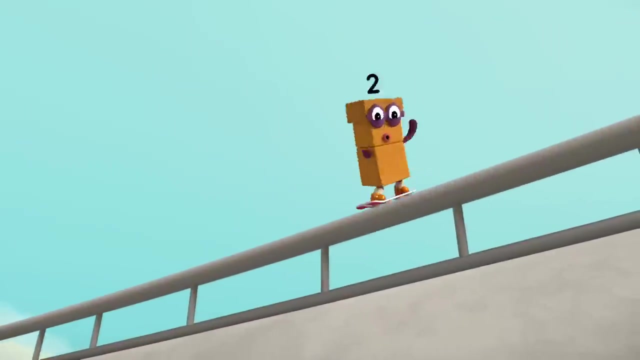 I'm extreme fourteen And I'm keen to show you What my lucky double seven can do. Lucky double seven. Maybe you've got a lucky double too. Double ones make two. Two. Double twos make four. Four. Double threes make six, Six. Double threes make six. 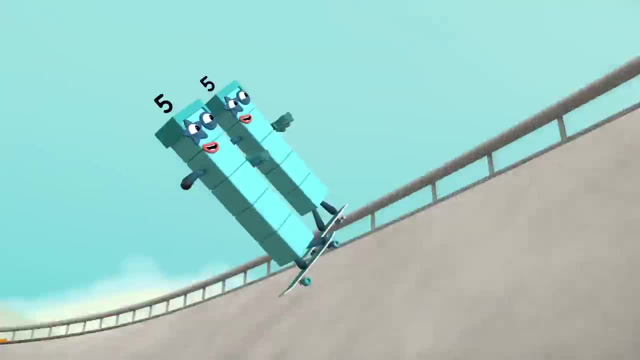 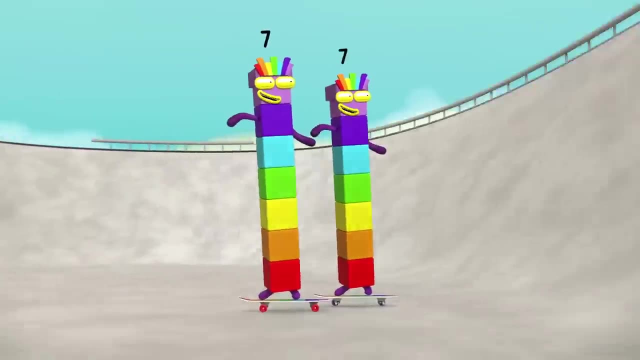 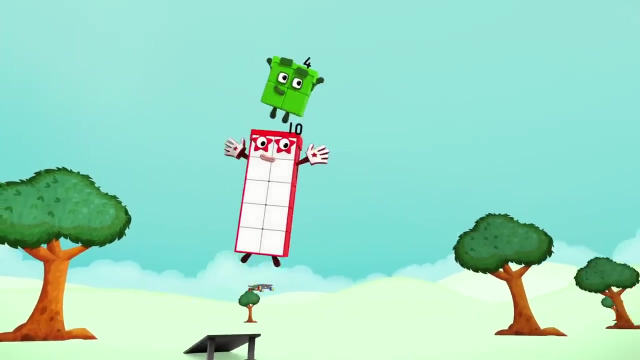 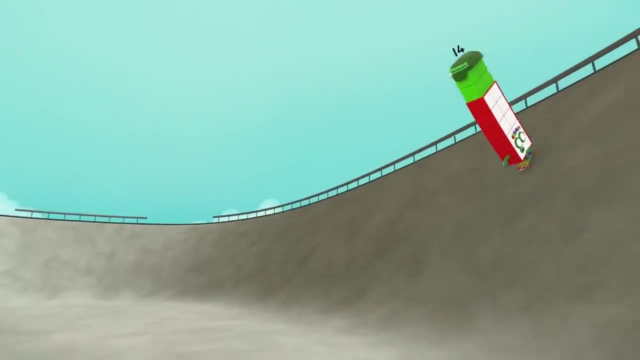 Double fours make eight. Eight. Double fives make ten, Ten. Double sixes twelve. Twelve. Double sevens make fourteen. Ooh, that's us Extreme. fourteen, I'm fourteen, I'm ten and four, I'm also double seven. I'm riding on an elevator Straight to skater heaven. 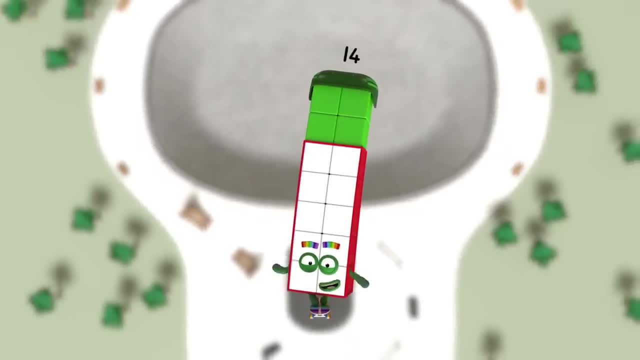 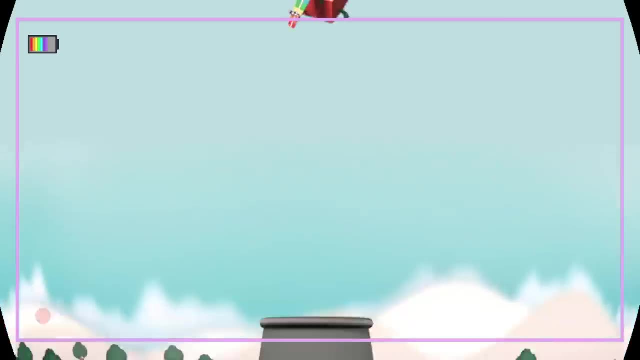 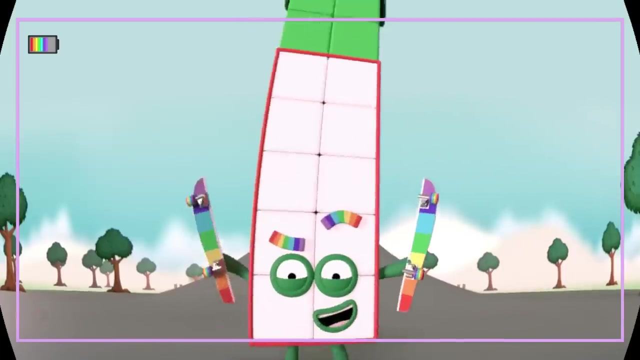 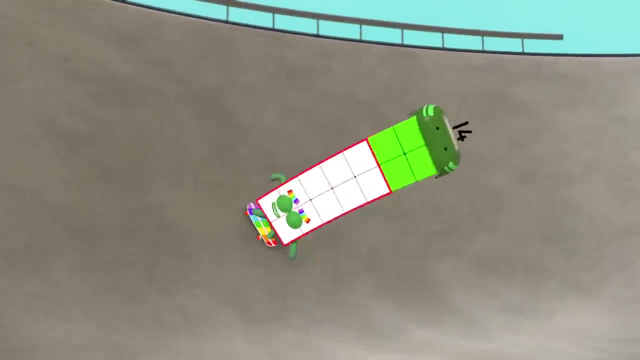 And whenever I get into a fix In the middle of one of my brand new shoes And new tricks, I've got my lucky double To get me out of trouble. Lucky double seven. Maybe you've got a lucky double too. I wanna be a skater. I wanna be greater than the rest. 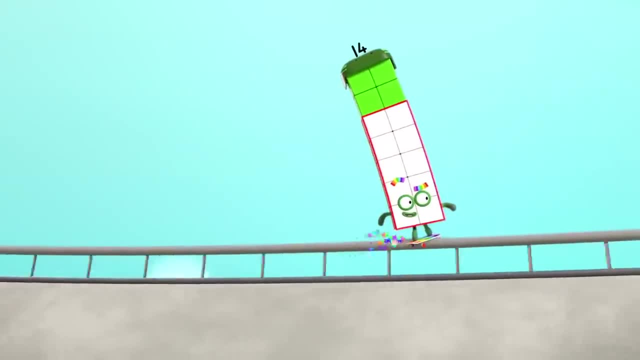 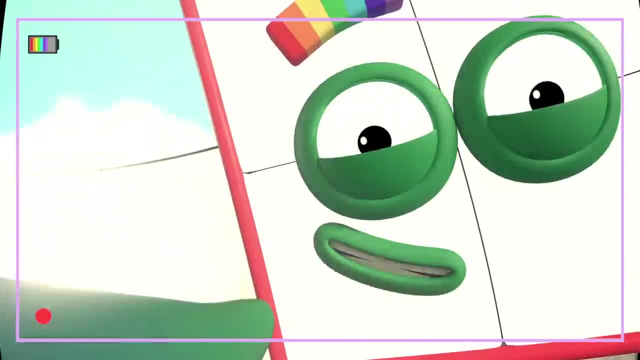 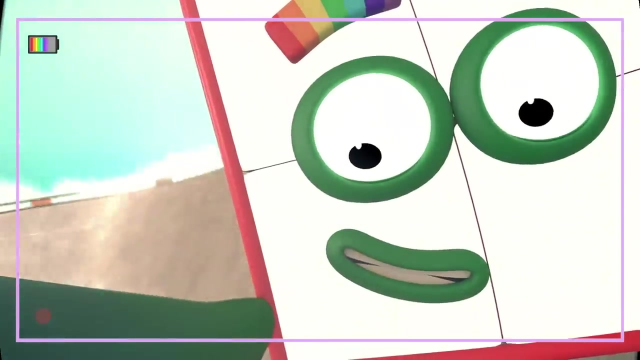 I'm gonna ride, do a tail slide. I wanna be better than the best. I'm gonna nail all the tricks, All the ollies, popsicles and all the other tricks, Pops and kickflips. Trust me, sooner or later I'm gonna be a skater. 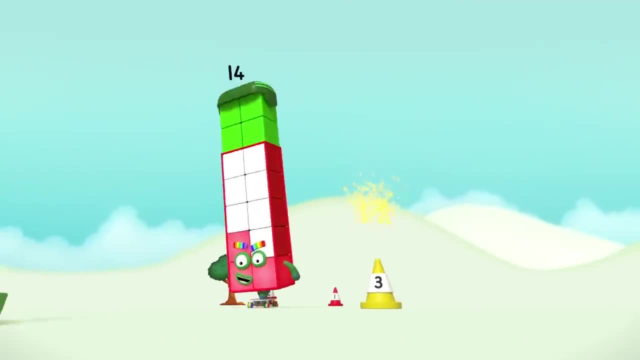 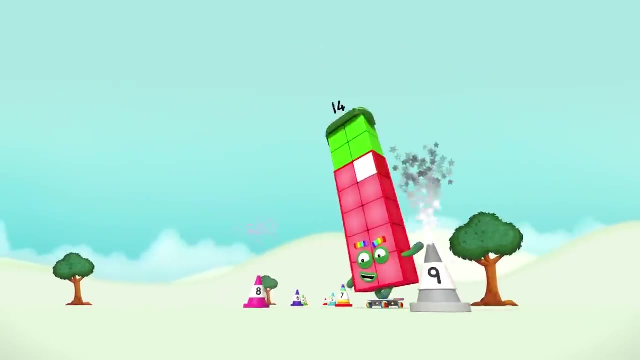 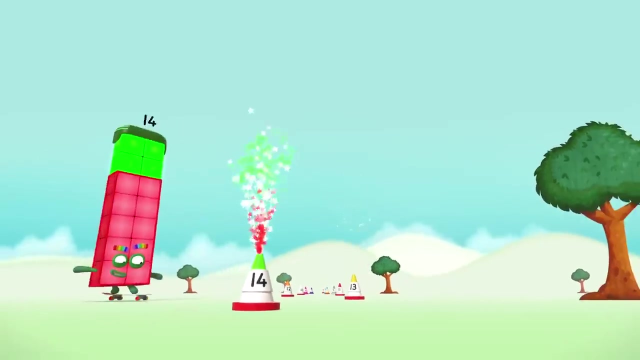 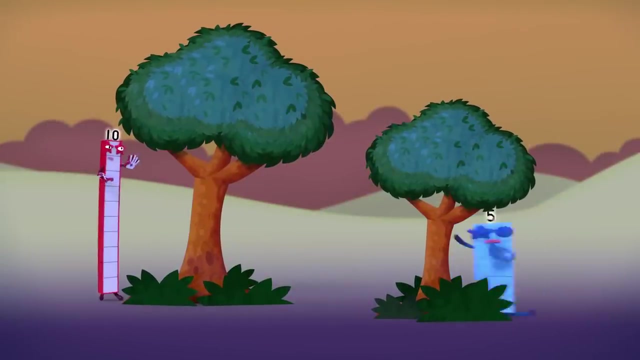 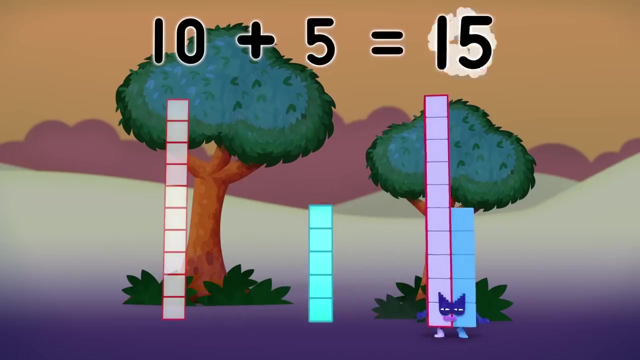 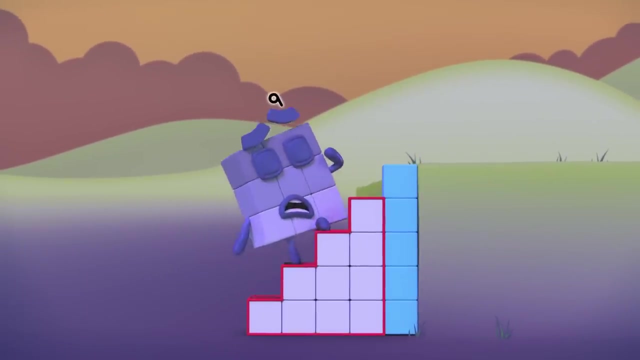 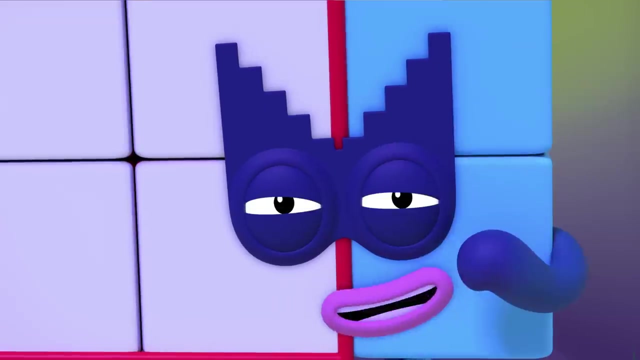 One, Two, Three, Four, Five, Six, Seven, Eight, Nine, Ten, Eleven, Twelve, Thirteen, Fourteen, Thirteen, I wanna be a skater. Yeaah Hush hush. Ten plus five equals fifteen. Hush hush, I am fifteen and I am. 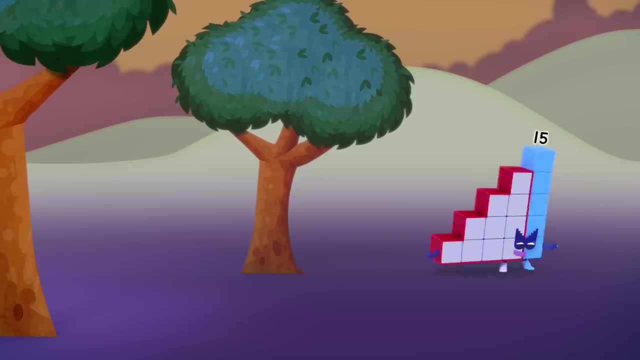 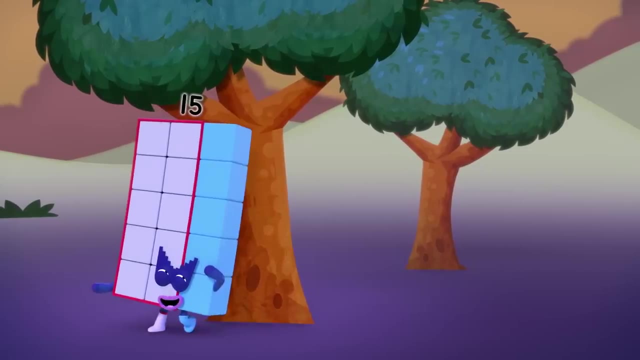 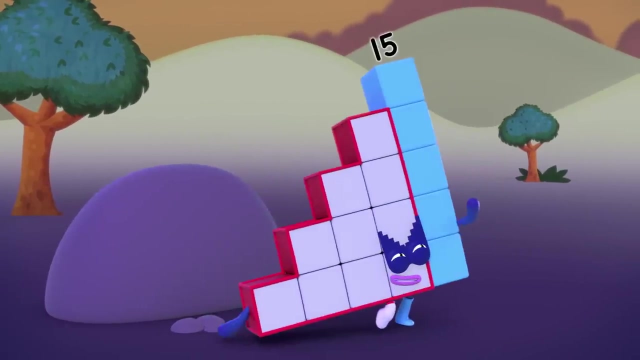 a super special, step shaped secret agent. I'm a number with ambition. I'm a number on a mission, With a talent that you won't believe, Despite my size. I'm a master of disguise And I've got a little trick up my sleeve: Hush, hush. 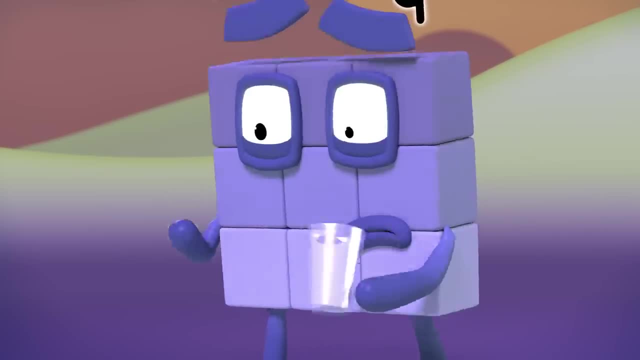 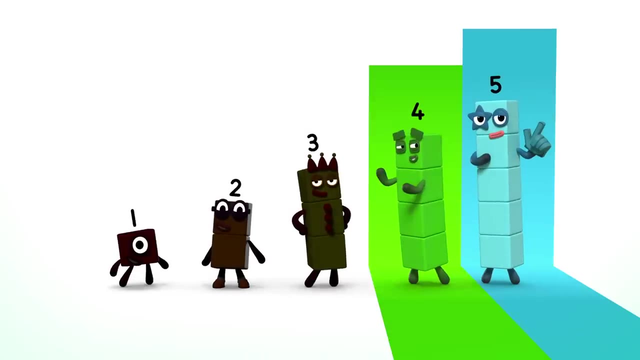 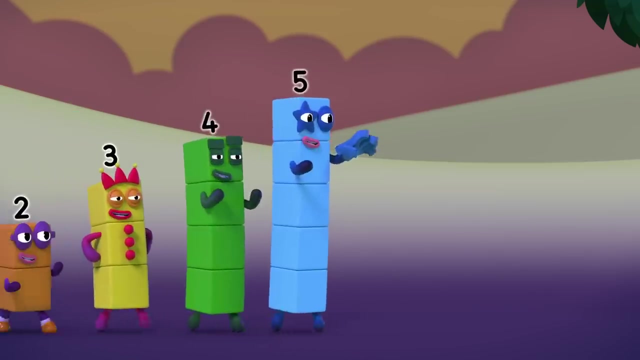 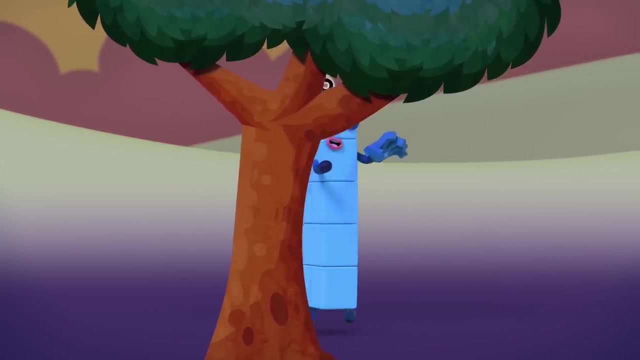 Ah, Help, My biscuit has fallen into my milk. This is a job for Step Squad. Five, four, three, two, one Step Squad. We're the super special secret Step Squad. We can make your problem disappear. We're the super special secret Step Squad. 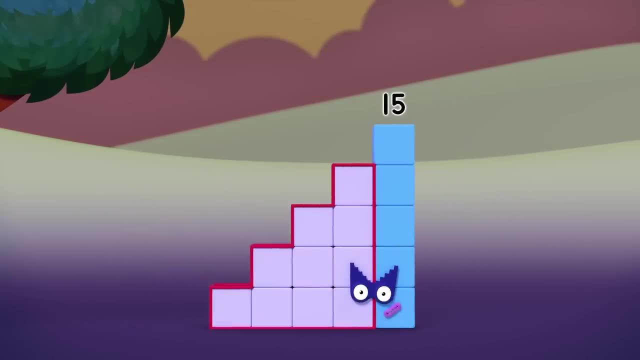 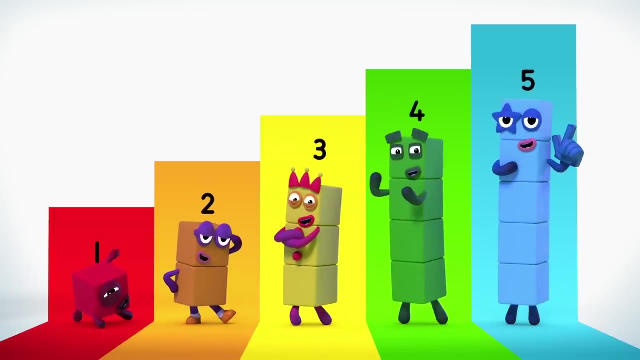 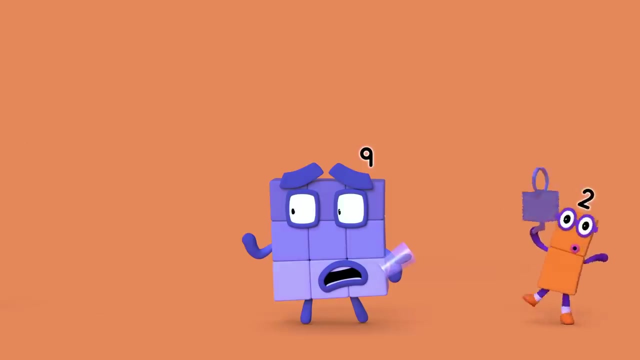 We're gonna make it better. You'll never even know I was here. My super special secret Step Squad is here. Step one: remove the milk. That'll get you started. Step two: remove the biscuits, And now we're on our way. Step three: replace the milk. 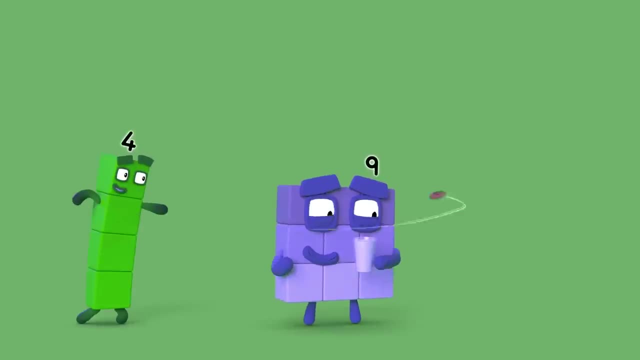 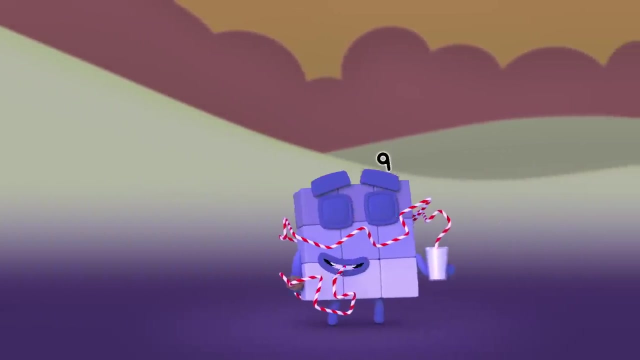 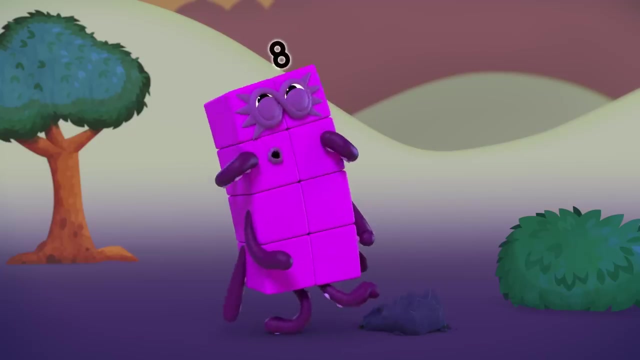 Don't be downhearted. Step four: replace the biscuits, We're gonna save the day. Step five: we're going to overtime As we give you a straw, Thanks, And vanish away. Yum yum, Octoblock. ouch, I've got an octoboo-boo. 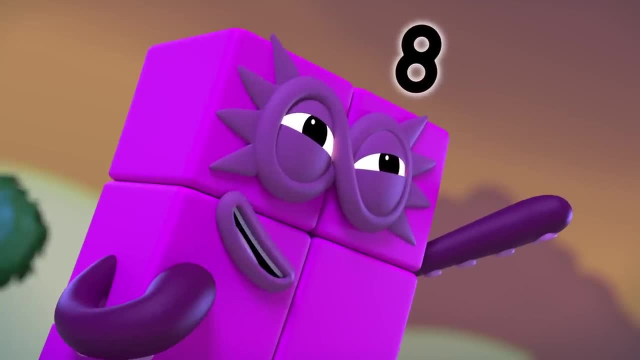 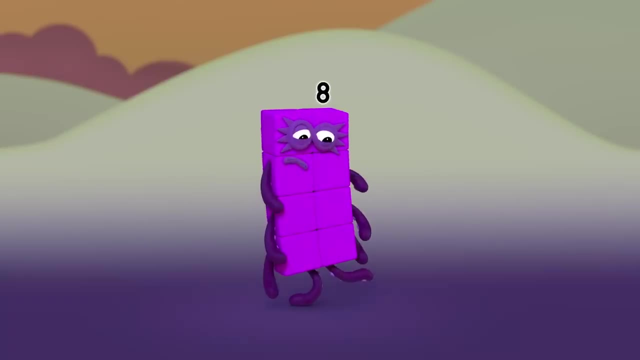 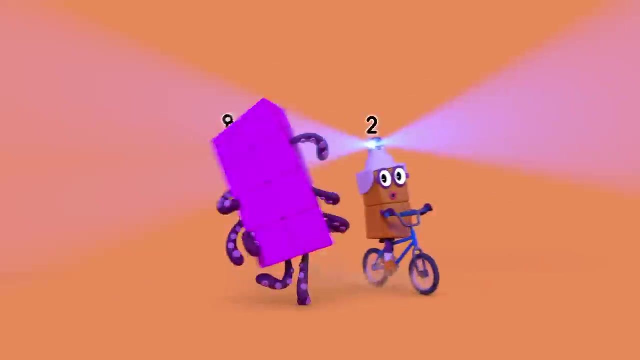 This is a job for Step Squad, The super special secret. Step Squad is here. Step one: check the boo-boo, That'll get you started. Step two: knee-naw, knee-naw, And now we're ready to go. Now we're on our way. 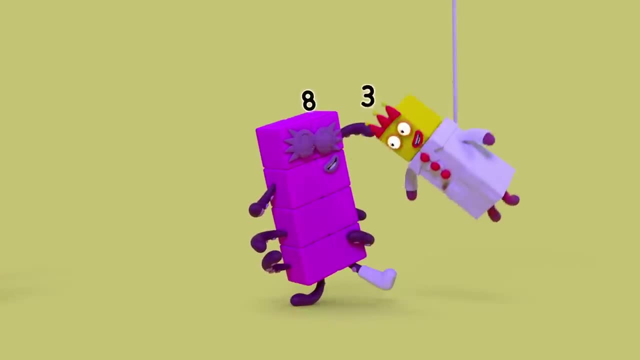 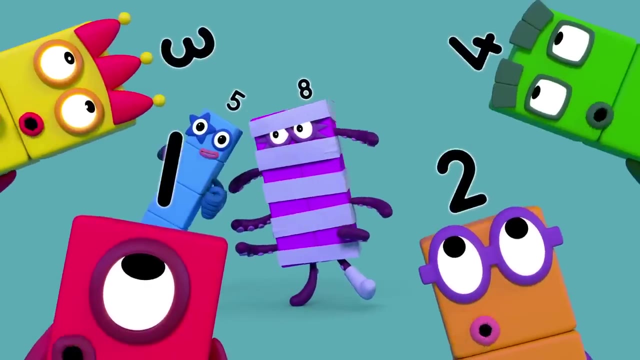 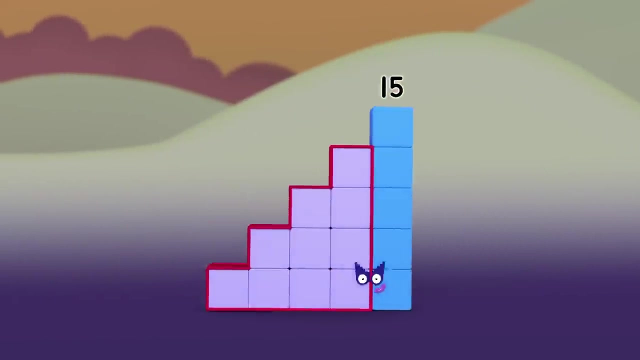 Step three: see the doctor, Don't be downhearted. Step four: bandage- boo-boo, We're gonna save the day. Step five: we're going to overdrive As we make it all better And vanish away. All better now, Meow, Meow, meow, meow, meow, meow. 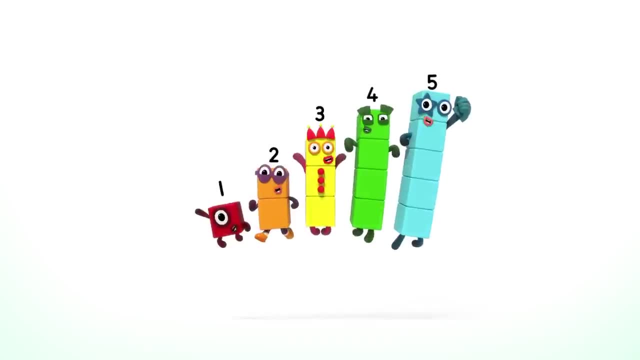 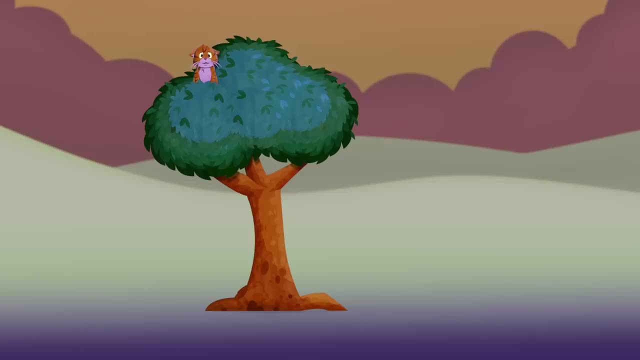 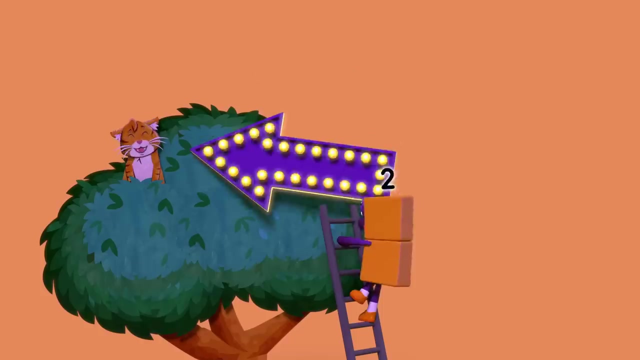 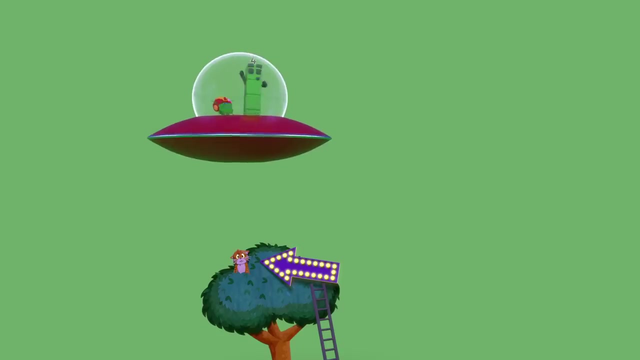 Here's to the terrestrial secret. Step Squad is here. Step one: ginger lauder, That'll get you started. Step two: light up the tree, And now we're on our way. Step three: call an alien, Don't be downhearted. Step four: beam up the cock. 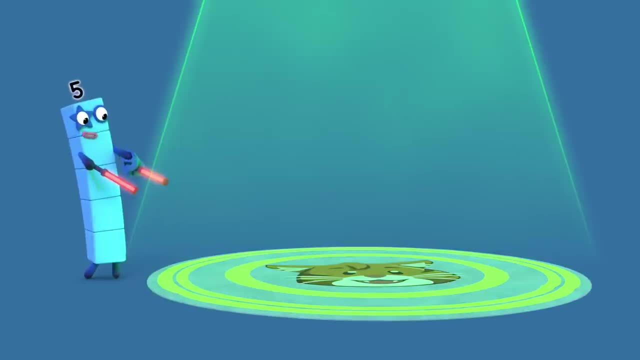 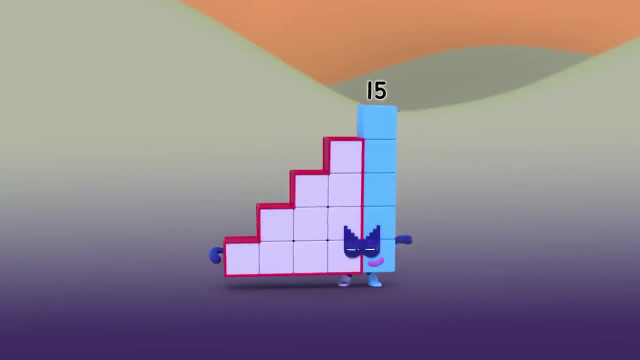 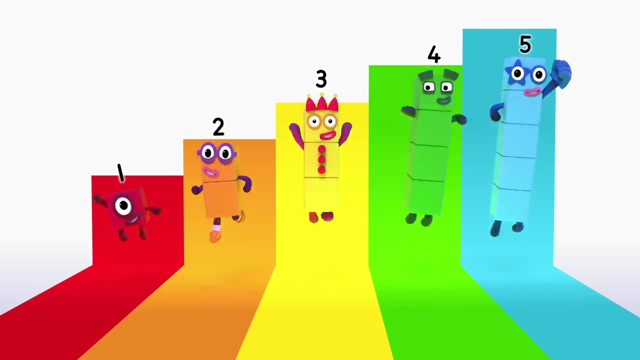 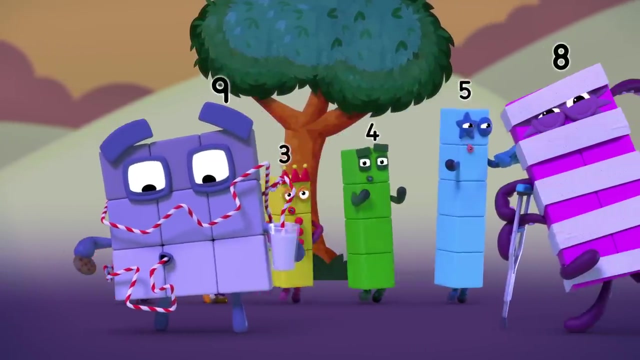 We're gonna save the day. Step five: we go into overdrive As we beam it back down Meow, meow. Five, four, three, two, one Step Squad. We're the super special secret Step Squad. We can make your problem disappear. 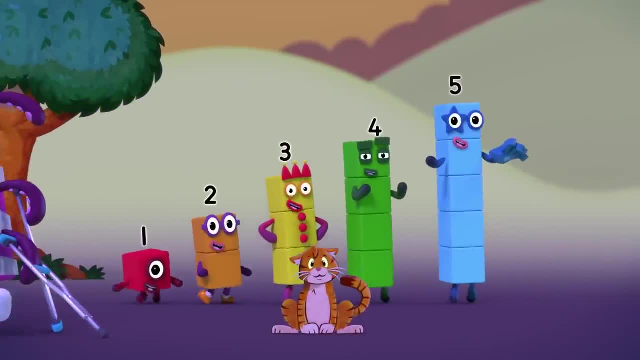 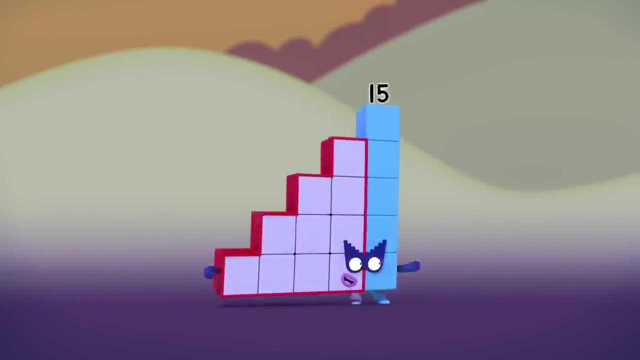 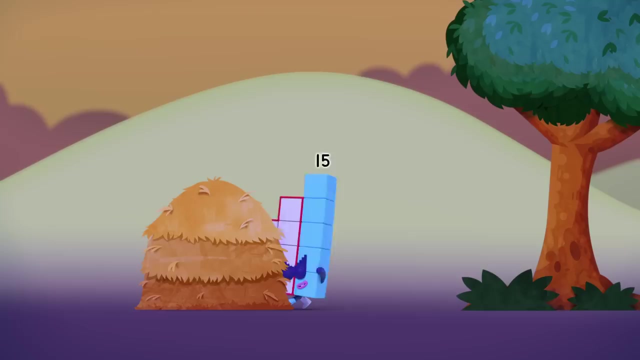 We're the super special secret Step Squad. We're gonna make it better And you'll never even know we were here. I'm a number with ambition. I'm a number on a mission, With a talent that you won't believe. Despite my size, I'm a master of disguise. 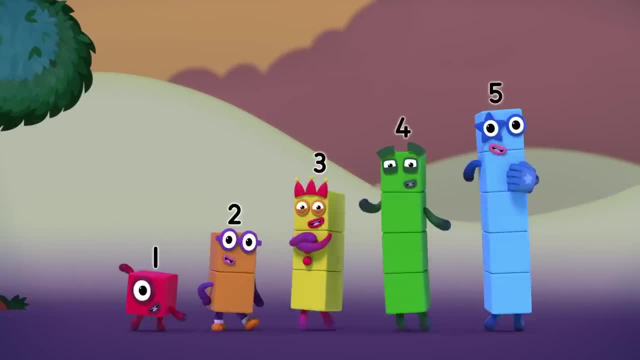 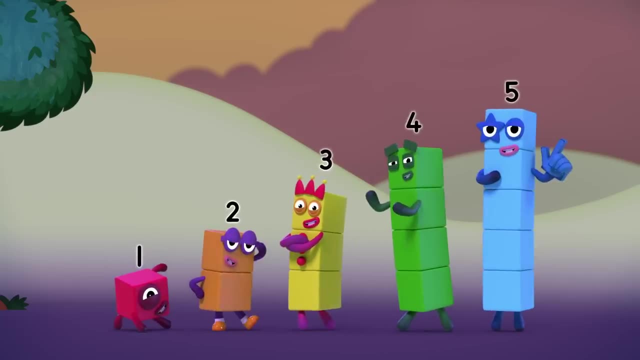 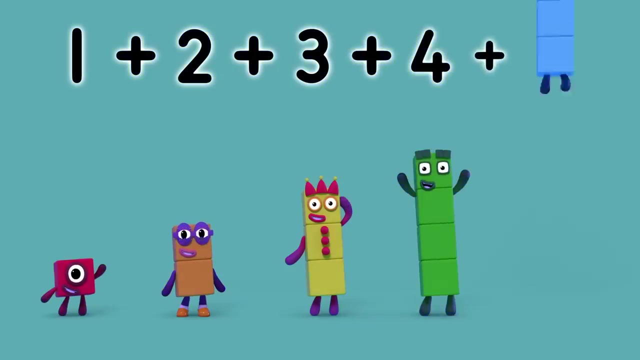 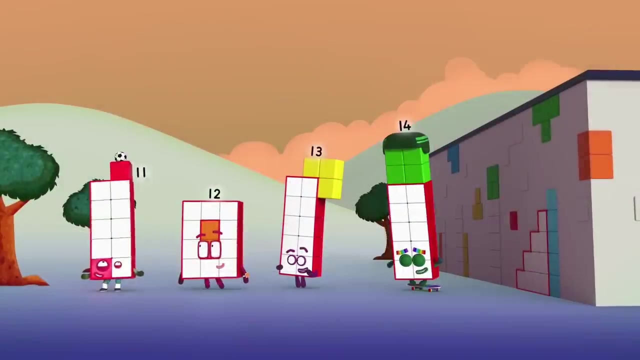 And I've got five friends Who will come and solve your problem. Then we'll leave, Cause we're the super special secret Step Squad. One plus two plus three plus four Plus five equals fifteen Hush hush. One, two, three, four, five, six, seven, eight, nine ten. 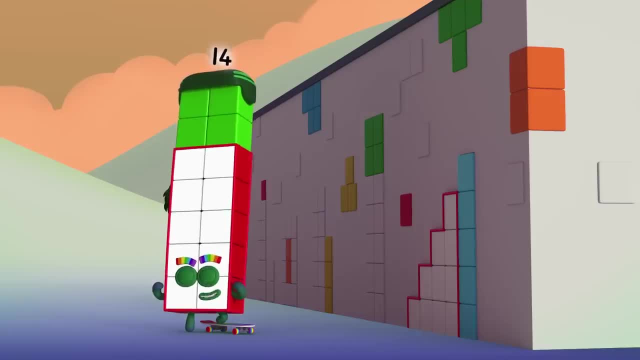 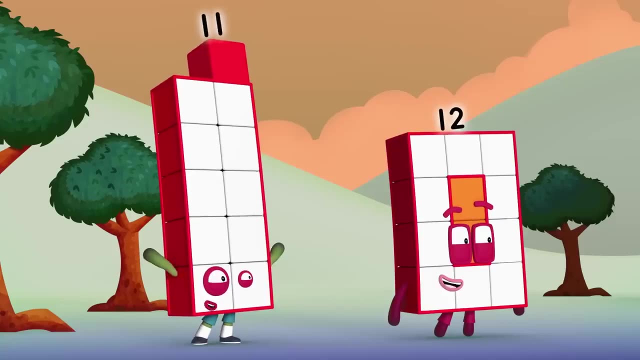 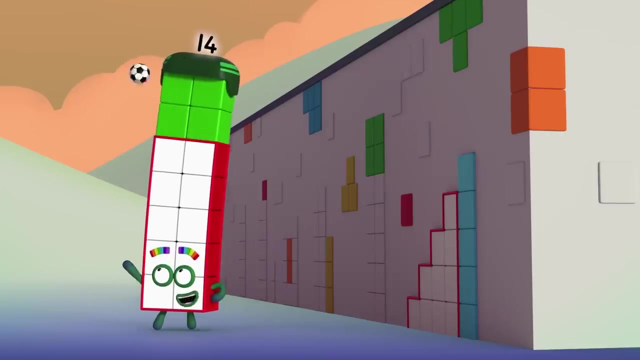 And one more is eleven. Whoa extreme. Let me try. Two heads are better than one. Great idea. Fourteen: Everyone grab a partner for a head-to-ball contest. I'll be the ref. Awesome, I pick twelve. Time for this super rectangle to get in shape. 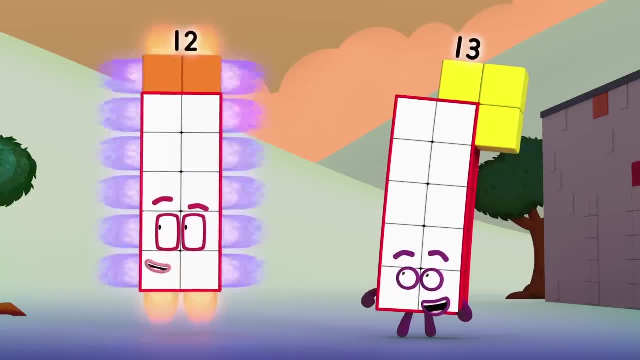 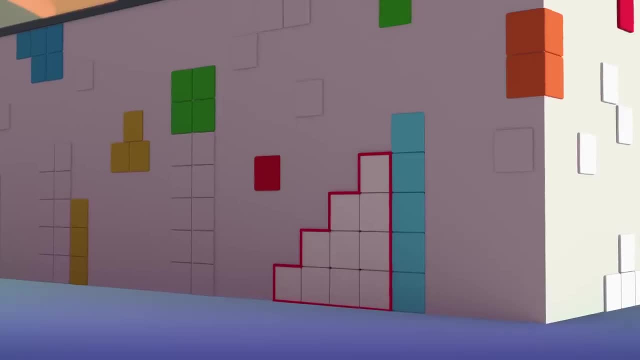 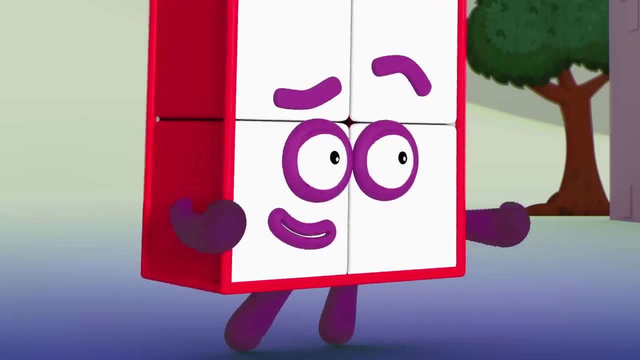 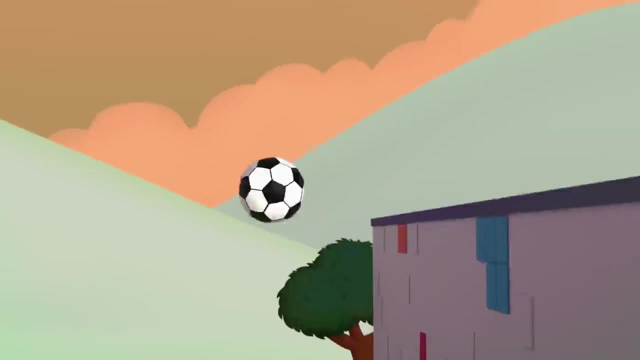 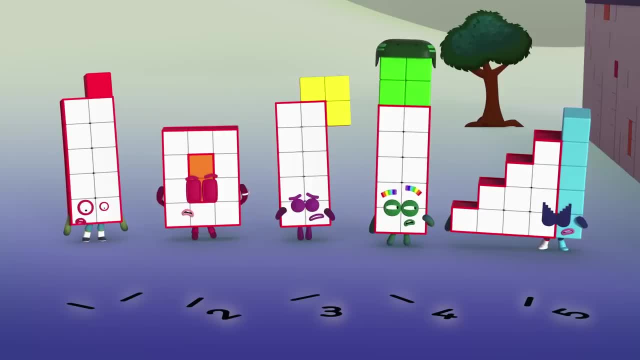 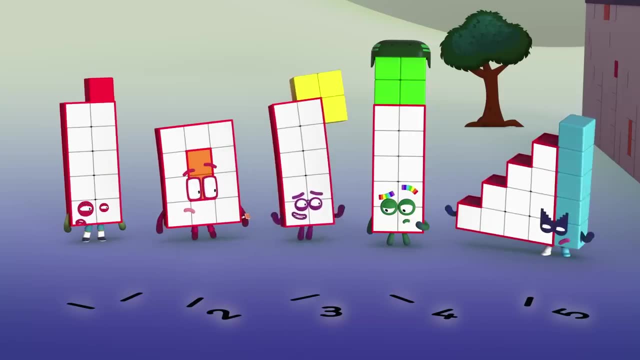 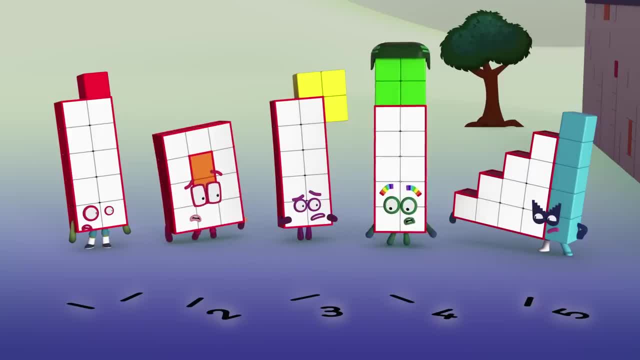 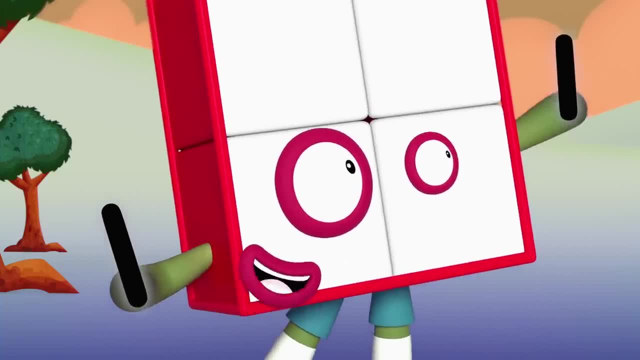 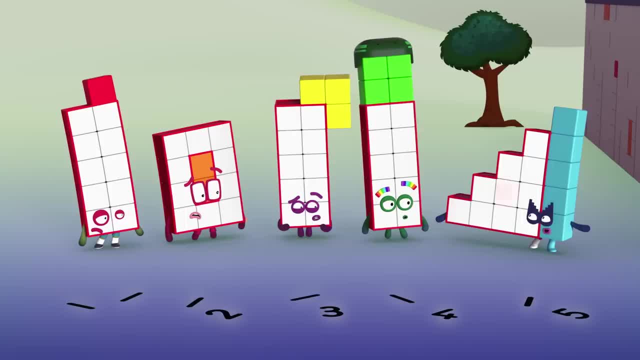 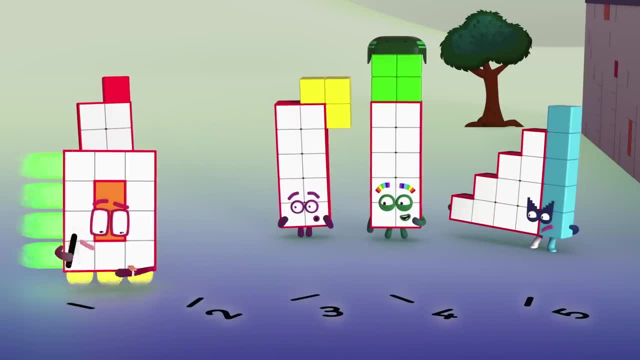 Is that? Anyone feel like number one? Oh, umm, Oh Mm. We've all got more than one block. I've got one umm. Well, more than one. anyway, Arranging things neatly in rows can help. 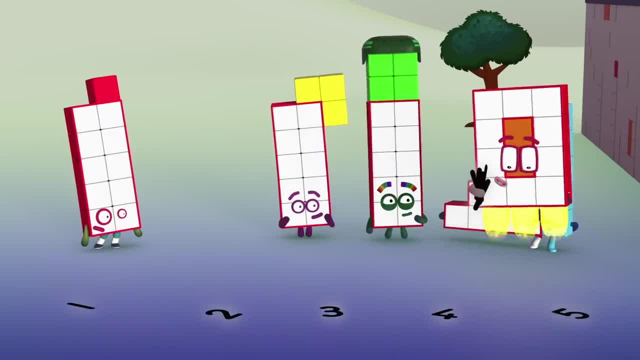 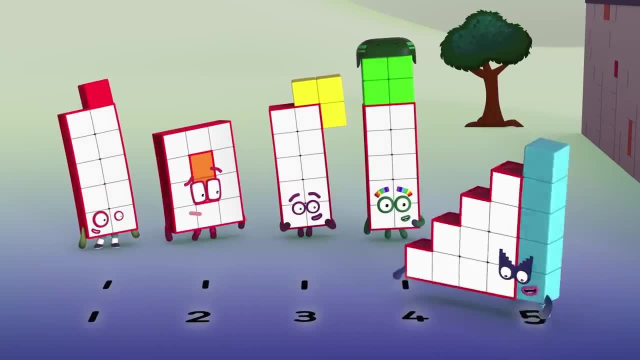 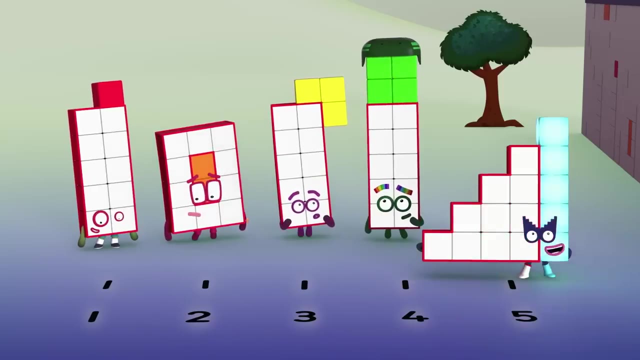 Oh, Huh, Huh, Let's put all the ones here, And then this feels right: One, two, three, four, five. Hmm, That feels familiar. One One, One, two, three, four, five. 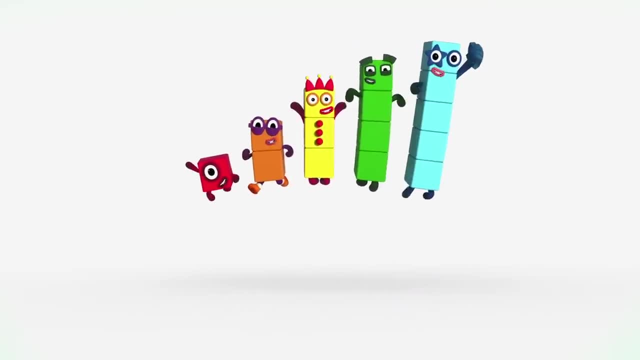 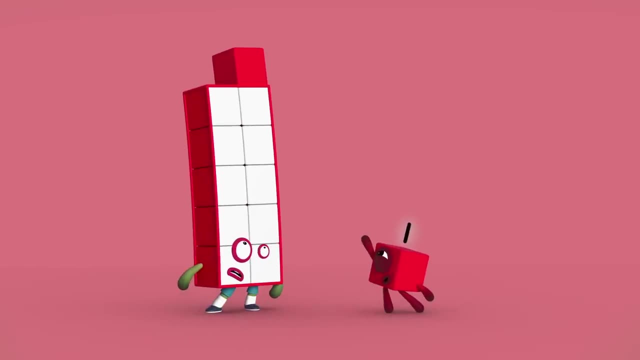 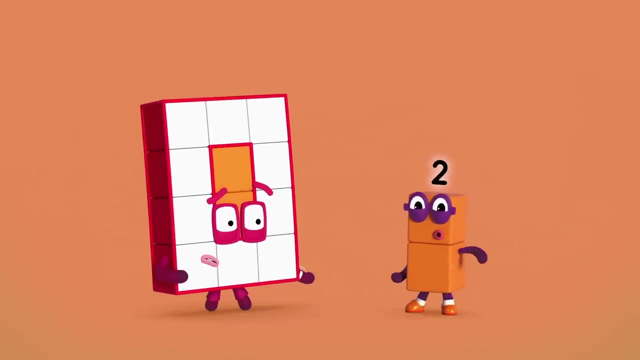 Hush, hush. The super special secret step squad is here. Step one: Look on top of your big block. you've got one red block like me. Step two: You've got two orange blocks like you. Step three: 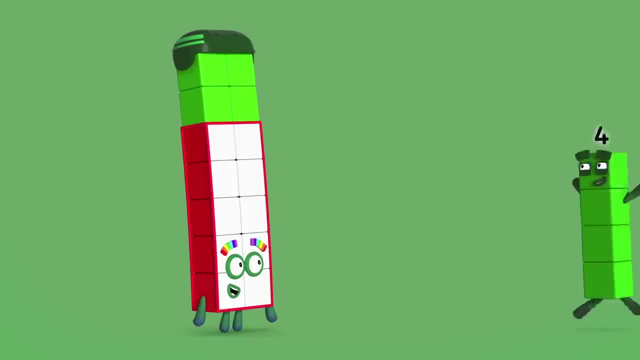 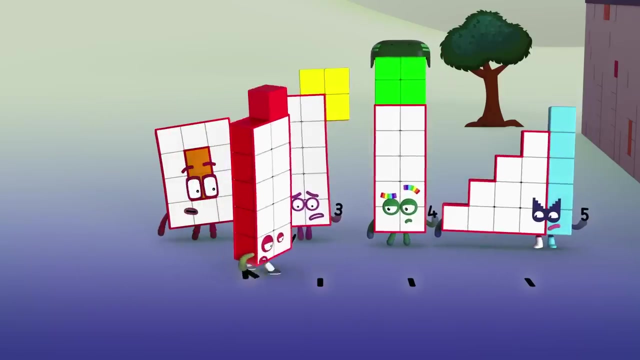 Look at me, Hooray, Hooray. Step four, Four green blocks And step five, Five blue, one blocks, Hush, hush. But what about all these leftover ones? There's enough for one each, But what are they for? 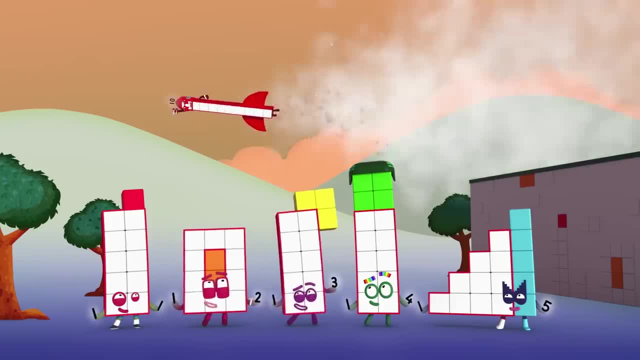 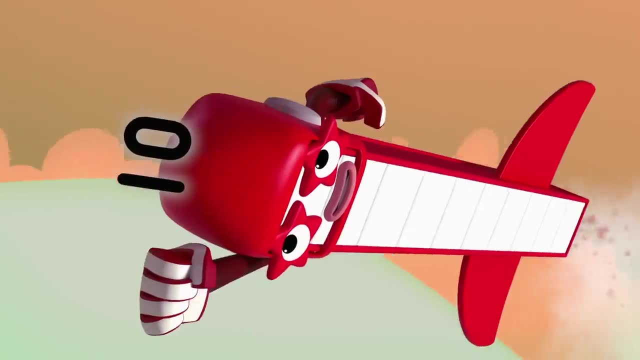 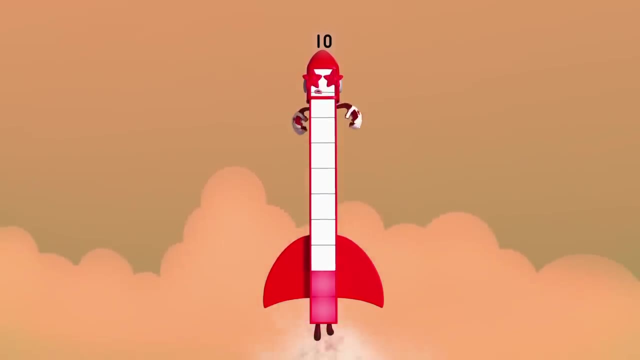 Look up in the sky. Is it a bird? Is it a plane? No, it's a big white block with red sides Coming in for landing in ten, nine, eight, seven, six, five, four, three, two, one. 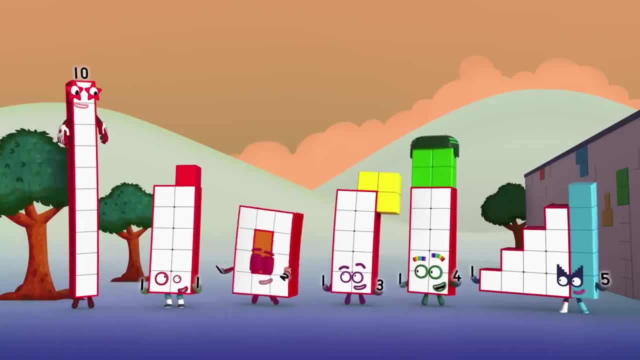 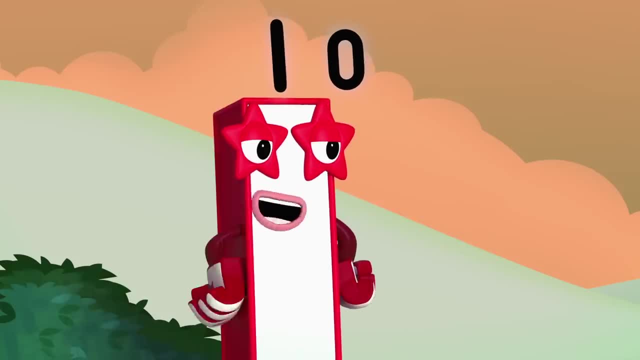 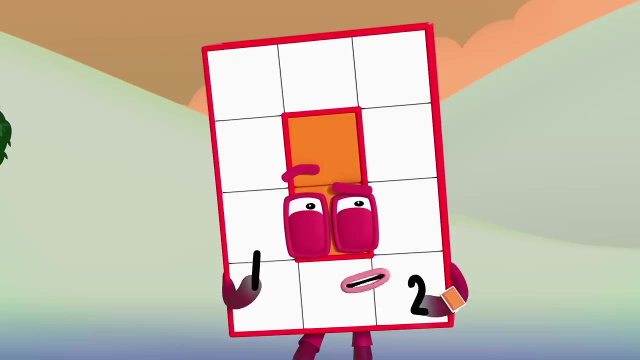 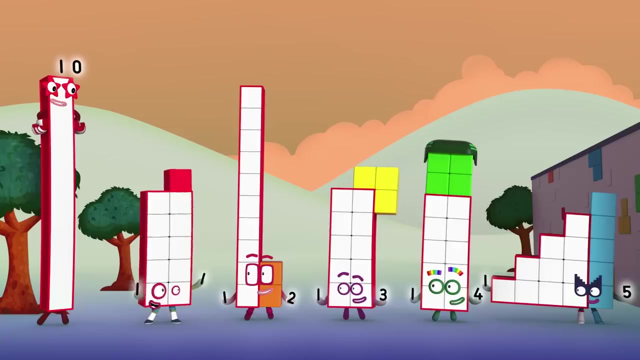 Touchdown Ten, You're ten, Ten, lots of one, Or one ten. This one stands for one ten, One ten and no more, No more ones. Nothing could be simpler. So each of us needs two numberlings: One numberling for the big ten block and one for the rest. 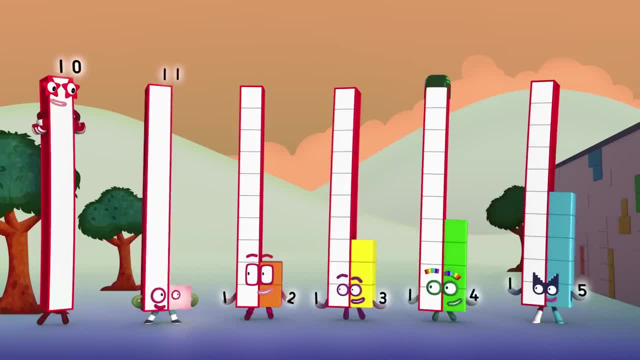 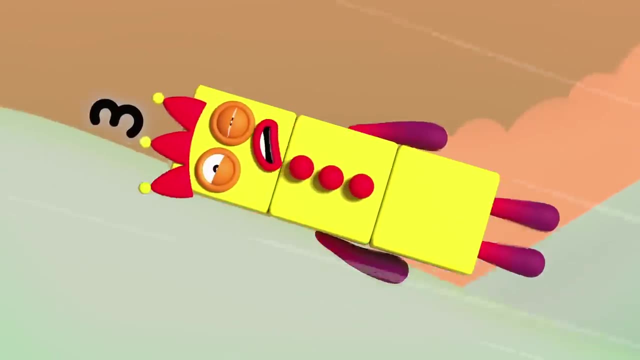 I'm one ten block and one block more. I'm eleven. I'm one ten block and two one blocks. I'm twelve. I'm one ten block and three one blocks. I'm thirteen. Whoa, Duck, Duck, Nice, save ten. 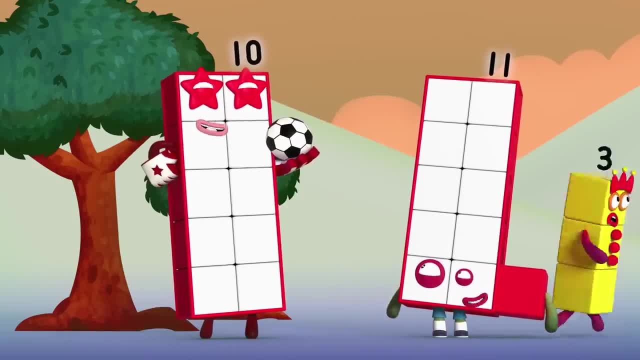 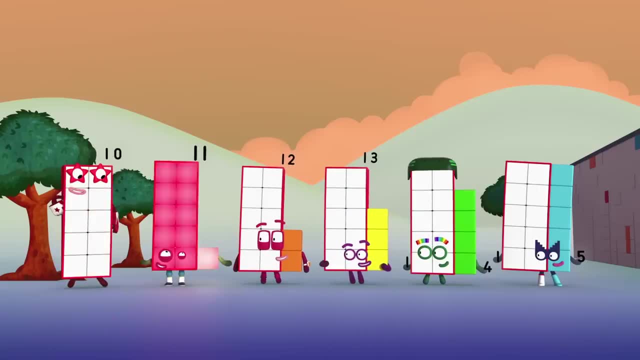 Thanks. Now, where were we? One ten and zero Ten. One ten and one Eleven. One ten and two Twelve, One ten and three, Thirteen. One ten and four, Fourteen, One ten and five Fifteen. 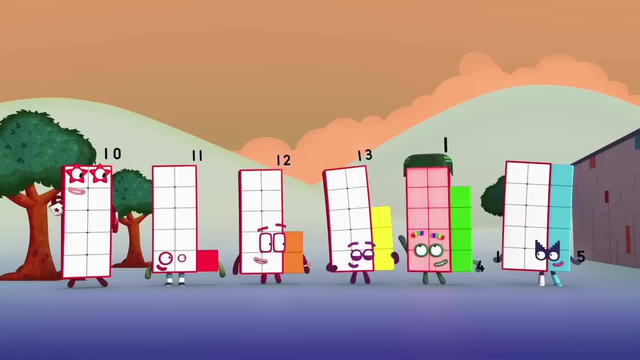 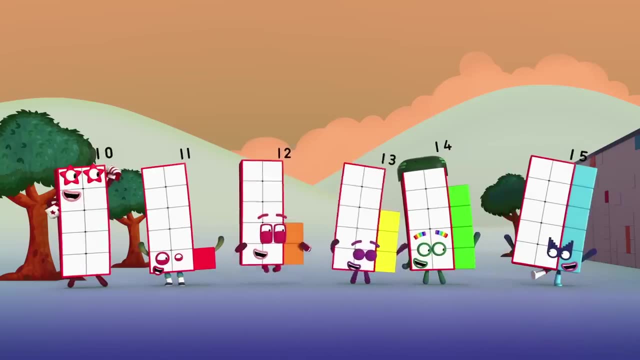 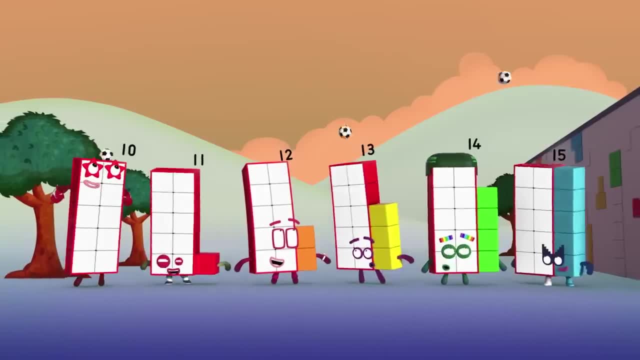 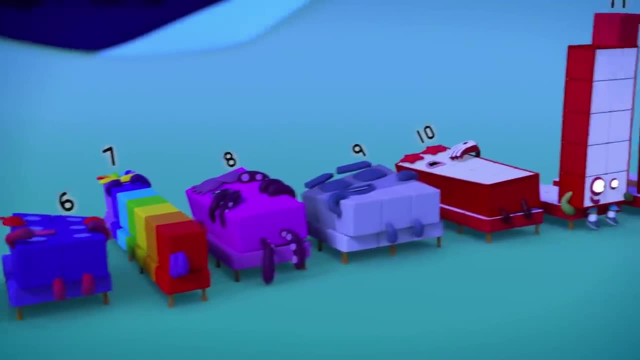 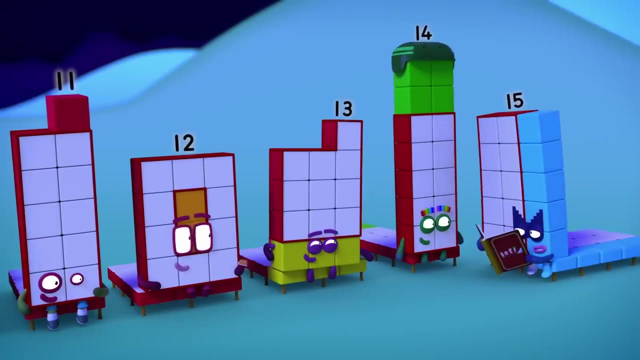 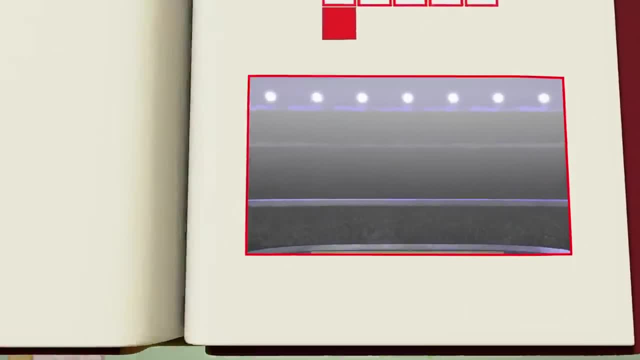 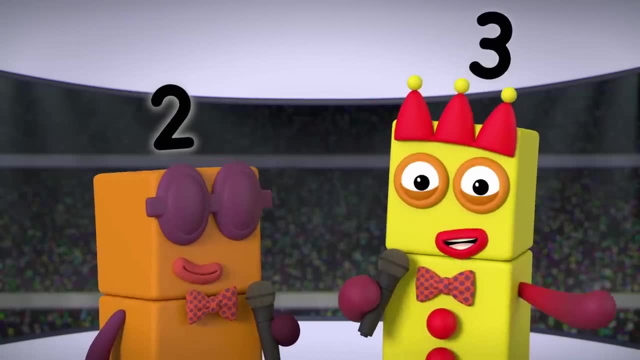 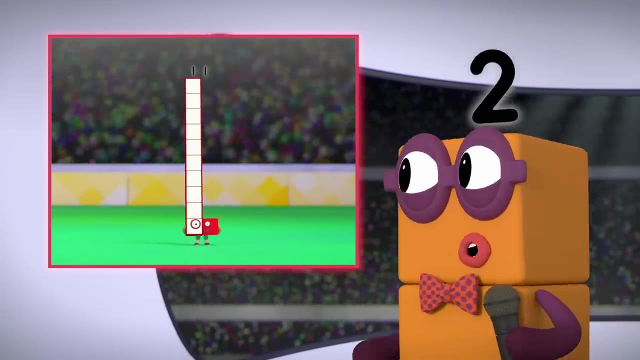 Chapter 11, Back of the Net. With time running out and the score tied at ten goals each, this free kick could decide. I am eleven and I love football. Her numbering's there, standing for one ten block and one block more. 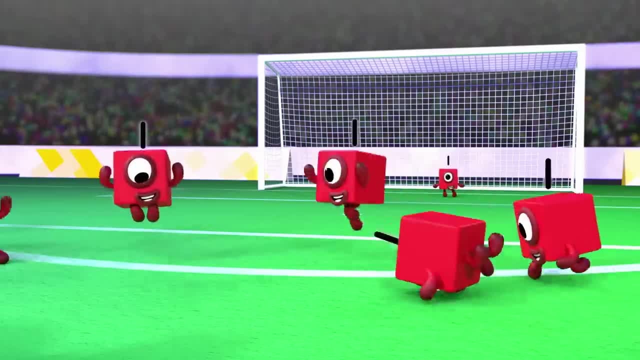 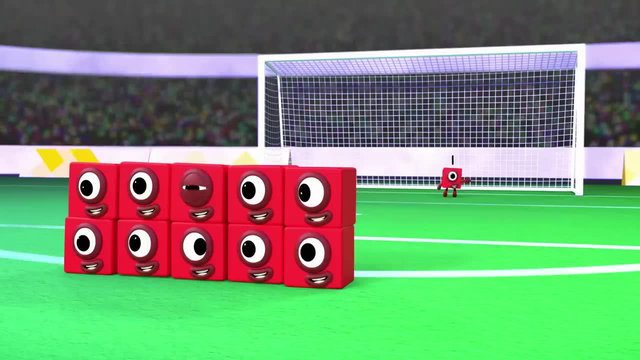 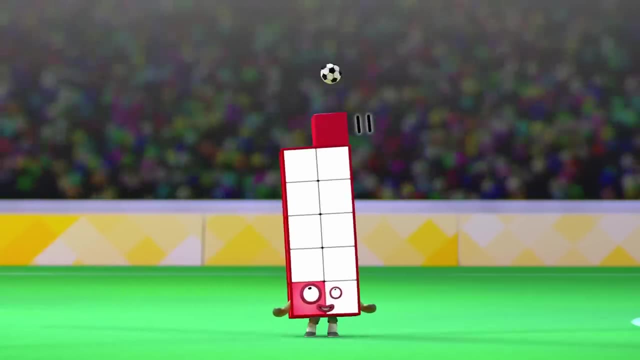 Ten and one making eleven. The defending team, ones united get to make a wall. One, ten, Ten ones And one more. in goal is eleven ones to beat: One, two, three, four, five, six, seven, eight, nine and ten. 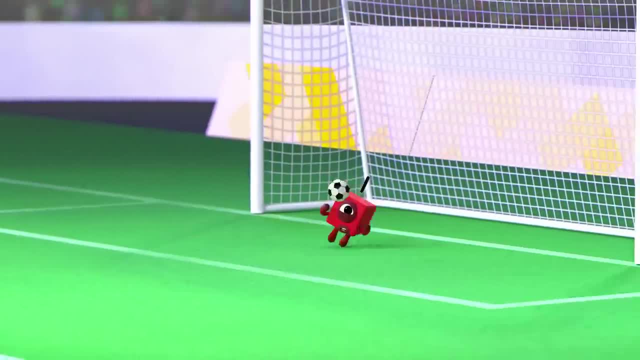 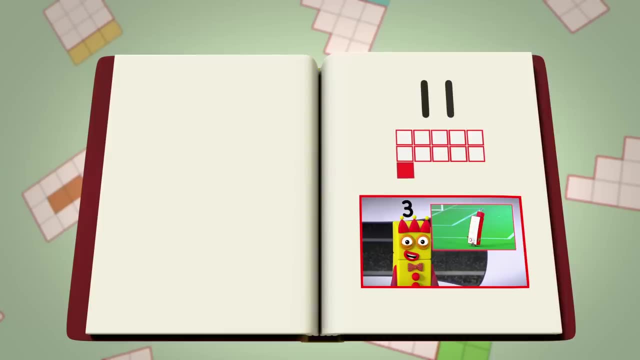 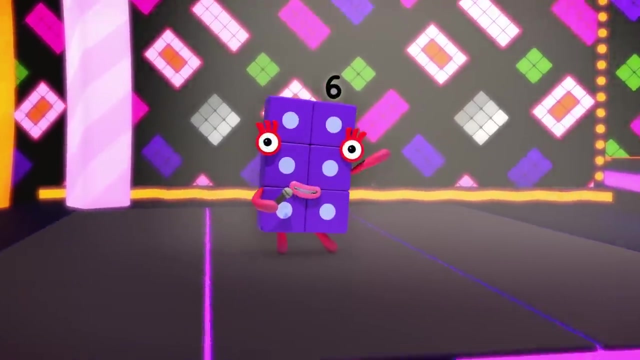 And one more is eleven. She's sent. She scores One, ten, one one. There's only one, eleven. Chapter 12, Rectangle Rush: Yay, Welcome to Rectangle Rush. Let's see who's next to brave the crush. 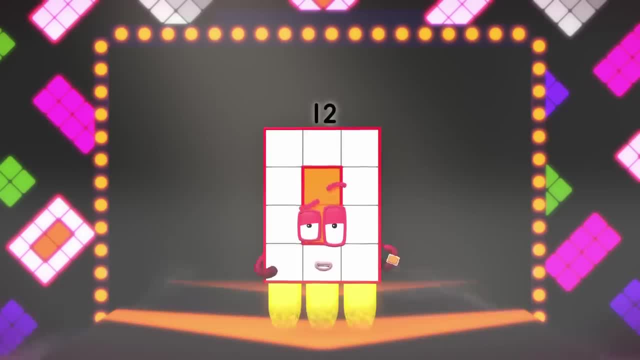 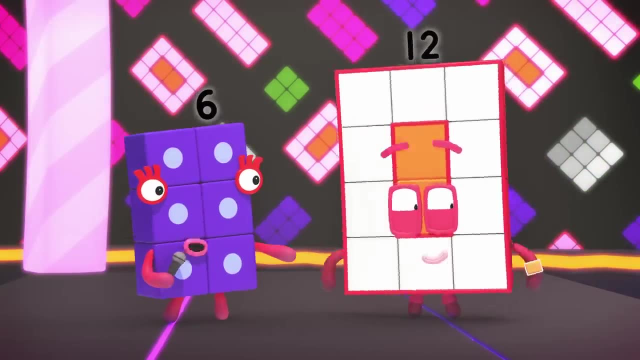 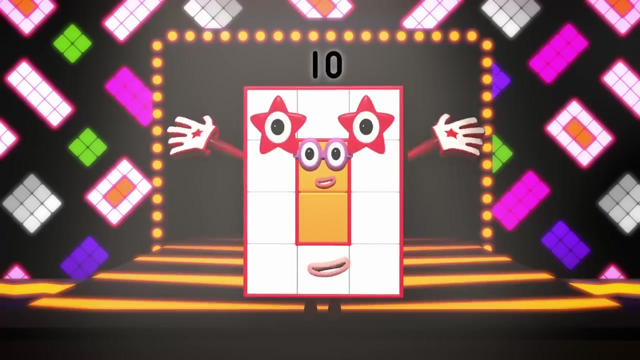 I am twelve and I am a super rectangle. That means I can make lots of different rectangles. Show us what you've got Game on. I am twelve, I am ten and two And I am three blocks by four blocks. I am. 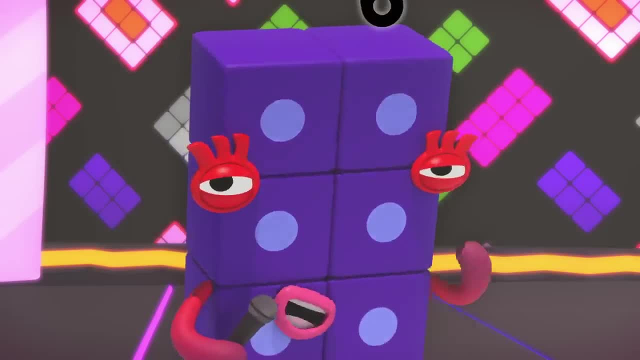 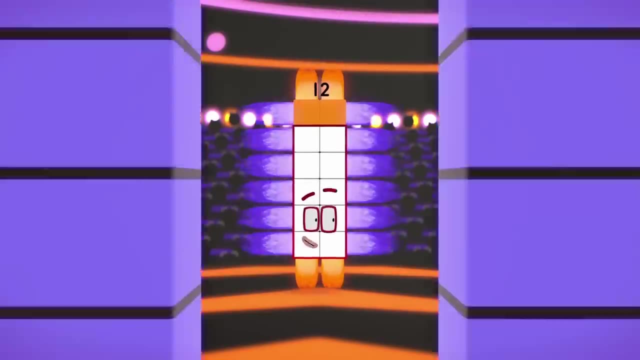 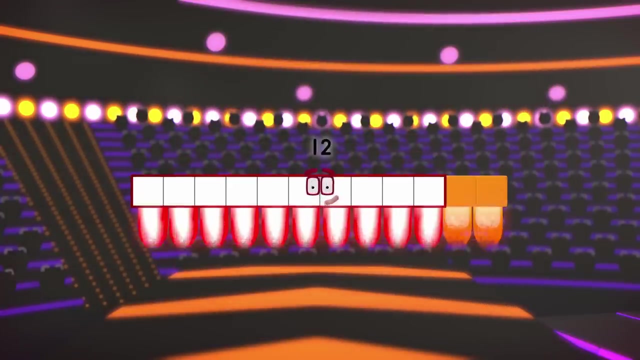 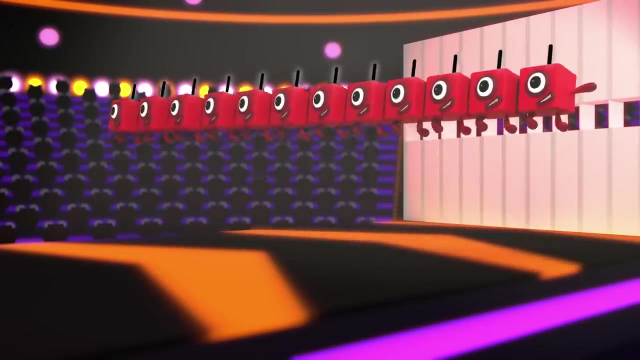 I am a rectangle, Ooh, rectangle race Turn. I am four by three Switch. I am two by six Turn. I am six by two Switch. I am twelve by one, Which means I am also Twelve blocks of one. 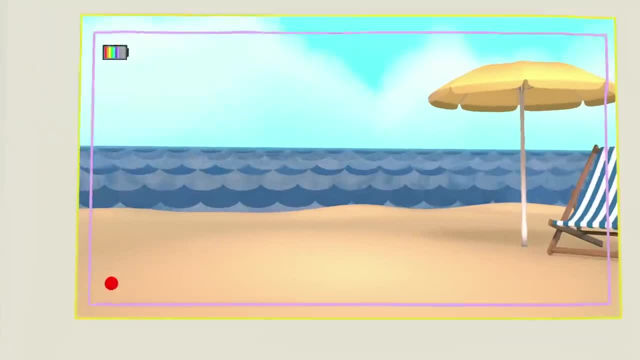 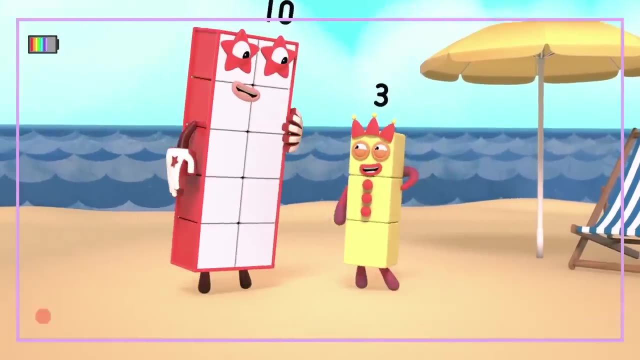 I am seven by eight When the triangle shifts one. What about the triangle? It is one by two Is helping? It is helping. What about when one half, one half And I lose all of the bonds of the triangle? so I win the game. 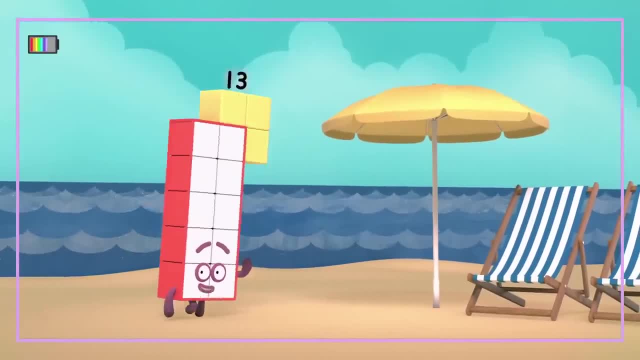 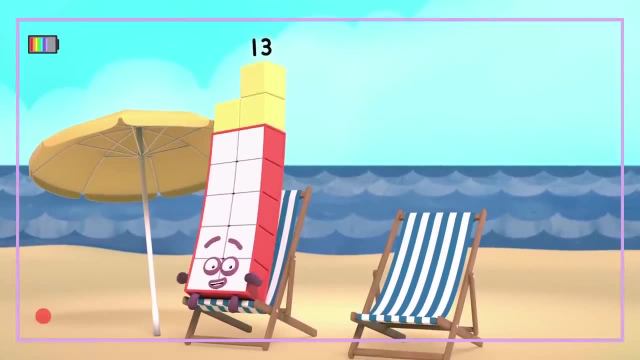 UP, UP, UP 13B. I mean considered Three, two, Three, two one UGH UGH, UGH UGH U Reach Nice, well done. There's three halfs on my clock. 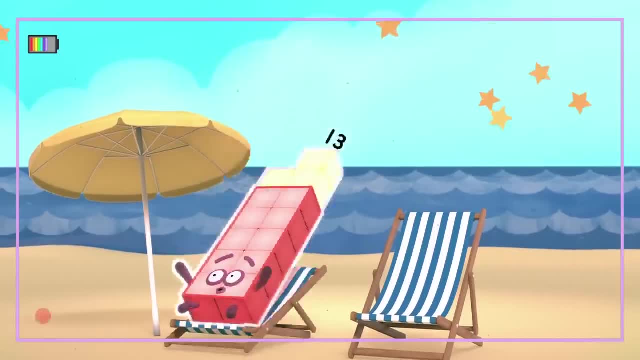 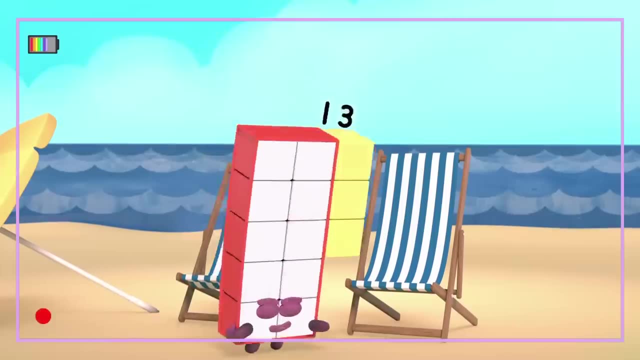 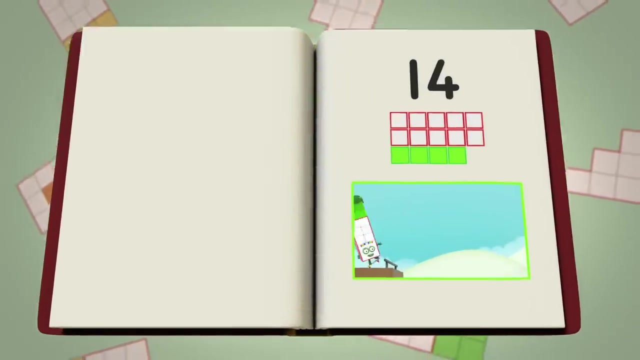 Finally, World этойائ's gonna beat that card. I wanna get some luck. You, I'm lucky. Chapter 14, downhill all the way, dude. Hang ten Plus four, I'm extreme 14.. Check this out. 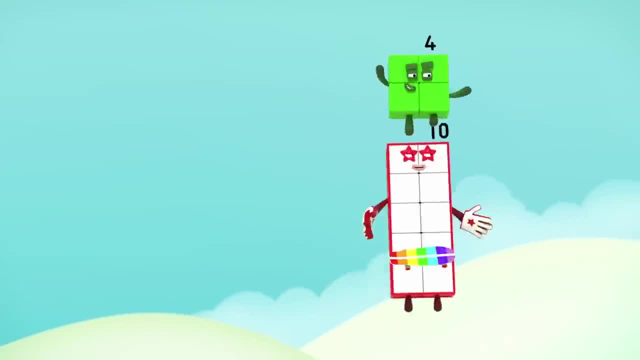 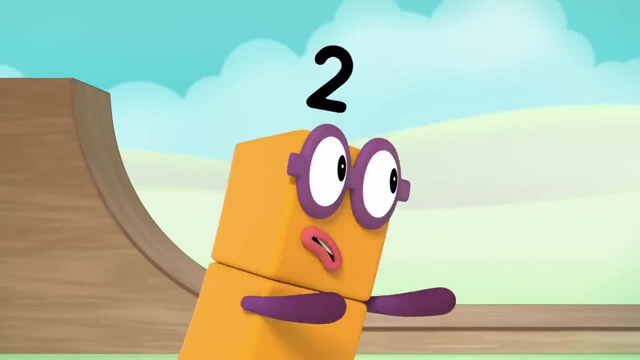 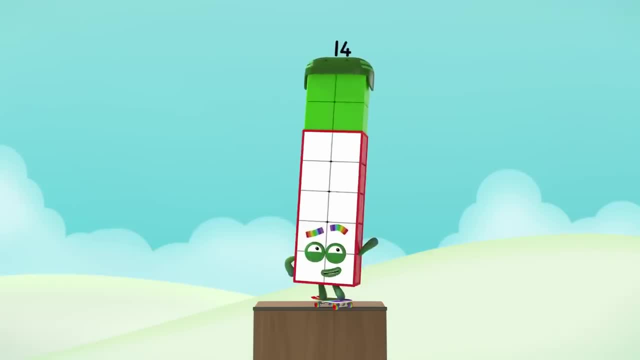 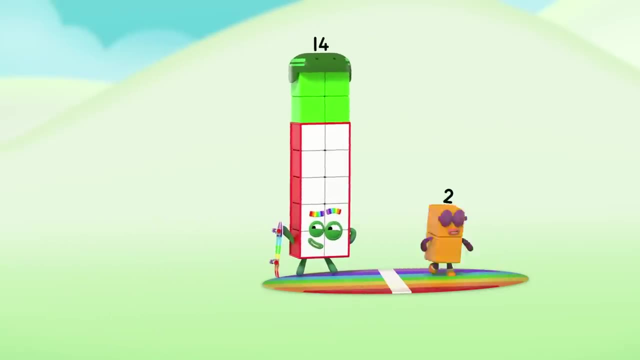 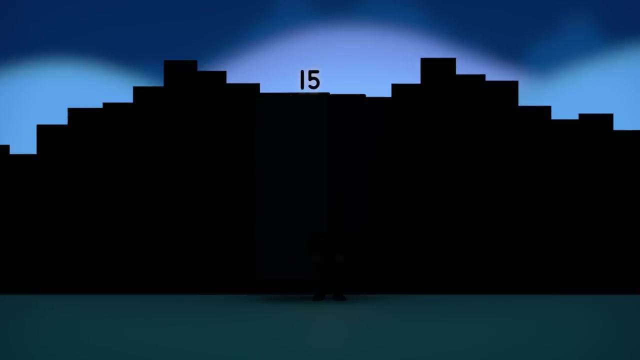 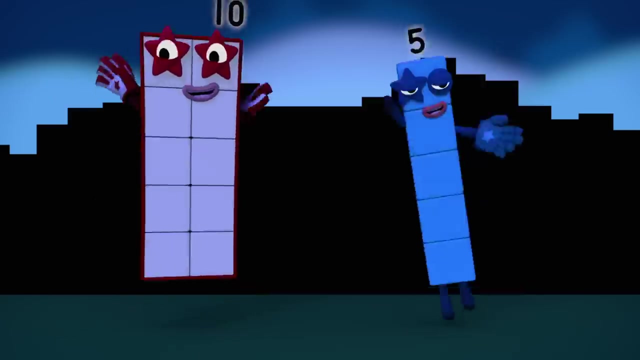 Worry, not bro, I'm 14.. I'm not just lucky, I'm double seven, Double lucky, Woo-hoo, Hey tense. Chapter 15.. Night mission: Hush hush Agent 15 here. 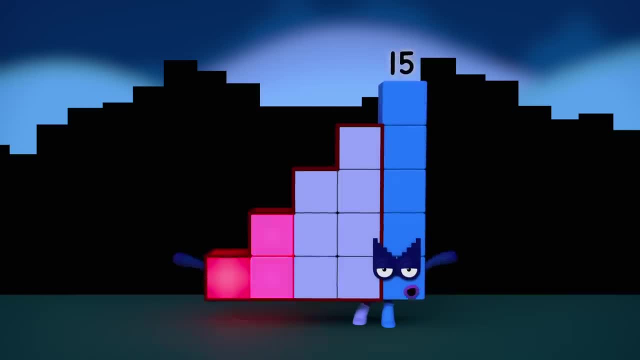 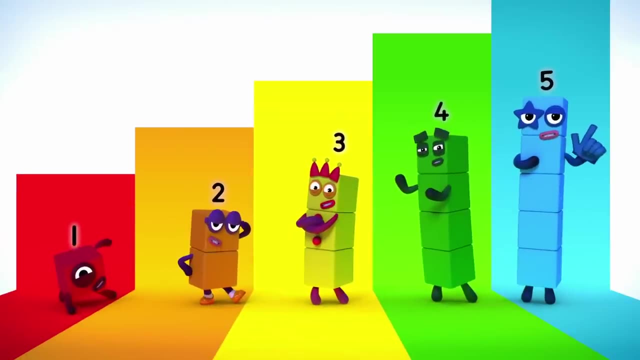 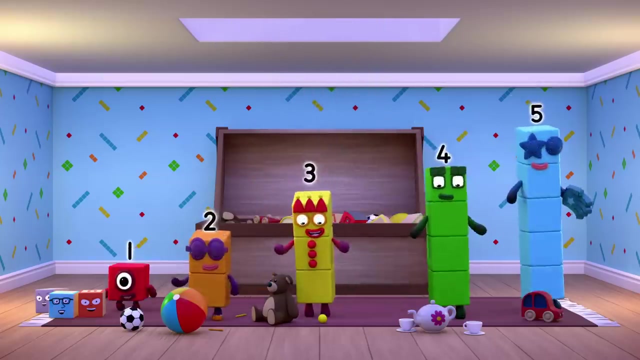 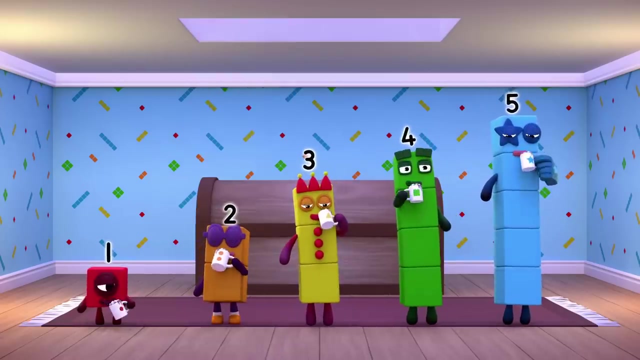 But on the quiet, I'm also one plus two plus three plus four plus five. That's right, I'm Super Special Secret Step Squad On a top secret night-time mission. Step one: tidy. Step two: drink cocoa. Step three: brush our teeth. 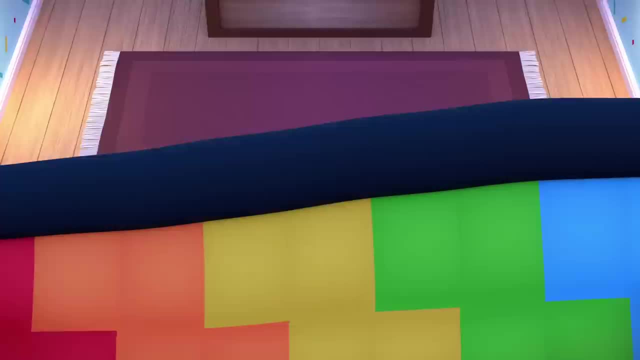 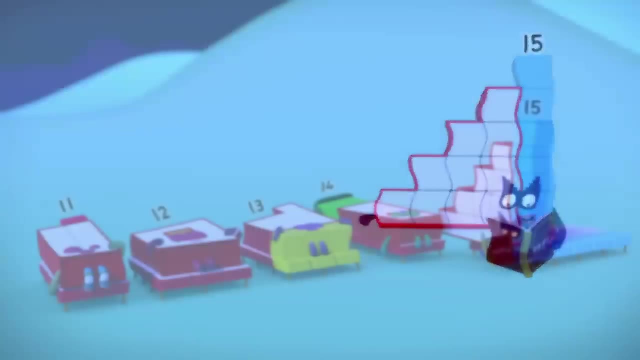 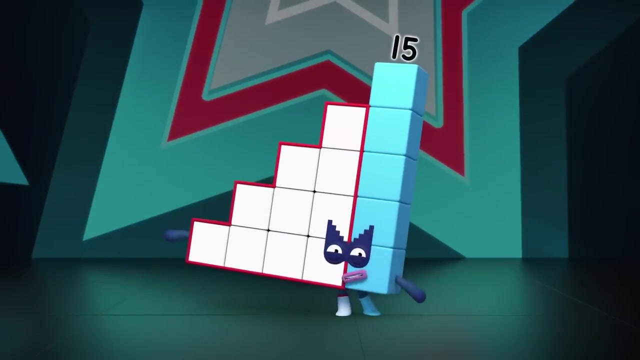 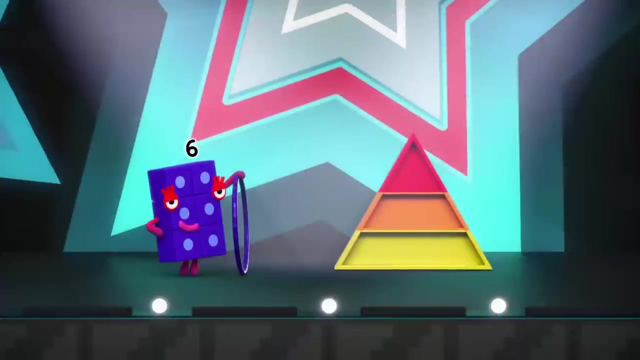 Step four: get on to the bed. Step five: read a nice bedtime story. Welcome back to Fifteen's Minute of Fame, The show where number blocks show you their tremendous talents. So far tonight we've seen Six and her bobbing number blocks. 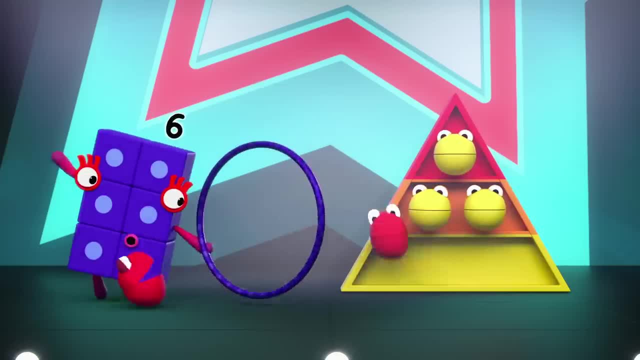 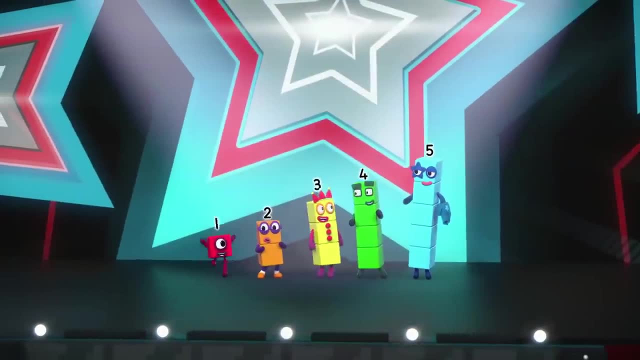 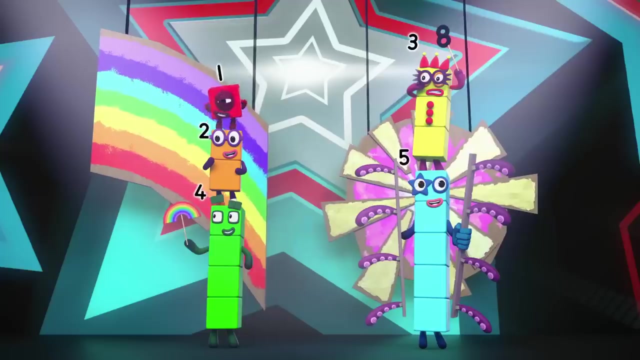 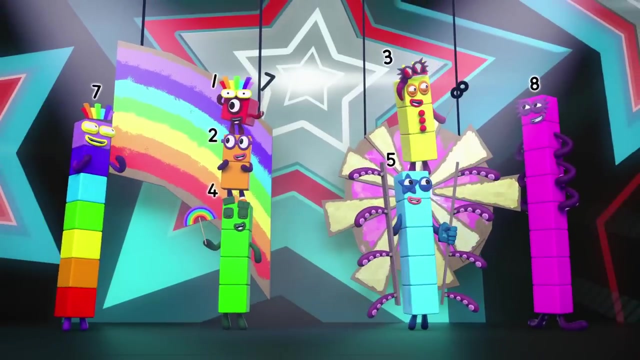 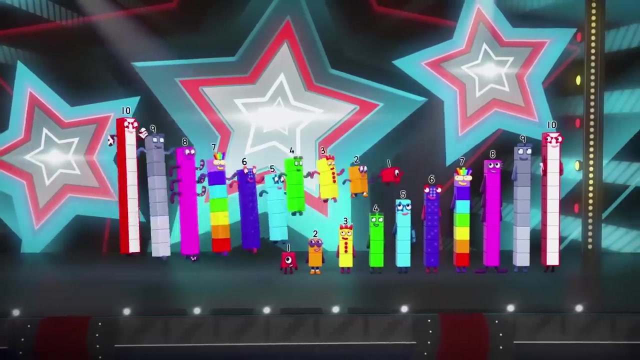 One, two, three, triangle, Four, five, six triangle. Impressive impressions. Octoblock to the rescue. Oh, that's lovely And mystical magic acts. Ho ho, ho, ho, ho, ho ho. 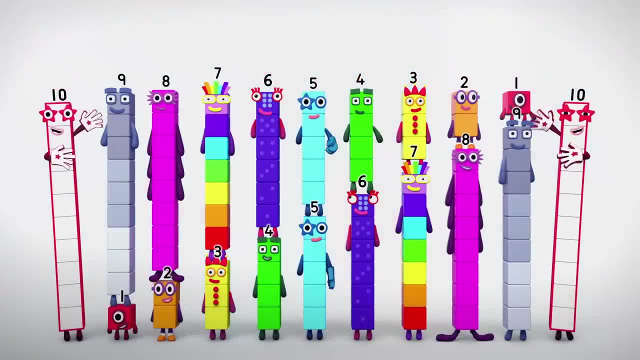 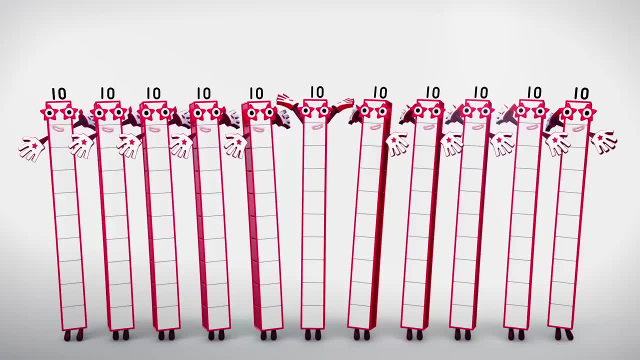 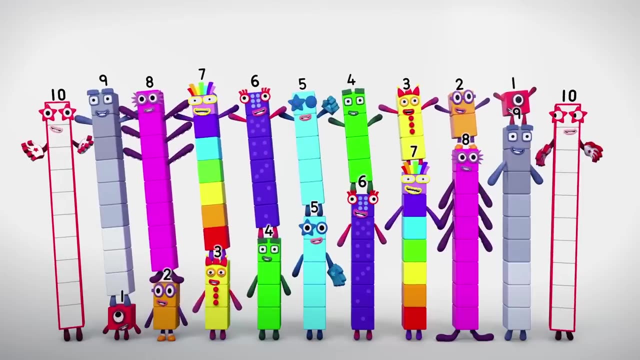 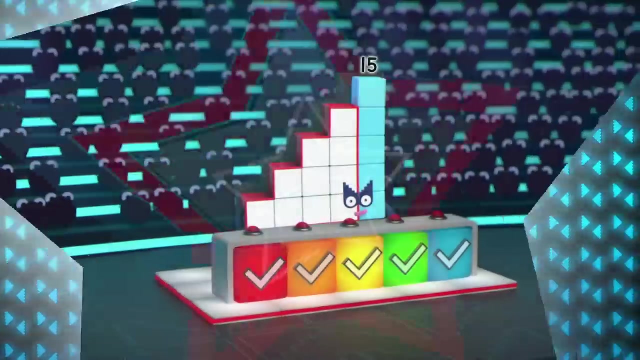 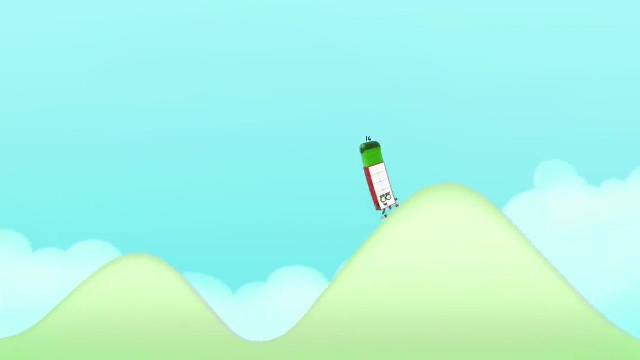 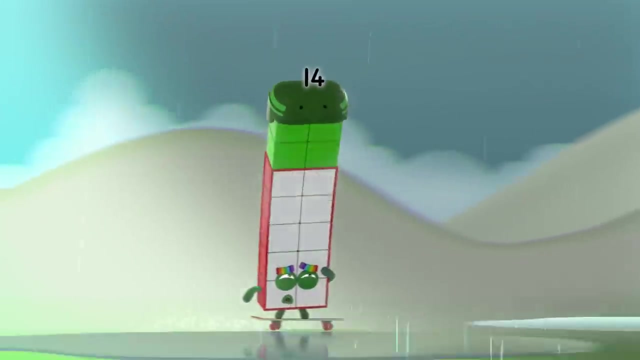 Ha ha. Numbra Cadabra Eleven. tenths Numbra Cadabra Seven-eleven. Now it's time to see what some of our bigger numbers have in store. For as long as I can remember, I've always wanted to skate in wind, rain and snow. 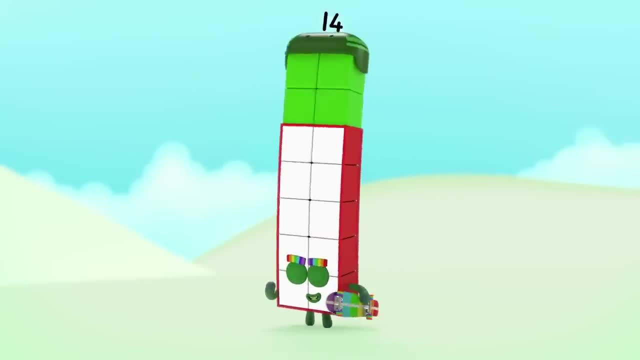 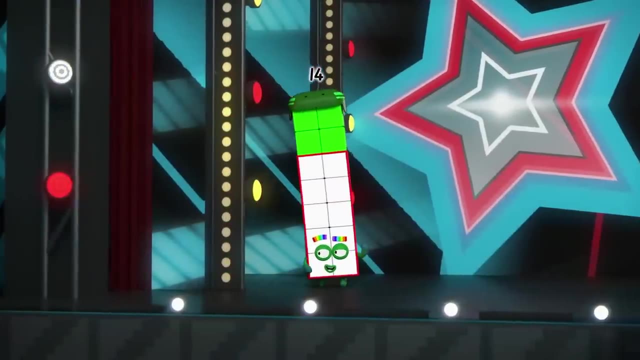 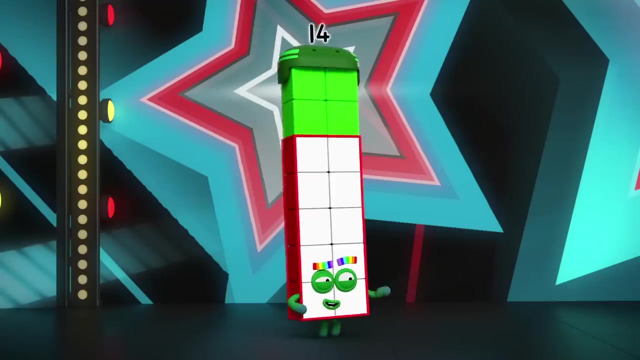 No matter how gnarly it gets, I put in the hours, Cos practice makes perfect. Welcome to Fifteen's Minute of Fame. Show us what you've got. Fourteen, No problemo, But I need a volunteer for this trick. 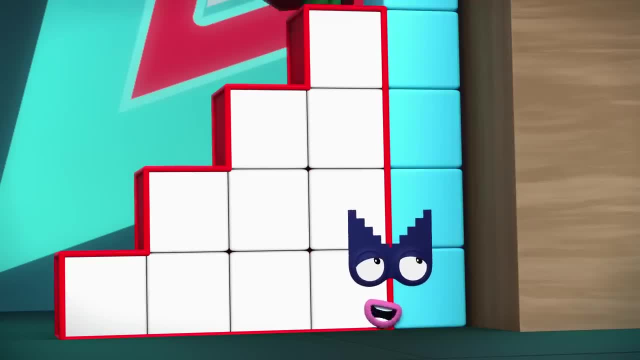 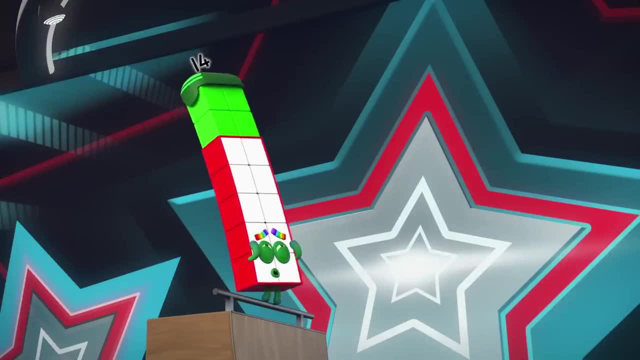 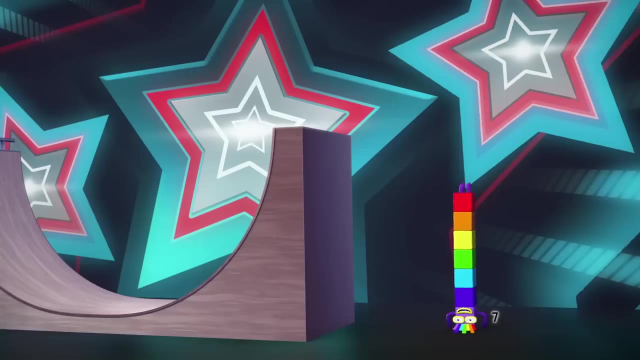 Fifteen: No, no, I'm not the act He is, I'm just helping him take it to the next level. Fourteen: Oh no, I forgot my skateboard, Whoa-ho. Ah Well, Yep, that was lucky, Double lucky. 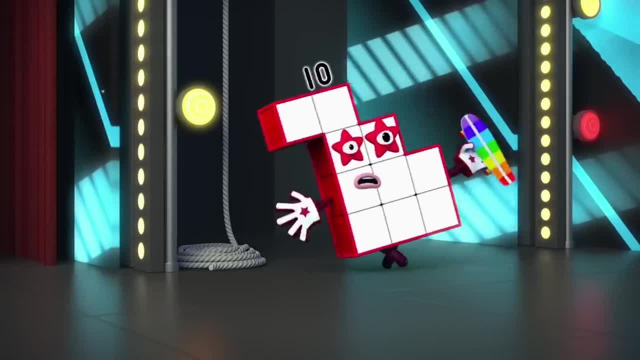 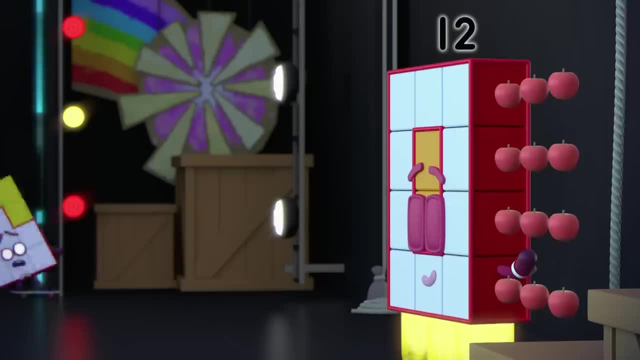 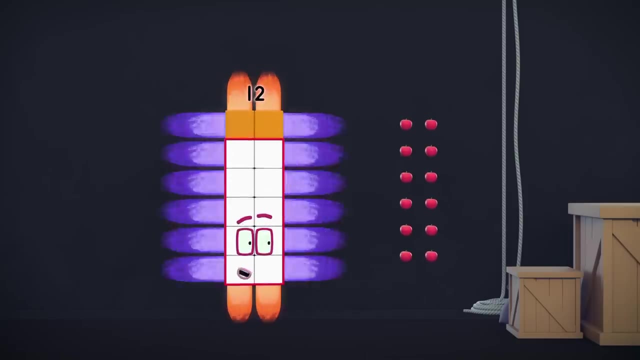 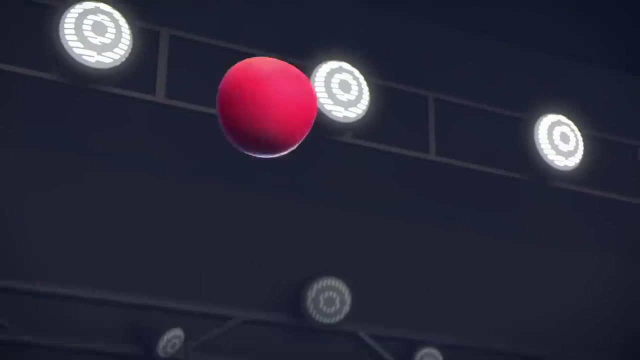 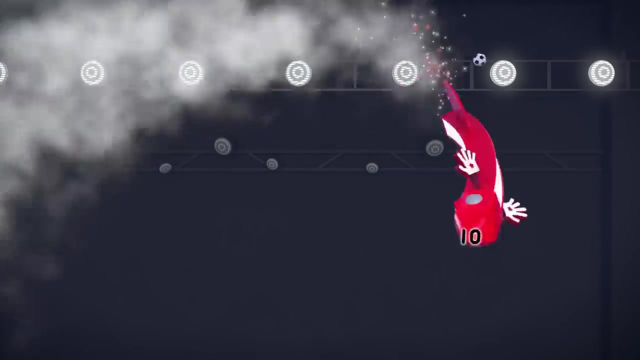 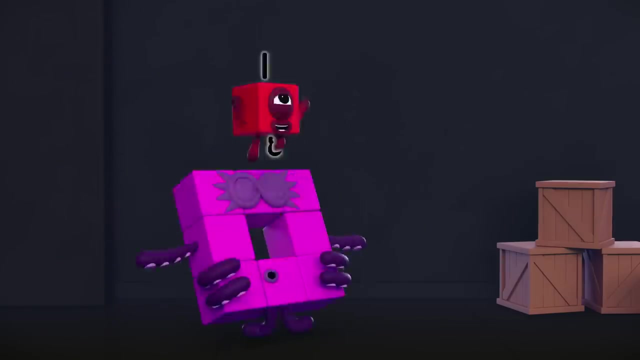 I found it Thirteen, Twelve, No, No, No. Three by four, Switch, Two by six. Mind your backs. No, Whoa. Eleven, Oh dear Ten, I've got it Nine, Achoo. 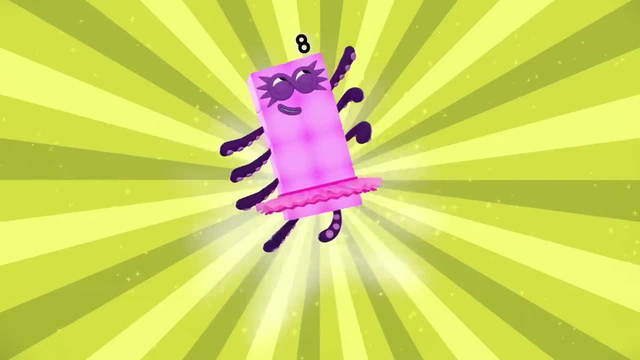 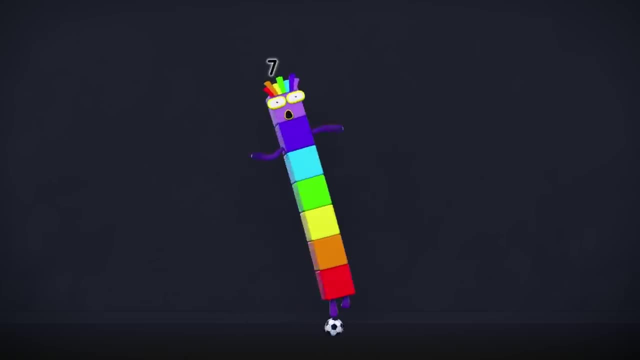 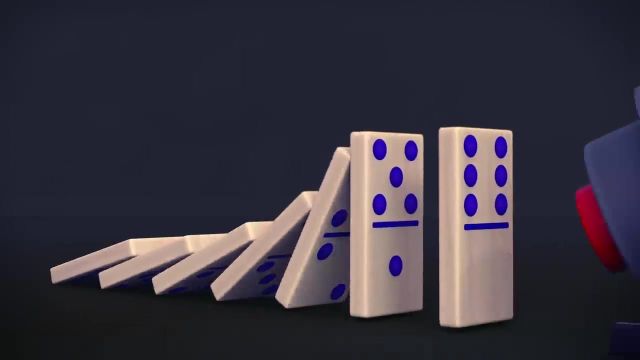 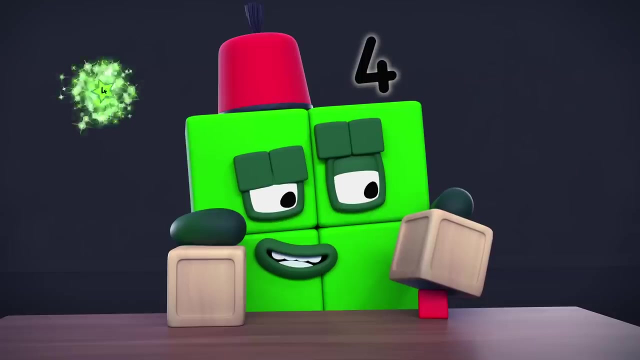 Eight Octoblock: pirouette One, two, three, four, five, six, seven, eight. Pirouette Seven, Lucky me- Six, Five, Four, Screw, screw, Screw, screw Round thing. 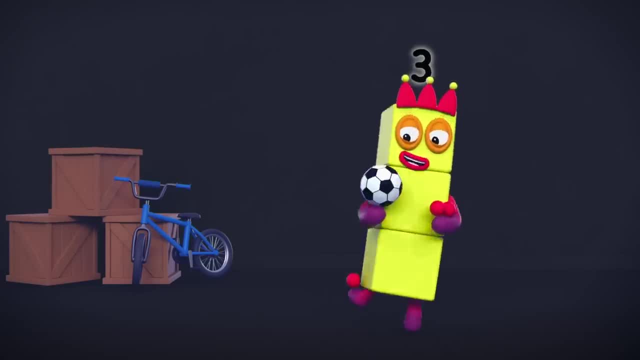 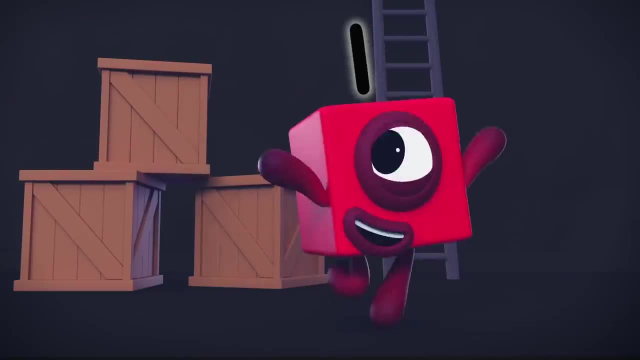 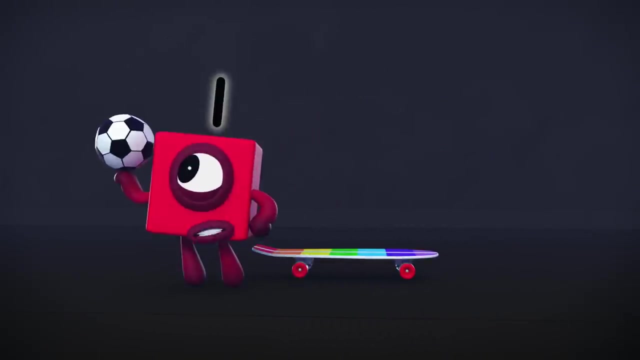 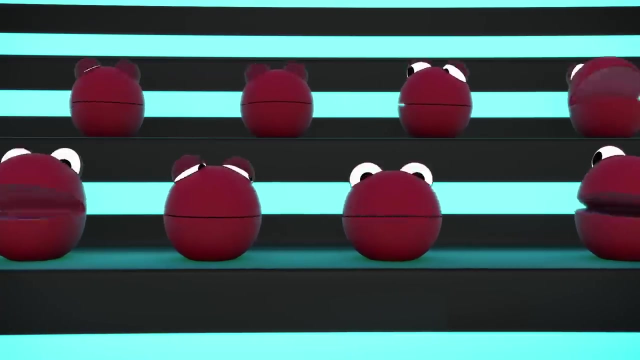 Three. Look at me. Two, One oops, Two, oops, One, Ta-da, Woo-hoo. Anyone lost a football Or a skateboard? Zero, Nothing to it. Ha-ha, Yay, Hooray. 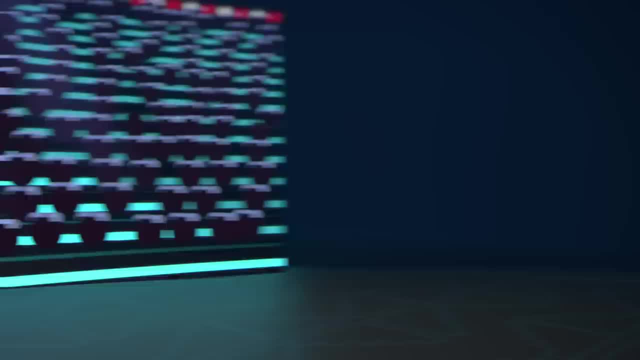 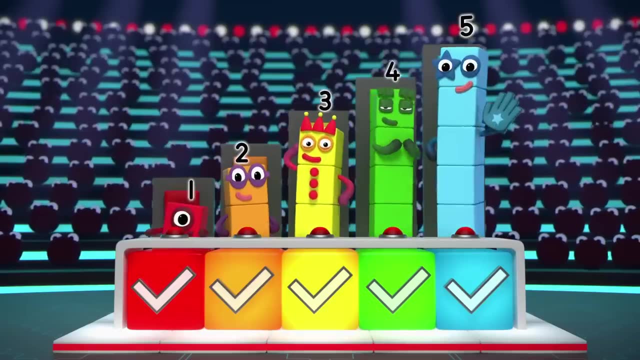 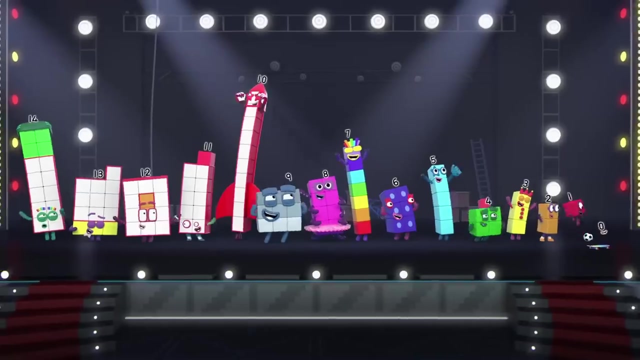 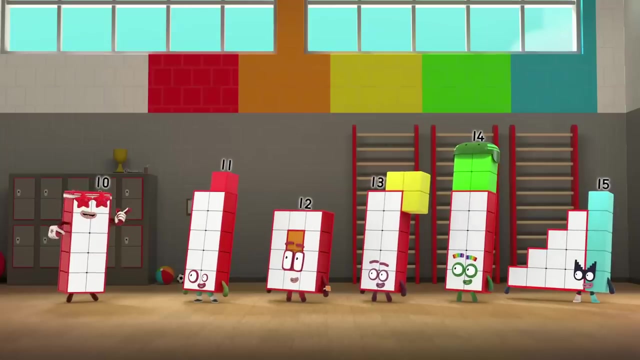 Let's see what our judges made of that Hush-hush. Everyone's a winner. Hooray, Welcome to Ten's Place. All of you are bigger than me. That means each of you has a ten inside you, You see. 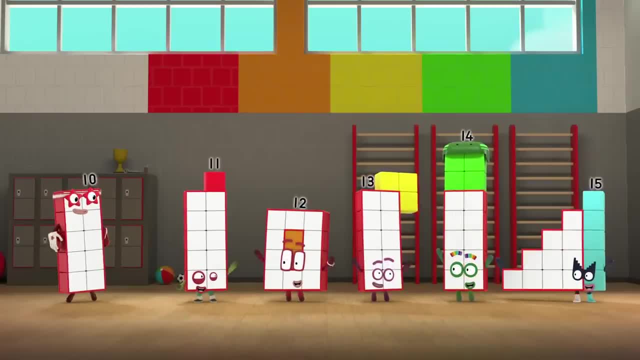 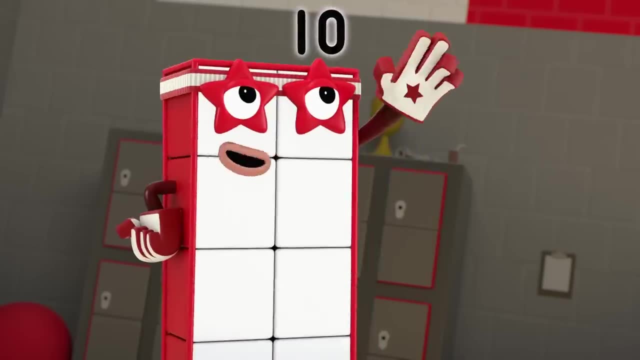 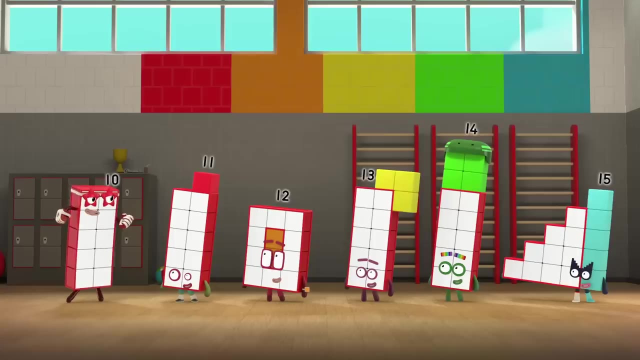 You are greater than ten And you've got big dreams. You want fun? Well, fun it is. And right now is where you start playing Hooray. Okay, let's pump those numbers. Hooray, Hooray. 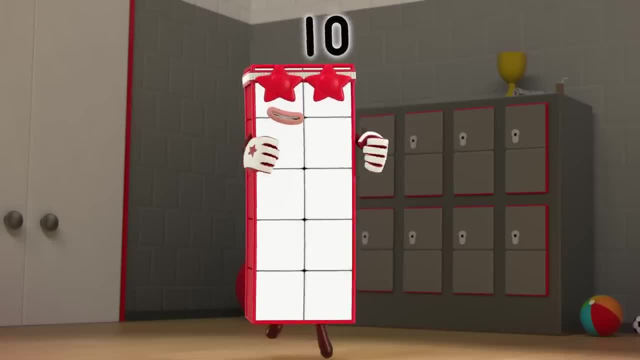 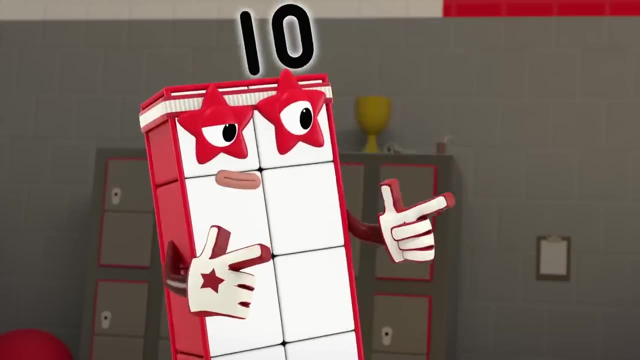 Hooray, That's right Now, give me some squats. Let me see you do the jump and bump. Let me see you do the jump and bump. Let me see you do the jump and bump. Ten Plus one is eleven. 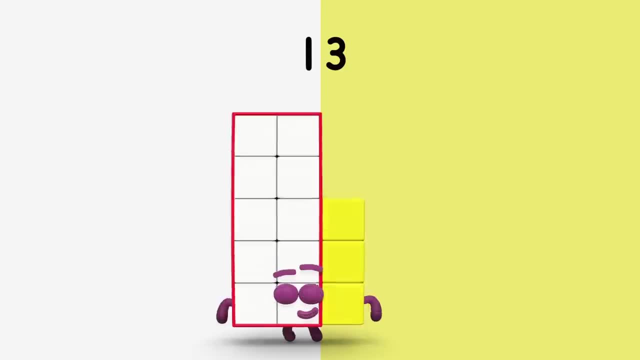 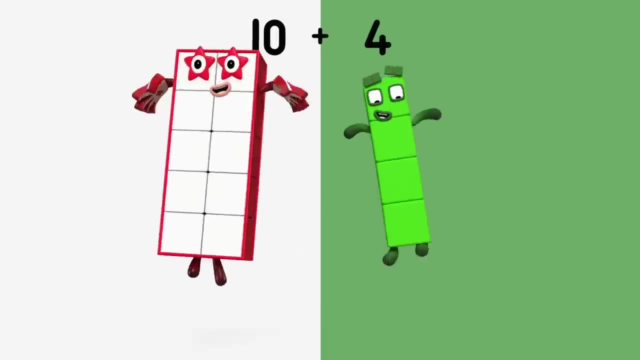 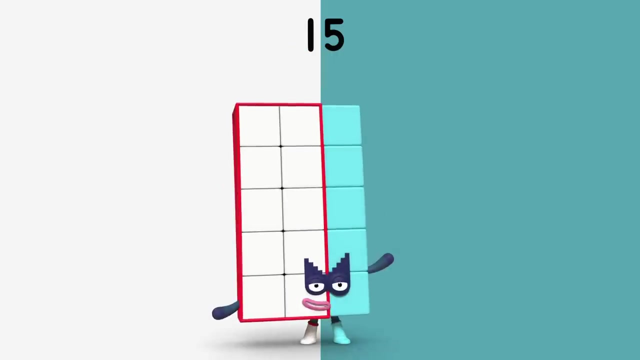 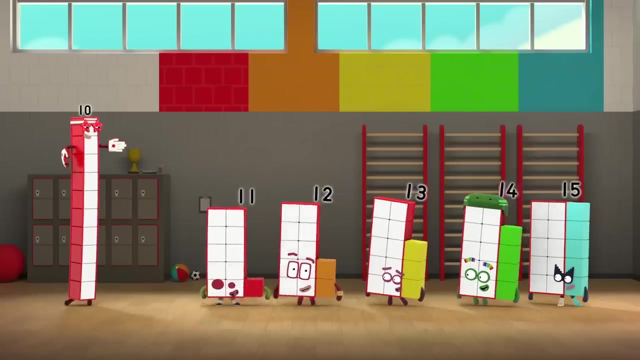 Ten Plus two is twelve. Ten Plus three is thirteen. Hooray, Ten Plus four is forty. Ten Plus five is fifteen. Terrific, Now, let's stretch our tens: Nice and tall, Nice and tall. 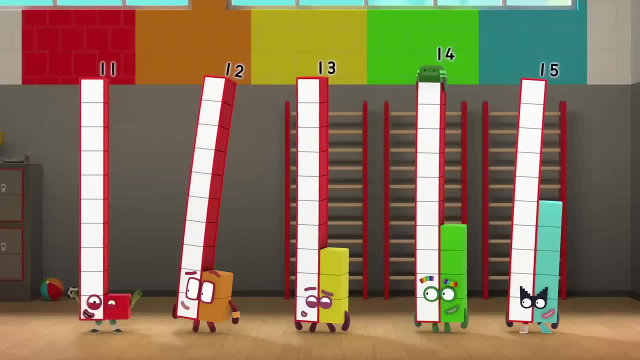 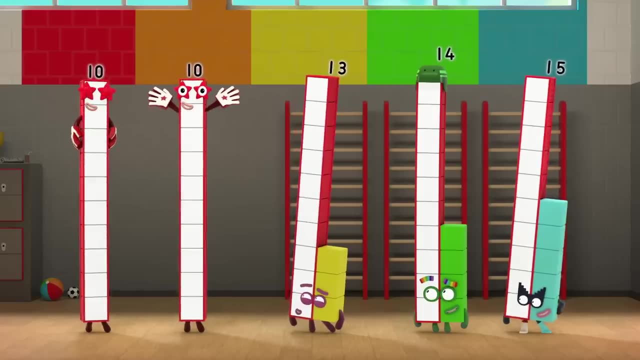 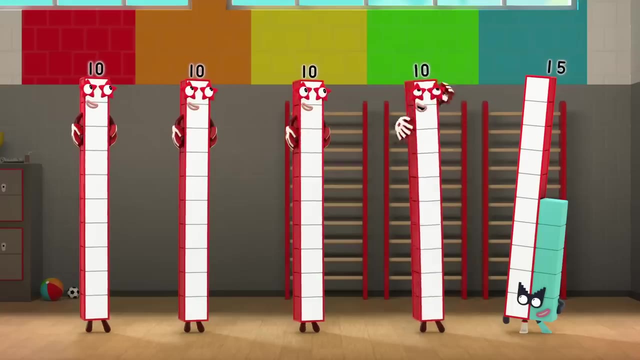 Fling those ones high in the air, Take it away. Minus one is ten Twelve. Minus two is ten Thirteen. Minus three is ten Fourteen. Minus four is ten Fifteen. Minus five is ten. 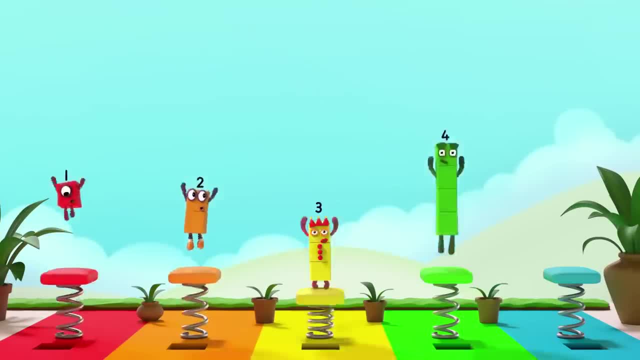 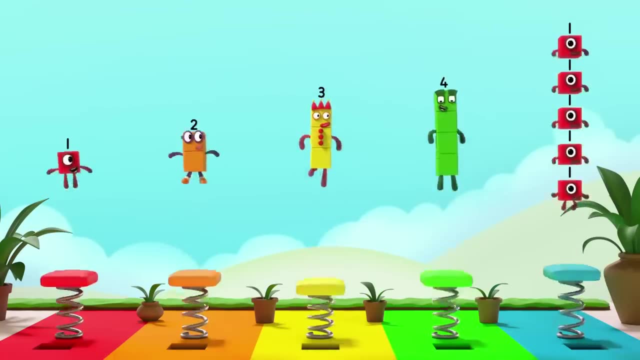 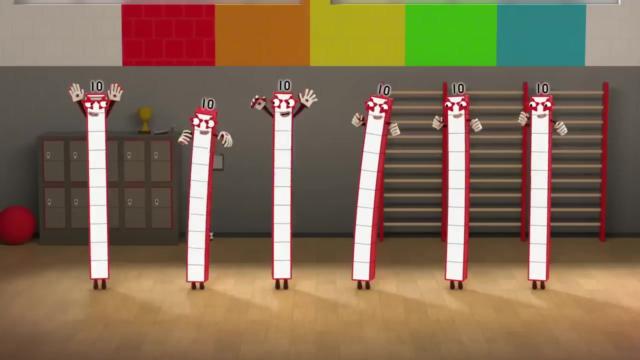 Boing woe, Boing, woe, Boing woe. One, Two ones, Three ones, Four ones, Five ones. Ready, Let's work those tens. Yeah, Tall, Slide, Two eyes, Slide and go low. 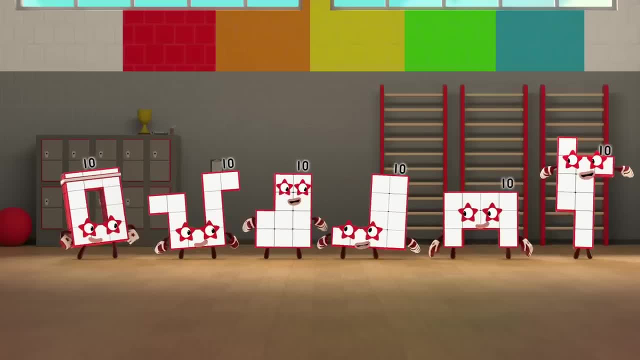 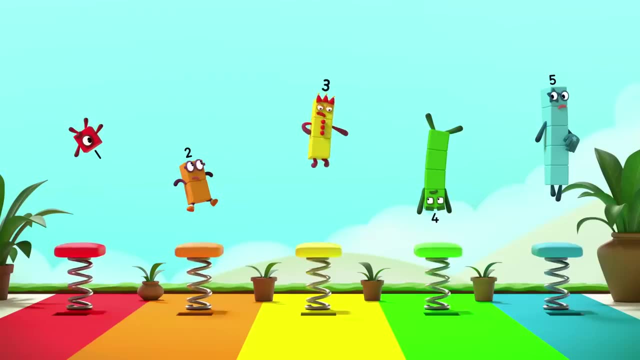 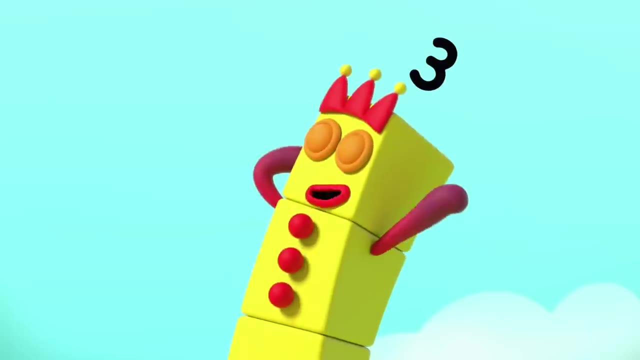 Rectangle with a hole And freestyle: Yeah, Boing, woe, Boing, woe, Boing, woe, Stop, Stop, Stop. If this is tens place, where are the tens? Um, I say we make this floor. 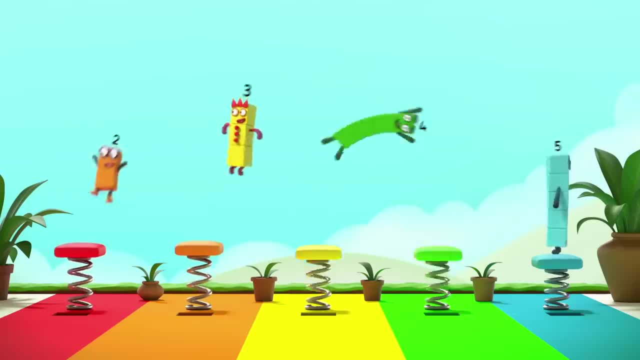 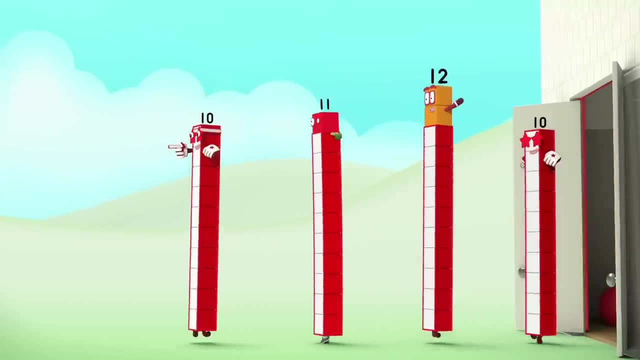 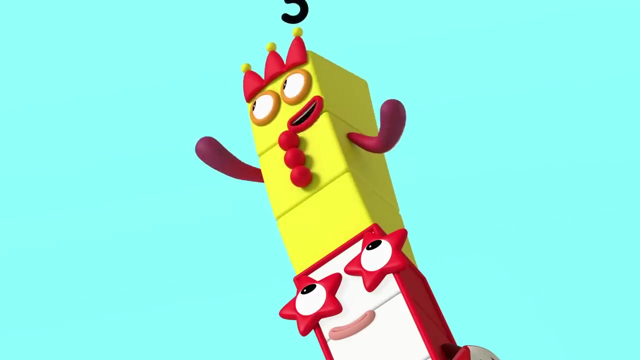 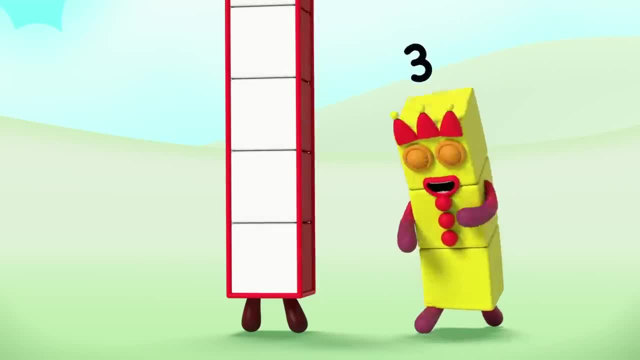 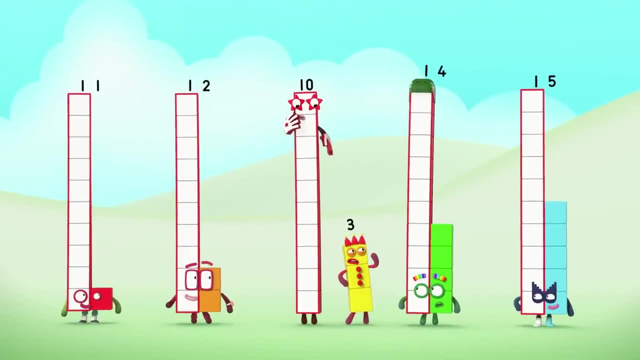 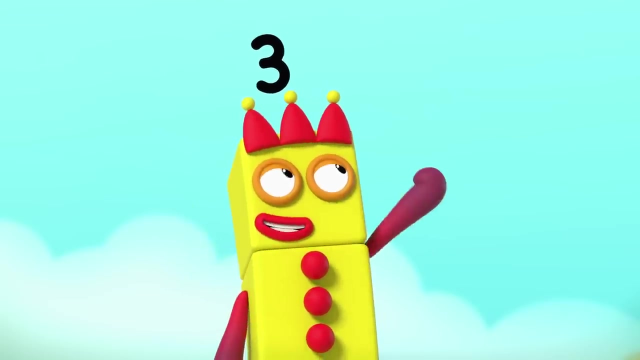 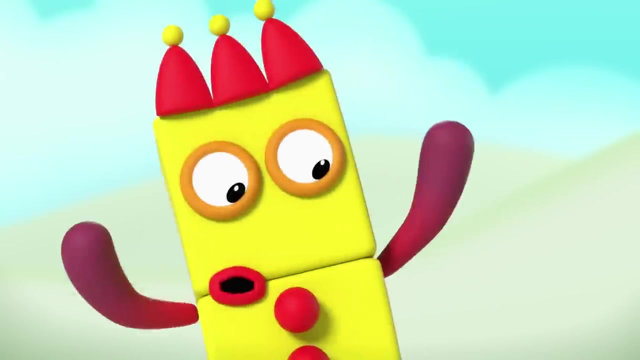 Put me down. All of you are bigger than me, So make yourself shorter, Even shorter. You've all got a three inside you, Well, except for thirteen. He already pinged the part into ten and me, Oh, Fourteen. 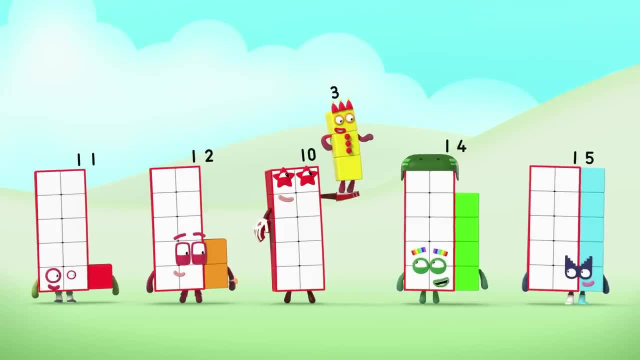 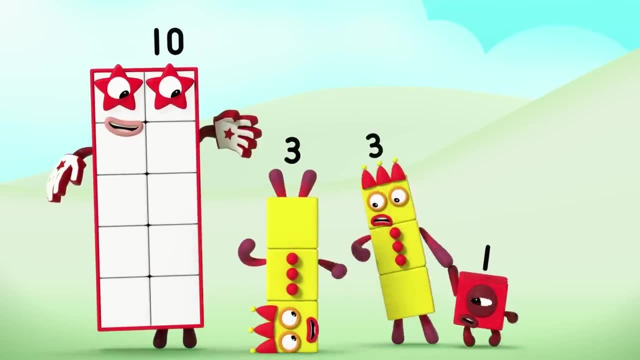 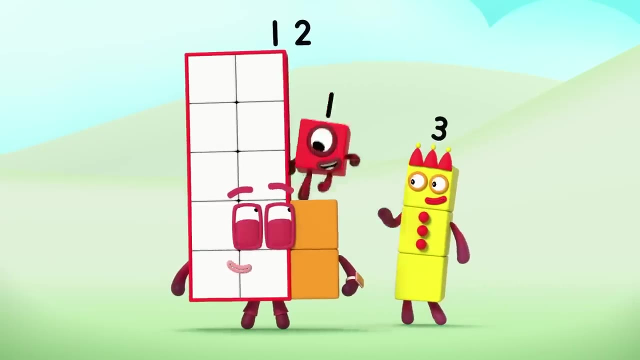 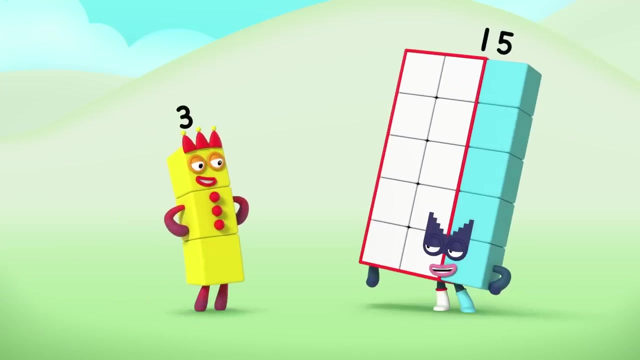 You're one more than thirteen. Extreme fourteen Minus one, I close thirteen. And for my next trick, twelve Plus one equals ten and three. Oh no, Your turn Fifteen. Let's say ten and five, But I want ten and three. 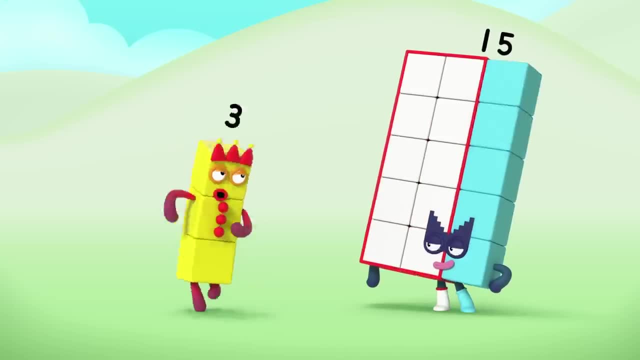 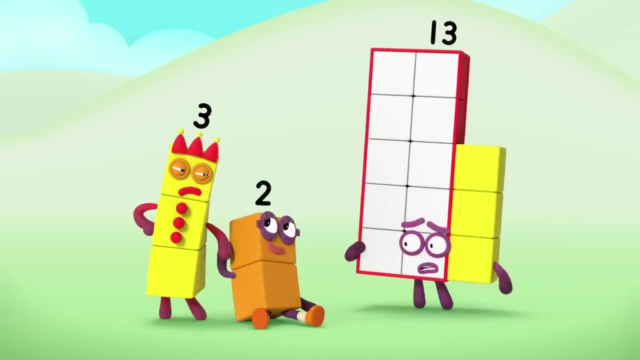 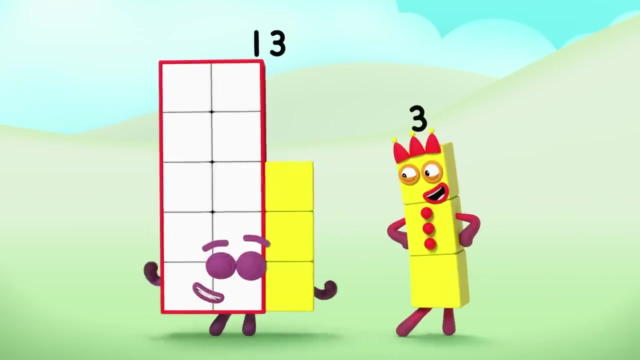 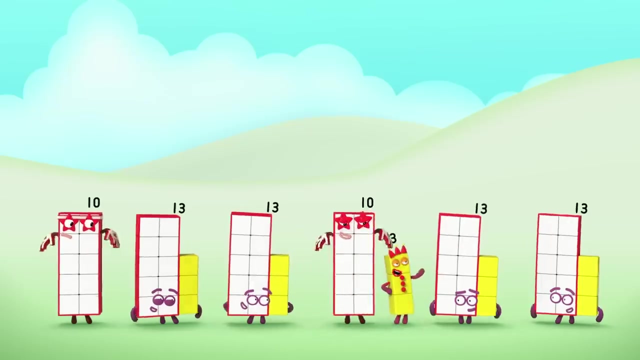 And three is two less than five. So let's pop off a two, Ten and five minus two equals ten and three. Ten and one plus two equals three. Only joking Ten and three There. Now everybody stand tall When I say go. 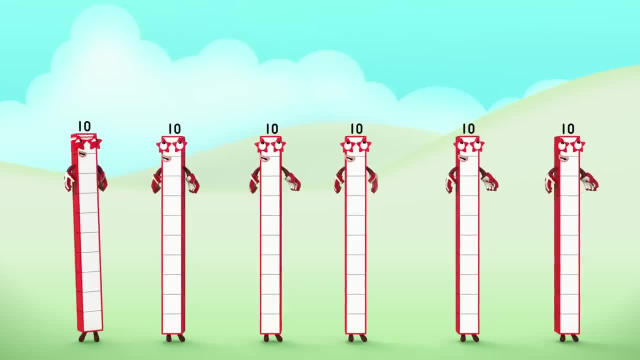 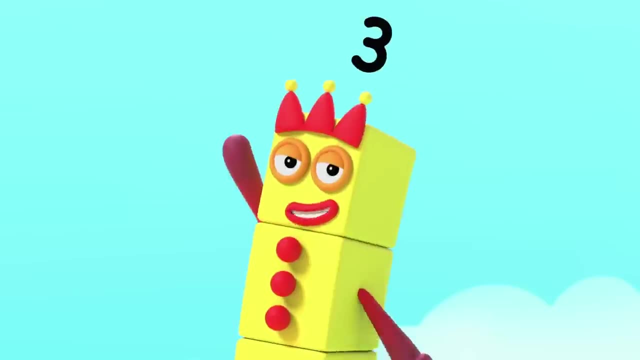 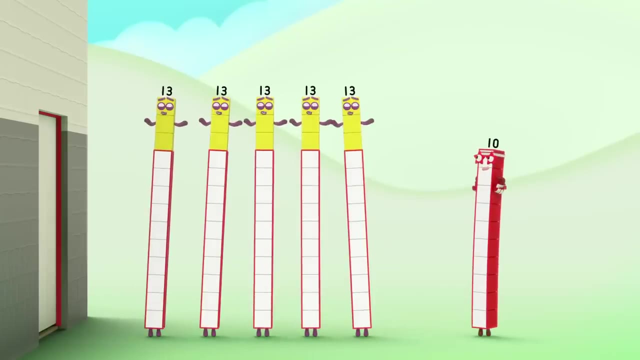 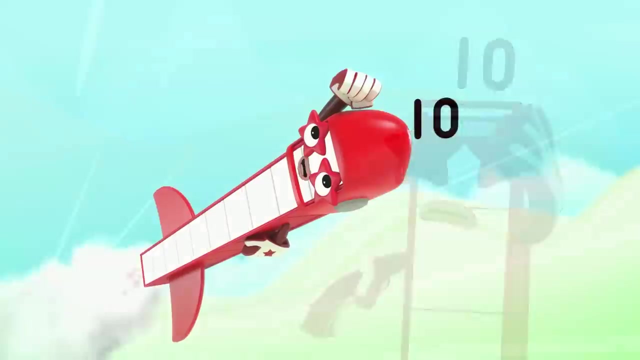 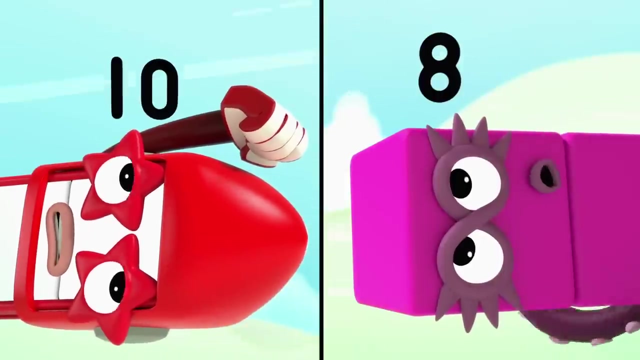 go, go, my lovely thirteen. Welcome to three's place. Never mind ten's place or three's place, We should call this thirteen. Play fast as a rocket. Octo Speedy Too fast, Uh-oh, Ten plus eight equals. 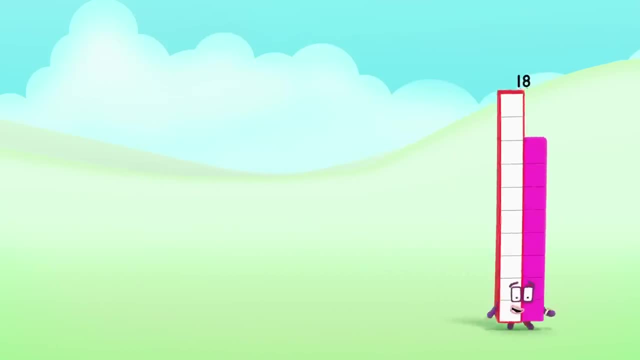 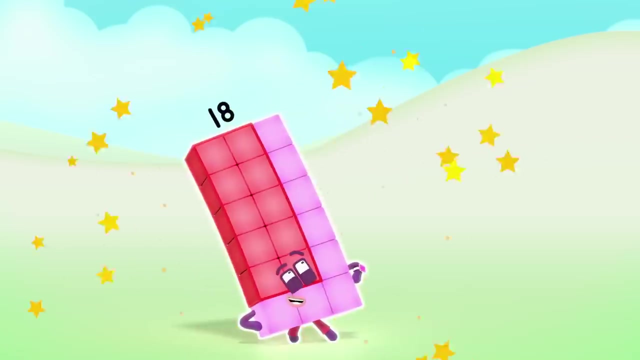 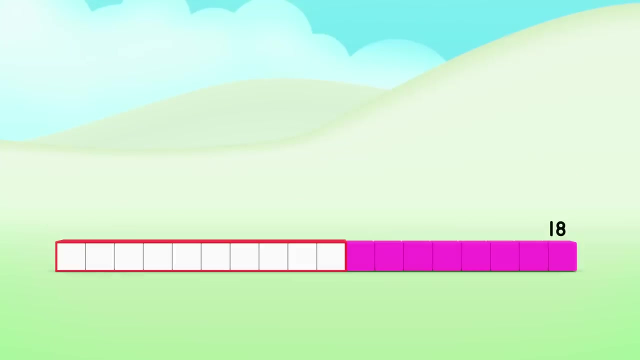 eighteen, Brr, Refreshing, Hey time to discover who I am. Done, I am eighteen and I'm a super speedy, super rectangle and I like to go fast. Oh, so tall Falling over competition. Oh, I win. 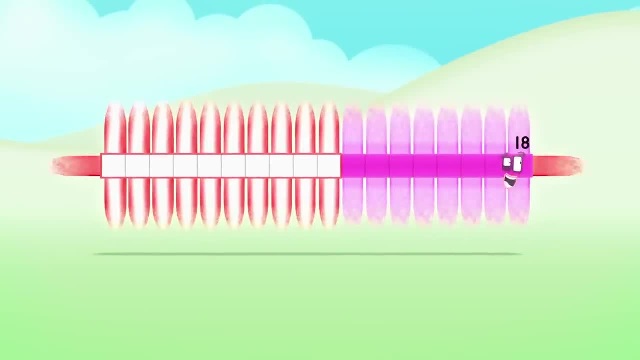 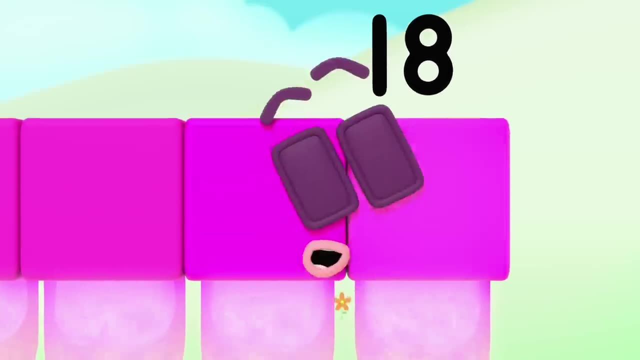 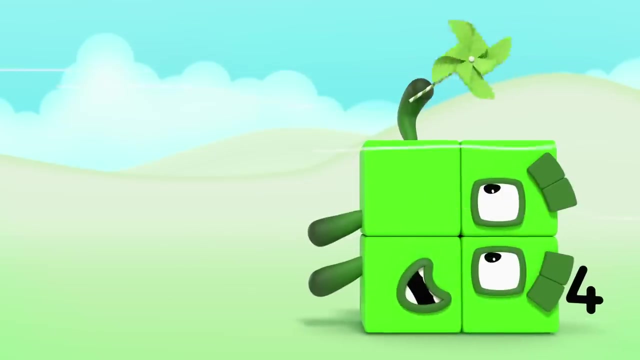 Aha, Eighteen by one. One ray is all. I need One ray to build up speed. I start to go and I go, go, go. Whoa, Haha, Oh, Eighteen ones. This is fun Too fast. One, two. 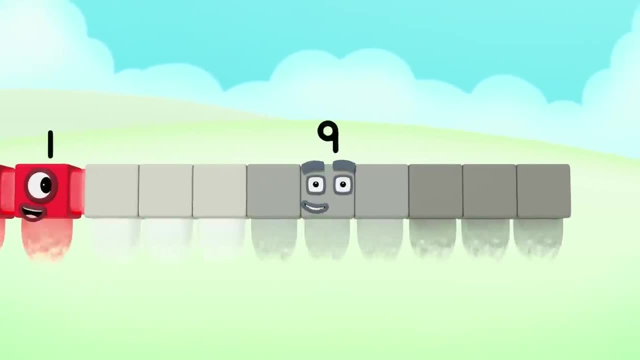 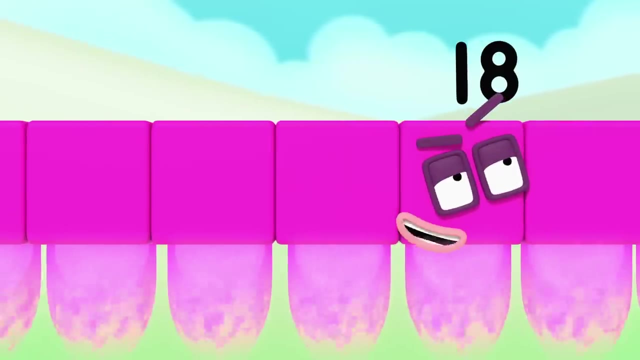 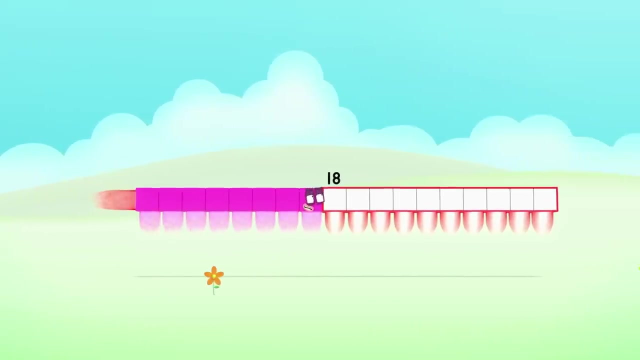 three, four, five, six, seven, eight, nine, ten, eleven, twelve, fourteen, fifteen, sixteen, seventeen, eighteen. When it comes to acceleration, I'm the undisputed master. I'm the quickest in the nation. 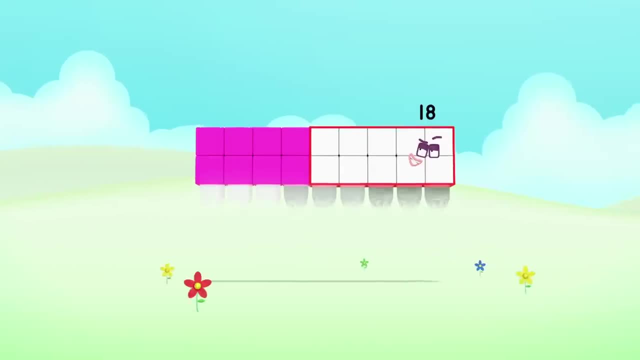 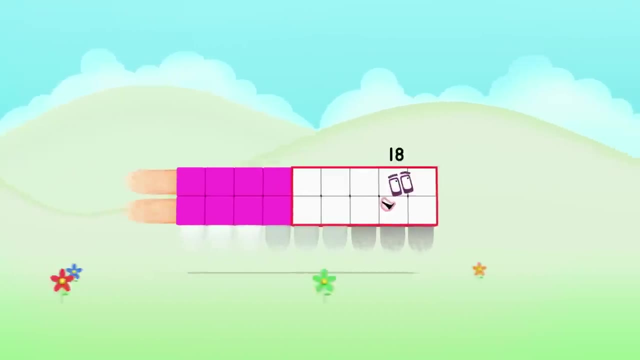 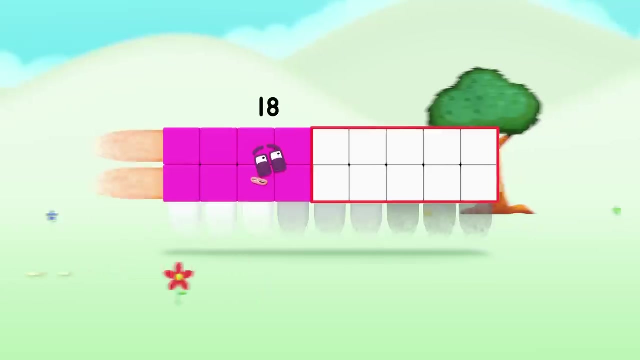 I change shape when I want to go faster. Switch nine by two to raise it away. I'm eighteen, I'm a speed machine. I can set the world ablaze. Watch me zoom with a sonic boom. I was born to ride the razor. 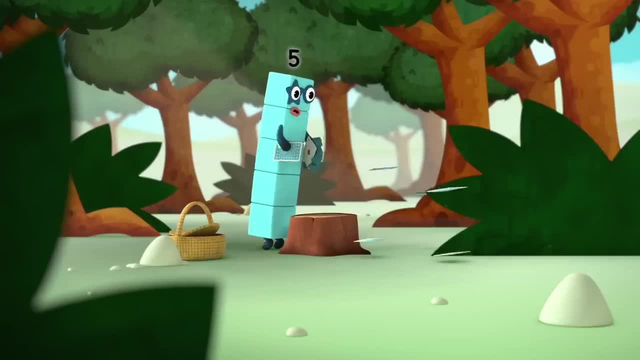 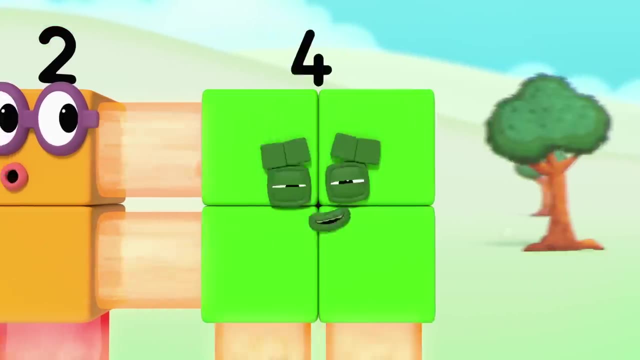 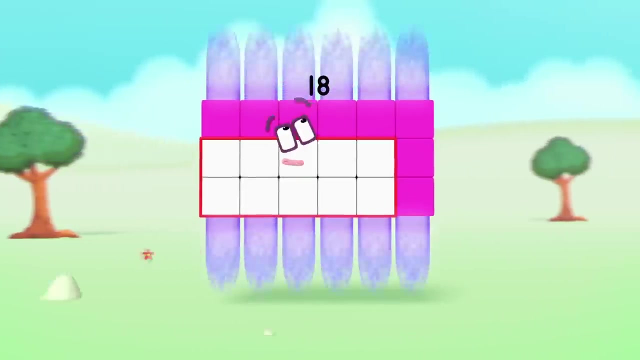 Yeah, Oh, Nine, twos, Woohoo, Oh. Two, four, six, eight, ten, twelve, fourteen, fifteen, eighteen. Switch six by three. Three rays are what I need, Three rays, and I build up speed. 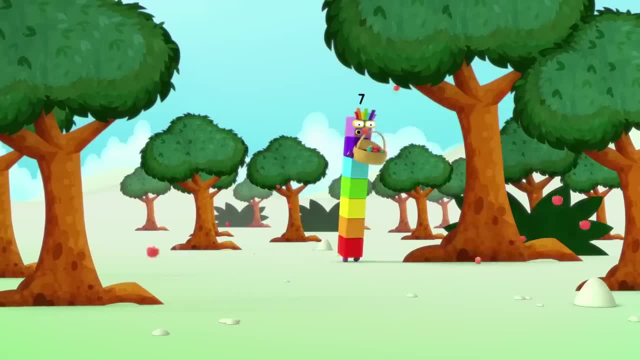 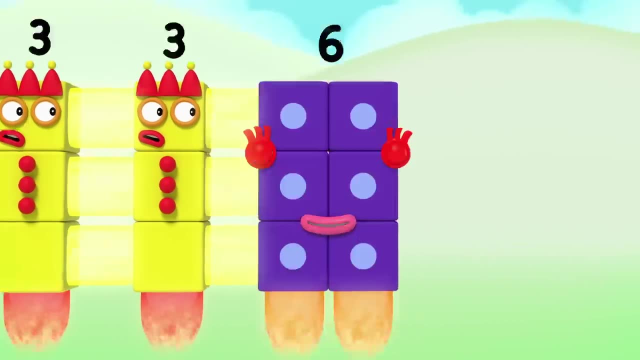 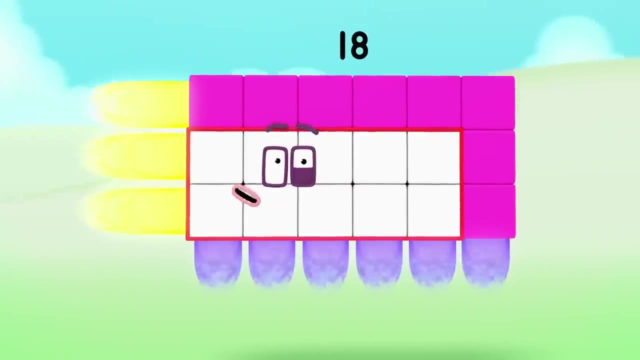 I start to glow and I go, go, go, Whoa, Wow, Six, threes, Yippee. Two, three, six, nine, twelve, fifteen, eighteen, Cool time. When it comes to acceleration, I'm the undisputed master. 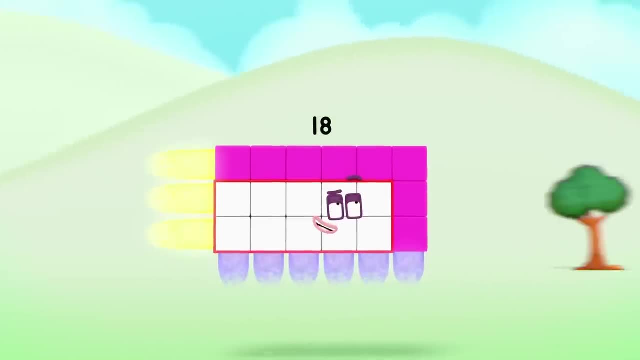 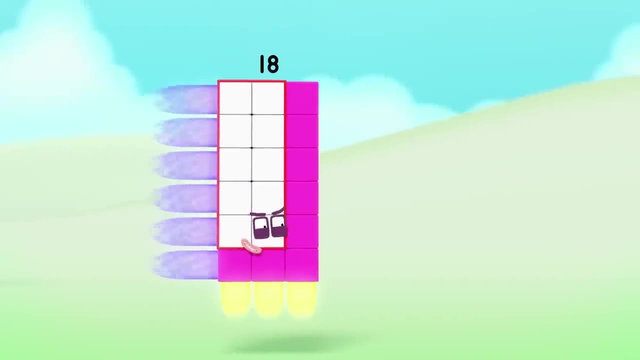 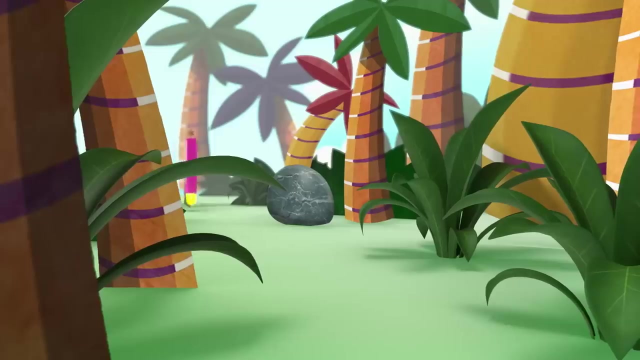 I'm the quickest in the nation. I change shape when I want to go faster. Turn three by six, Six rays and away. I'm eighteen, I'm a speed machine. I can set the world ablaze. Watch me zoom with a sonic boom. I was born to ride the rays. Hey Woo, Whoa, Yeah, Three sixes, Let's remix this. We're coming past, We're going too fast. Yikes, Six, Twelve, Eighteen, Me again Switch. 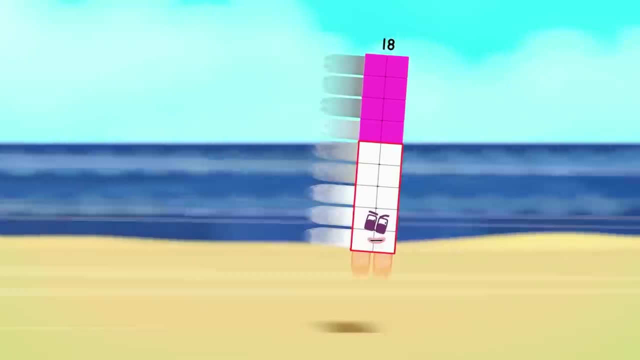 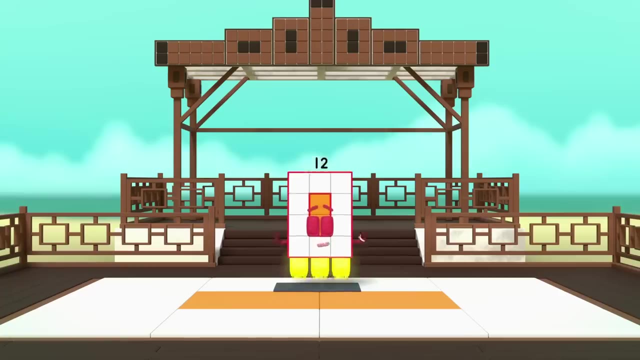 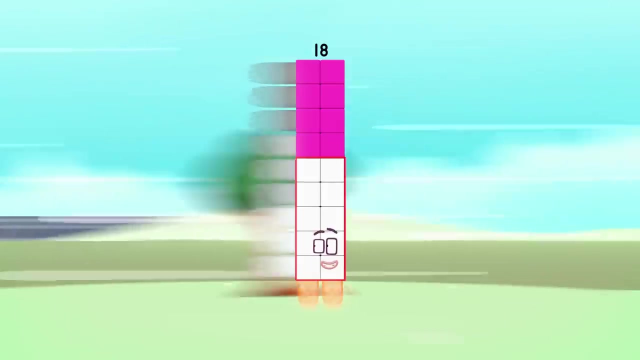 Two by nine. Nine rays are what I need, Nine rays and I build up speed, I start to glow and I go, go, go. Ah, Three, five, four, Whoa, Whoa Cool. Two, nines Parallel. 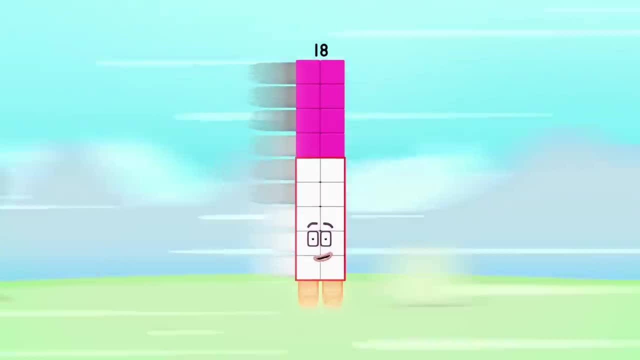 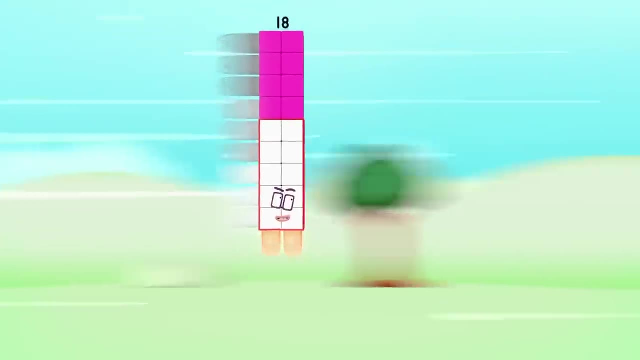 lines Nine Eighteen. Did you miss me? When it comes to acceleration, I'm the undisputed master. I'm the quickest in the nation. I change shape when I want to go faster, Ready for the big one: Switch. 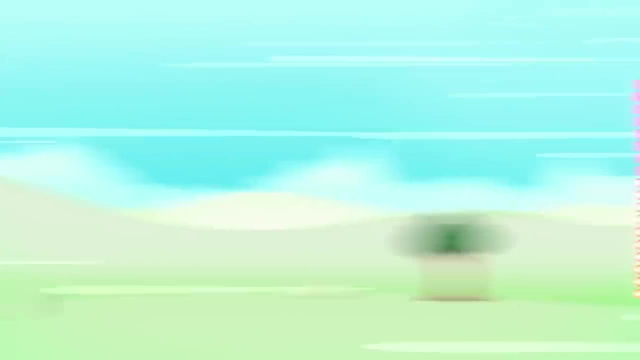 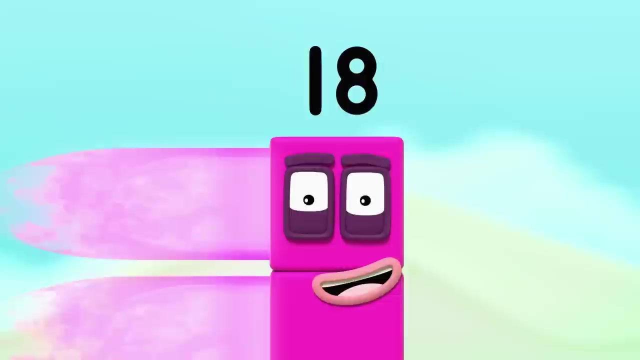 One by eighteen, Eighteen rays and away. I'm so fast I'll be out of the gate before you can lock it. I go at a rate no one can clock it. I'm ten and eight. I'm never late. I'm Octoclock on a rocket. 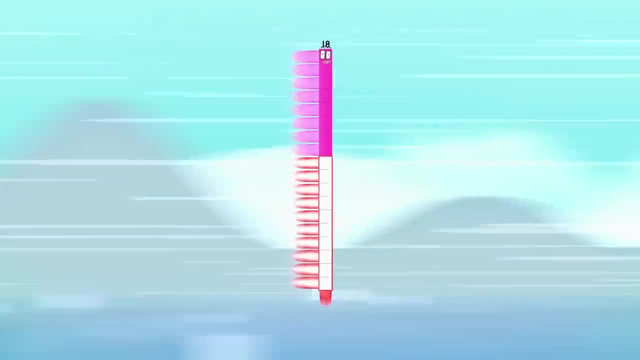 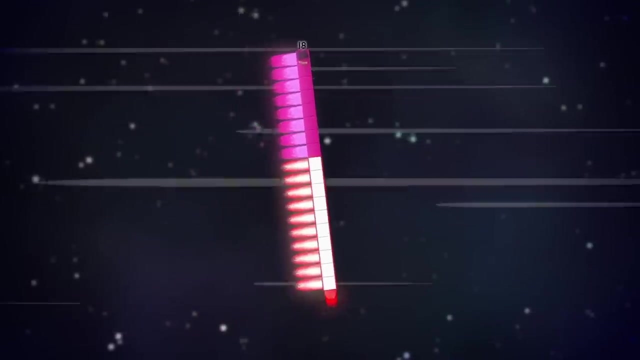 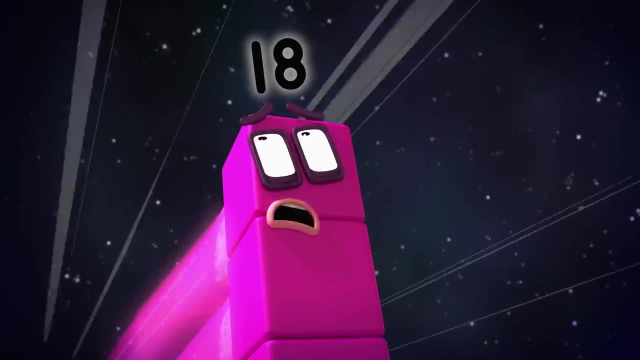 Yeehaw, I'm eighteen. I'm a speed machine. I can set the world ablaze. Watch me zoom with a sonic boom. I was born to ride the rays Round the world. How do I stop this thing? That's one way to do it. 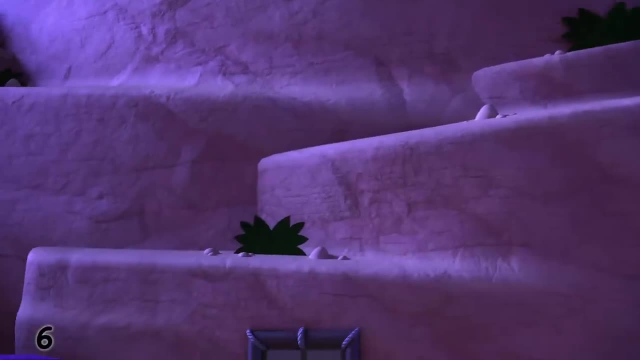 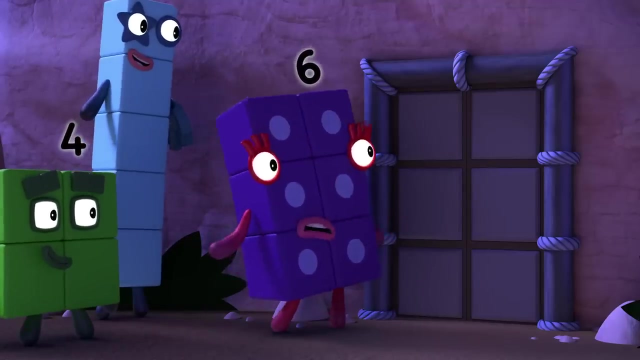 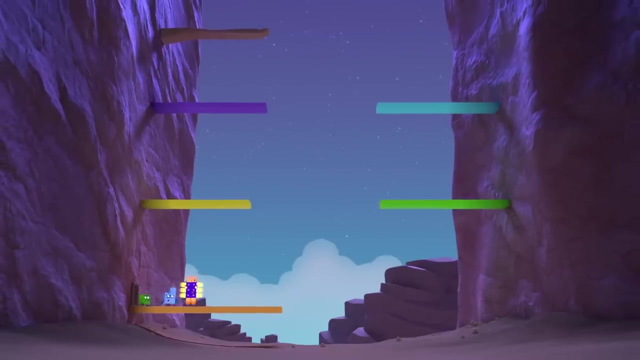 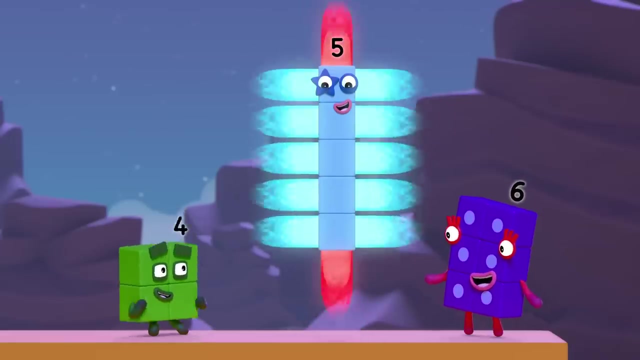 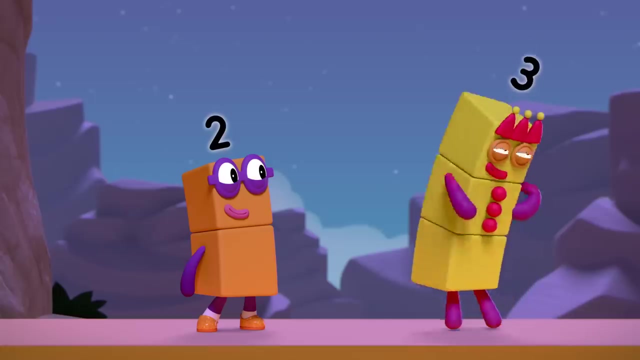 Refreshing. Here it is Right where Twelve told us The doors to Ray Canyon. I wonder why it's called. Oh, Ray Canyon, Rectangle rays. Twelve said: if one of you can get to the top, you'll find a big surprise. Yes, we. 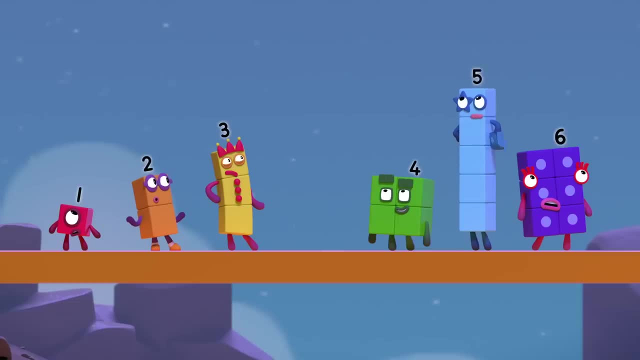 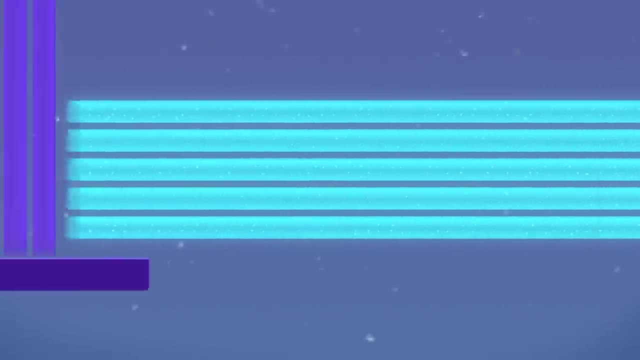 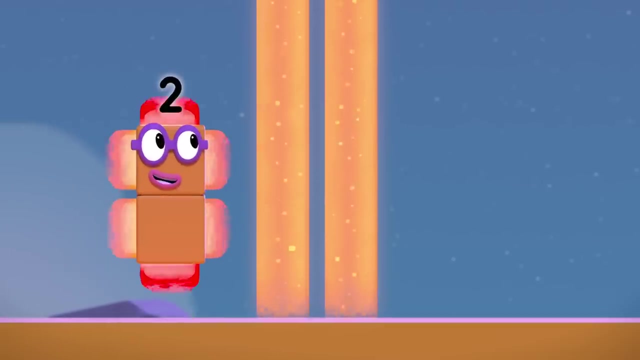 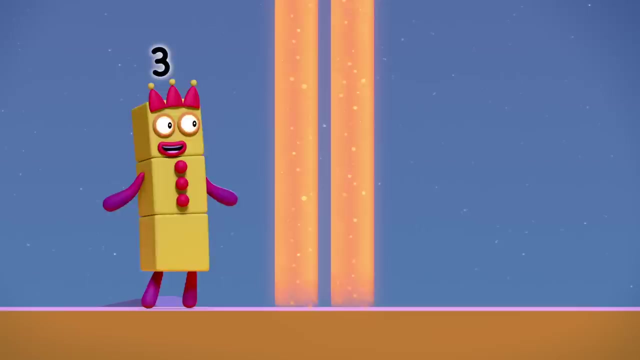 knew But how. It's too far to jump. Ride the rays, Oh Oh, How do we ride them? These are two rays, So maybe Whoa Whee Come up, It's fun, Oh Oh. 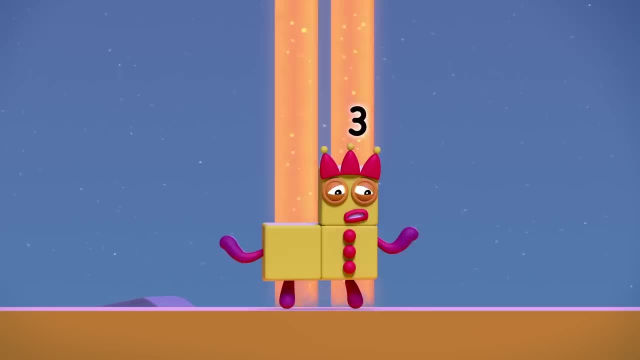 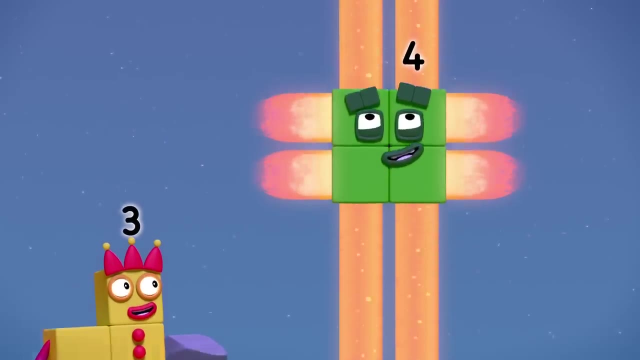 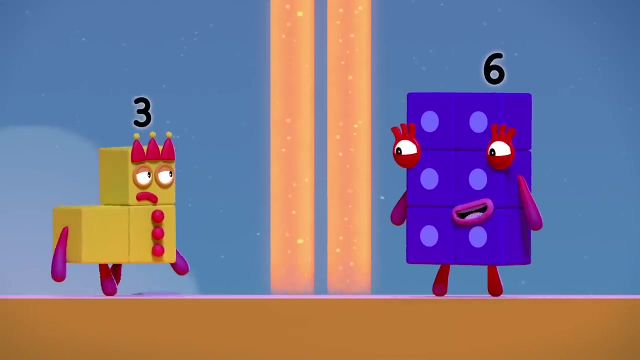 Oh, that's no use. I can't make a rectangle that's two blocks wide. No, But I can. I'm a two by two square. Whee Whee. If you think that ride is smooth, wait till you check out. 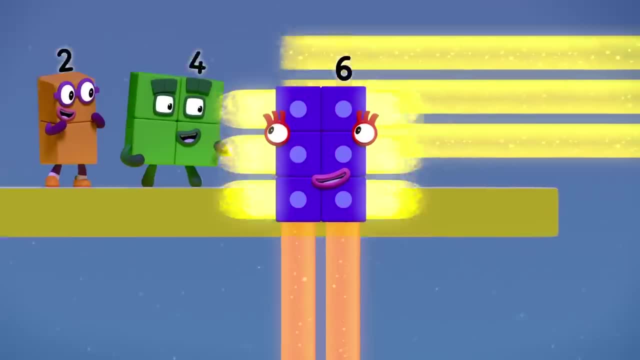 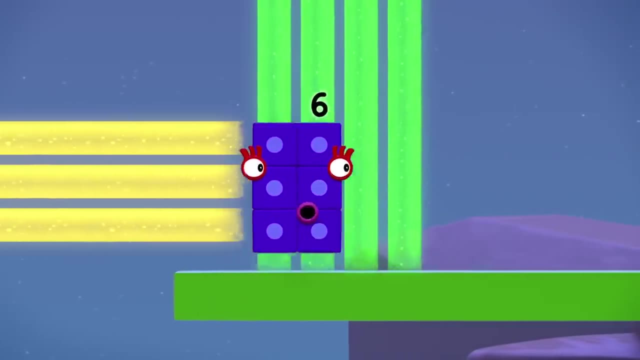 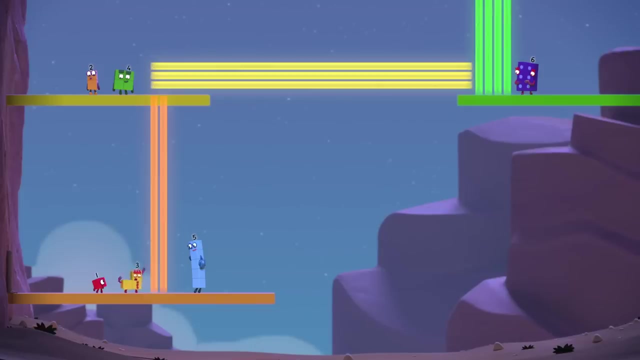 this move. Wow, I'm two, lots of three. I've got two rays and three rays. Ha, I've got three rays too. you know, I could ride across just like six if I could get up there. Odd numbers like us just can't. 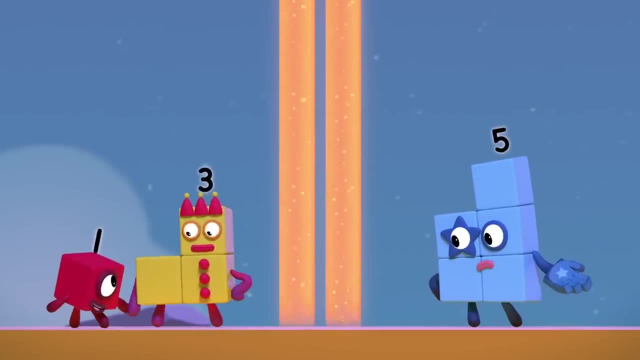 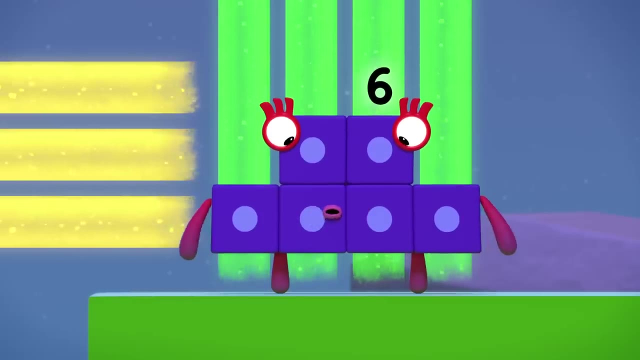 make a rectangle that's two blocks wide. Twelve said only one of us had to get to the top. remember, We can all work together to find a way. I don't see how We're out of luck. I can't make four blocks. 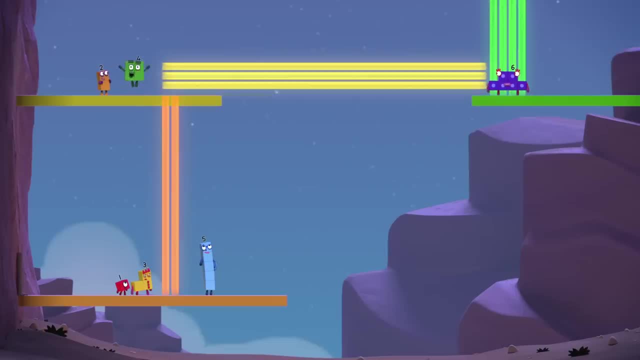 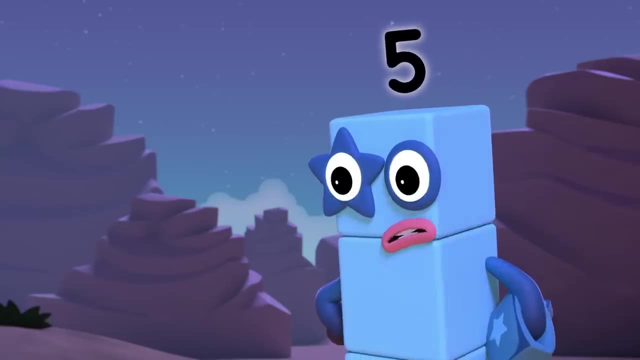 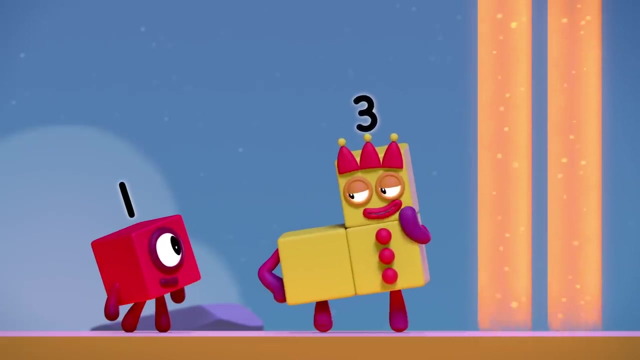 wide. I'm stuck. I can, I can, But I'm stuck here. We're all stuck. Twelve must have made a mistake. Wait a moment. Maybe there's more than one way to solve this problem. Sometimes you need to think round corners. 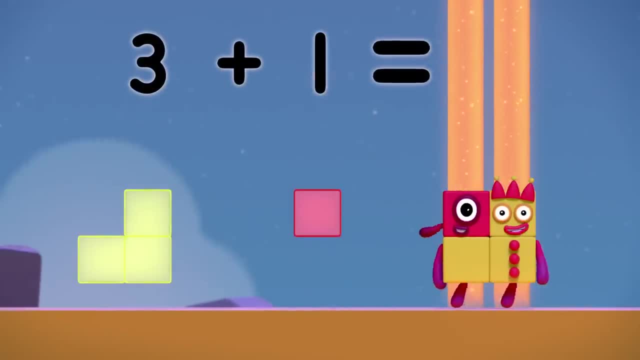 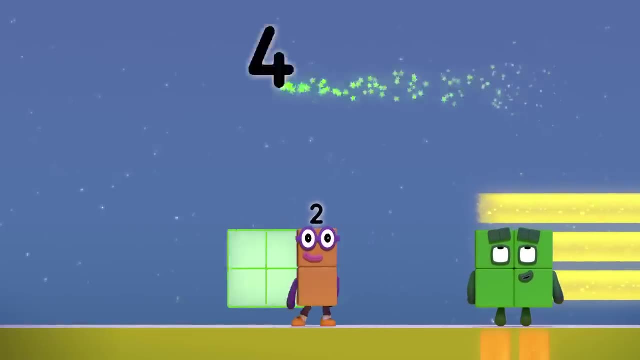 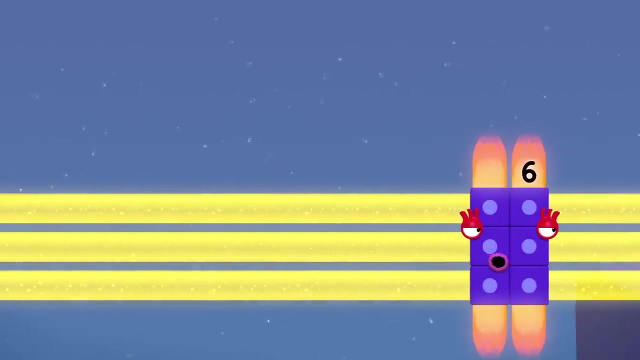 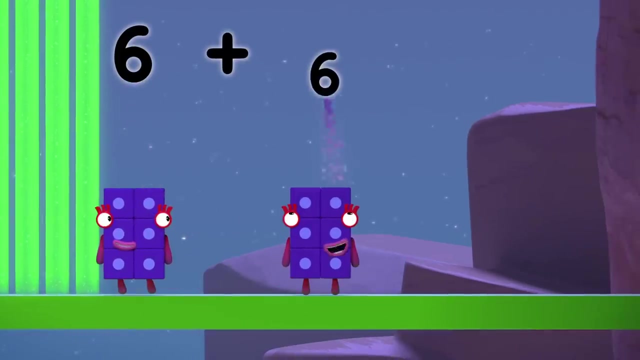 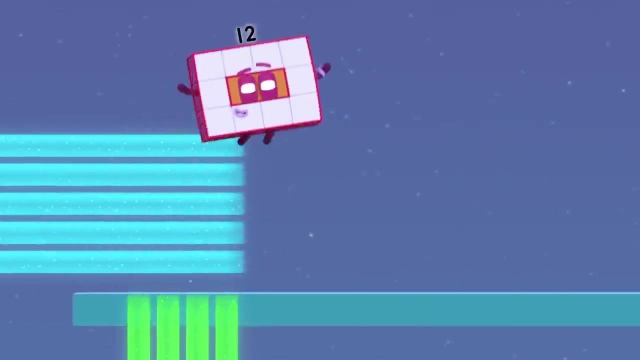 Three plus one equals four. Four plus two equals six. I'm so glad I can reach this shelf, So happy I'm beside myself. Six plus six equals twelve. Oh, well done. Who came up with this idea? Me, me, me. 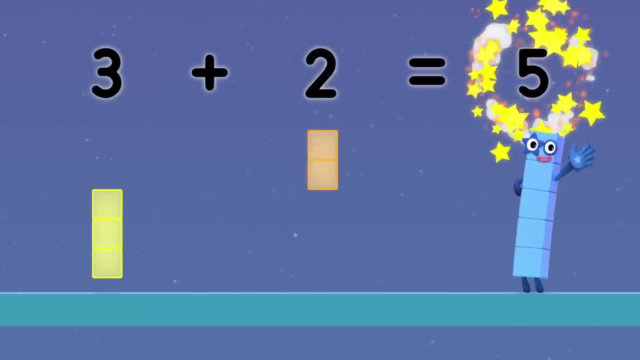 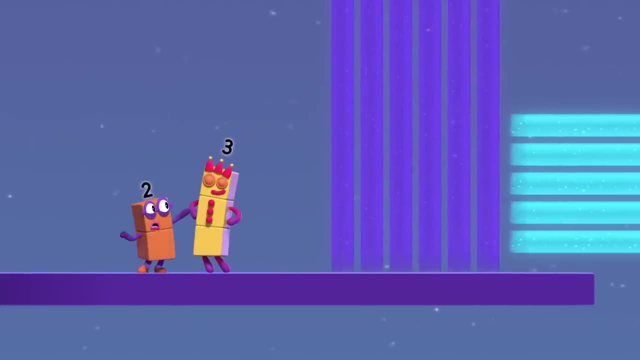 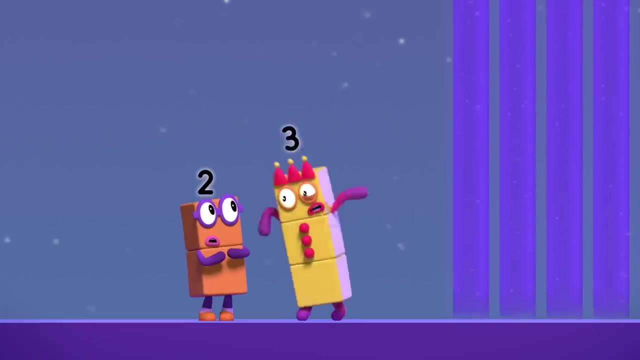 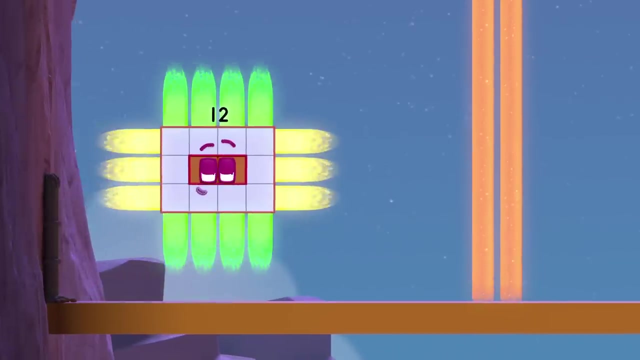 Three plus two equals five. Hooray, Yeah, Um, but how do we get up there? We can't make anything. that's six blocks wide. We've only got five blocks between us. Hello, my friends, Twelve Switch. 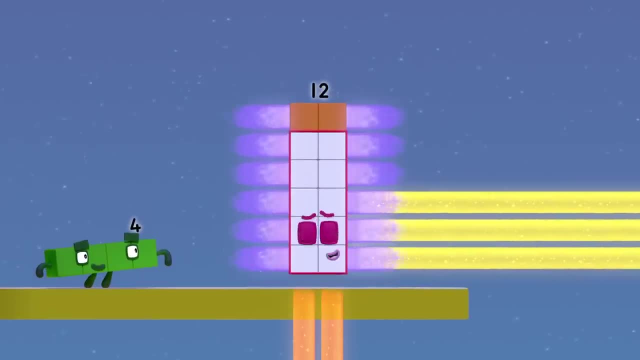 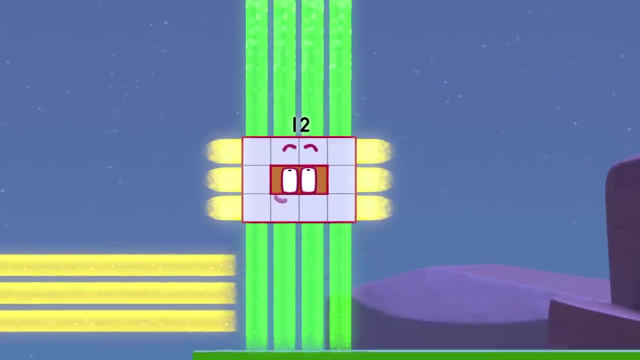 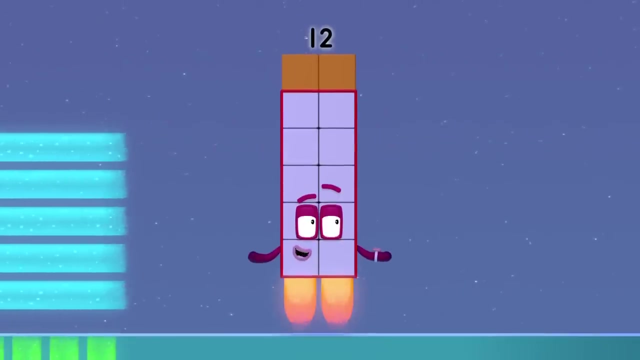 Congratulations on getting so far. Switch Four. By working together you've nearly reached the top. What a super rectangle. But not even I can make every size of rectangle. I can't make a rectangle that's five blocks tall. Three. 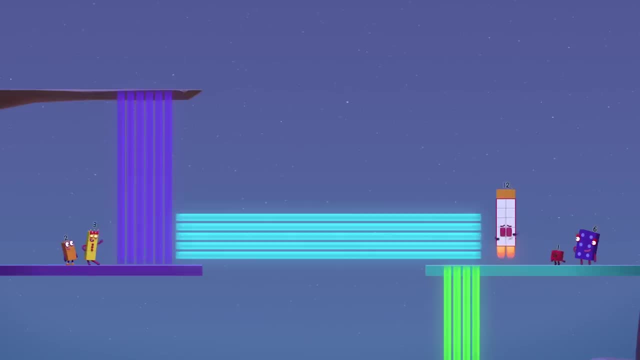 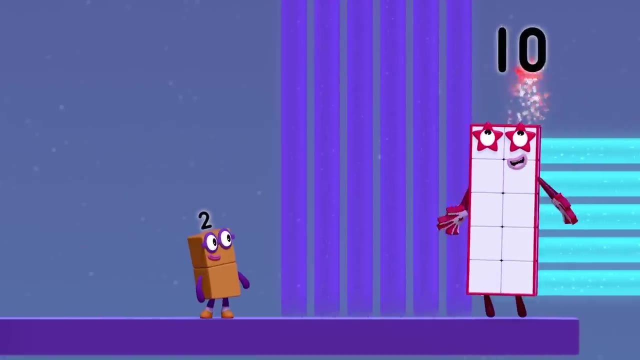 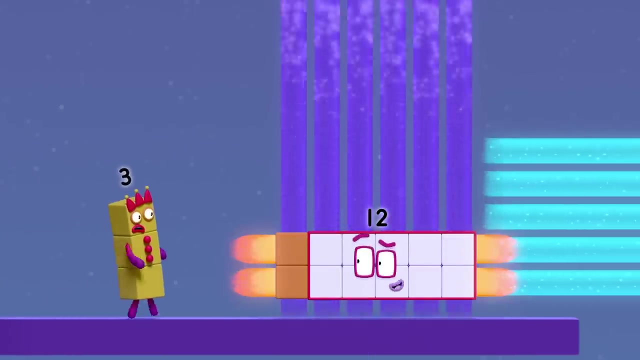 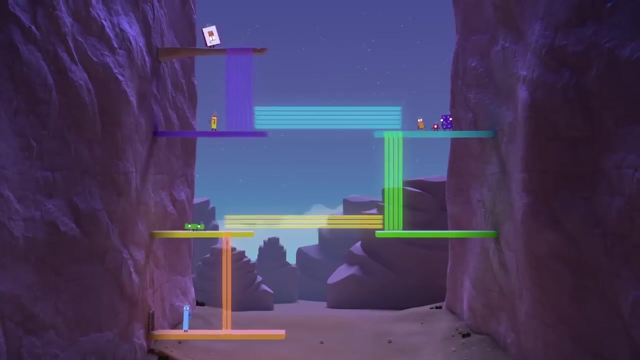 But, like you said, Three. sometimes there's more than one way to solve a problem. Twelve is ten plus two. Ten plus two equals twelve Ten. I'll drop you a line. What does that mean? I'll drop four. Oh, 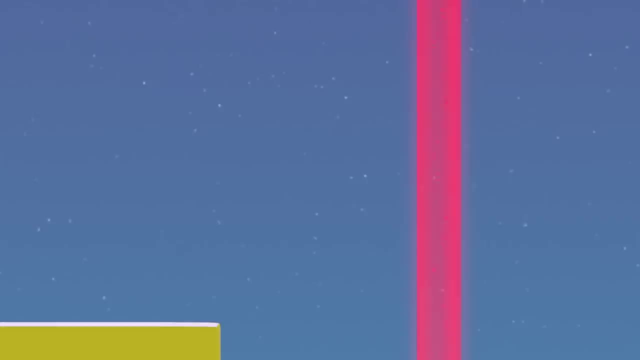 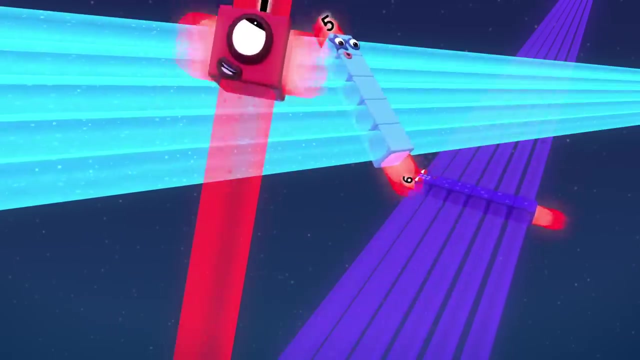 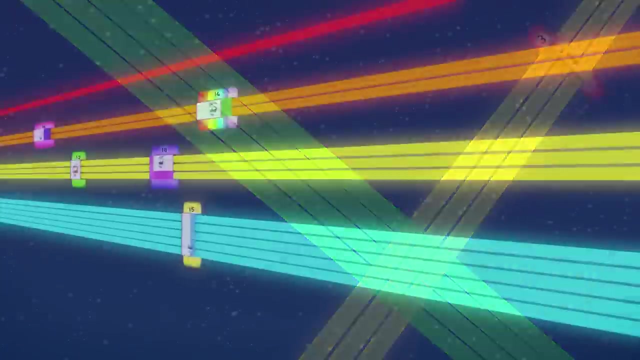 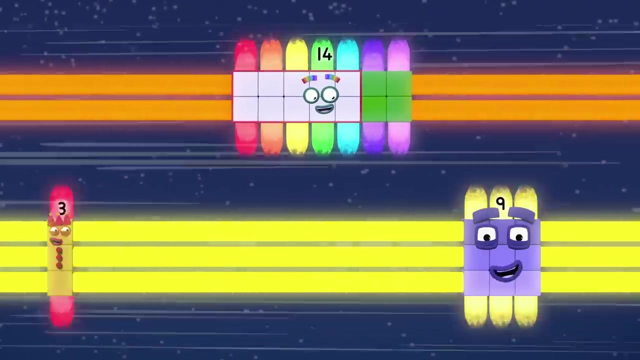 Ten plus two equals three. Ten plus two equals five, Three. Oh, I've got an idea What. What The seasons have gone so fast. We've been doing this for a long long time. Eighteen makes the scene. You think this is fast? 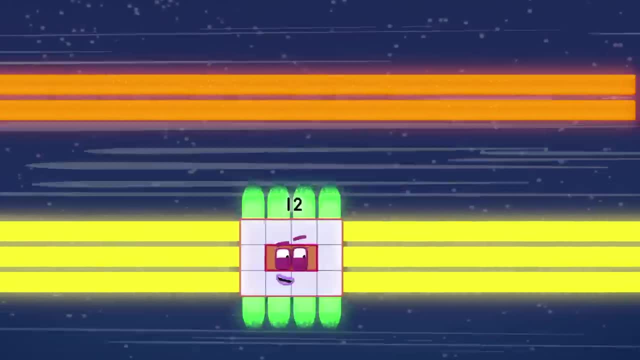 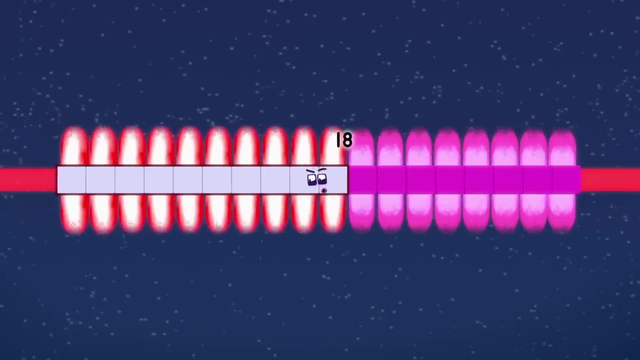 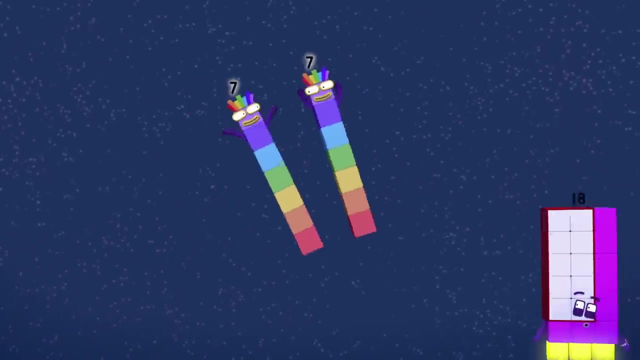 Follow me for some real speed. Woo-hoo, Yes, Whoa, Woo-hoo, Whee. Are you fast enough to loop the loop? Go, go, go, Go, Woo-hoo. Awesome, Let's do it again. 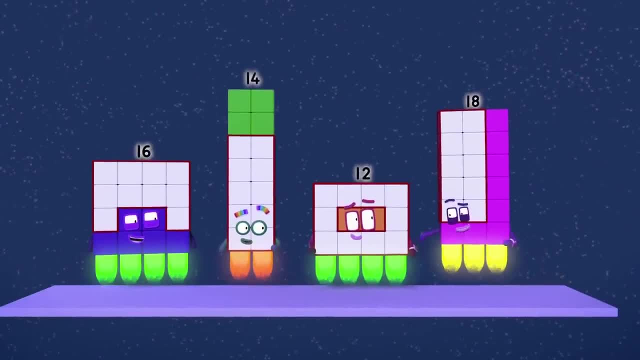 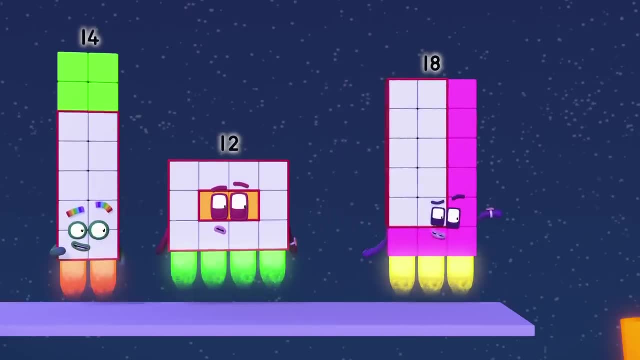 Woo-hoo Ha, Anyone can ride that thing. Check this out. Whoa, The double looper has a two-ray mateys, So you can only ride it if you can make a rectangle that's two blocks wide, Like this. 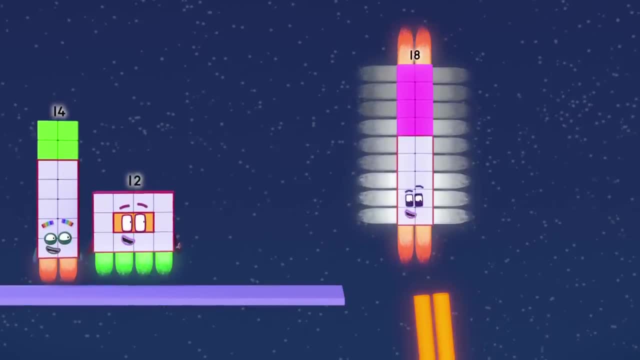 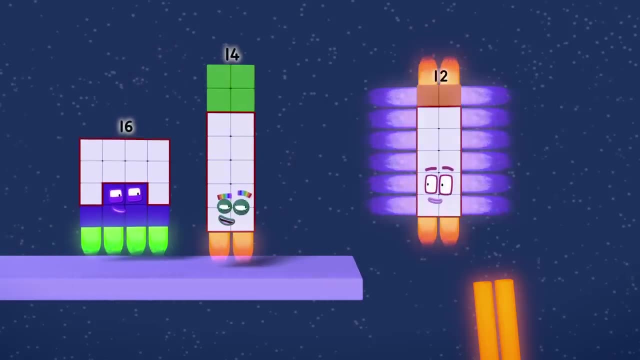 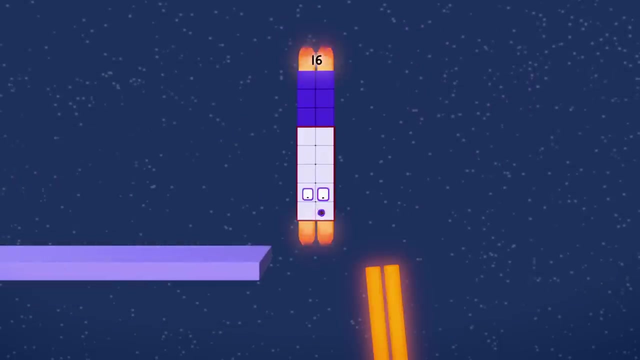 Two by nine, Two rays and away. One, Two, Woo-hoo Land. Two by six, Whoa. Two by seven, Double lucky, Double seven, Hey-hey. Two by eight, Yay, Woo-hoo. 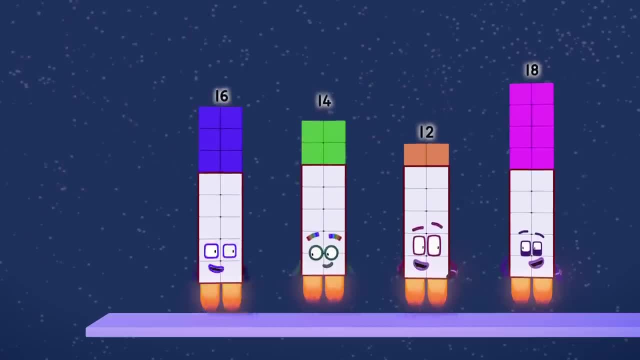 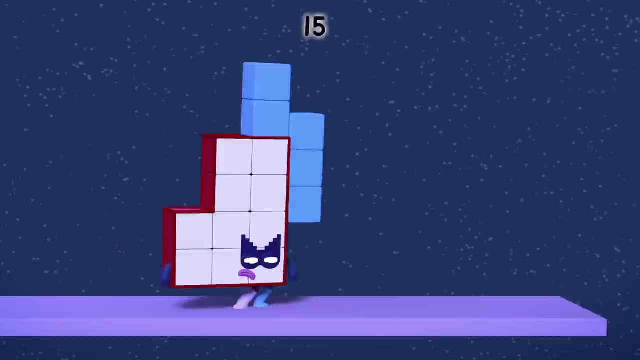 Woo-hoo, Woo-hoo, Woo-hoo. Ah, That does look like fun, But odd numbers like me can't make a rectangle two blocks wide. See, Don't let that slow you down. Fifteen: This next one could be made for you. 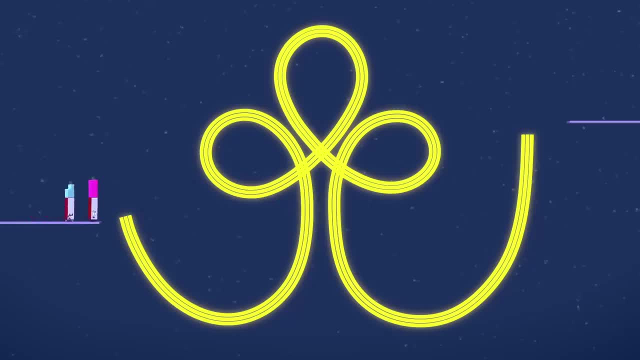 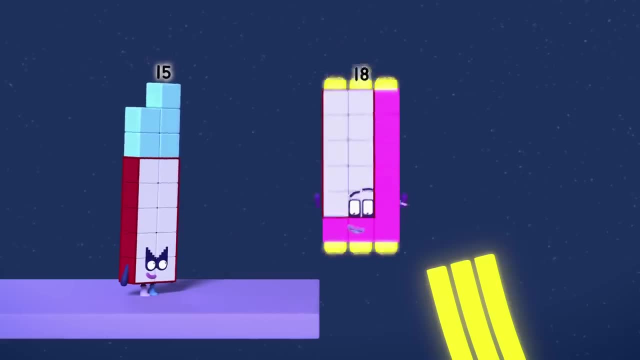 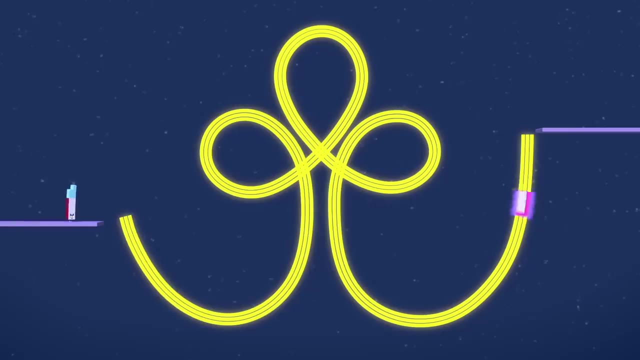 A triple looper with three rays, So you need to make a rectangle that's three blocks wide, Like this. Three by six, Three rays and away. Three by six, Woo-hoo Land again, Now that I can do. 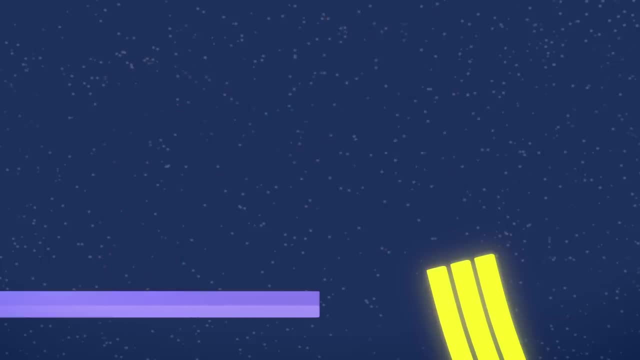 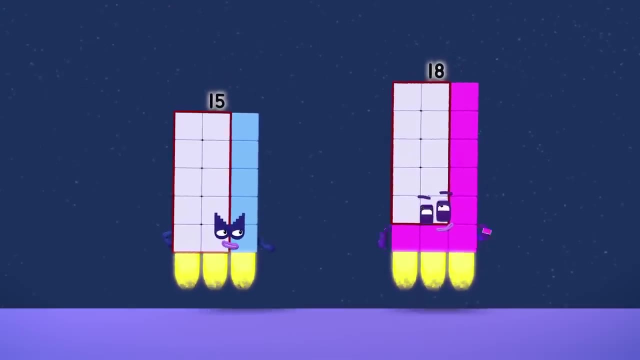 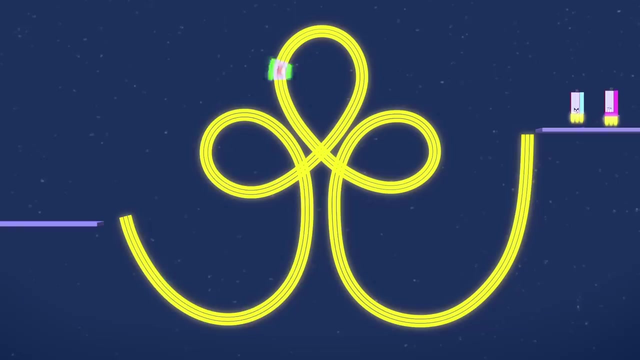 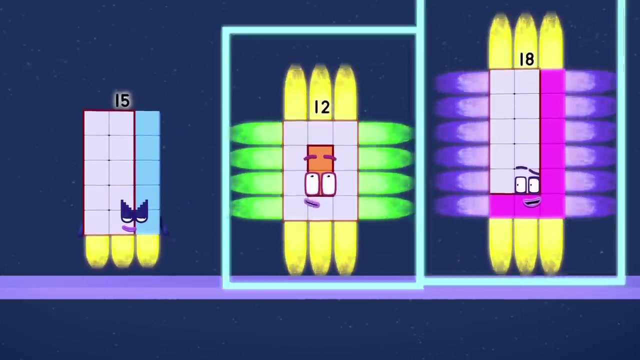 Three by five, Ha-ha-ha-ha. Three by five. Amazing, You're built for speed. Eighteen, You can ride loopers and double loopers and triple loopers. Three by four. Ha, That's because my brother and I are both super rectangles. 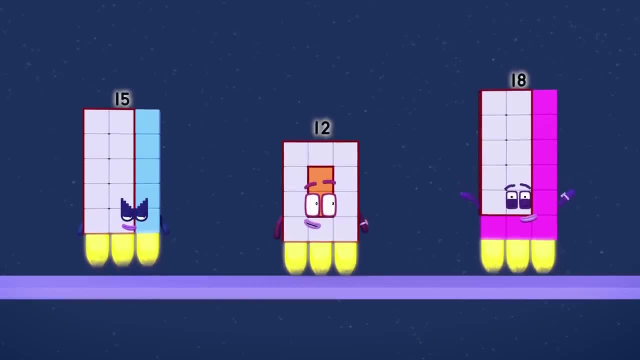 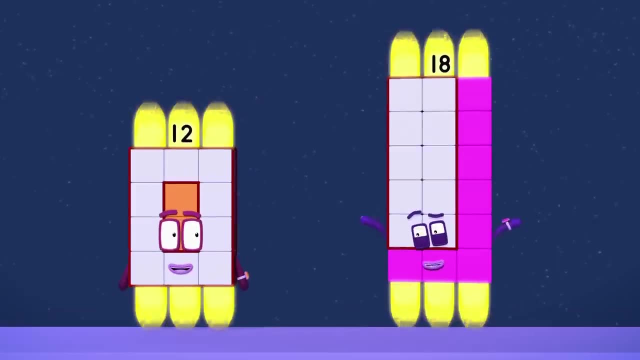 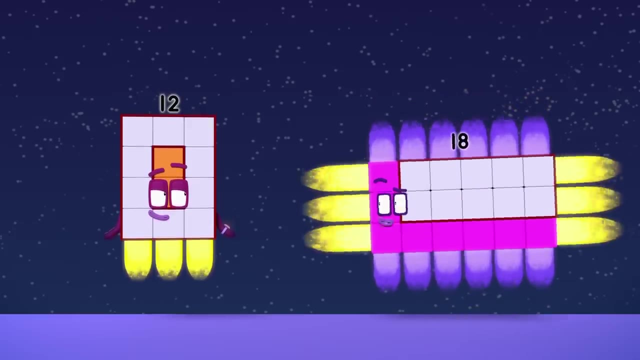 Which means we can make lots of different rectangles. So we can make one rays And two rays And three rays, And that's not all. We can both make six rays, Six by three. Well, yes, that's true. 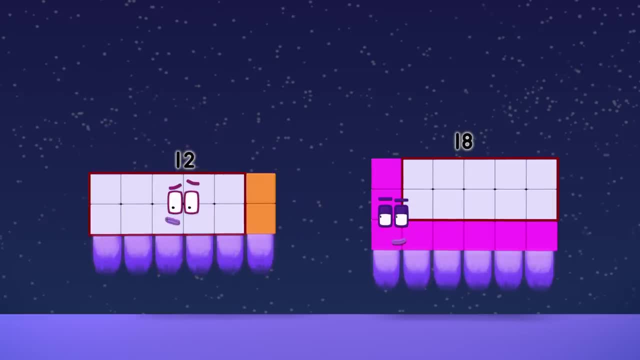 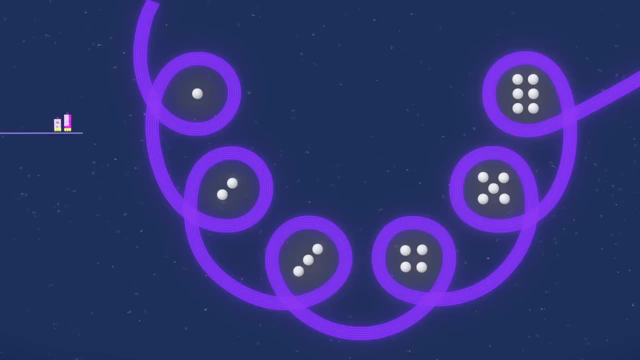 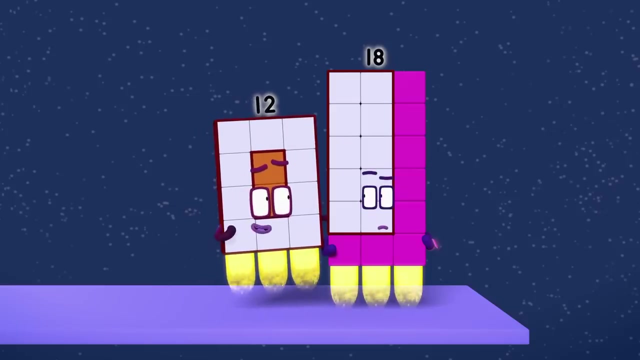 Six by two. But why do we need six rays, Unless There's a six-looper? Oh no, How do we get up there? Relax, Let me handle this. I am Twelve. I am a super rectangle Master of the rays. 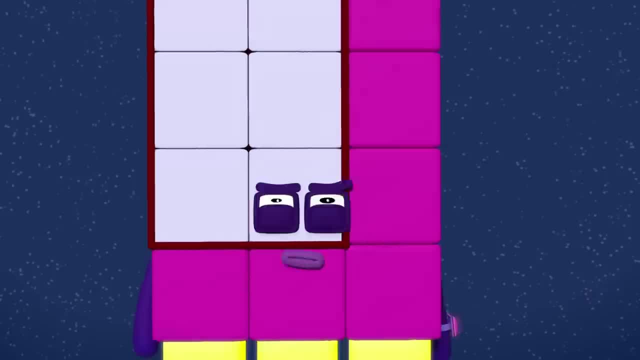 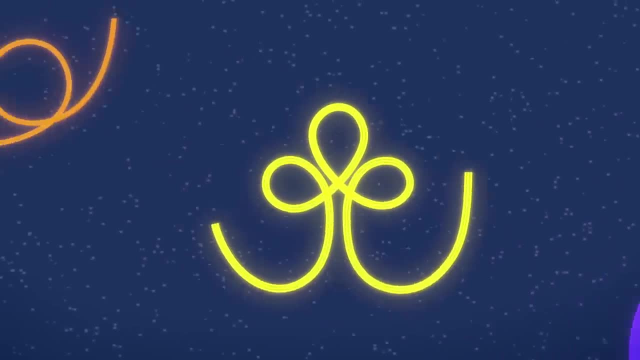 Oh, Oh, Oh, Oh Wait, Can you do that again? Behold The Super Dooper Looper, Go, go, go, go. Switch. One by Eighteen, Huh, One by Twelve. Wow, Nice. 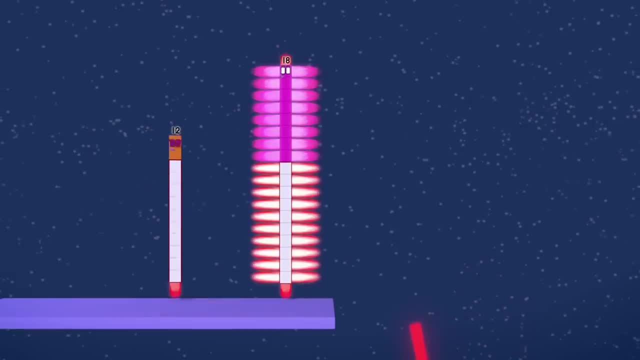 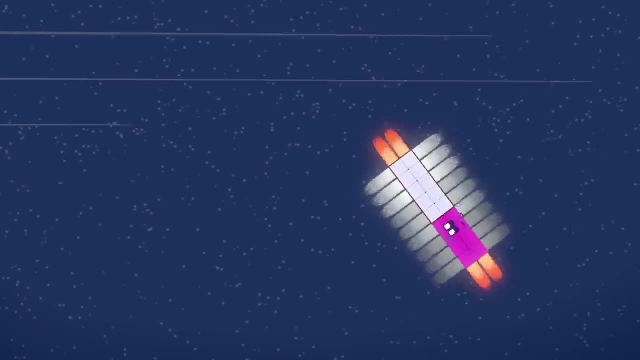 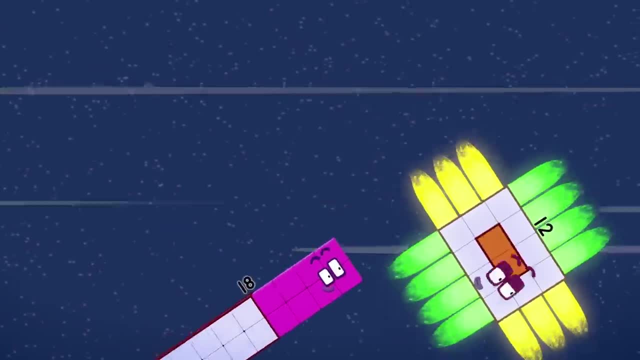 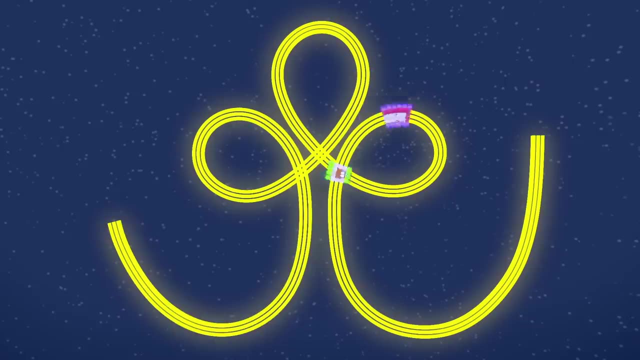 Switch Three by Four. Fast work, sis Race on Three by Six, Woo-hoo, Yeah, Whoa, Whoa, Whoa, Whoa. Six by Three, See ya. Switch Six by Two, Whoa. 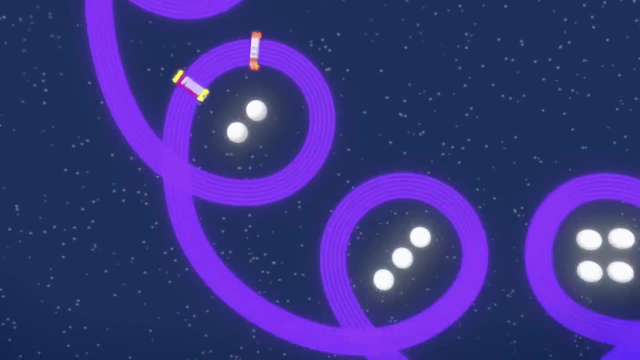 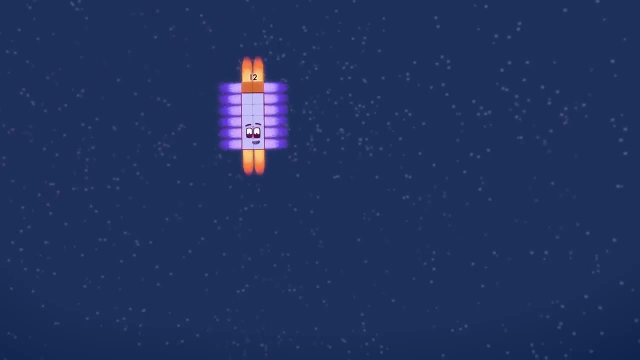 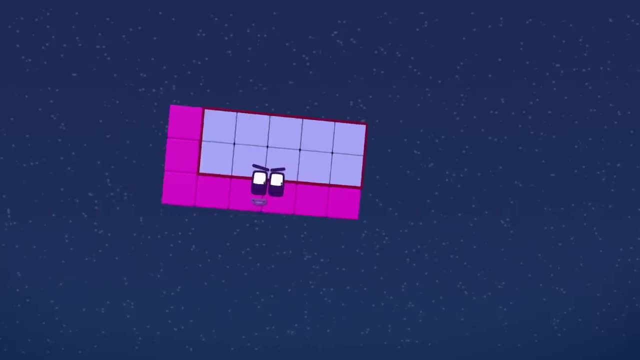 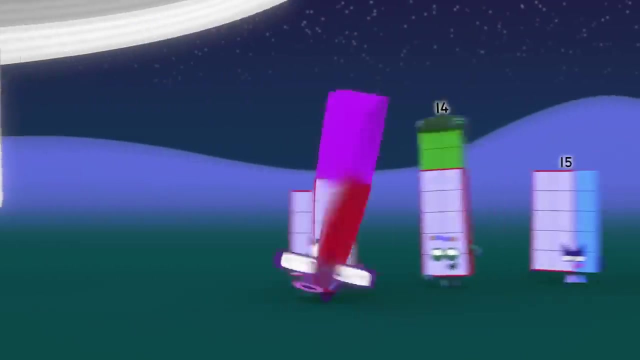 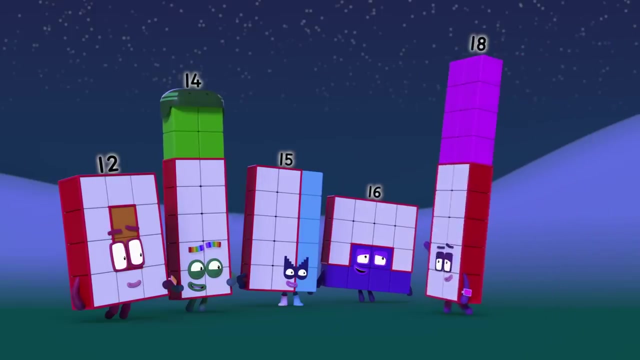 Here comes the Nine Looper, Nine by Two Coming through: Whoa, Whoa, Whoa, Whoa, Whoa, Whoa Whoa. Extreme: Whoa, Whoa, Whoa, Whoa Woo. 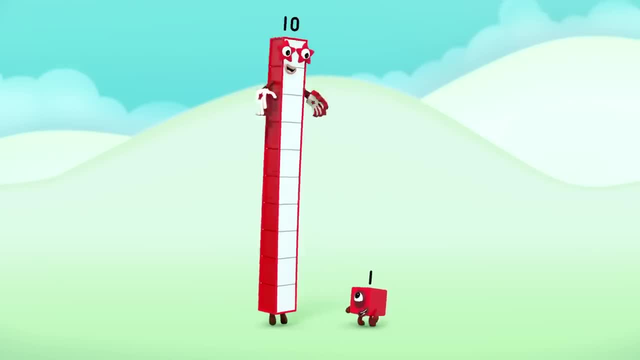 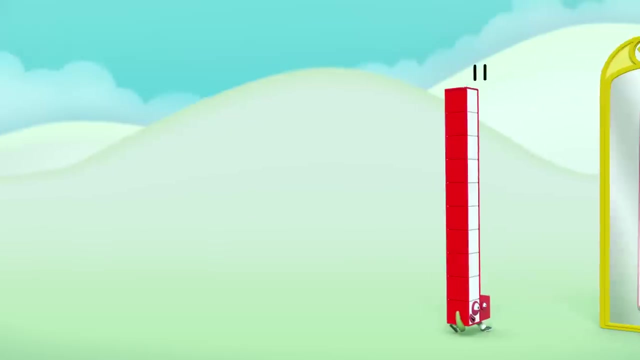 You're the extreme dude, Are you okay? Ooh, um, hmm, What was that? Who was that? A new number, block Ten plus one Equals Eleven. Hello, I'm Eleven, So am I, And I'm Ten and One. 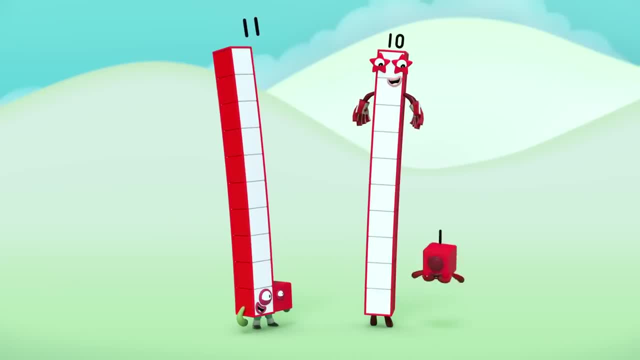 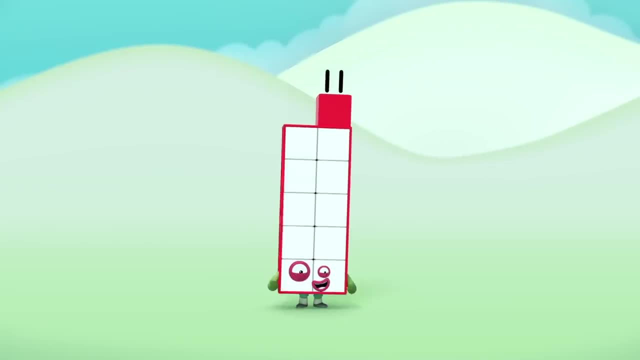 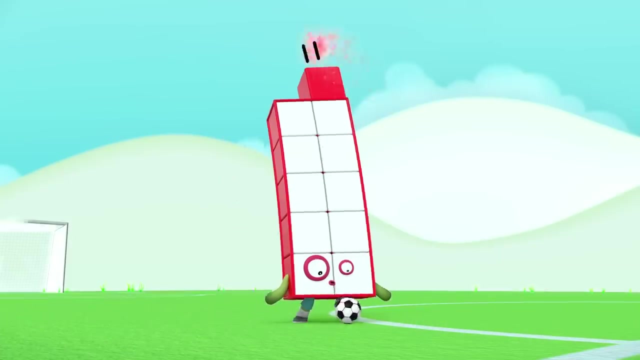 That's better, Whoa. One, two, three, four, five, six, seven, eight, nine and ten, And one more is Eleven. I am Eleven And I know how to play. I'm Eleven And I'm Ten. 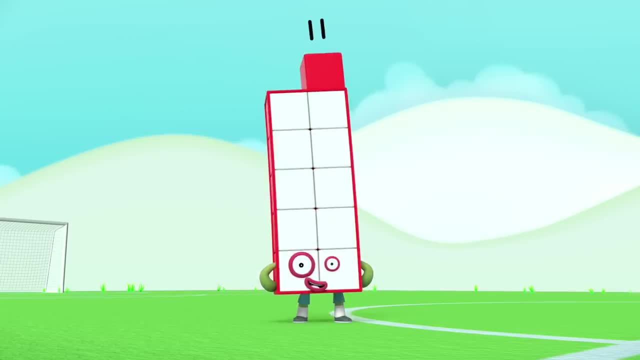 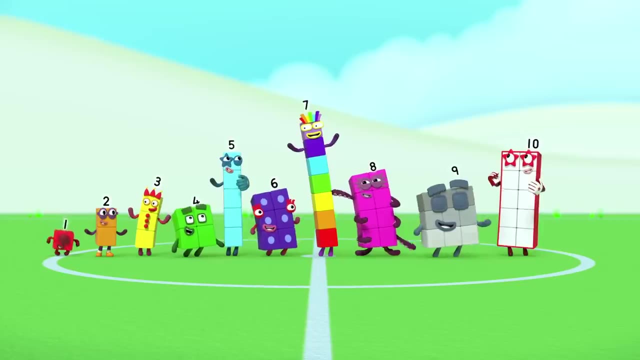 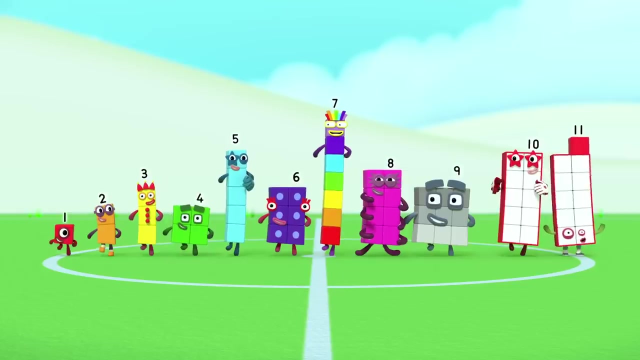 And I know how to play, And I know how to play. I love football. Wow, Let's play football, Hooray. One, two, three, four, five, six, seven, eight, nine and ten, And one more is Eleven. 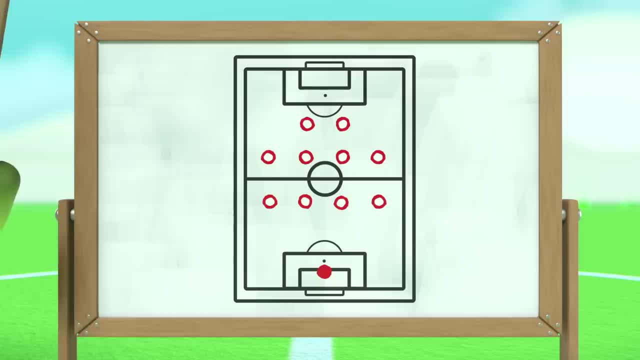 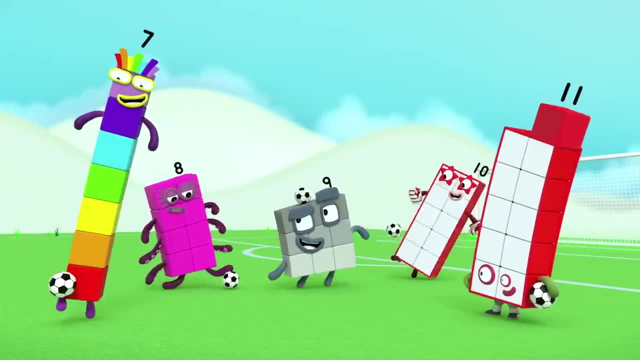 We're on our way to victory. We're on a roll With ten on the pitch and one in goal. We will never be denied. We'll take it in our pride With ten and one, ten and one Eleven on our side. 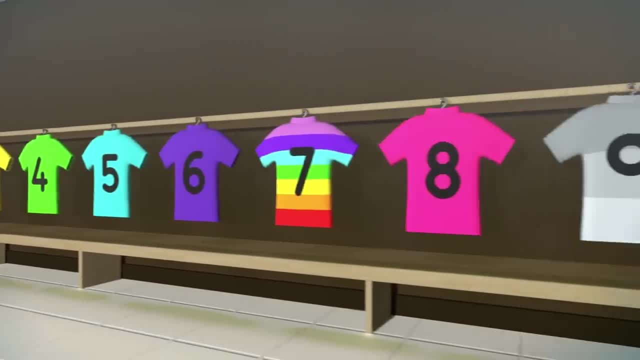 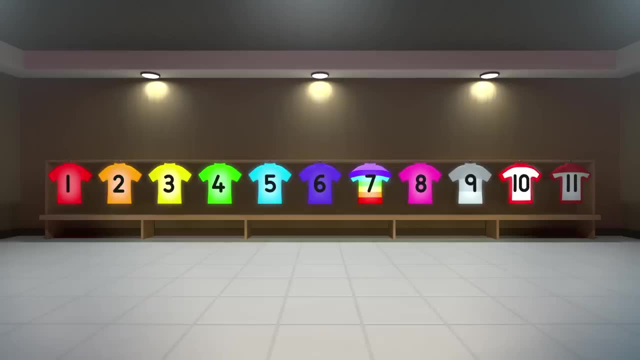 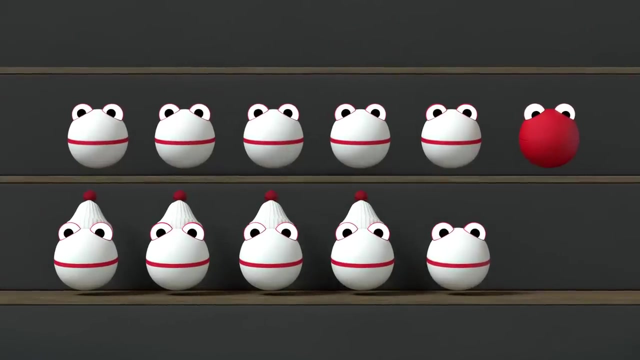 Football shirts. Football shirts, One for every number. block Football shirts: One, two, three, four, five, six, seven, eight, nine and ten, And one more is Eleven. Hooray Bubble hats. Bubble hats. 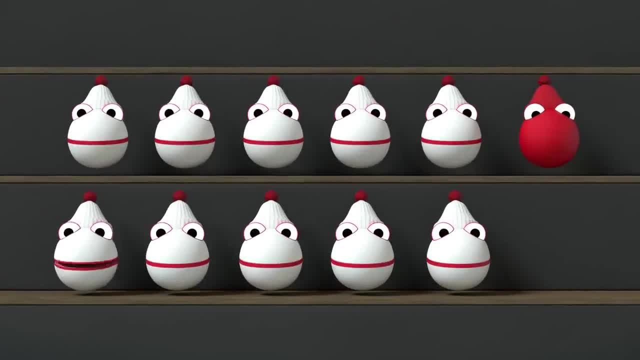 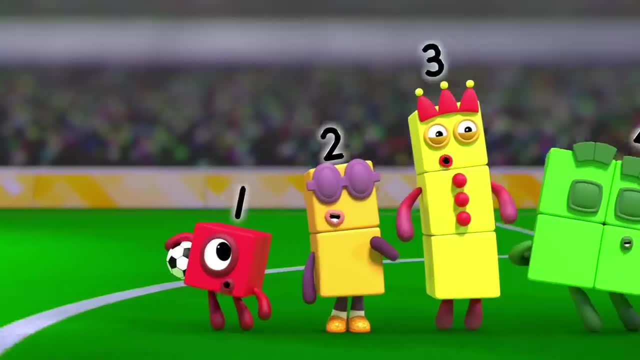 One for every number: block Bubble hats: One, two, three, four, five, six, seven, eight, nine and ten, And one more is Eleven. Hooray, We're on our way to victory. We're on a roll. 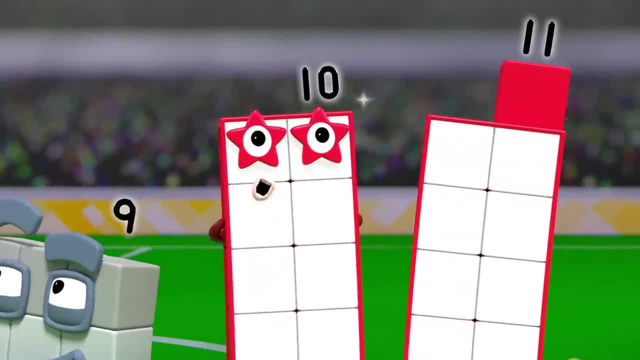 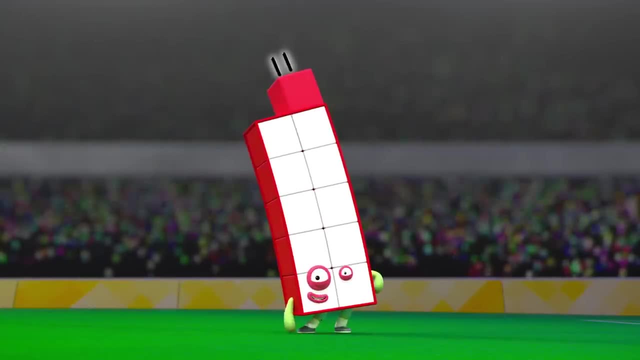 With ten on the pitch and one in goal. We will never be denied. We'll take it in our pride. With ten and one, ten and one eleven on our side, We're ten one one, ten and one eleven. 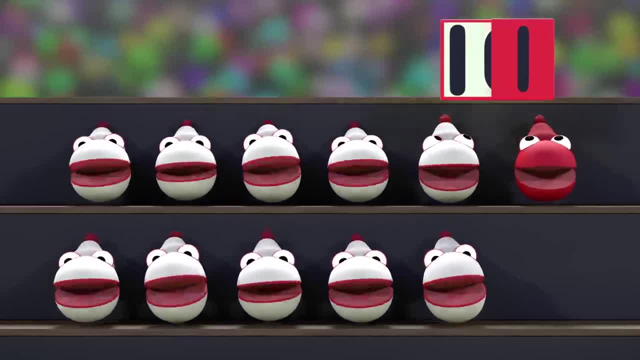 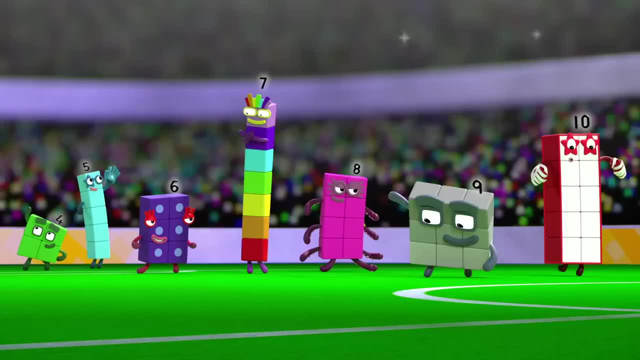 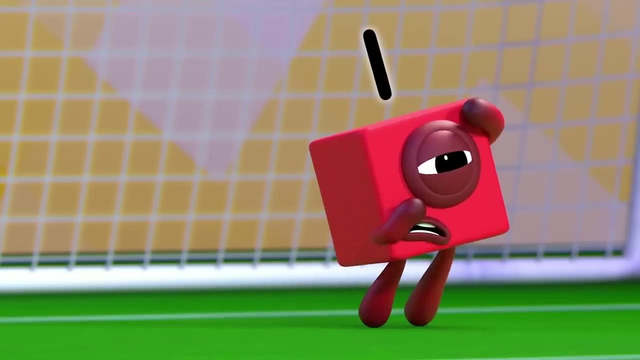 We're ten, one, one, ten and one eleven. The number blocks are out on the pitch for the big match And they're capped in 11. And 11 looks ready to lead the team to victory. Something's wrong. What can it be? 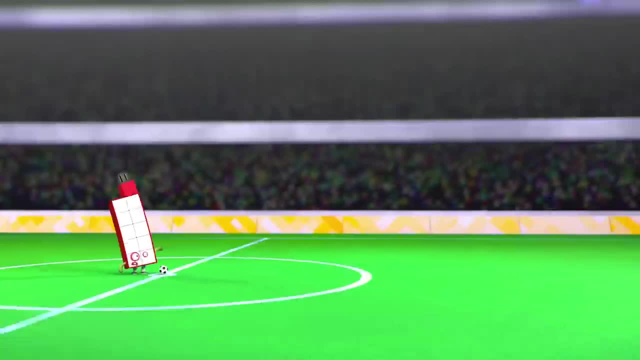 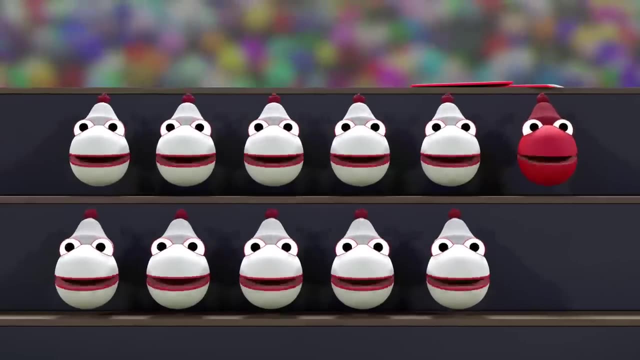 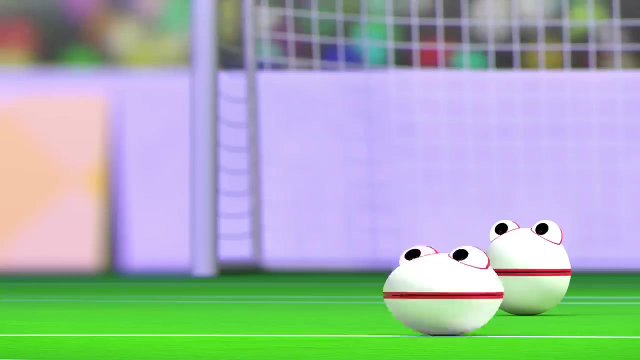 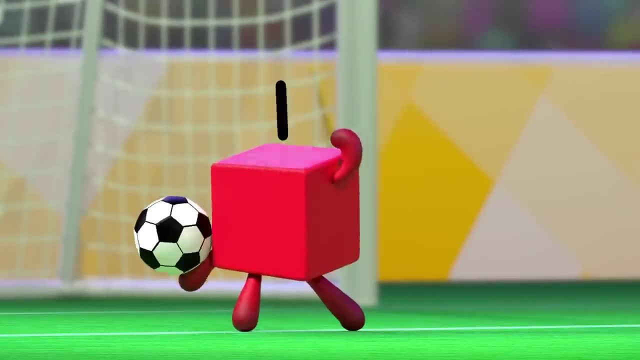 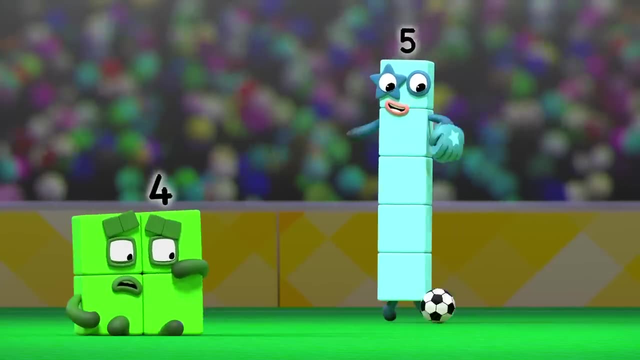 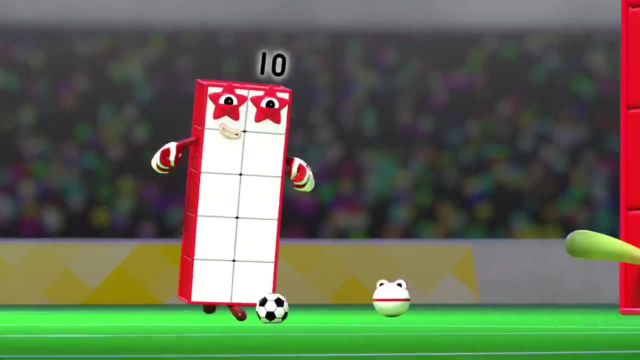 And saved by one. Take a bow one. One throws it out to two who passes it? That's right to three, four, five, six, seven, eight, nine and ten. Now pass it to 11.. 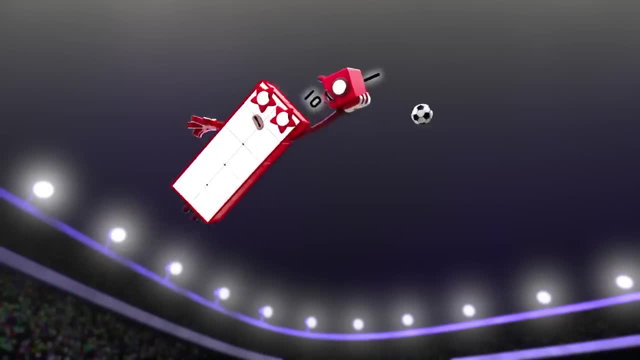 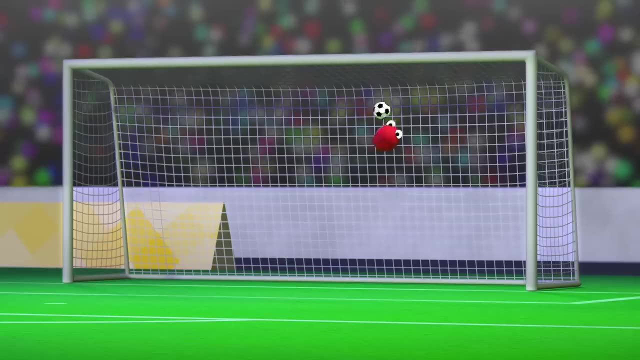 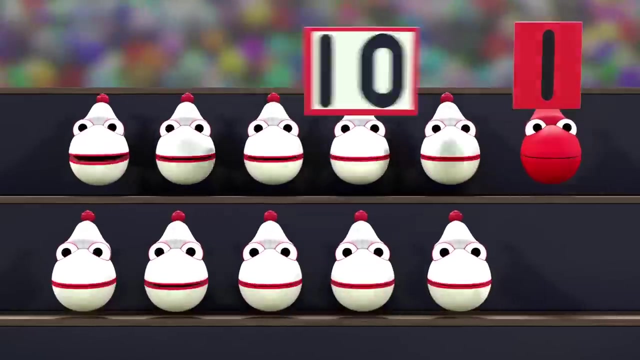 Ten passes, 11 leaps for the header and, oh my, splits into ten and one to reach the ball. Incredible, And it's a save. What a save. Cut it up to 11,. you're too louder than the rest. 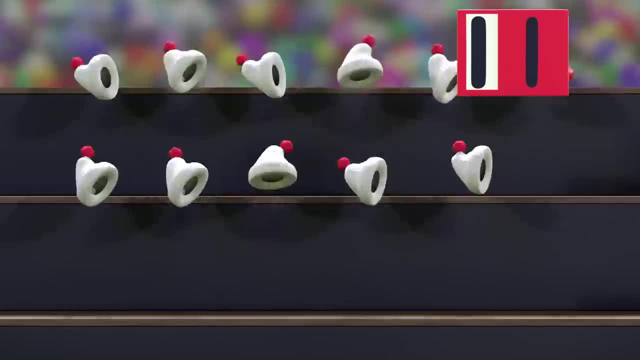 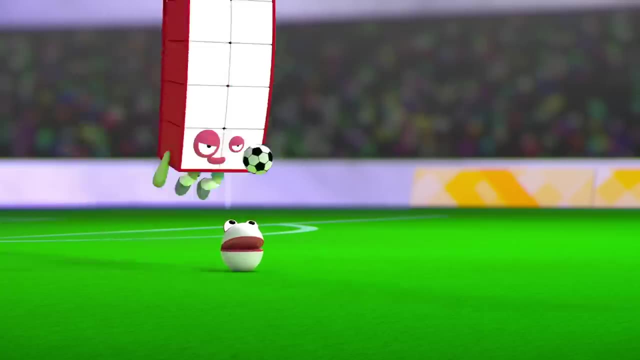 Ten and one. ten and one. 11 is the best Number blob passes to number blob. He'll find number blob And a lovely header there to number blob, Look 11.. He heads it to 11. And it's 11.. 11., 11.. Yes, We're on our way to victory. We're on the road With ten on the pitch and one in goal. We will never be denied. We'll take it in our stride With ten and one, ten and one- 11- on our side. 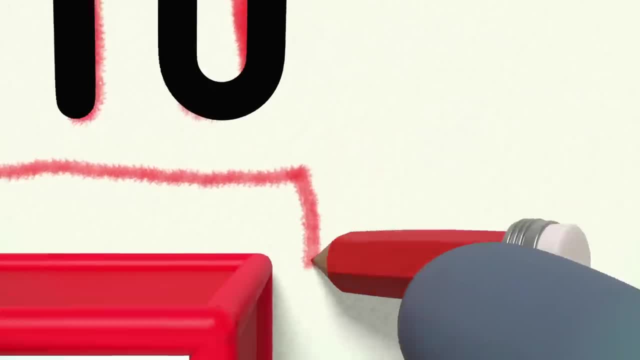 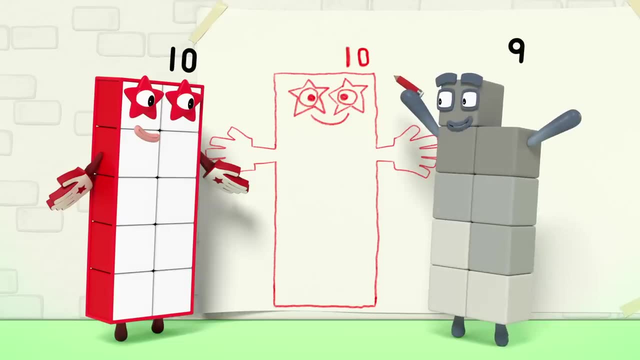 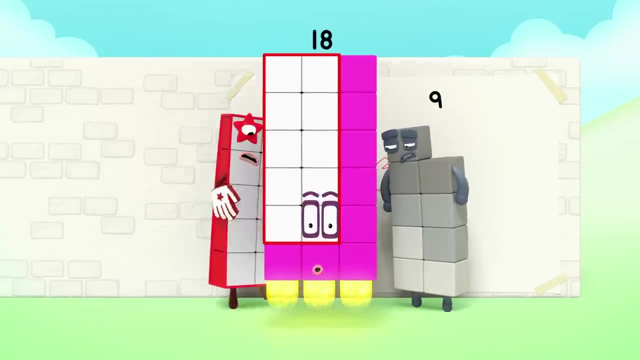 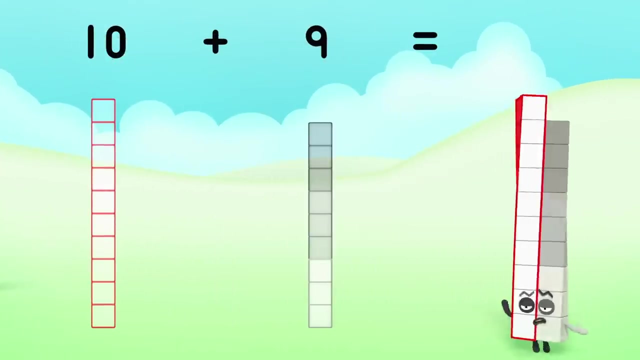 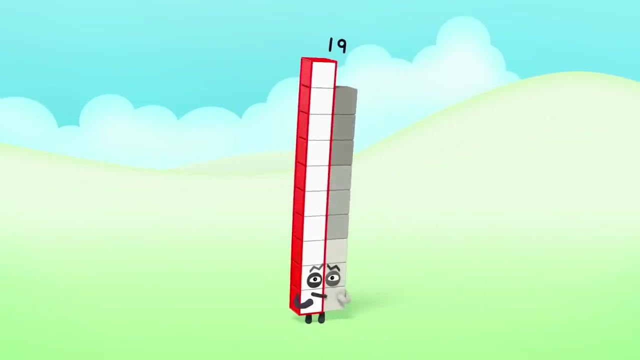 Ten and one. ten and one, 11. Um, I love it, Your turn, Super Rectangle. Whoa. Ten plus nine equals Nineteen. All right, then, I am 19.. And I, Who am I? 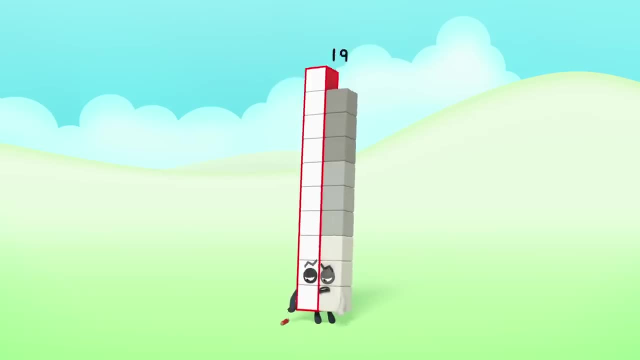 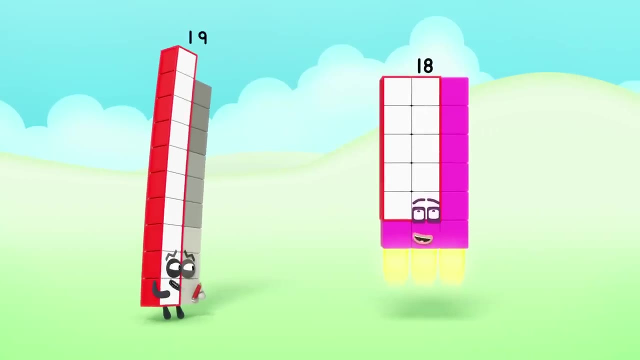 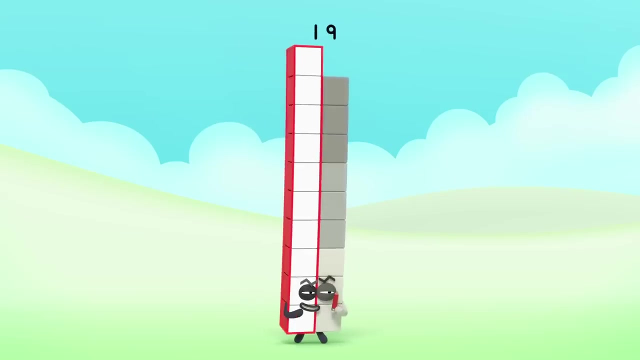 Maybe it's something to do with Super Rectangle Ha-ha Switch, Switch Turn. See ya? Ooh, maybe I can make lots of rectangles. Right, let's do this Two by Oh, Oh, silly me. 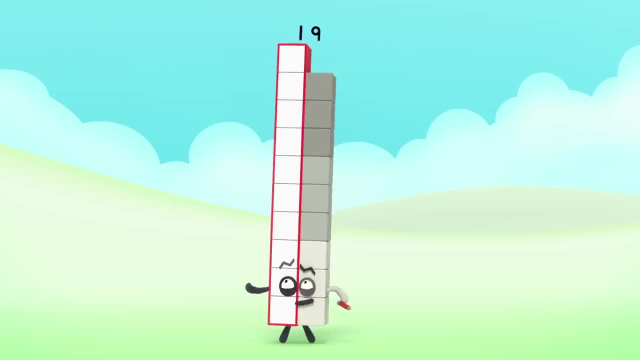 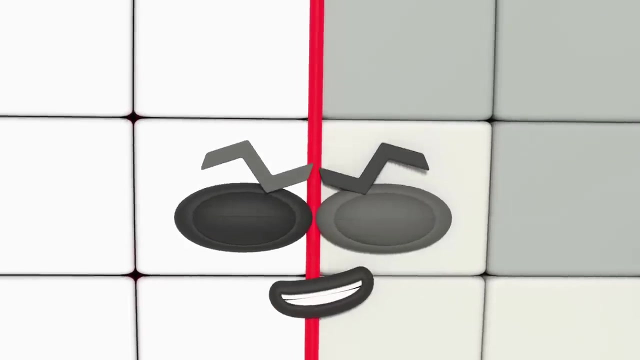 Oh silly me. Oh silly me. One block missing, Try again. Three by Ah. One block too many, Never mind. Four by Ugh. One off again. You can do this. Whoops, Not a rectangle. 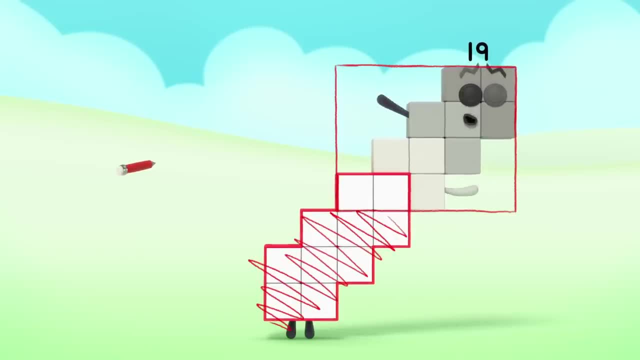 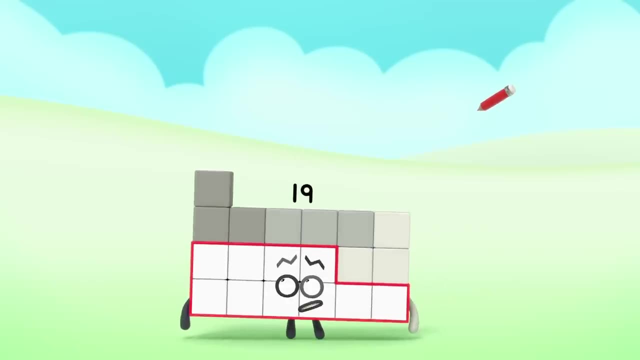 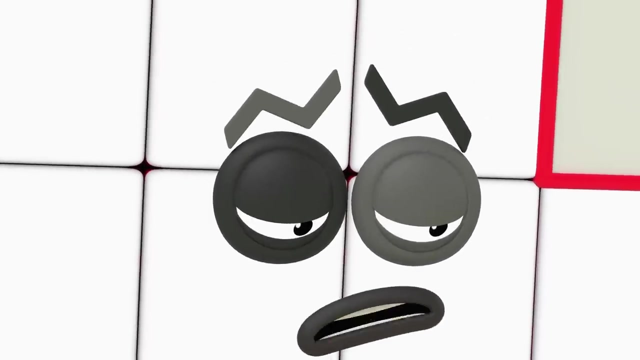 Come on 19.. Concentrate: Five by Nope One off. Six by One off. Oh, I can't do it. Oh, I'll never be a Super Rectangle, I'm just a silly old Teapot. 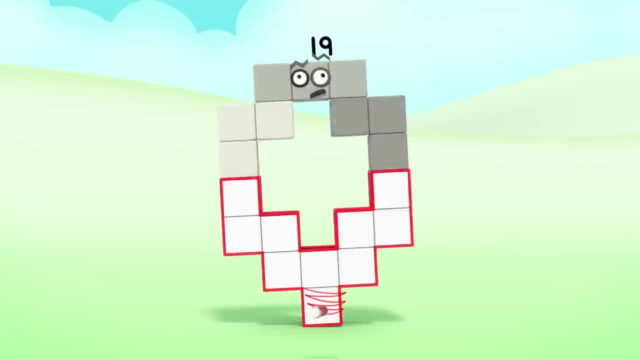 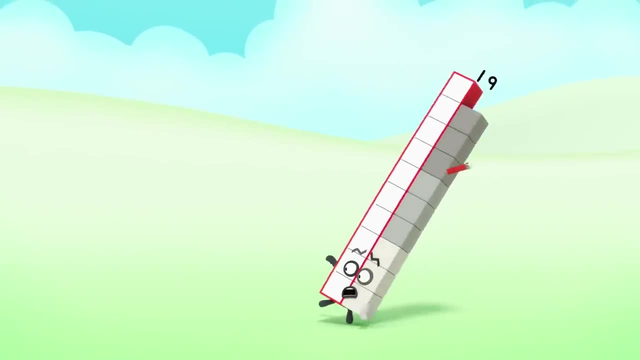 I mean Elephant, I mean Like, I mean Monster, Mmm, Super Rectangle. Ah, I wish I could be like Like 18. Make everyday shapes With neat, straight lines, But there's always something Not quite right, So I make crazy shapes. 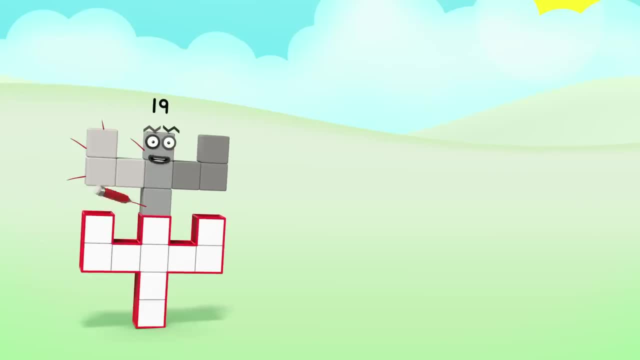 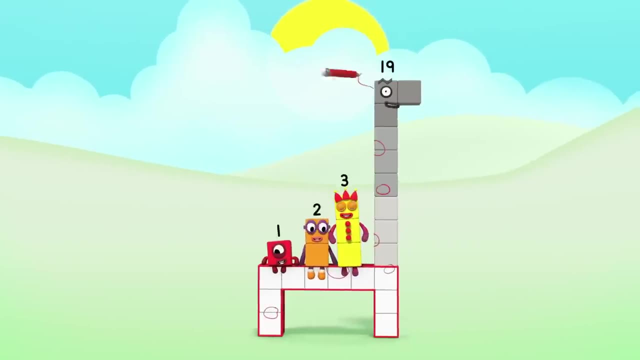 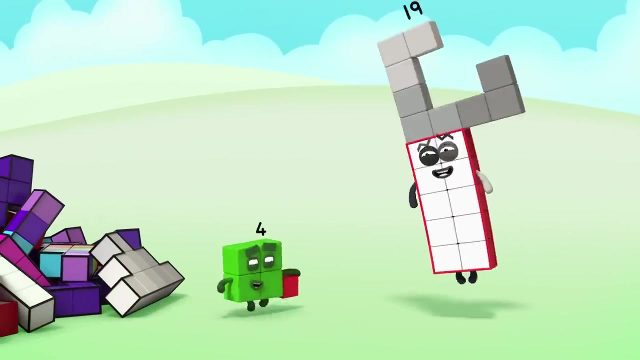 That's where 19 shines. I can be a cactus in the desert, An umbrella when it rains- Ooh. I can stretch right out To make a tall giraffe, Oh thanks. And if you need some building blocks, I can make a crane And make lots of funny faces. 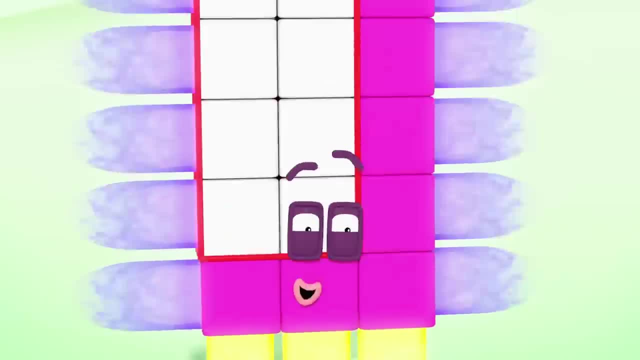 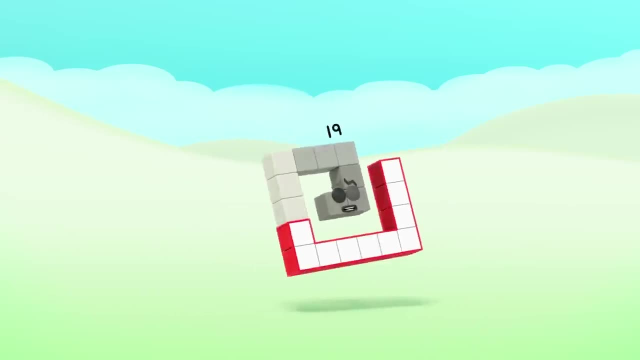 To make you laugh, Cos I make crazy shapes. Crazy shapes are what I do. Thingamabobs and whatsits And whatchamacallits too. I can make most anything. So put me to the test: Crazy shapes. crazy shapes Are the thing that I do best. 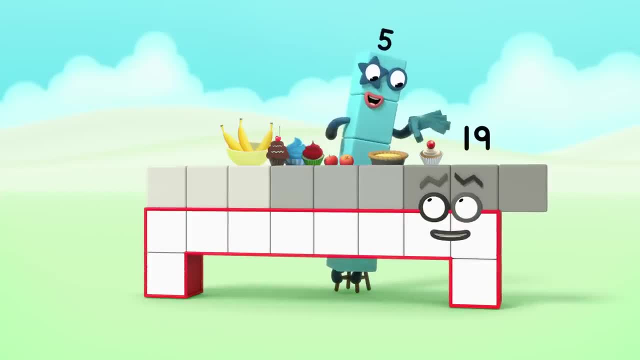 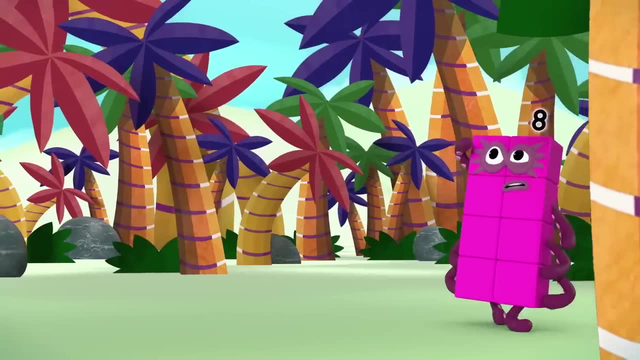 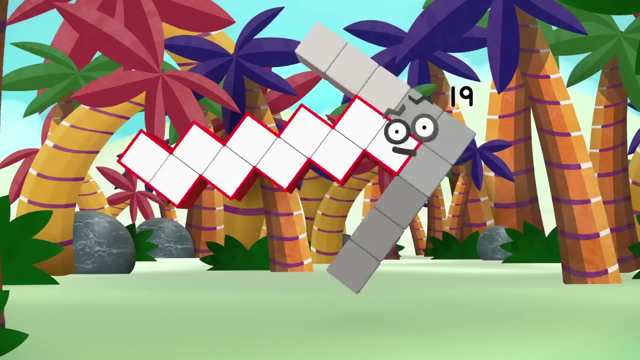 I can make a table, A table you can eat at, Or a funny kind of fish When you're digging. I can make a garden spade. When you're lost, I'll give directions With an arrow if you wish. When it comes to making wacky shapes, I've got it made. 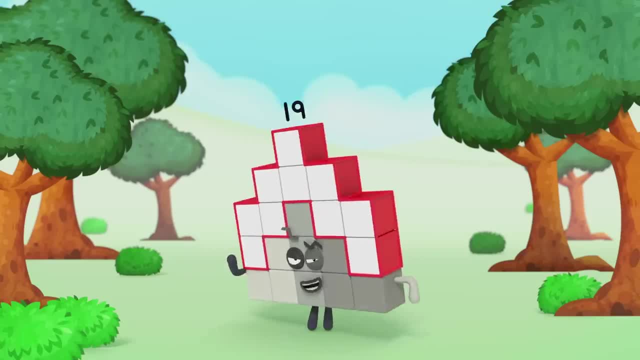 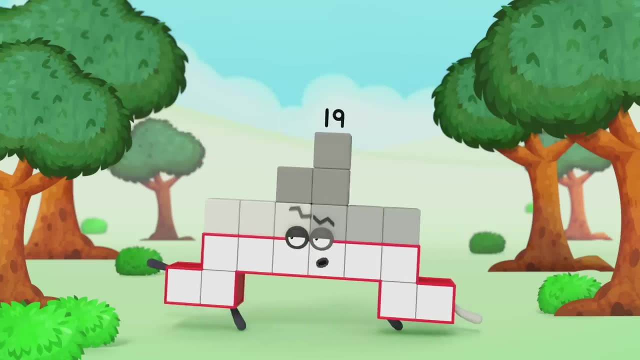 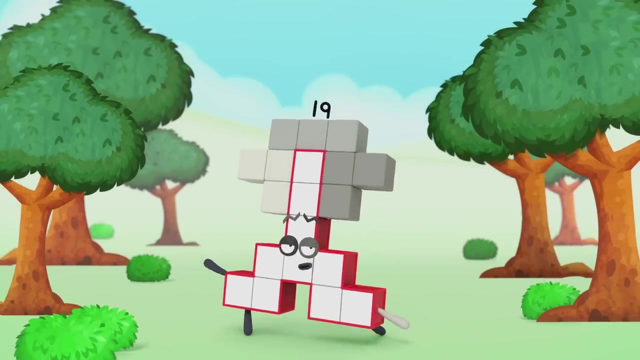 Cos I make crazy shapes. Crazy shapes are what I do: Thingamabobs and whatsits And whatchamacallits too. I can make most anything. So put me to the test: Crazy shapes. crazy shapes Are the thing that I do best. Oops, I'm a one-off.